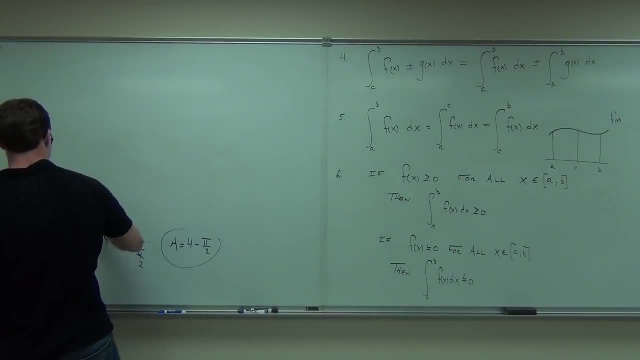 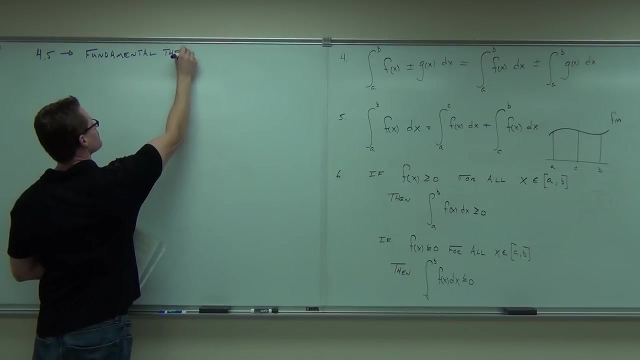 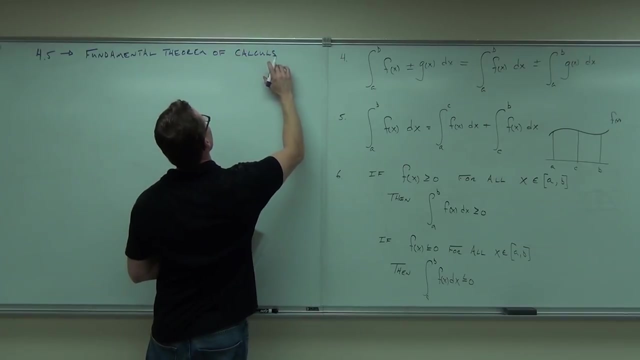 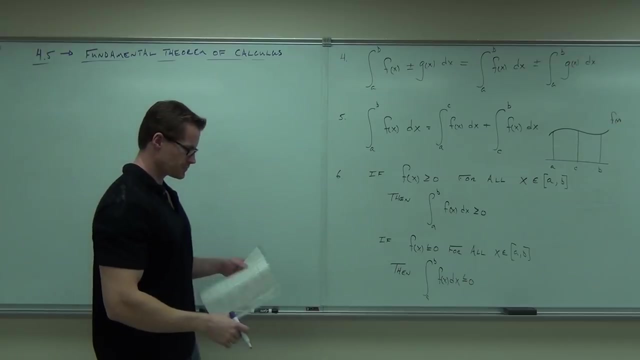 and calculus. When I go to the gym to get my pump done, I just go derivative. No, that's not true. I think of that kid that you picked up. That's good. All semester they're just looking at you with your other companies. 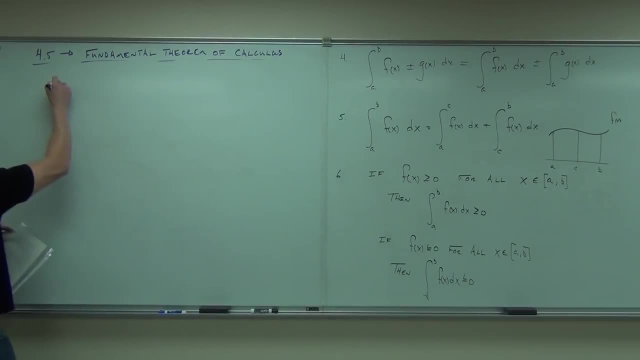 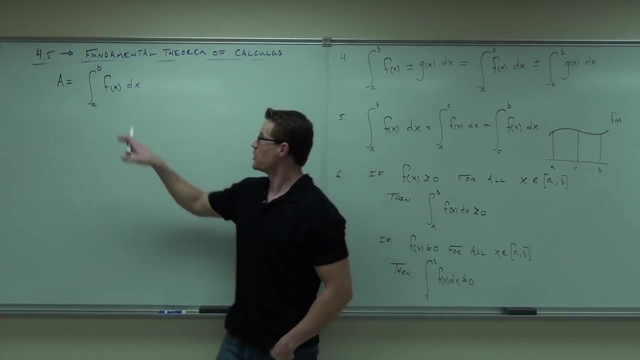 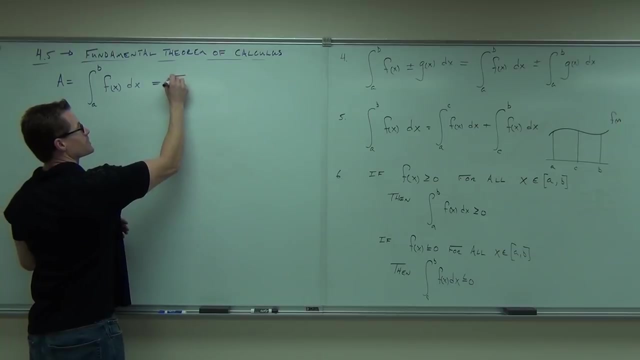 Yeah, basically Here's what you know so far. You know that this is an area. You also know how to calculate indefinite integrals. You know how to calculate them like this: that this was capital F of X plus C. Remember the plus C part. all doing that, We know how to do integrals. We've done. 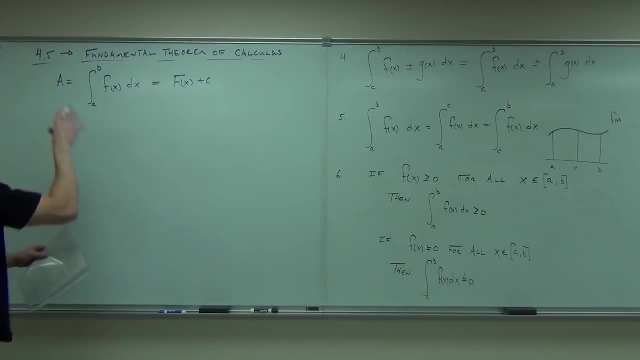 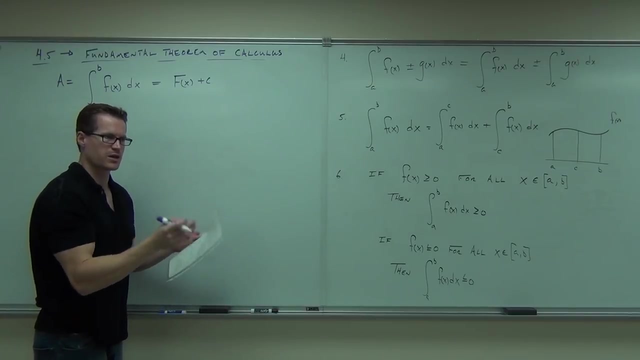 that already. Here's what this represents, though What this says is okay. an integral represents an area. This is the antiderivative, but what do we do with that plus C? We do an integral plus C. Let's talk about that for right now, and then we'll have a really good. 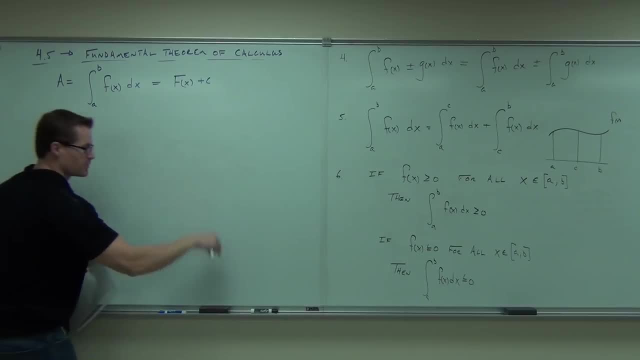 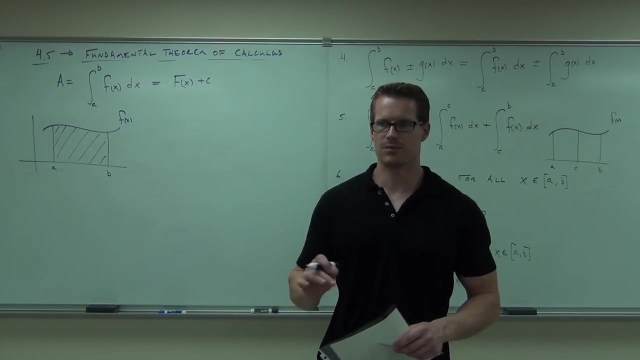 picture of what's going on. Here's our. I'll use the same graph I have over there. Here's our graph, and this is F of X. We're looking for the area. What we want to do is find the area from A to B. That's the goal, Without using our 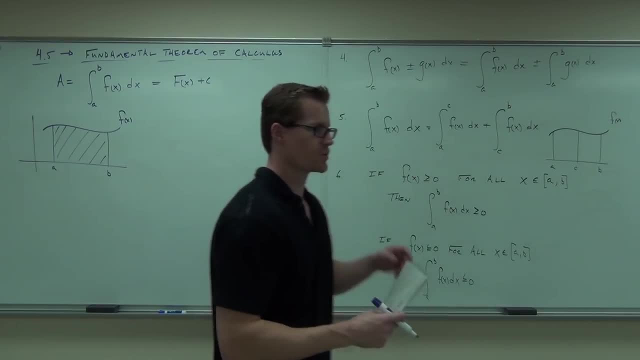 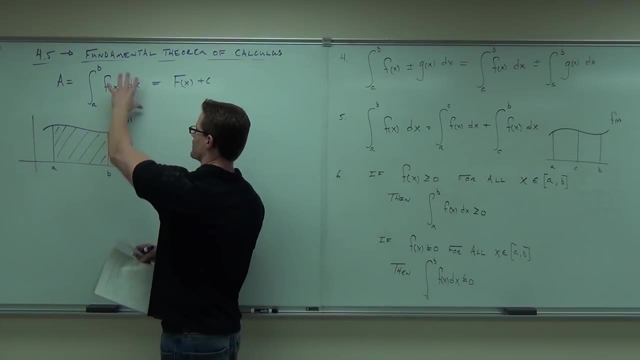 Riemann sums or the summation notation. we don't want to do that. We want to really just think of this as an integral, because we know an integral geometrically represents the area. How can we go from this picture and this thing and tie it all together? What we want is the 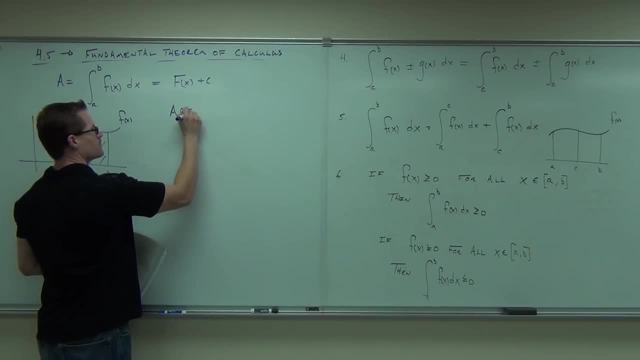 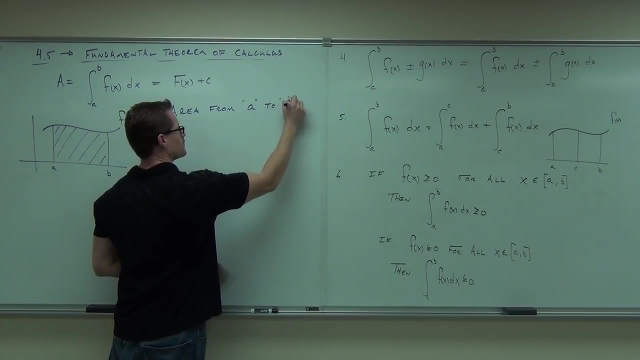 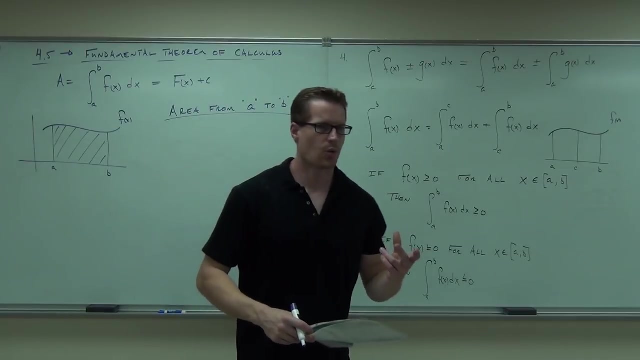 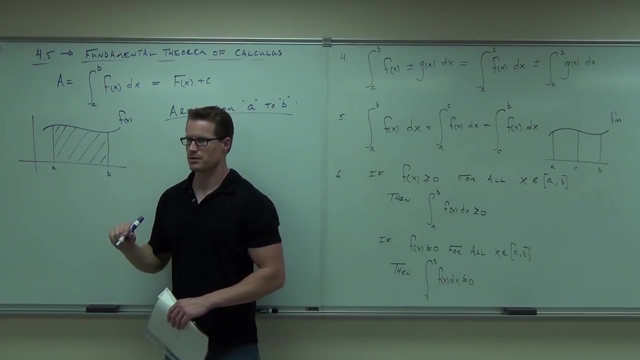 area from A to B. Here's how we're going to think of it. We're going to think of it as well. how about this? Could you find the distance from A to B? How would you do it? You would do B minus A. If this was 10 and that was 3, you'd do 10 minus 3, right, We're going to do basically the same thing. We're going to say: let's take the area up to B minus the area up to A. Would that make sense to you? 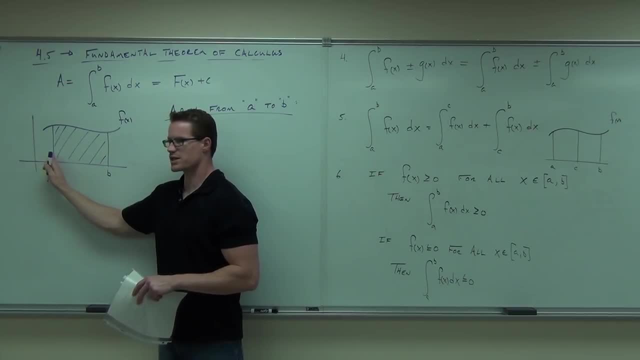 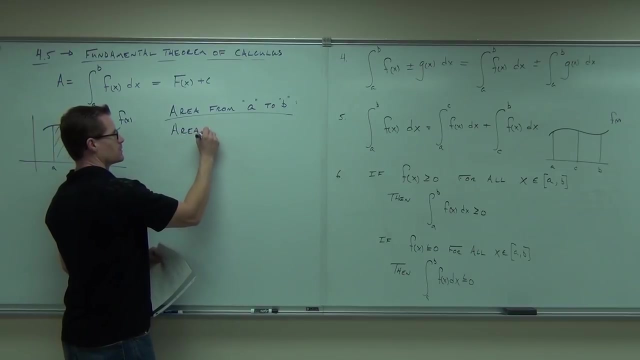 We'll take all of this area, minus off all of this area, No matter where you start. that would work for you, Would you agree? We'll take all the area from left to right, all the area, no matter where we start, up to B and subtract off all the area up to A, and that would leave us with this little bit. How many people buy into that? Feel okay with it? That's exactly what we're going to do. So we'll take the area up to B, starting from wherever you want. It does not matter, As long as you start at the same point for both. 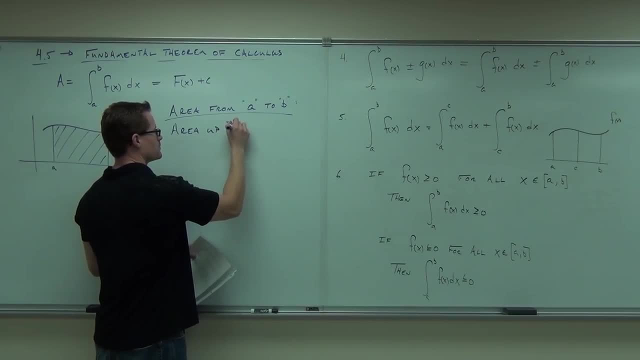 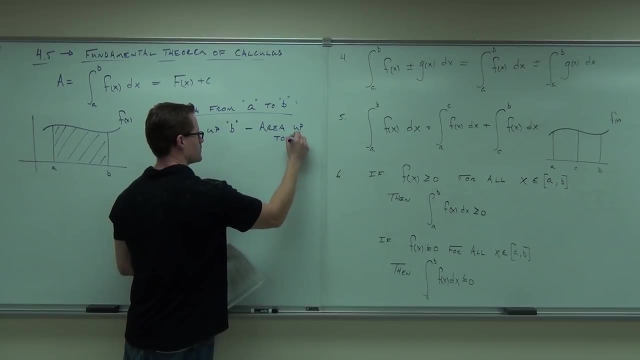 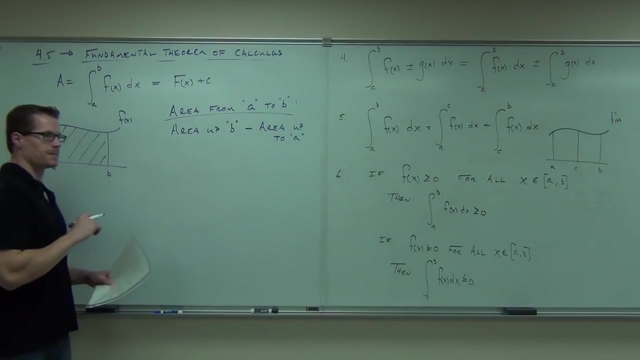 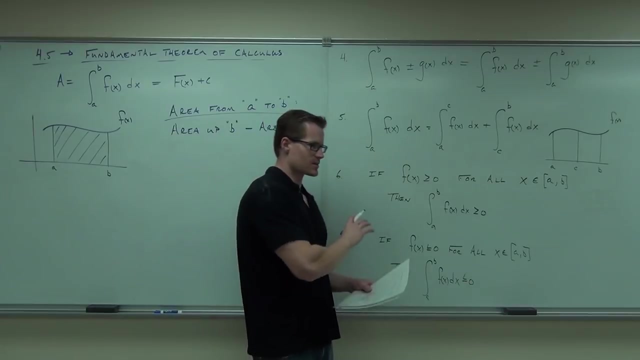 Yeah, Okay, All right, let's go to point A. Can you just make your starting point A so you can figure out the area to be in this track zero? Well, I have to give you something that this makes sense, right, And the way to do that. we are going to start at A and go to B but find the actual 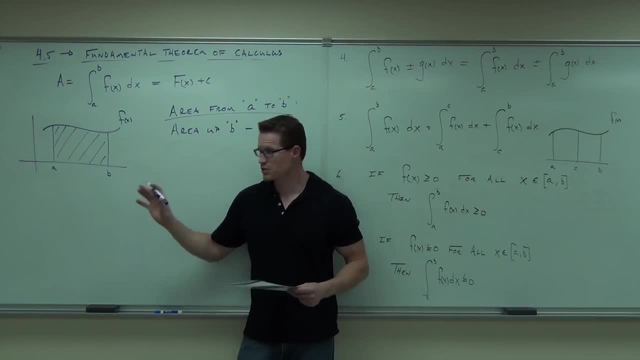 Because it tells me that I need to code this into B, right? Well, All right, I'm going to send it back to you. Cool Series B is the same number of times F minus A, so it's not relevant, It's the same number. 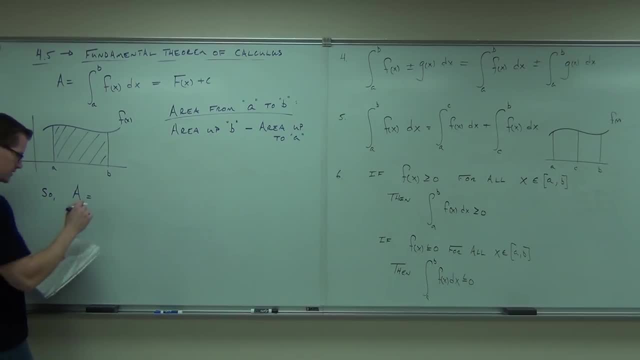 Well, that's all what I can write into B Terrible thing. Just to show you why we have this next piece in there Right now. if I give this to you, You'll probably follow it, but I want to understand the concept of why we'd have a subtraction of this at all. 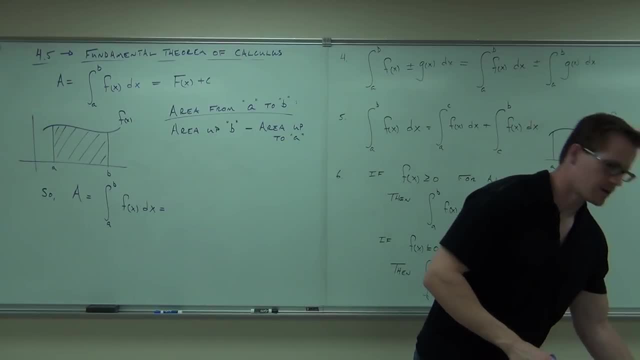 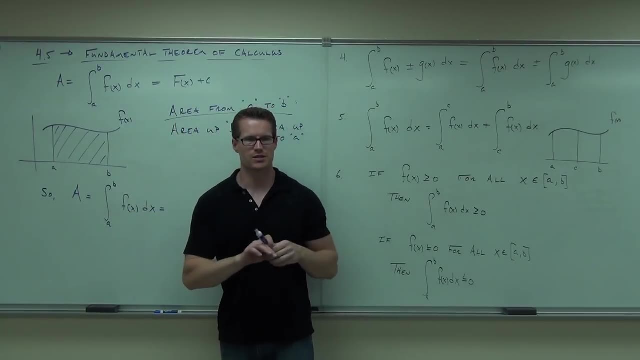 Okay, and we're going to have one right now, So let's think of it. So The area is: This is not changing. take the area up to b minus the area up to a. Now here's what you have to realize. 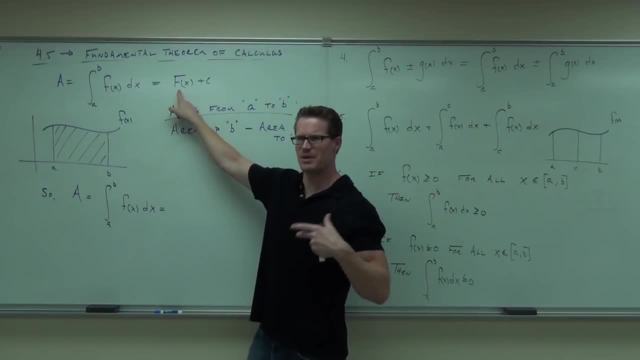 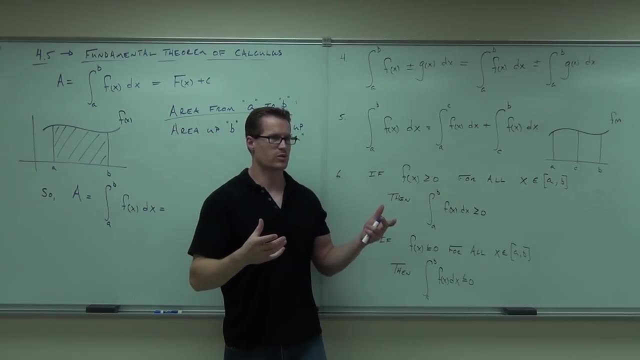 What we're doing here is calculating the area function. You remember me introducing that to you a long time ago, that this indefinite integral action is an area function. it was a family of curves. we just know which one it was. Well, if we have that family of curves, 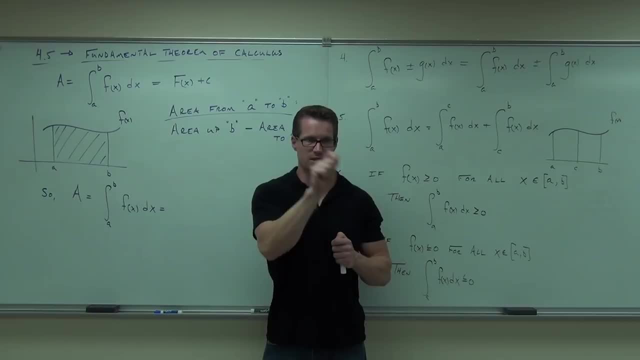 and we're going to an actual point that says: this is where you're going, you're stopping here. that solidifies it for you. It's no longer indefinite, it's definite. You're starting at one point, you're stopping at another point. 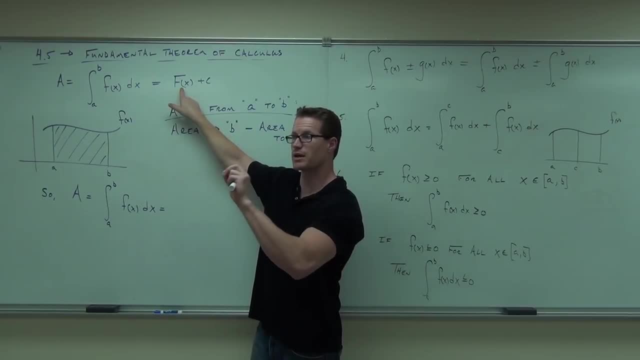 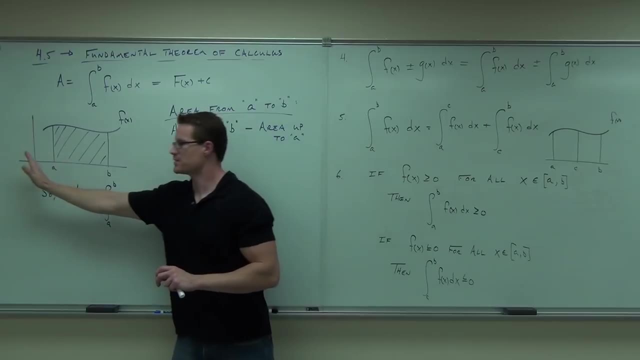 So this right here, that's an area function and we actually have something to plug into it. We have the point: well, where are we stopping? The area up to b: you find that area by plugging in b. The area up to a: you find that area by plugging in a. 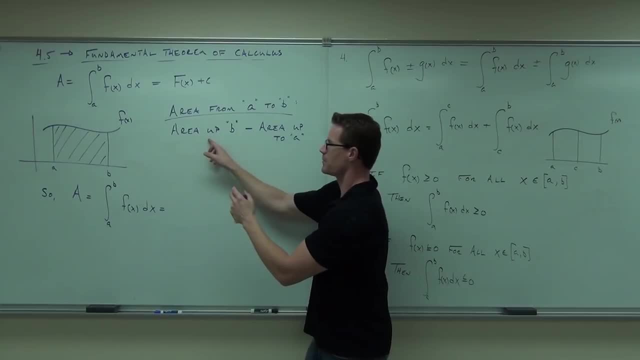 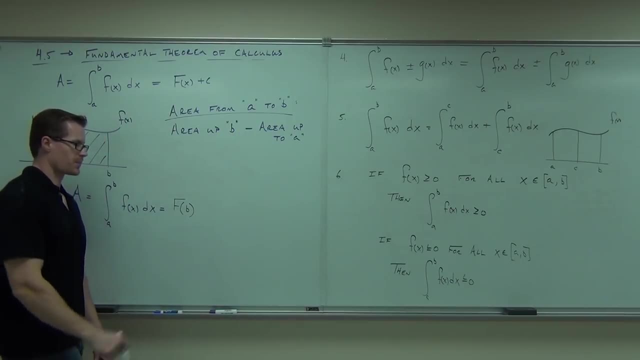 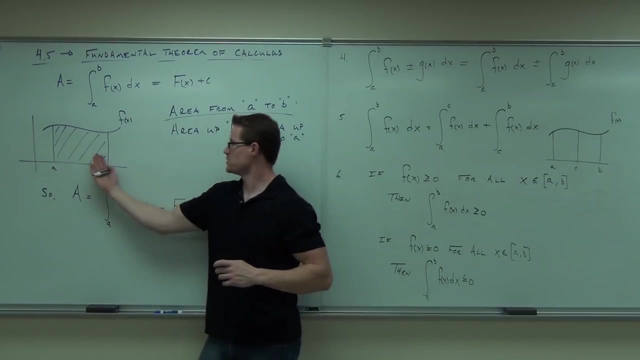 So the area from a to b is the area up to b. The area up to b That would include wherever your starting point is for area. that would include everything up to the point b, everything above the x-axis to the point b. you got me. 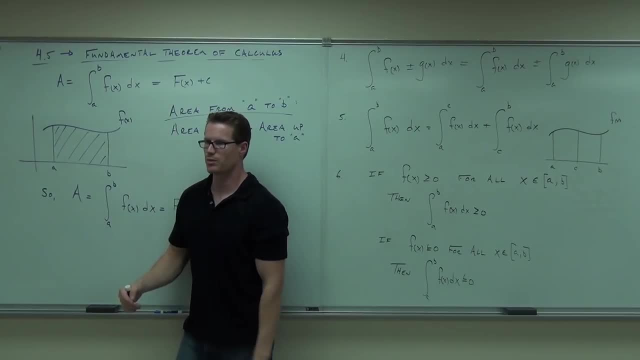 And then we'd subtract off this point a. Now, really, what we'd consider is starting from zero. That way we're not being silly about it and going way too far. We'd say: let's just go from zero, okay. 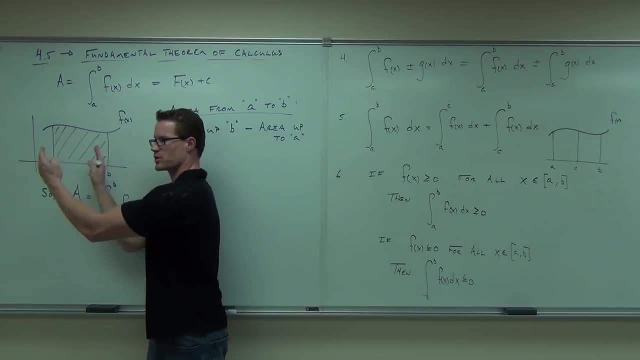 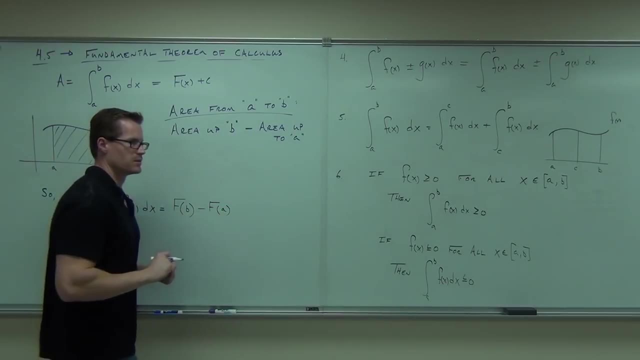 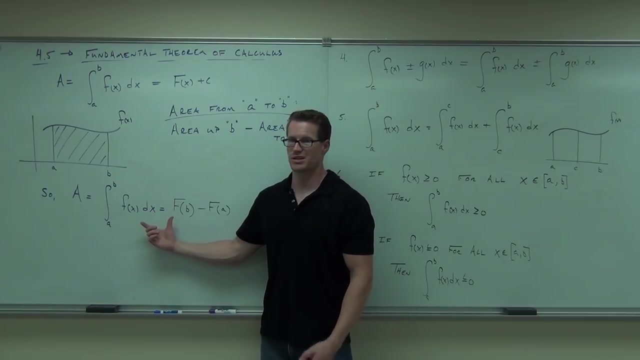 You'd have this area minus this area. it'd give you what's remaining. The area up to b- plug in b. The area up to a: plug in a. That's how you do: a definite interval, You find the antiderivative and you plug in your bounds. 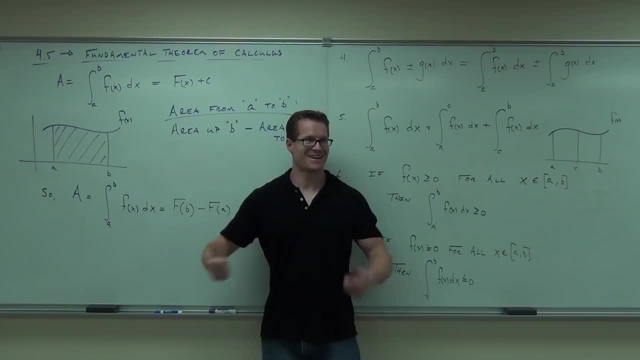 It's actually that easy, Not bad, Not bad. Look, come on now. there's one question out there. What's the question? What's c? Come on, do you see it? What do you do with c? Oh good, do you see it? 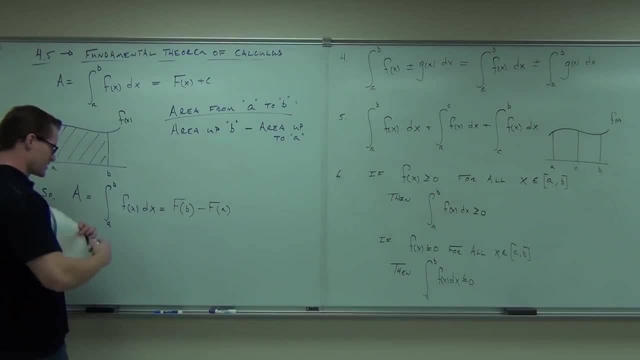 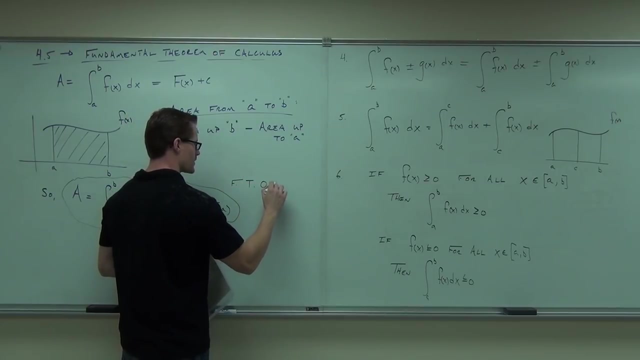 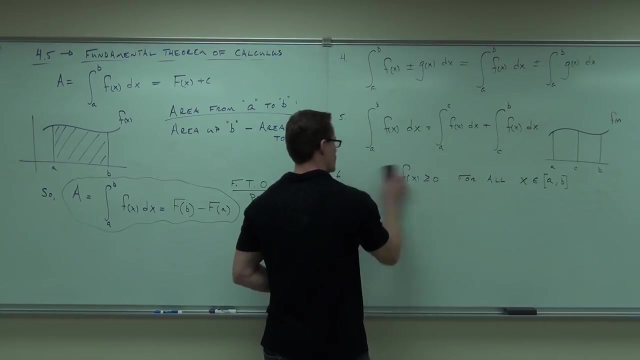 Where's the c? By the way, this right here, this right here, this statement, is the fundamental theorem of calculus, part two. I'll give you part one later. Fundamental theorem of calculus, Part two. Let me show you What happens to the c. 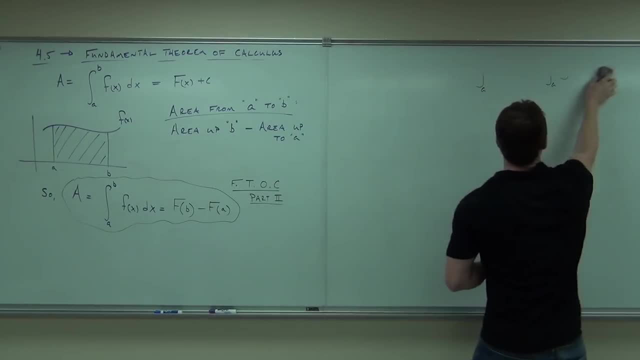 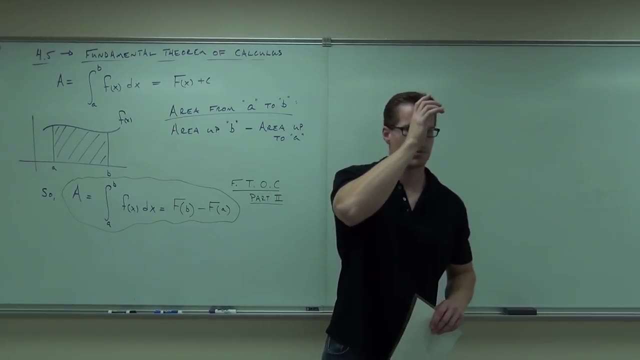 Oh dear, why don't we have a c? Why not Now? you know definitely why it's going to be c. Well, you do know definitely. so we shouldn't have a c. but when you think about it, remember when we're finding out this right here. 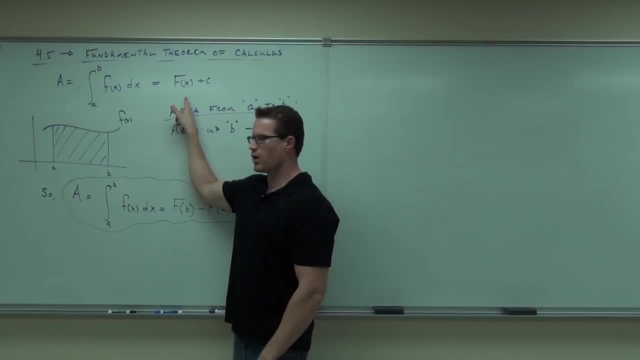 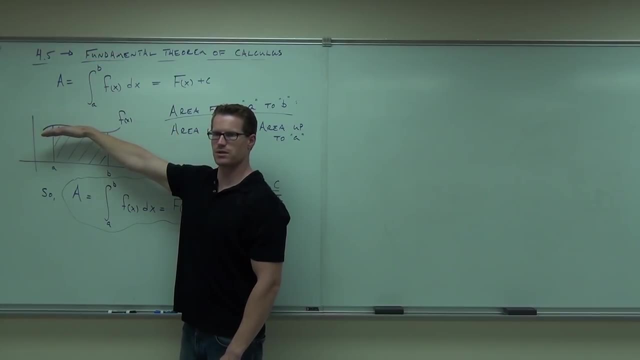 This is a family of curves, right? How do you actually know where it's at? Wouldn't a curve way up here have a different area than one right here? Clearly, the height would be different. So why does this even work? Well, think about this for a second. 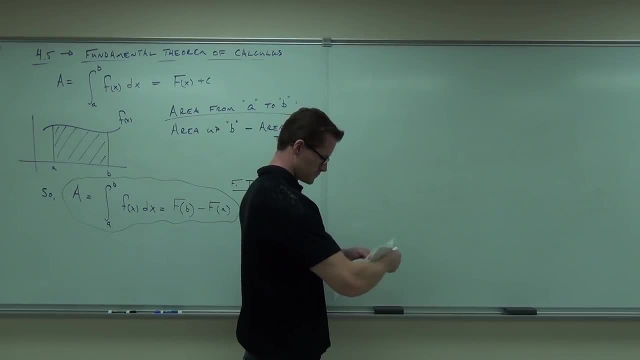 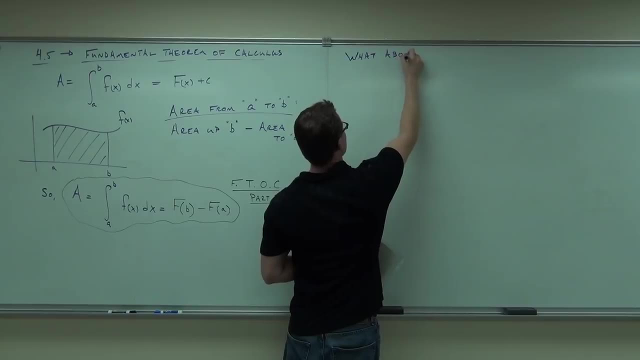 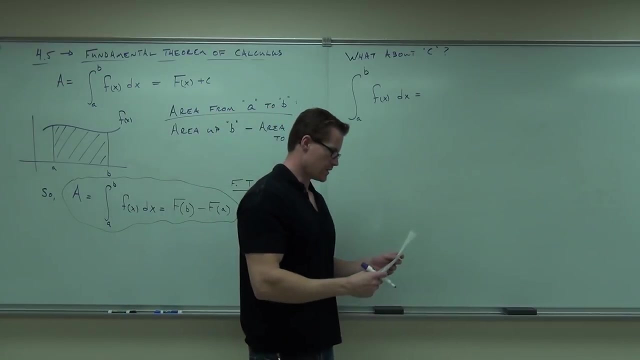 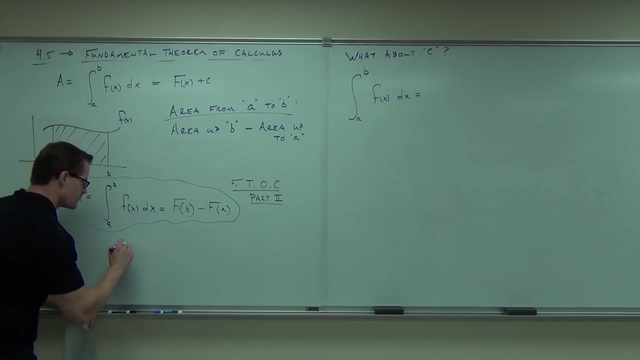 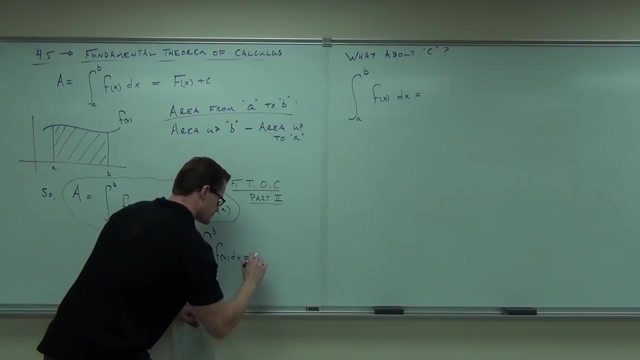 What about the c? How about c? Suppose you considered it. By the way, the way that you write this, I should actually give it to you this way. One more thing: this is also written as f of x, and that's an evaluation symbol from a to b. 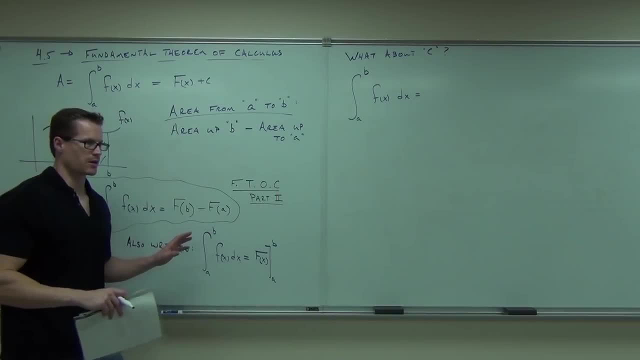 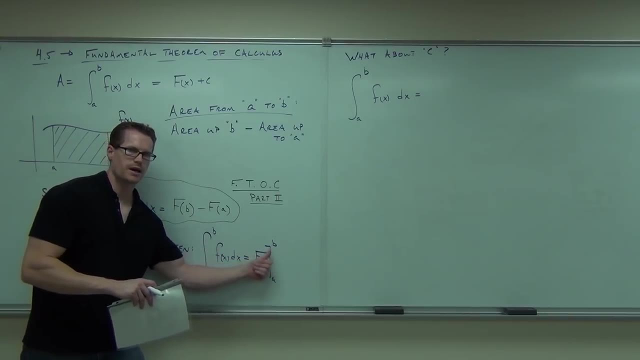 That's how you can write that and we're going to be practicing that as well. It says the same thing. okay, This and this is the same. How you do this is: you plug in b and you subtract off a. You plugged in b to your antiderivative. 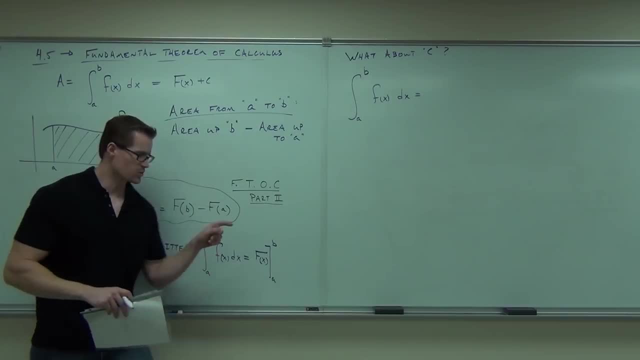 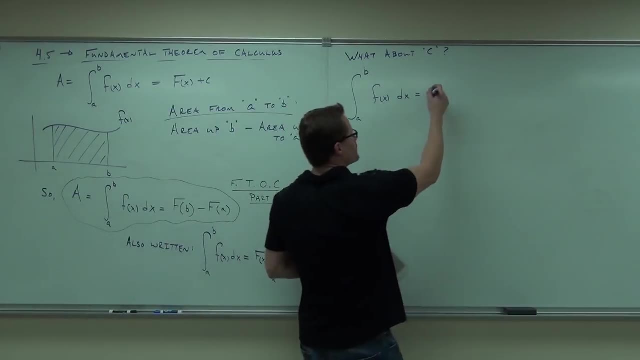 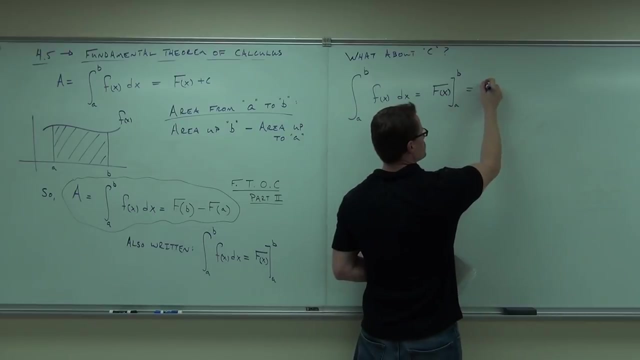 and you subtracted off f of a. Are you guys okay with the notation? So you see that line right there. It's like half a bracket. It goes from a to b. That's what that means. So this equals this And this equals this. 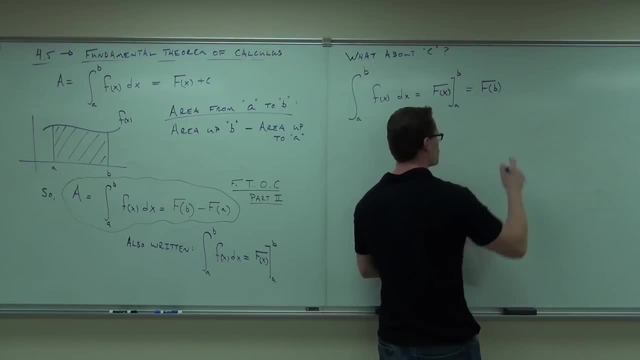 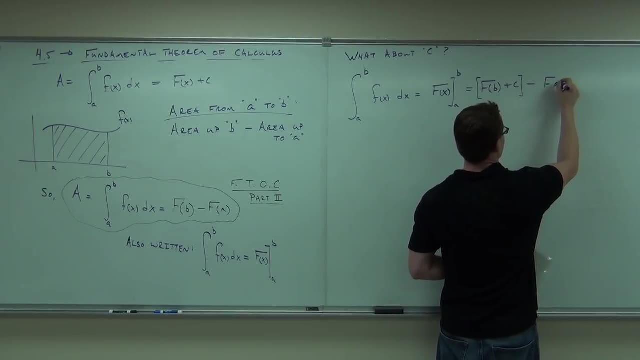 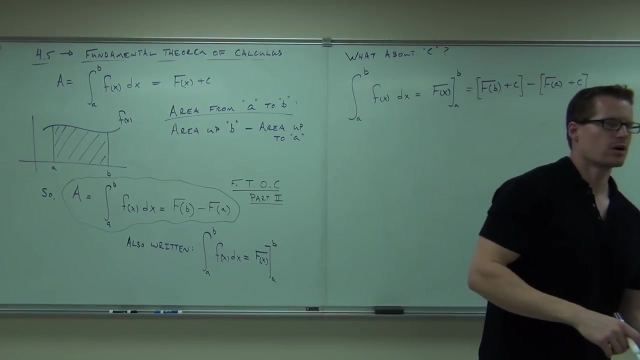 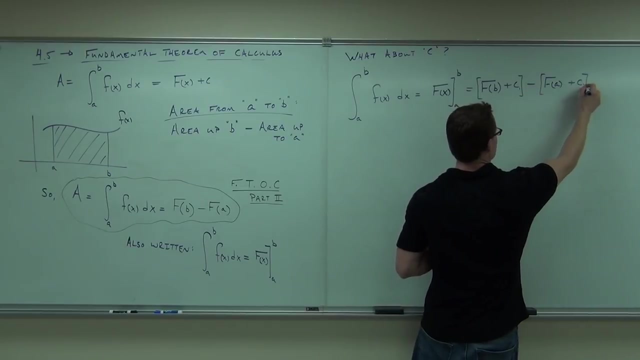 Let's suppose that we actually included the c. Now some of you might be wondering. well, when you think about it, you might be wondering: why don't we have a c one and a c two? Say it again: They're the same constant. 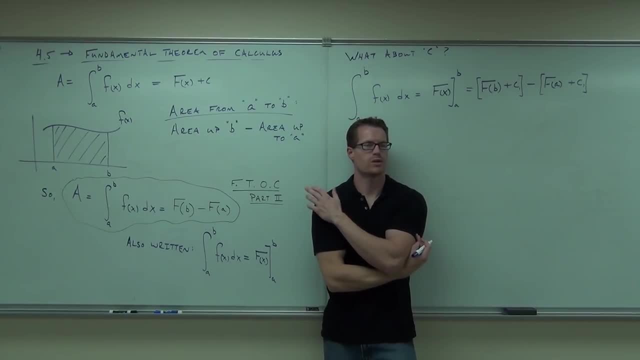 Why are they the same constant? How do we know that for sure? He's right? Why They're from the same function. Say it louder: They're from the same function. They're from the same function If you're integrating that same function. 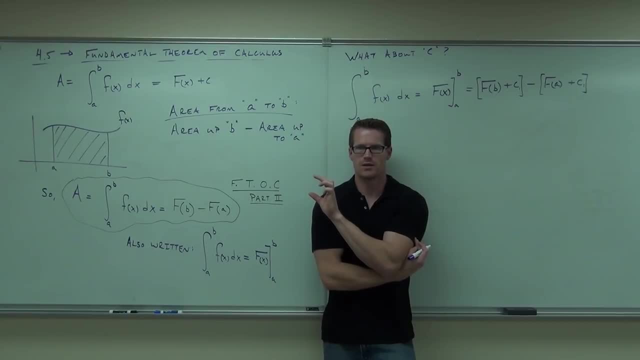 you're not switching functions on me, are you Integrating the same thing? Then whatever c you get is your c. No matter what you're plugging in, that's going to be the same function itself. Does that make sense? So wherever you're at, that's the same function. 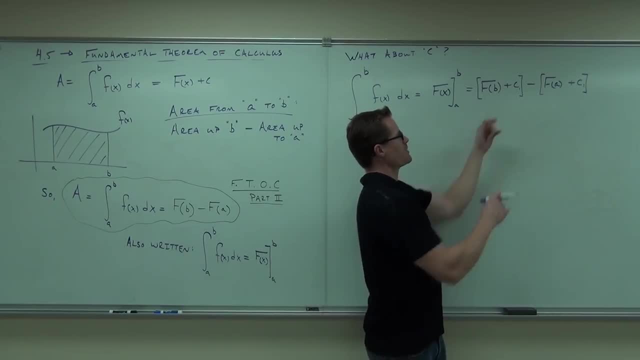 So we integrated one time. Look what's going to happen If you have f of b plus c. it's not c one, it's just c. f of a plus c is not c two, it's just c. What's going to happen to my c's? 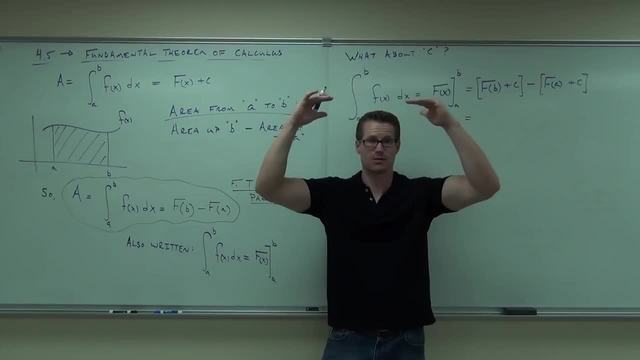 Wherever your c is, wherever your c is, that height difference will be eliminated. It drops out of your equation, as your book likes to call it. The c's are gone. So remember the plus c. that's just the height, right. 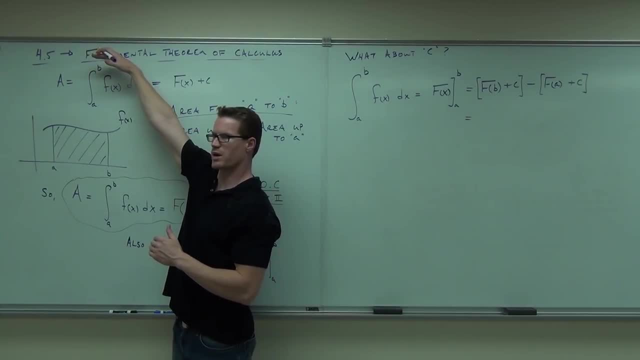 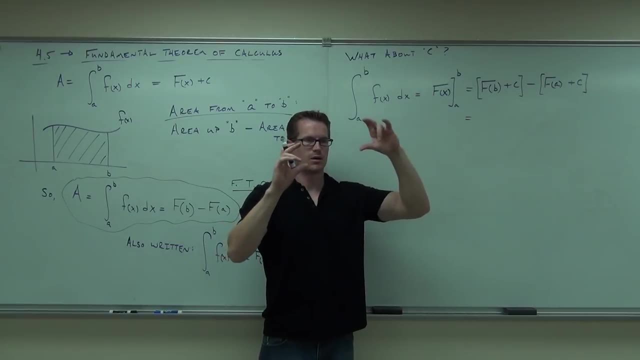 Height of your function, Even if it's way up here. Same type of function just way up there, But both of them we'll be way up there. The f of b plus c. f of a plus c. we're subtracting out that plus c part. 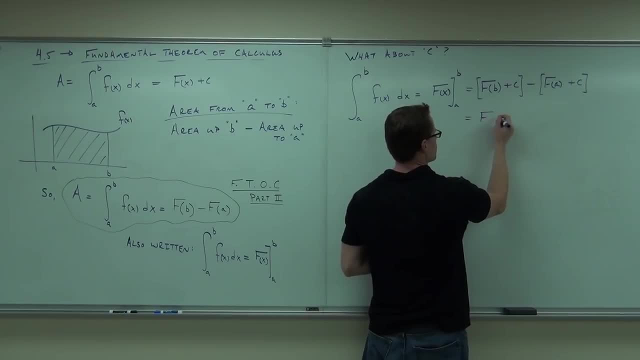 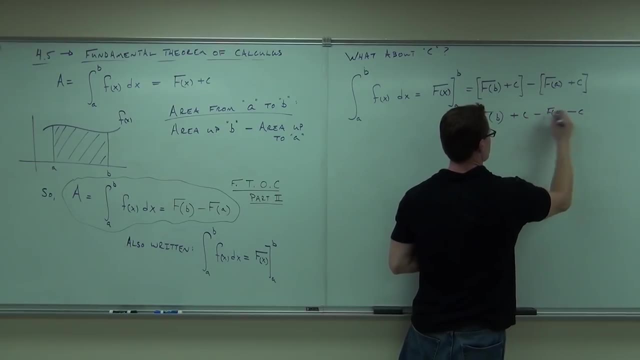 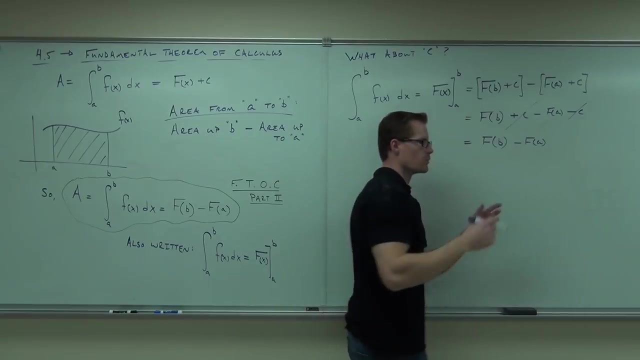 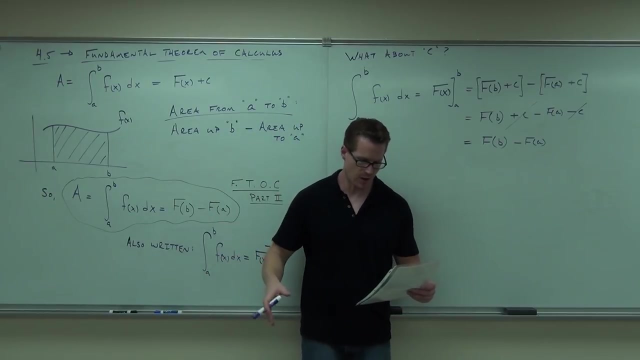 The plus c's will be eliminated from your equation And that's how we get what we get. So the solution to this is: C is gone, drops out, so we don't write it for our definite integrals, Indefinite, absolutely. 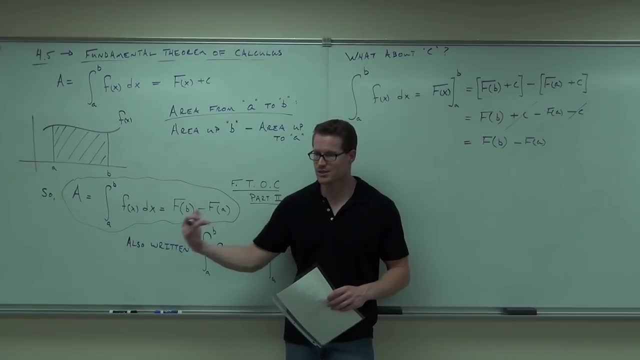 But definite. we should end with a number, end with an area, because this thing is an area By a show of hands. how many people feel okay with what we've talked about so far today? Would you like to try a couple examples? 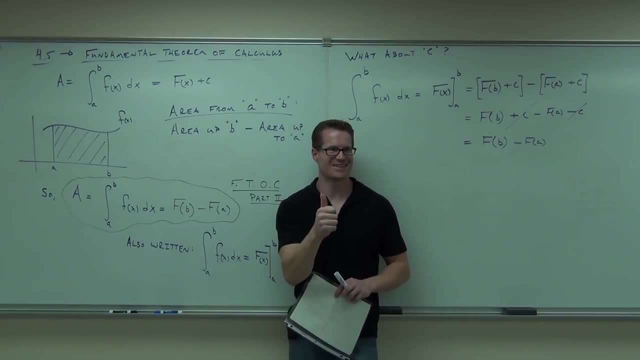 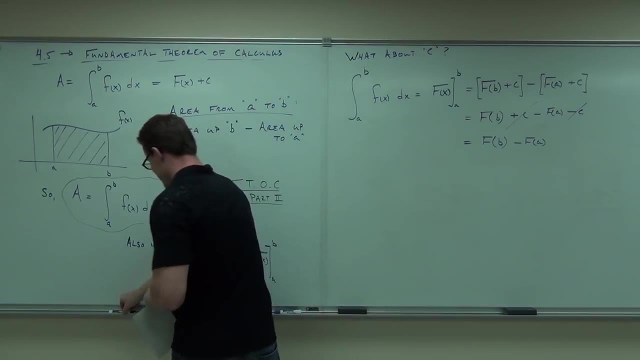 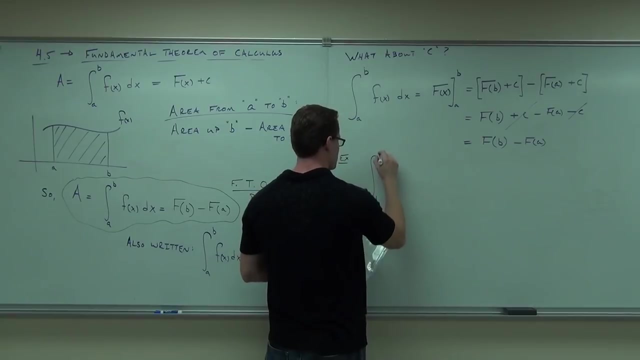 You're gonna really like these. by the way, Are you ready to really like something in this class? Oh, wow, Great, now we're over here. Yep, You're sunk now. Okay, so an integral from one to five of x dx. 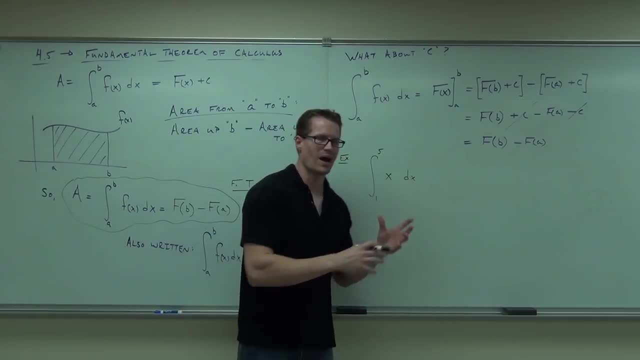 This is an area which means we should end with a number. It's actually a definite integral. Why is it a definite integral and not an indefinite integral? Right there there are bounds. are bounds of integration. We actually have numbers. We should end with an area. 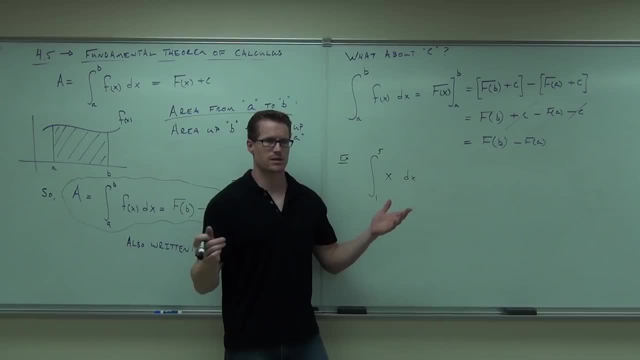 Now can you integrate x dx Easily? yeah, we already did that. No need for limits, no need for any of that stuff that you've spent your whole life doing just now. okay, It's doable, you did it right. 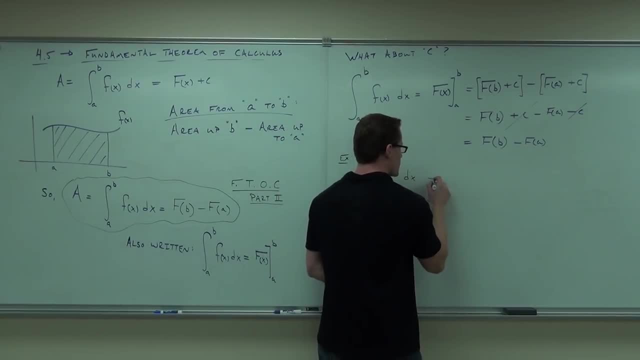 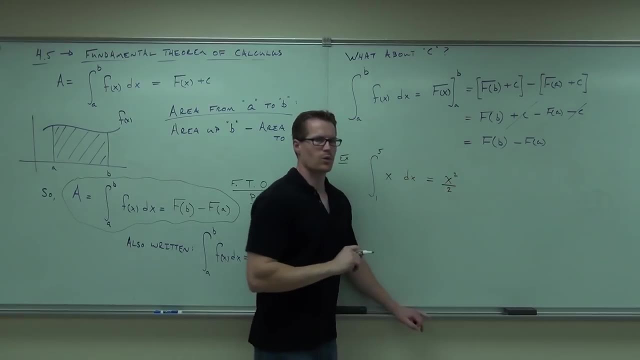 But this is a shortcut, not a shortcut. I guess it's a shortcut to doing it. What is the integral of x, please? Where are we integrating from? Where do we start our area? where do we stop our area? One to five. 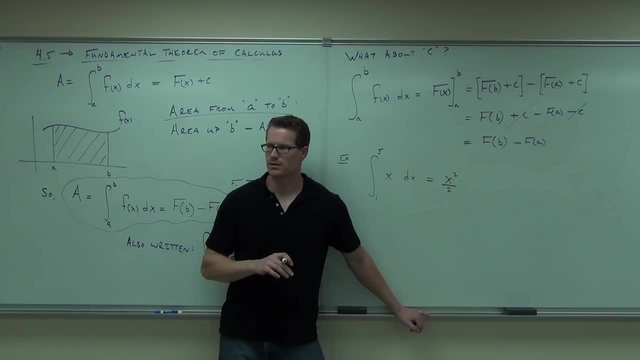 One to five. why don't we have a plus c here? Because we hit it, it fell out. Even if it fell out, even if we did, it's gone, because you can subtract it off anyway, it's the same plus c. 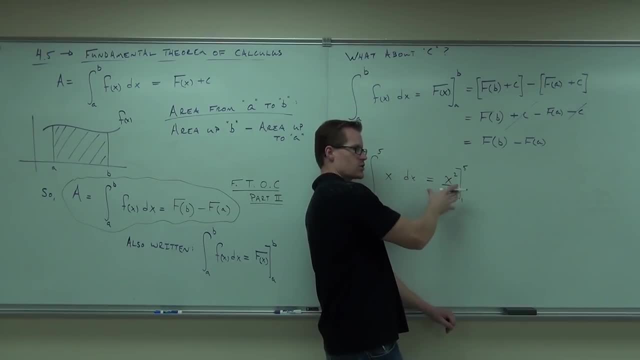 One to five. here's how you show your work. You do this step first. you show me what your integral is. You show me where you are plugging in numbers from. You plug in the top one first subtract, then plug in the bottom one. 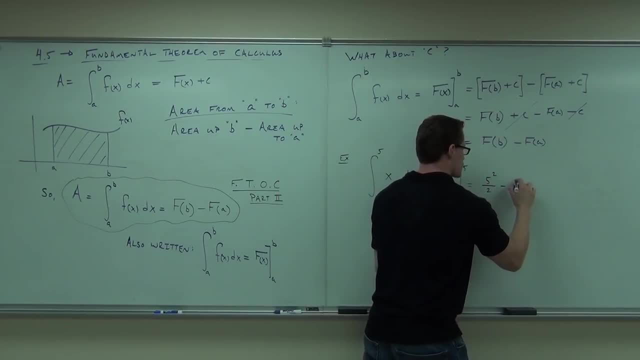 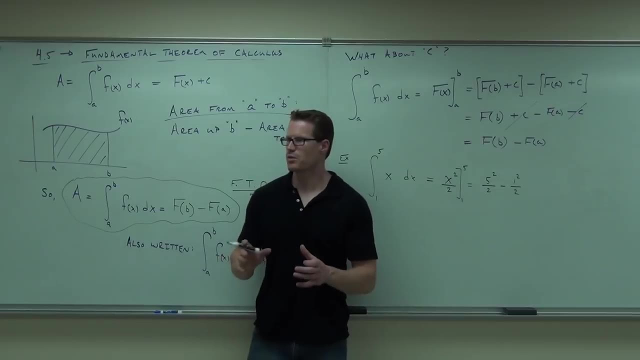 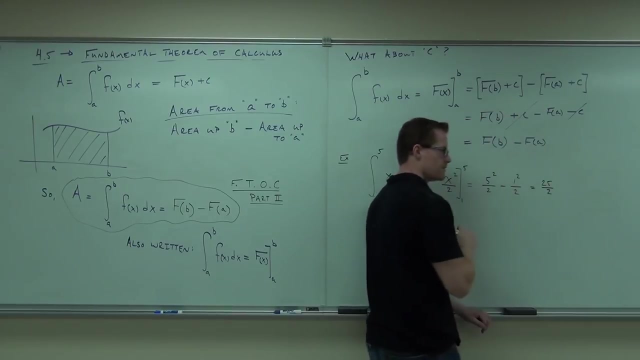 This would be five squared over two minus one squared over two. is how you show that? Do you see where the five and the one are coming from? So we're going to get 25 halves minus one half. how much is that? Twelve? 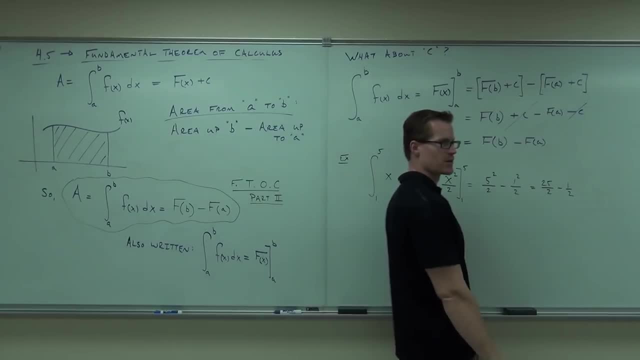 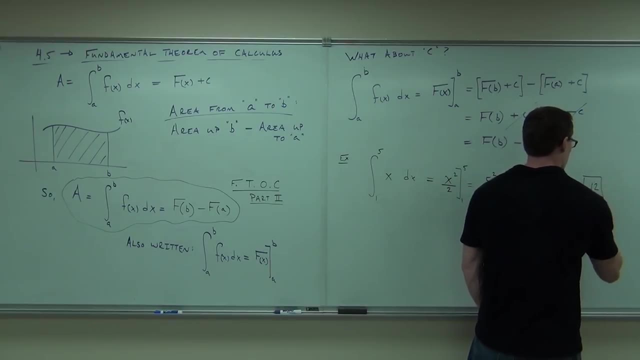 Twelve, yeah, 24 halves is 12.. Is that quicker than a Riemann sum? all the stuff you can do with left end points? Yeah, What is 12,? what's 12?? The area under that section, Exactly, right. 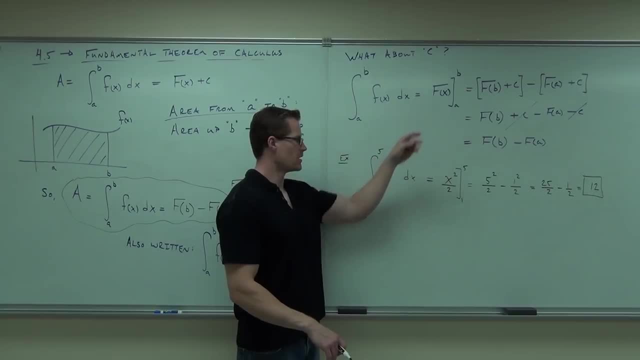 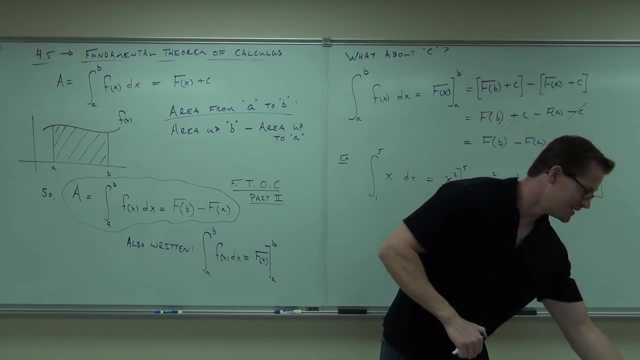 Area under that That curve, which is just a diagonal line from one to five. Yeah, thanks, You're welcome. Well, this stuff is good to know. It shows you where it's coming from. It shows you why you're doing it. it shows you how you do it. 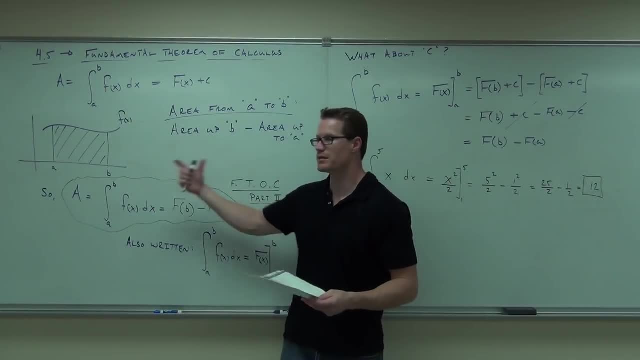 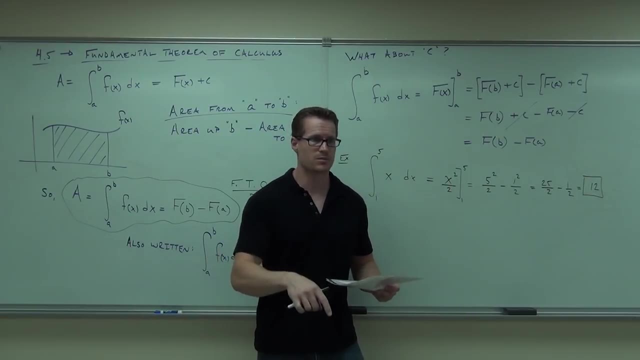 And you make sure you know what all this stuff means, right? If I just gave you that, you could do it, but you would not understand it. We did the limits of the sums so you would understand why you do this, how you do this. 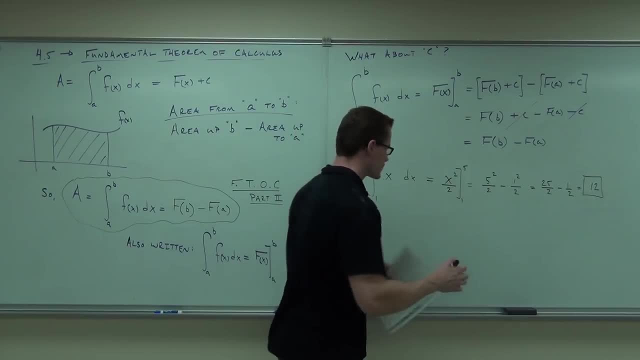 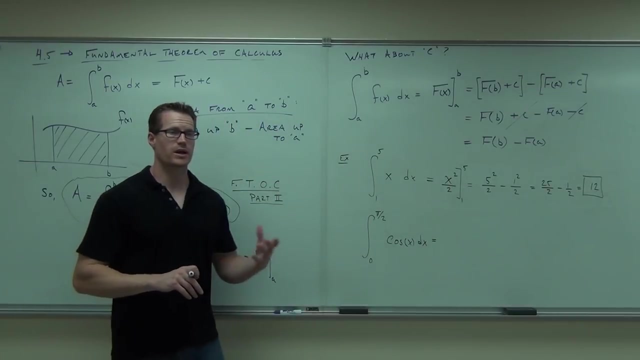 Now we needed something else though, because when we get to things like this, a Riemann sum doesn't work all that nice for that. Again, you'll do an integral with that. So this is also an area. it's an area from zero to pi over two of cosine x. that's your. 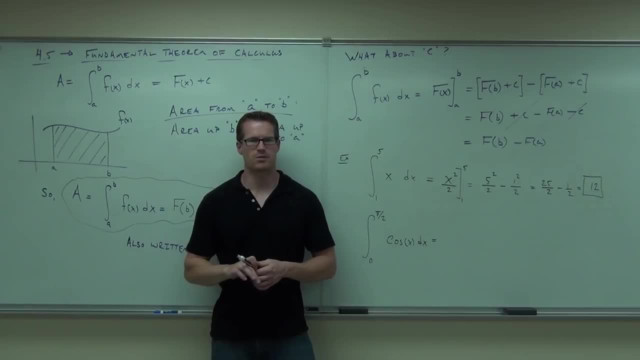 cosine curve, Now the integral of cosine x. you've got to be able to get these right, otherwise your areas are going to be wrong. You'd show an area above the x-axis when it's below, or below when it's actually above. 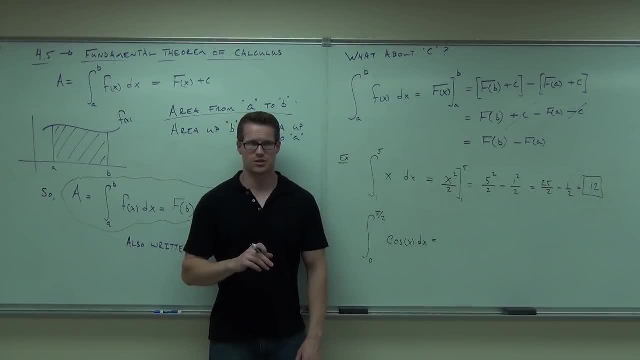 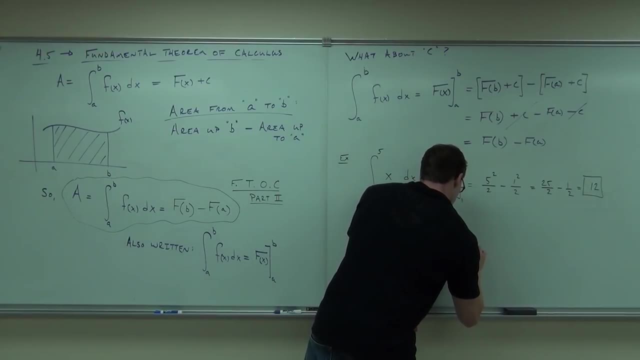 What is the integral of cosine x? please, Sine x. Do you need to memorize that? Yes, Yep, And where are we going? Which one do we plug in first? the pi over two or the zero Zero? All right, which one? 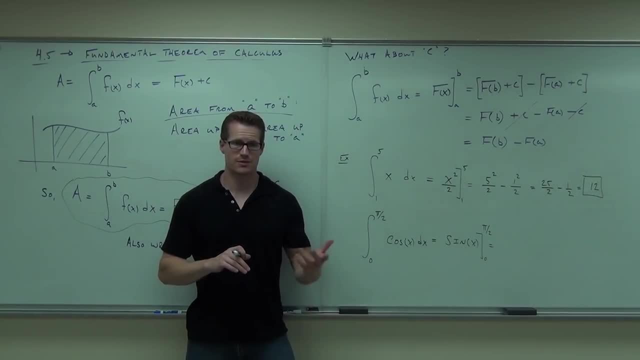 Pi over two, Pi over two, The pi over two. Otherwise you'd have negative which. by the way, if you notice that when your bounds are reversed, notice that you're subtracting off the wrong thing, that would switch your. 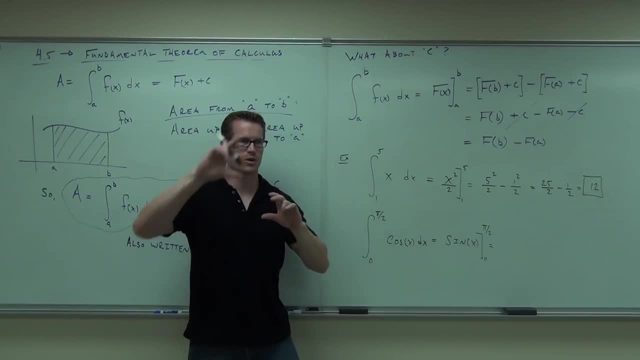 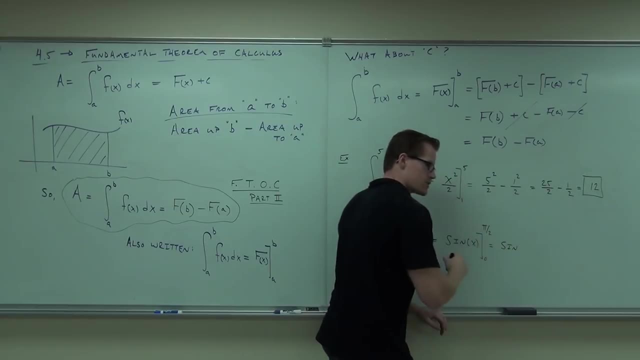 sine of your area, right. That's why the whole the property I gave you where you can switch your bounds, and it switches the sine of your integral. that's why that comes about. So here you'd have sine pi over two, minus sine of zero. 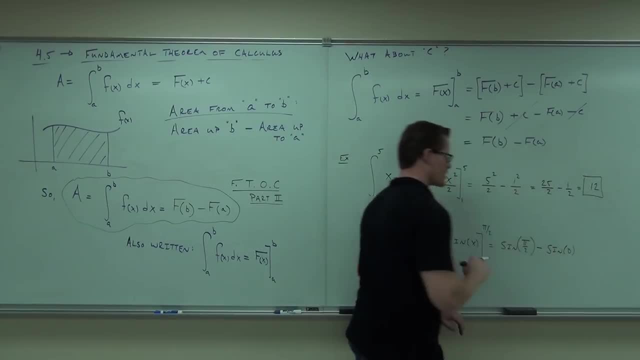 All right, come on now, people. I know you love some trig functions, throw it at me. One, One One. Which one's more Sine over two? One minus Zero. Zero Equals One One. 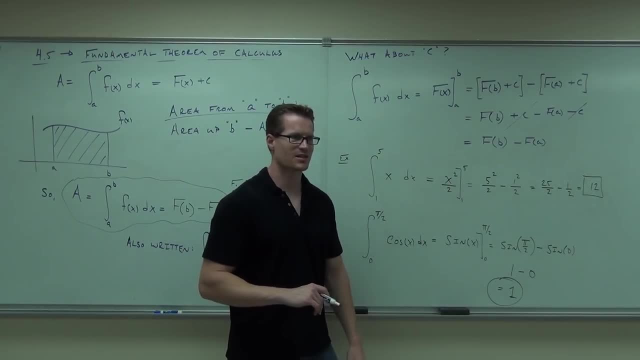 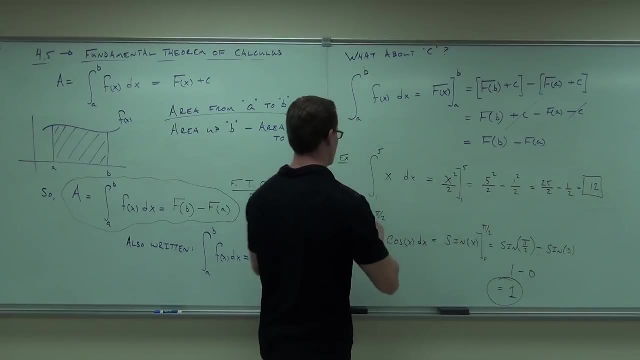 Your area is one That's weird. Oh my gosh, have you thought of this? What this is? Do you understand what this is? Yeah, What's the picture? Yeah, Maybe you should pick one of those. Yeah, Yeah. 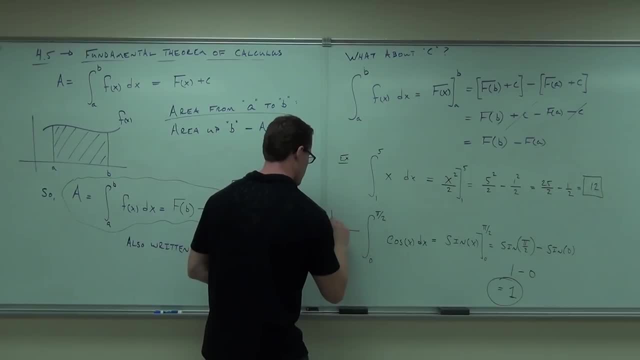 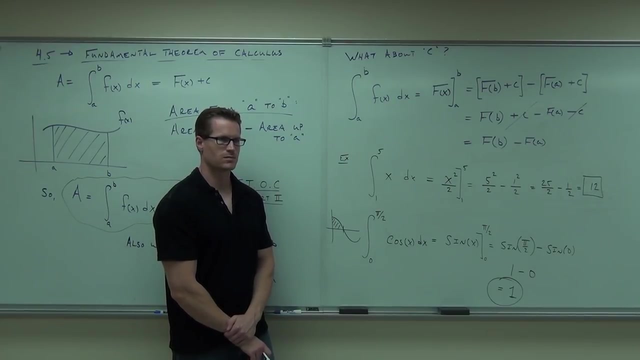 Maybe you should pick one of those Starts here Goes like that, Here or there, Of course. Right, Yeah, I hope so. That's a cosine, That's a cosine, Cosine, Cosine, Cosine, Cosine. 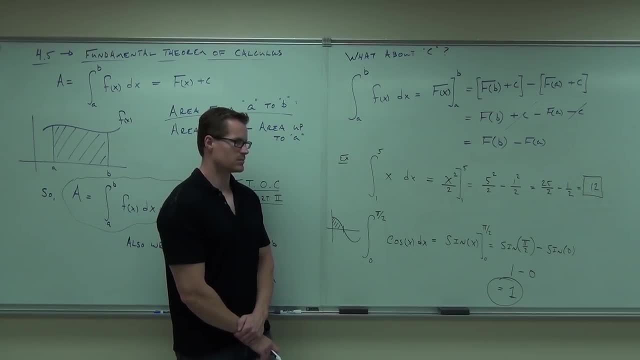 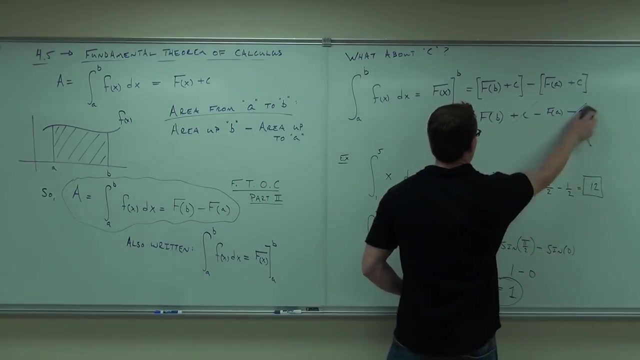 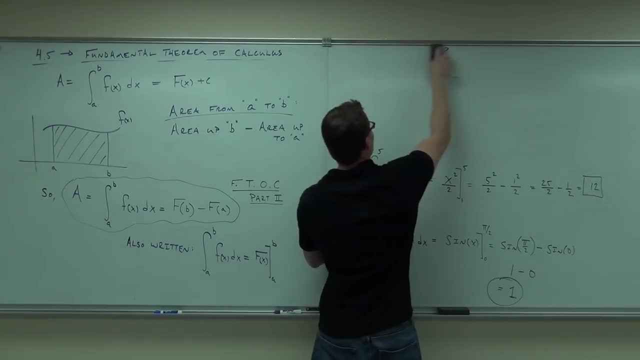 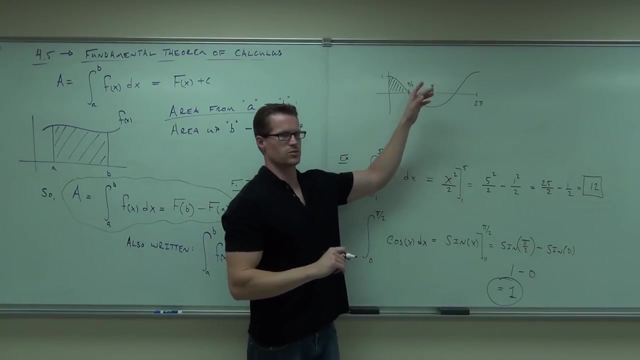 Did you have questions on that? No, What's the video On what On? what You just found? Don't draw these first. draw your curve first, Shoot. come on now, So a teacher who masters your reading, boom yeah. 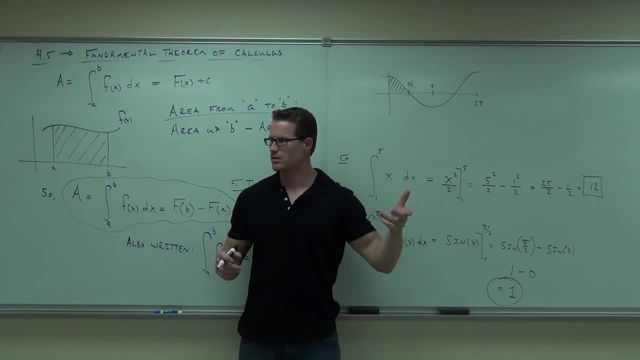 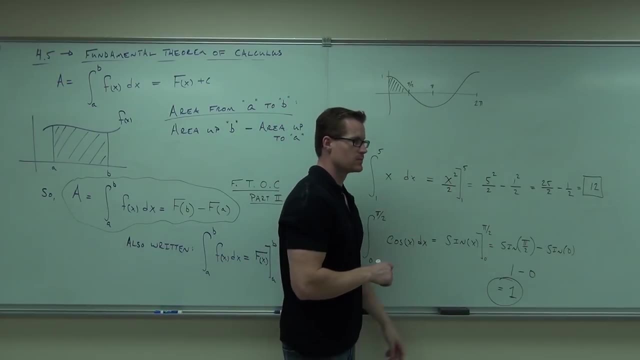 Yeah, that's your area. that you just found that's equal to one. isn't that very interesting? That's interesting, it really is interesting, Which means the next section will be equal to negative one- Hopefully negative one, And then it'd be a positive one, and so on and so forth. 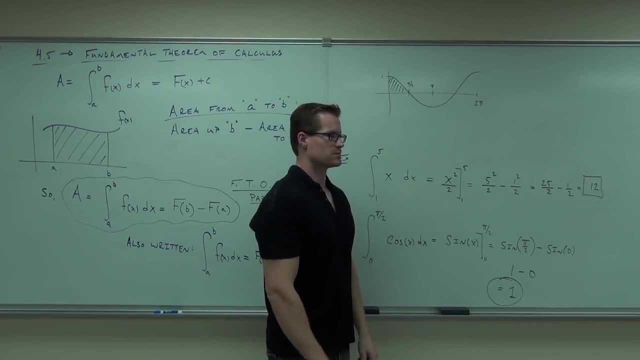 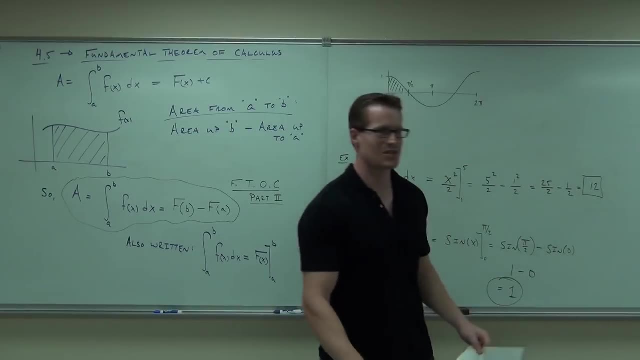 Positive one, negative one, negative one, positive one, Okay, and then it'd be positive one, so it'd be all up. Add it all up Zero. Yes, Okay, Is that just true? You gave a circle zero. did you catch that? 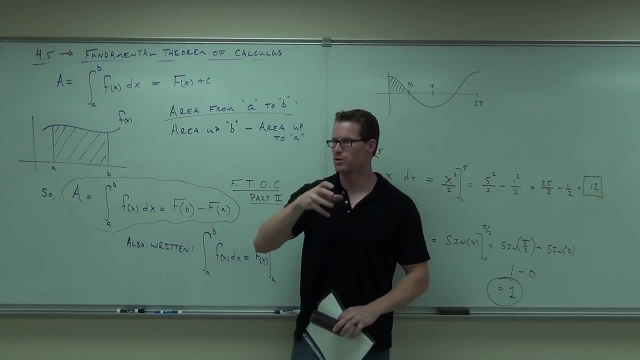 Wouldn't it be if you did an integral Yeah? Yeah, because you have the area above and the area below would match up. Because we're talking about net signed area right now, We haven't made it to total area, which is what we'll do in just a little while. 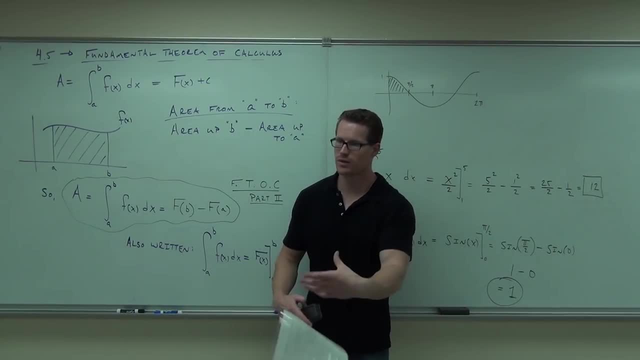 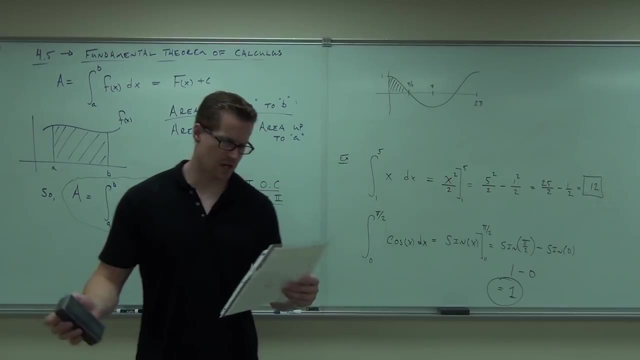 We haven't made it there yet. Total area would change the area below the x-axis into something above the x-axis, so that you could actually add it together. We'll talk about that in just a bit. Right now we'll do a couple more examples. 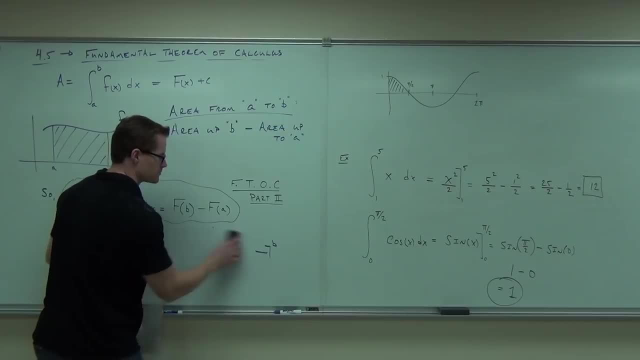 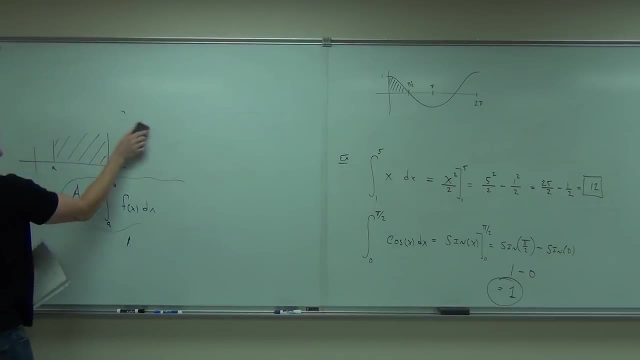 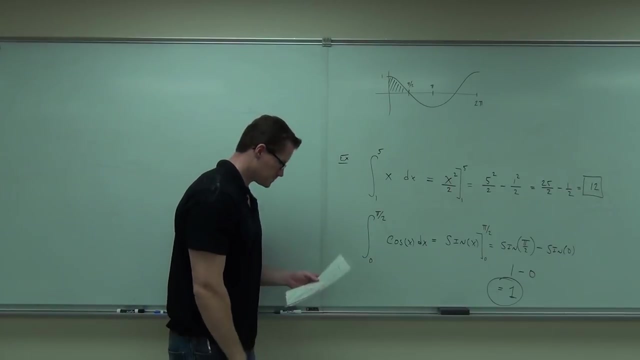 just to really illustrate this stuff. and then we'll go to the next class. Now are we heading up to zero? Is that still true for also tangent? No, tangent has undefined points. You can't go forever. If you think about tangent, tangent is this: 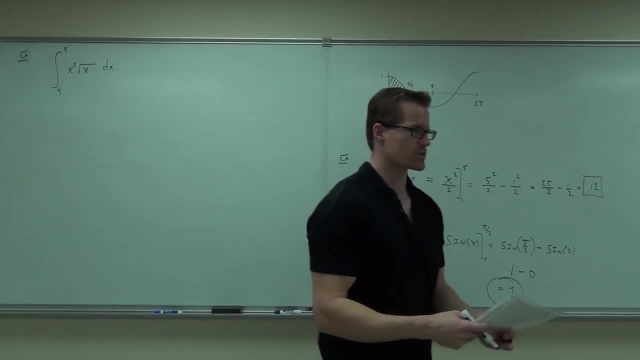 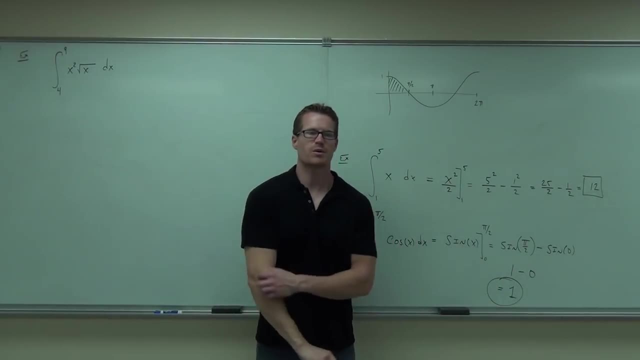 Also one that would probably be kind of hard with Riemann's sum and those limits. okay, Not one, that's great. However, can we do integrals with it? Sure, sure, You tell me what you'd do first. You can't split that. 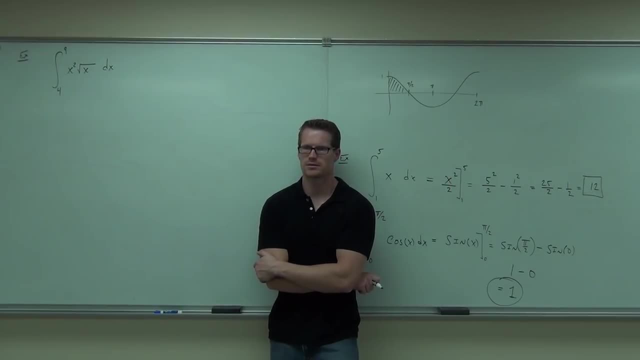 Why can't you split that up? Multiplication? Ah, darn it. I'd get rid of zero square root and turn it into x over 1 1⁄2.. X to the 1 1⁄2.. That'd be a good idea. 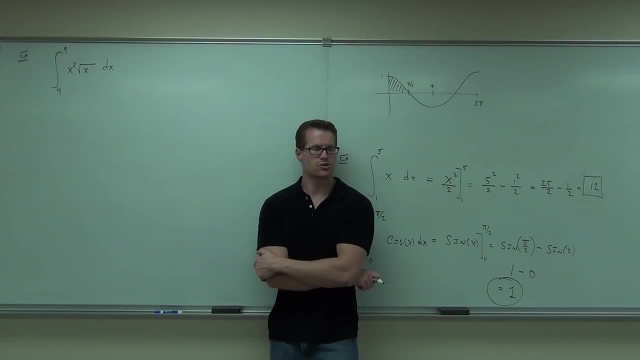 Then I'd combine the two, Then you could do standard integration. Sure, Don't jump to something super hard right away. Don't jump to a substitution. I haven't even showed you that for this yet, right? So that's off the table right now. 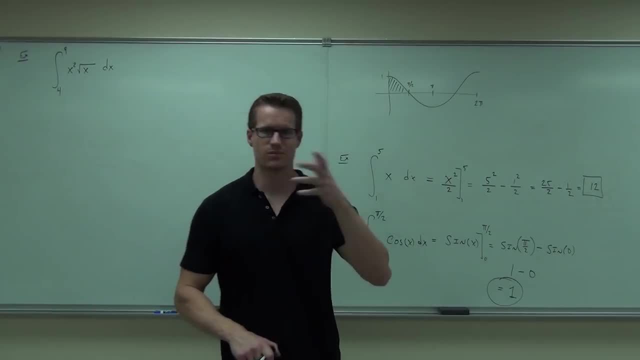 Don't jump to that stuff. See if you can do it easily. Make sure you maybe change a root or two. Substitutions often work when you have well trig functions is a good indication for that. you should probably try. Or if you have parentheses. 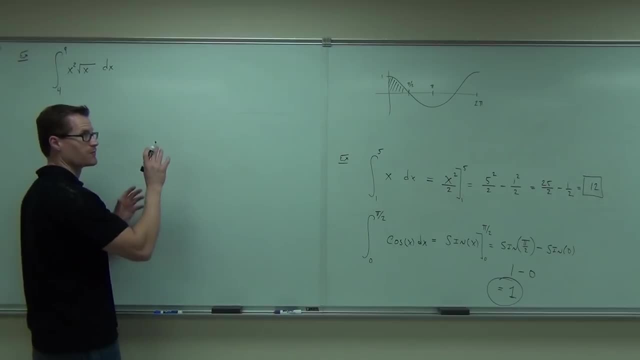 that's a really good indication. you should probably try. And it won't distribute nicely. That's a very good indication. you should probably try. So x to the 1 1⁄2,. yeah, I'll bind to that Dx. I like that. 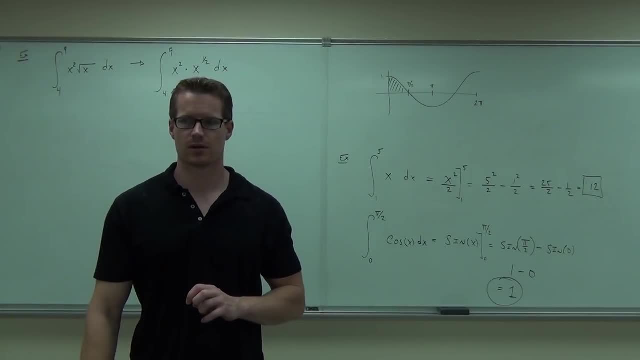 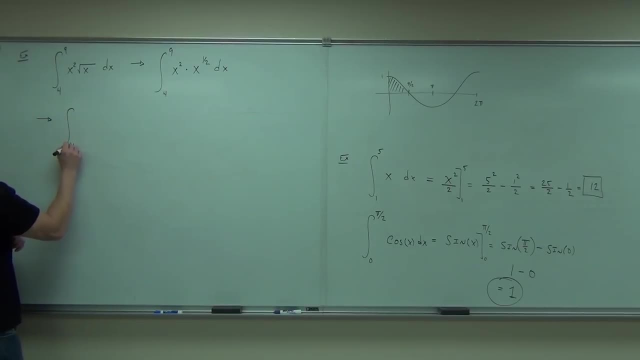 And combine them. x to the how much if we combine those 1 1⁄2.. You add right, You add to those 5 1⁄2.. Exactly, Mm-hmm 2 plus 1 1⁄2.. 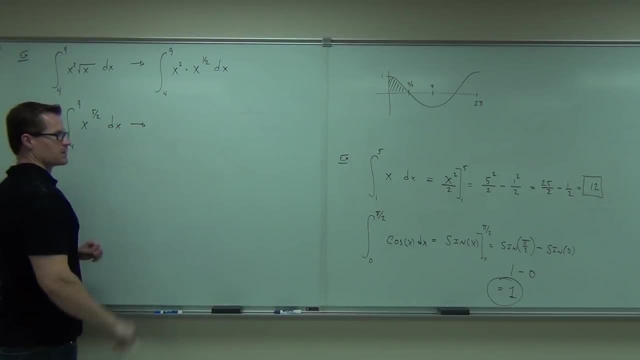 You seem to know my trig groups. I got a calculator: x to the 5 1⁄2,. yes, Can you take an integral of x to the 5 1⁄2?? Very easily, This would be x to the 7 1⁄2 over. 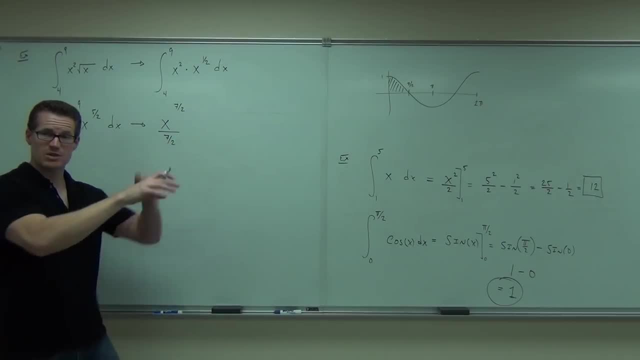 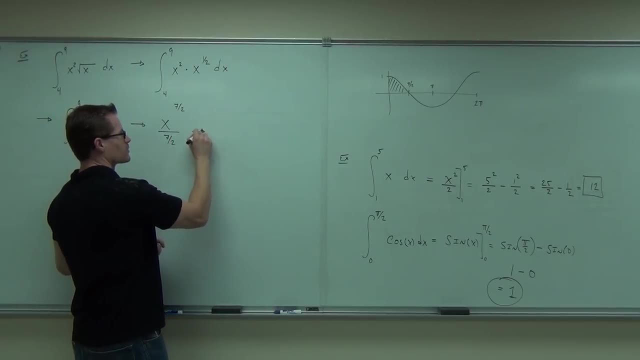 7 1⁄2.. 7 1⁄2.. Over 7 1⁄2.. Over the same exact variable. I'm sorry, exponent up top, exponent on the bottom, No problem, Make it a little bit prettier here. 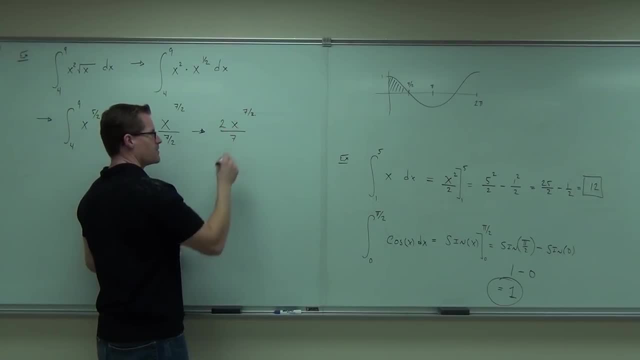 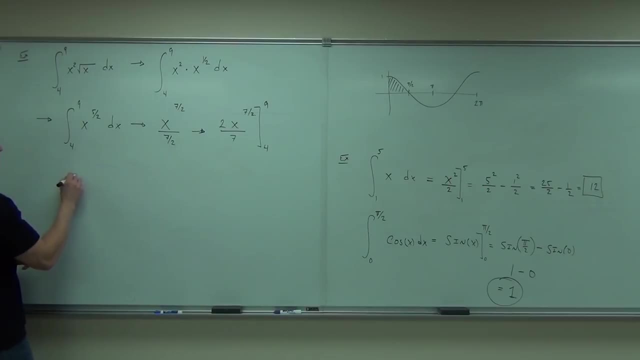 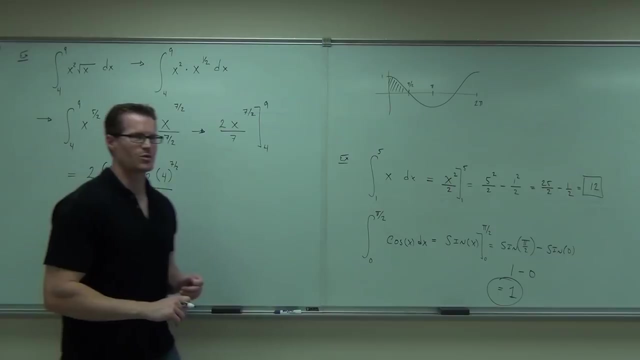 We're going to have 2x to the 7, 1⁄2 over 7.. And then we get to evaluate from 4 to 9.. If we plug in the 9 first, I've actually given you some nice numbers. 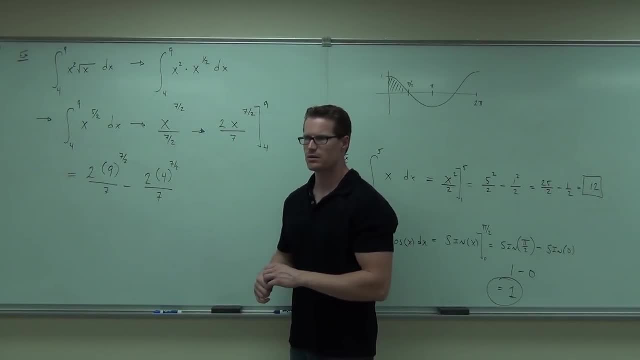 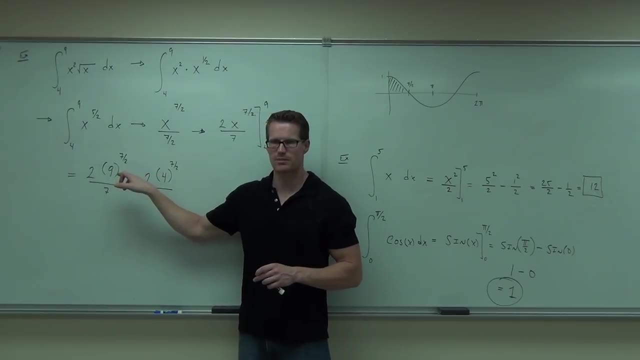 Do you know how to do 7 1⁄2 without a calculator, Or to make it quicker on a calculator? This is power over root, right? Oh jeez, I hope so. Do you remember that? Power over root? 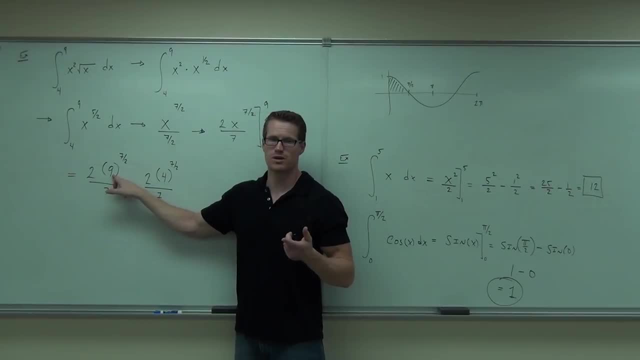 You can take either one, whatever you want. first I would take a square root of 9.. Square root of 9 is 3 to the 7th. That's what you plug in on your calculator. I can't do that in my head. 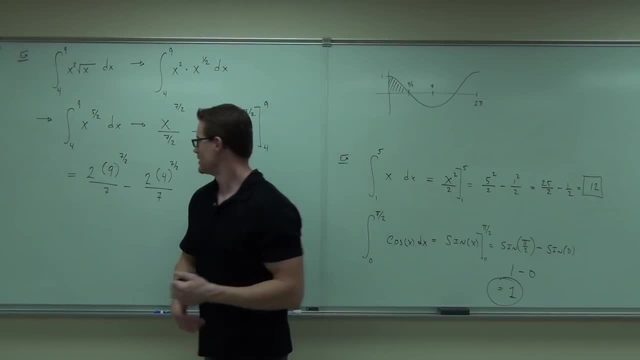 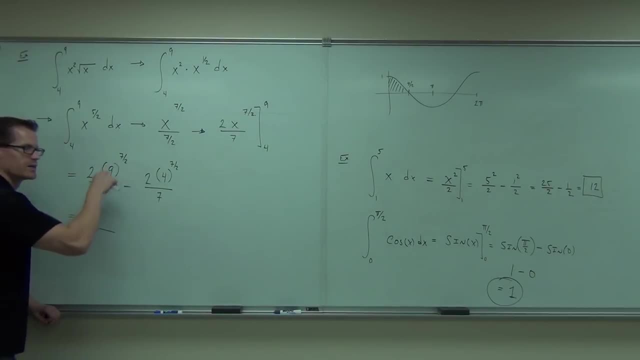 So this is 2 times. someone tell me what 9 to the 7⁄2 is, or 3 to the 7th, How much 3 to the 7th Minus this is the square root of 4- is 2, then you do 2 to the 7th. 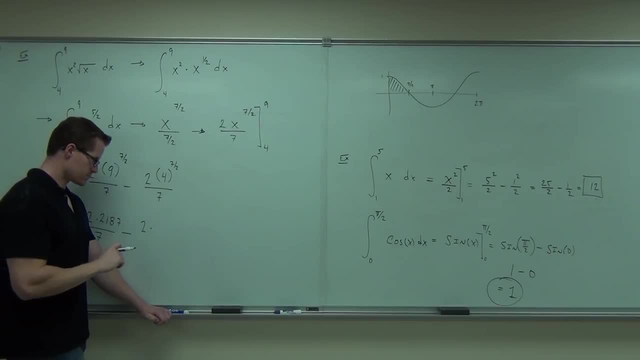 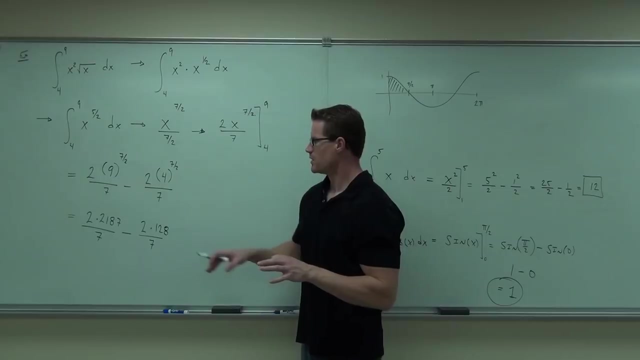 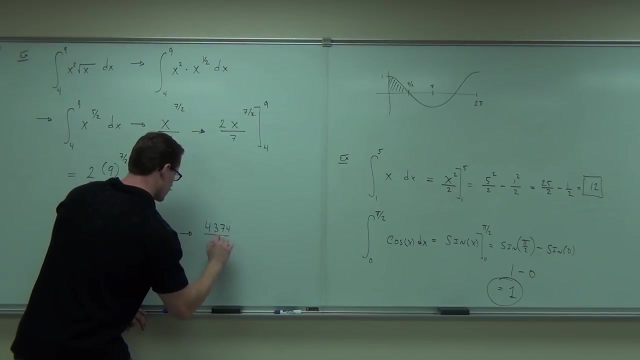 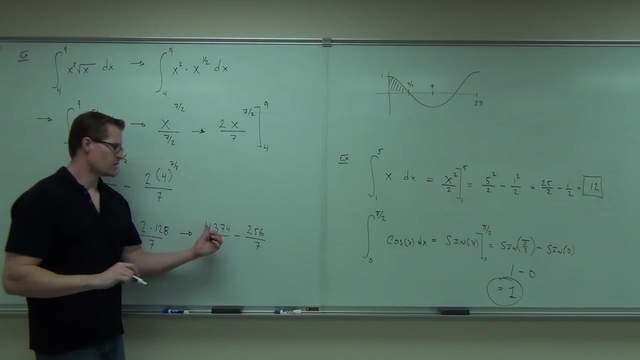 What's 2 to the 7th, The square root of 4.. Are you okay on getting those numbers out, ladies and gentlemen, 2 times 2187 is what This should be 256.. Someone give me, since we already have a common denominator. 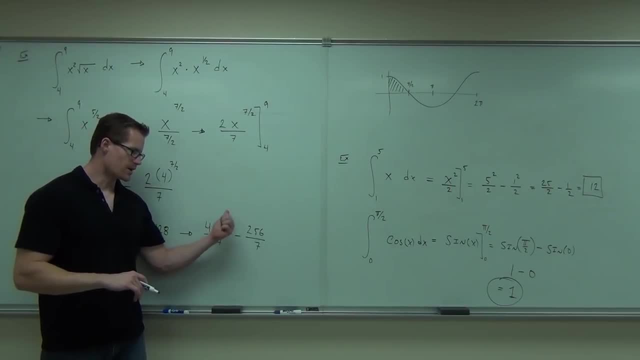 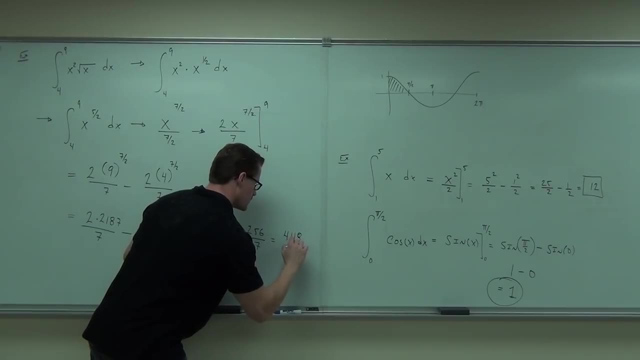 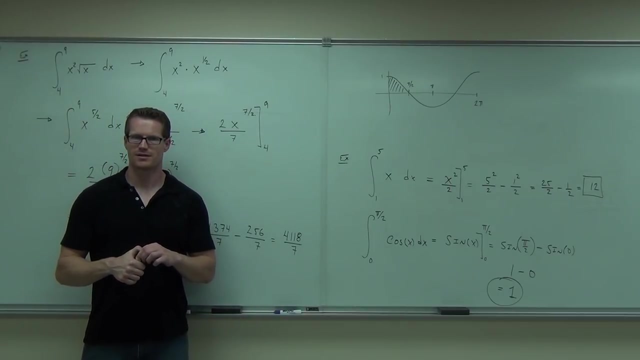 Someone give me 4374 minus 279.. 156,, please 4118.. Does that simplify at all? That's not. is it Y7?? Then you'll leave it. You could do a decimal if you really wanted to. 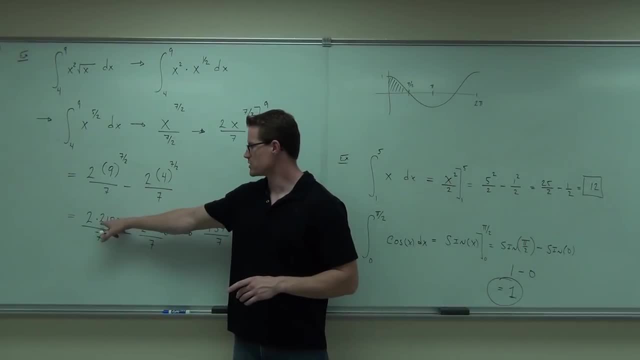 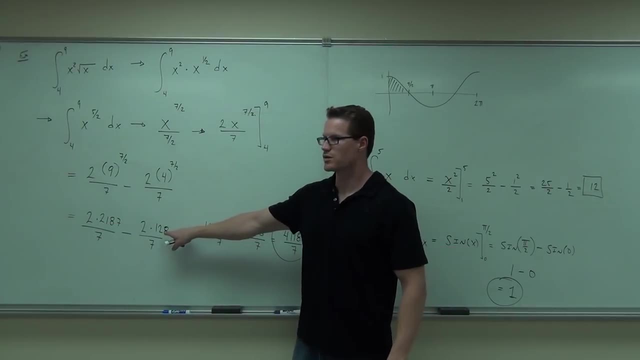 Let's make sure, before we end this, that our math is correct. Gotta get a double check on 2187.. You got that as well. Now you get a double check on the 128.. Same thing here as well. Alright, how many people feel good? 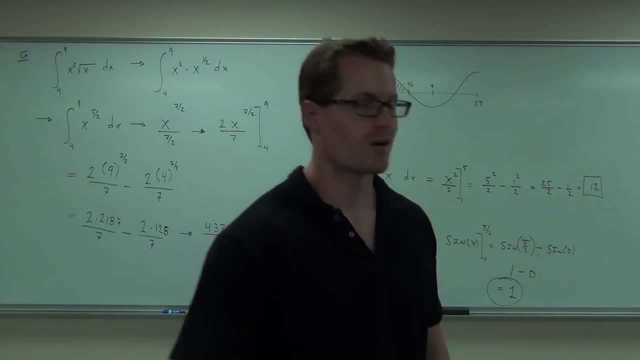 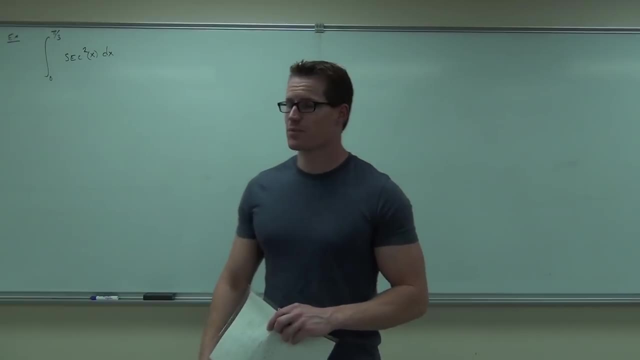 with what we talked about so far- Awesome. we'll try a couple more examples. We're almost done with our definite integrals, Alright, well, what do you say? we continue. some examples Here. we got the integral from zero to pi over three. 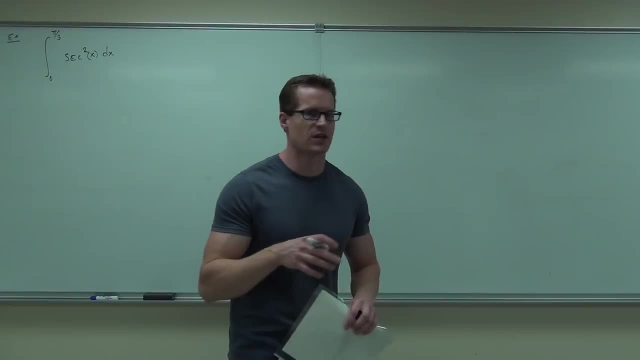 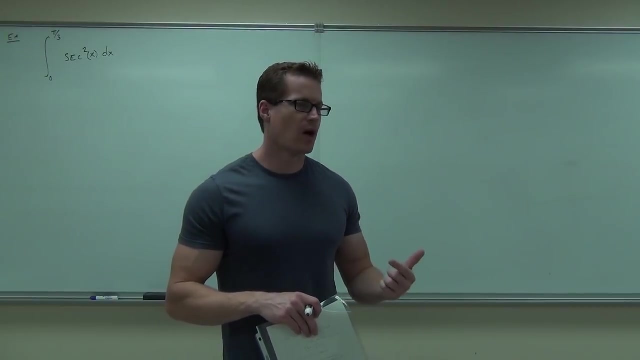 of secant squared x, dx. Now we don't have any substitution for definite integrals yet. I'm gonna show you something about that in a little bit. So right now, everything basically has to fit our integration table. What we learned last time was that 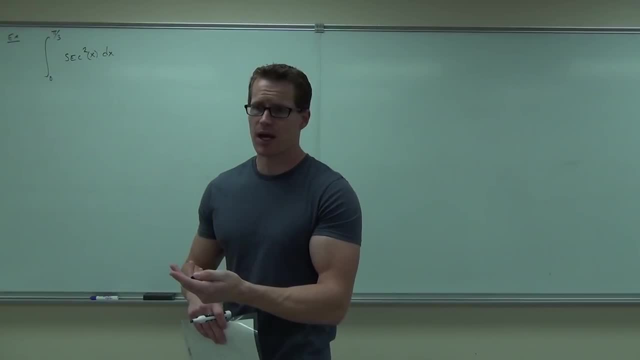 when we do an integral like this, a definite integral, we found out, firstly, how to do it and, secondly, that it's exactly like finding the area with the Riemann sum, or the sum of those partitions, which is very nice, very, very nice. 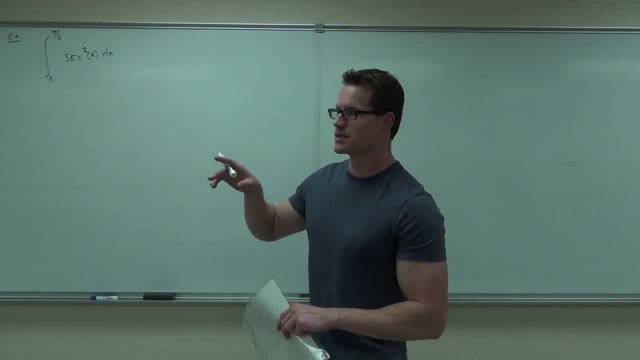 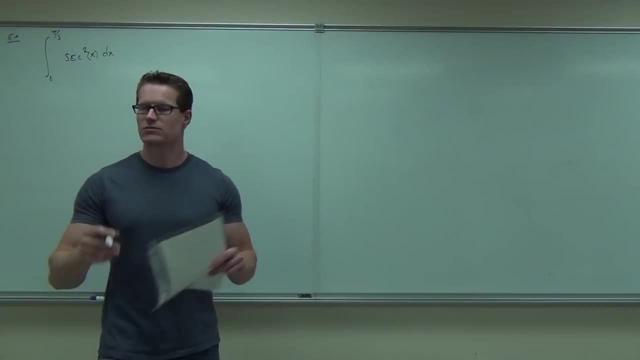 So let's go ahead and let's take the integral of secant squared x- dx. Do you all remember the integral of secant squared x- dx? Tangent, Tangent, Tangent, squared, or just tangent, Tangent, Good. So here's how you'd write that. 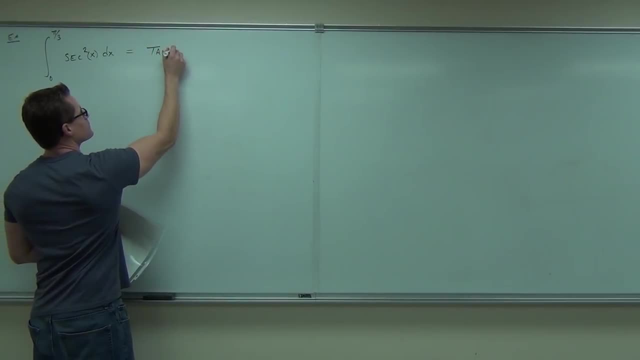 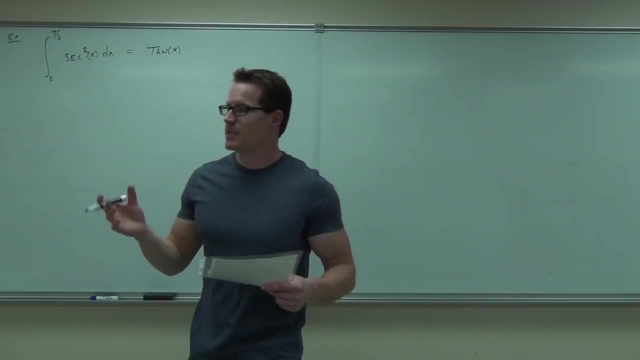 You'd say: okay, I know this is tan x, I know this is a plus c, A plus c or not, You know that one's never bound. What do I mean If it has bounds? no, because you're gonna find an actual area. 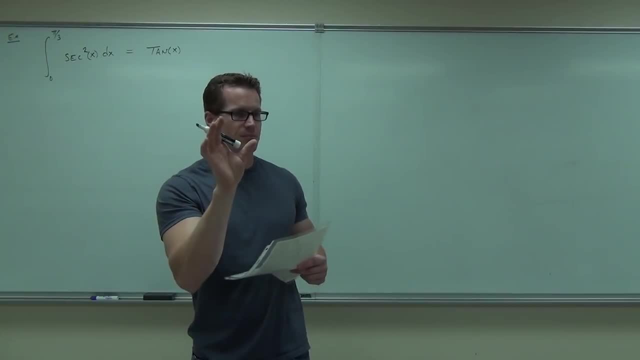 Because what you're gonna do right now is you're gonna be subtracting f of b minus f of a, And if those did include c, it'd be the same c. they would drop out of your equation anyway. So no, we don't have a plus c on this. 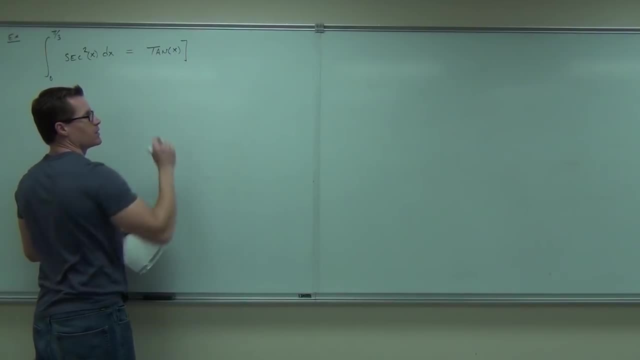 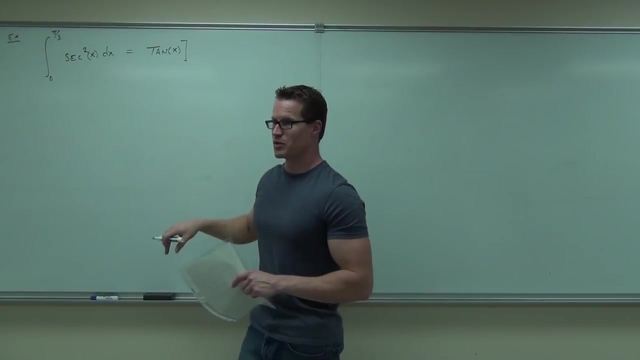 What you do do is you have this first and then you throw up. you don't throw up, sorry, That's when you get home for your homework. You put up The integration or, sorry, the evaluation symbol. You go. okay, I'm evaluating from zero to pi over three. 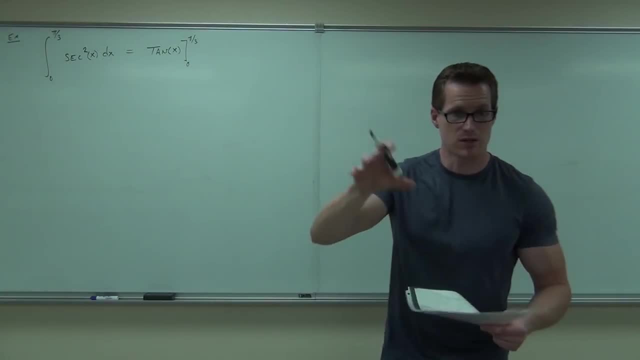 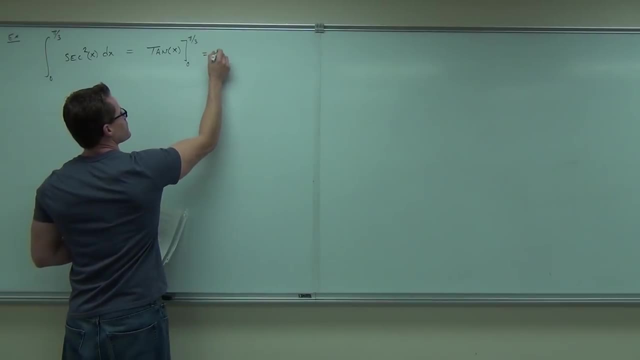 So, therefore, you show me what the integral is, You show me your bounds of integration, your bounds of evaluation, and then you plug them. in Which one do you plug in? first zero or the pi over three Zero? Okay, so what this says is: 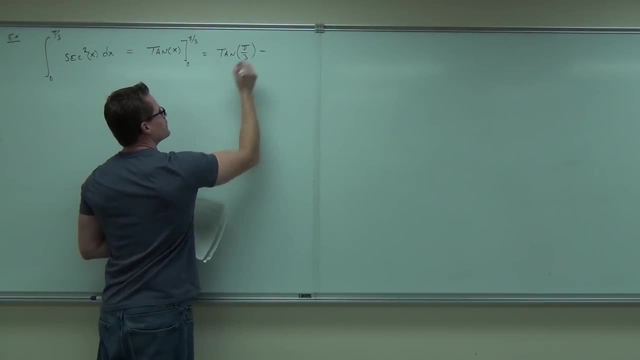 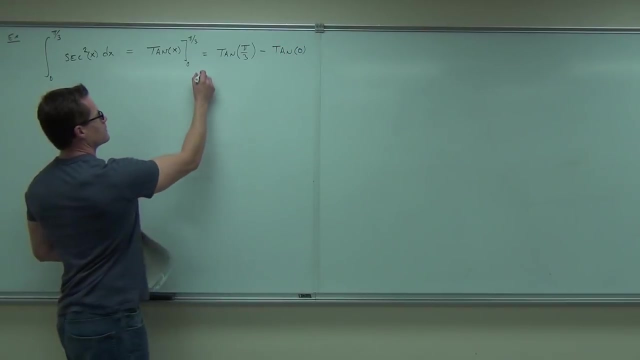 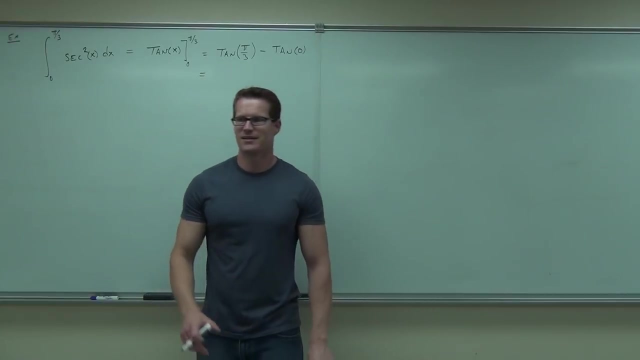 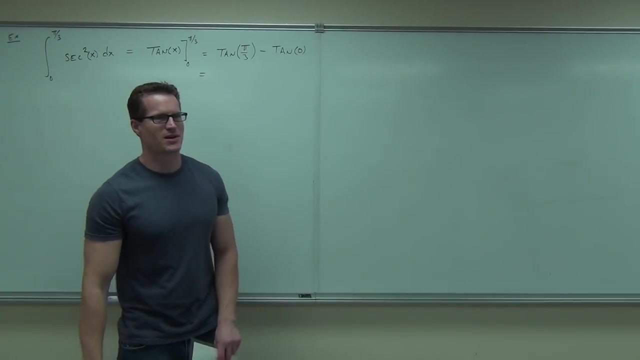 tangent of pi over three minus tangent of zero. Well, that's not too painful. How much is tan pi over three? Don't leave me hanging Awesome 1.73, like my calculator says. Yeah, okay, very good. 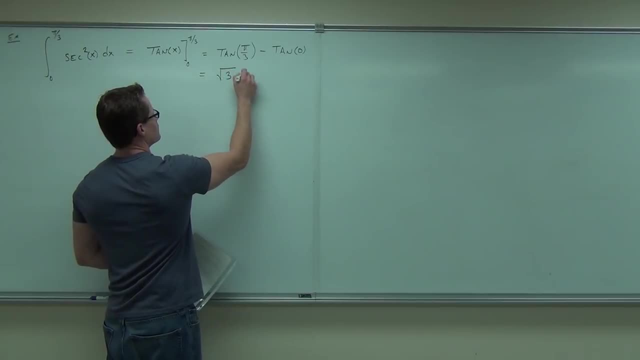 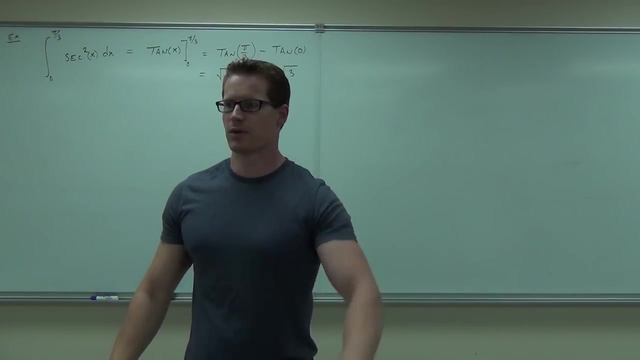 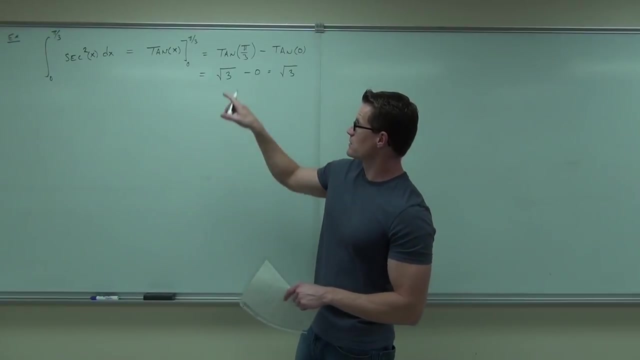 Learn to unit circle: Root three. Root three over two, divided by one, One half, reciprocate, multiply, you get root three. That's because it's sine over cosine. Ah, ah, you need to know that. Okay, anyway, so we have our integral. 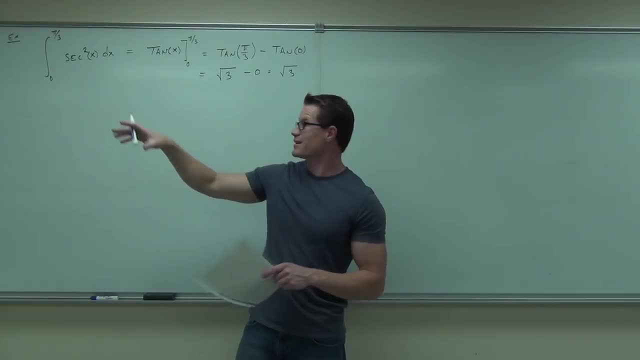 the area underneath the curve of secant, squared between zero and pi over three, is: ah- ah, we got it- square root of three. It's interesting, right? It's kind of weird that we're able to find those areas so nice and neatly. 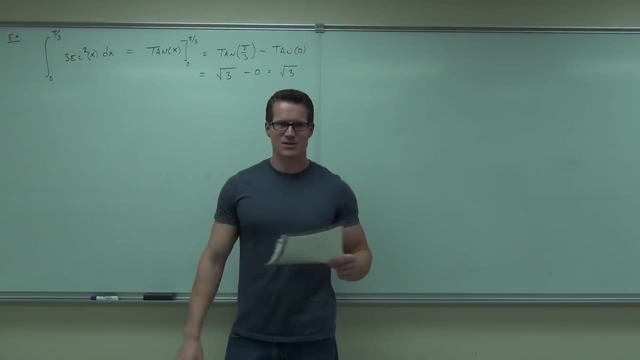 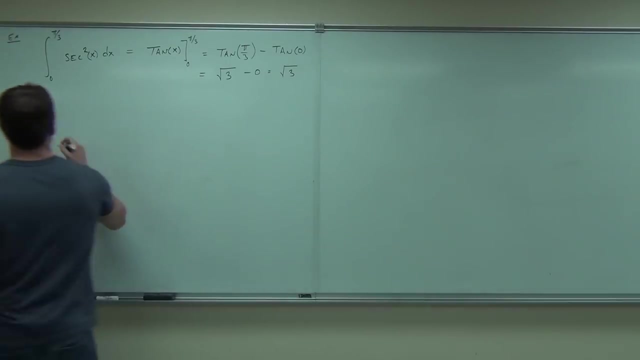 Are we gonna try a couple more of these things? Yes, no, Yes. Did that make sense to you, Besides the square root of three, which you all just kind of screwed up right now? All right, You have so much faith in this one. 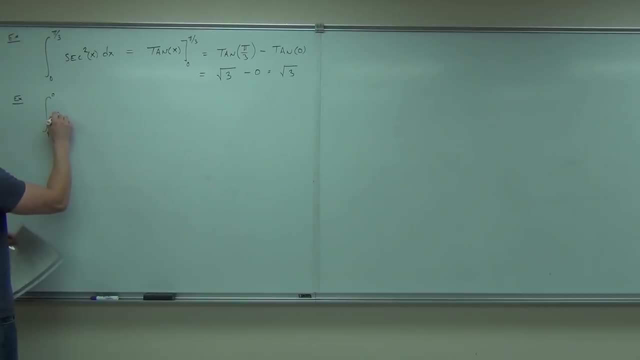 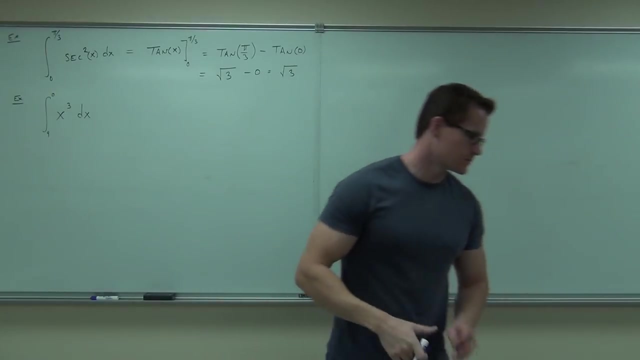 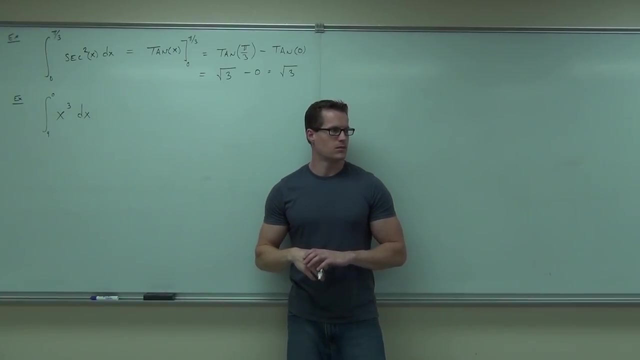 Hey, you're the one who screwed up, not me. Okay, explain to me something about this problem. You have to invert it and change it to negative or to zero or whatever. Okay, very good, explain why. What's wrong with this problem? 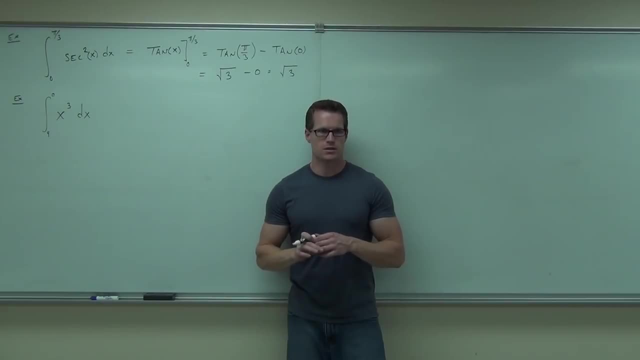 It's backwards, the bounds are backwards, It is. It should go from smaller to larger bounds. In fact, you know what, if you did it like this? if you did, you would get. I don't believe you'd get the right answer actually. 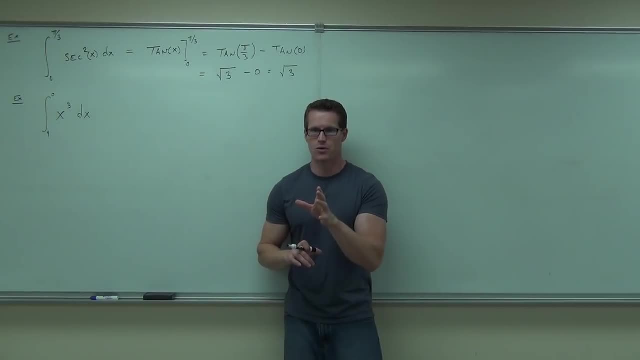 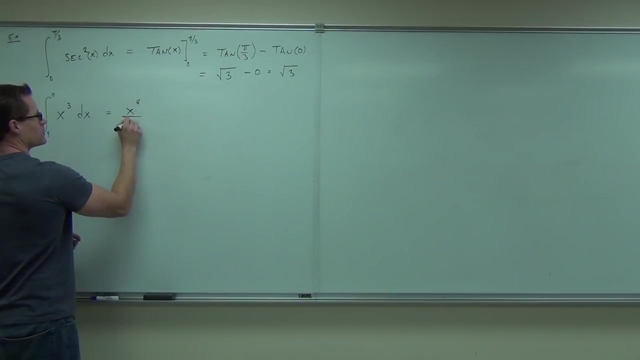 If you try it right now, you'll get the right answer, but that proves the statement that we made before, that this is gonna be negative. So, for instance, if you did this, you'd get x to the fourth over four right. 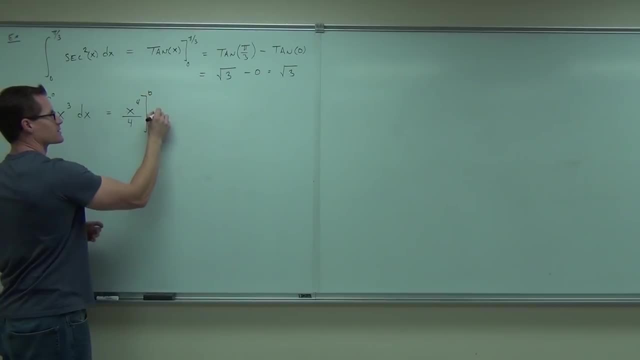 No plus C. but if you evaluated from four to zero, like it says, you'd have zero to the fourth over four minus four to the fourth over four. So what that would end up being is negative four to the fourth over four, so four cubed negative 64.. 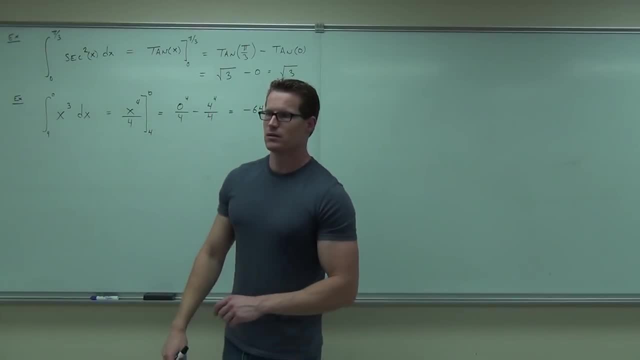 So if I've done my math correct, Did I do my math correct? Yeah, Yeah, Now let's check to see if we get the right answer the other way as well, We also knew from a property that, if I reverse this, 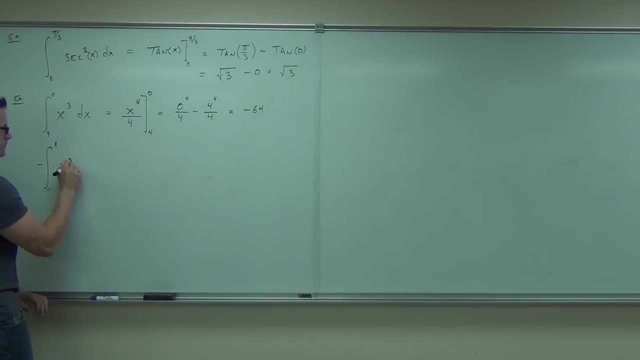 and go zero to four, that becomes a negative. Well, let's see That would be negative. x to the fourth over four, That would be negative. See the brackets there, because you can have a sign in the middle of that- And that's evaluated from zero to four. 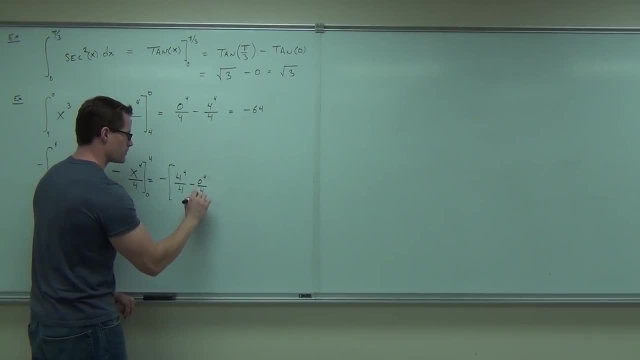 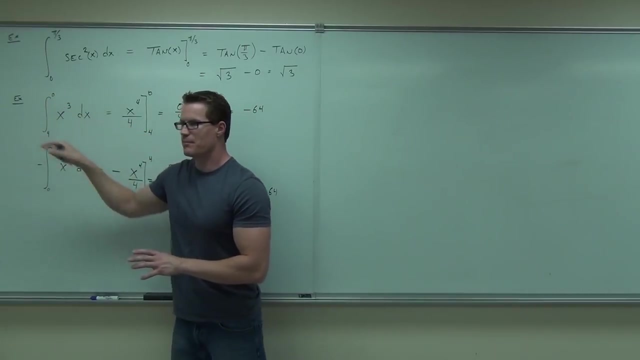 Four to the fourth over four minus zero to the fourth over four, And that would give you negative 64 to 64, which, by example, kind of proves that that was true, that I can reverse my bounds, and that makes me change my sign. 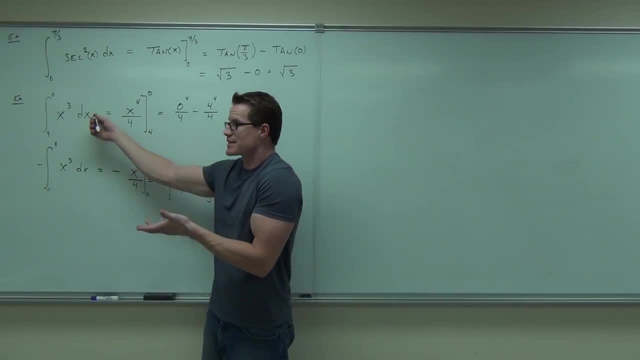 So just by example, we see that that is true. Notice how you do actually get the same exact answer either way. That's because it is true, It has to be. What it represents, though, is kind of awkward, because this looks like it's an area above the x-axis. 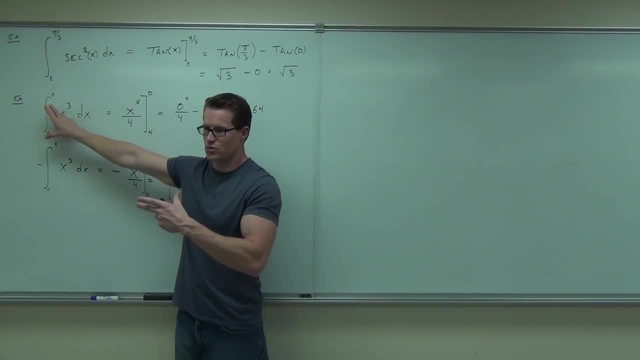 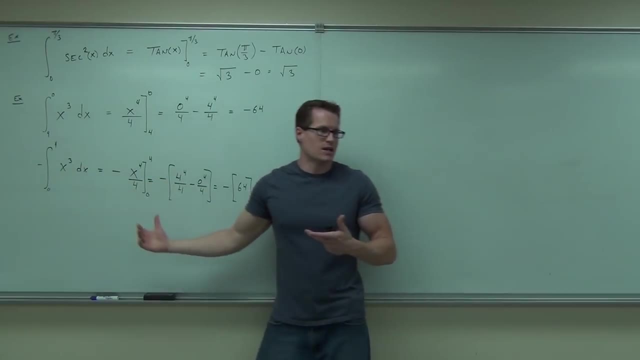 when in fact it's not. This is just read wrongly, incorrectly. So the correct way to do this problem would be to write the bounds in the appropriate order, with the negative out in front of it, and that would give you negative 64.. 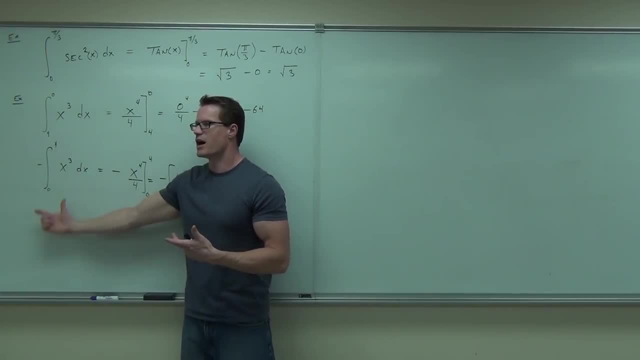 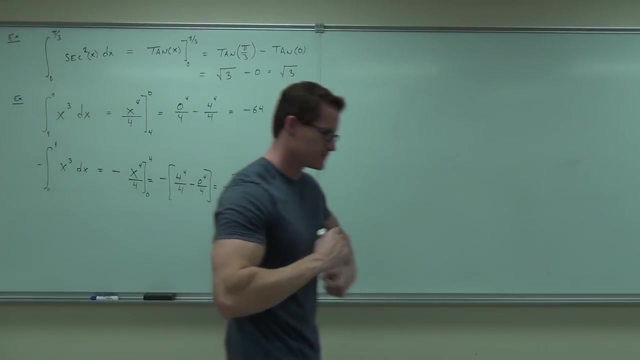 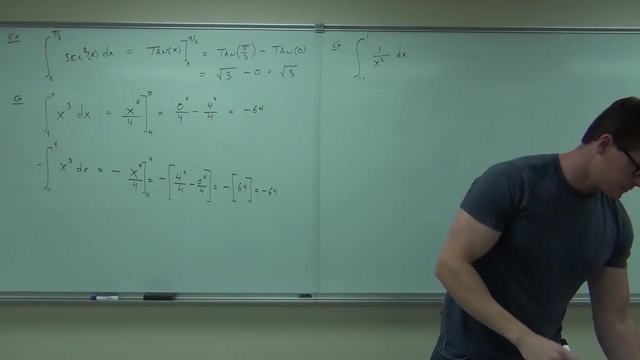 Either way, but this is kind of showing you- okay, this is an area underneath the x-axis, not above it- How many of you feel okay with that one? Okay, Oh, lost it. Okay, We could bring the x-axis to the top. 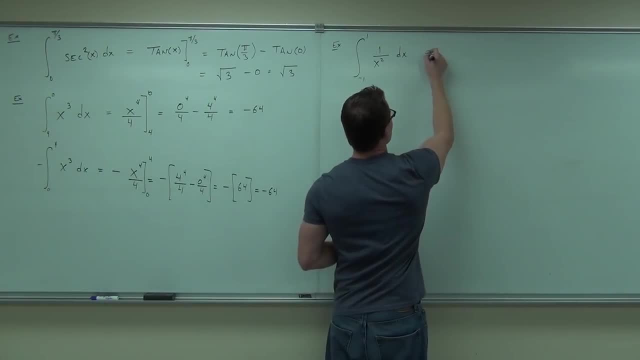 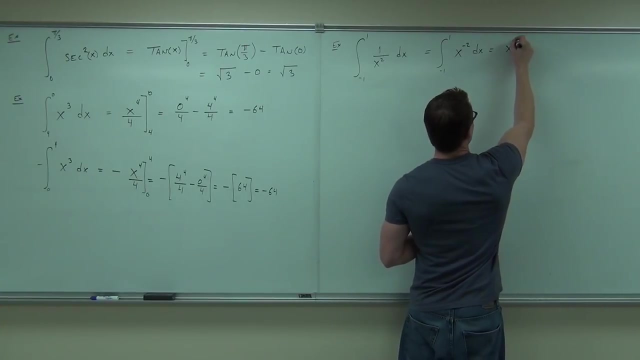 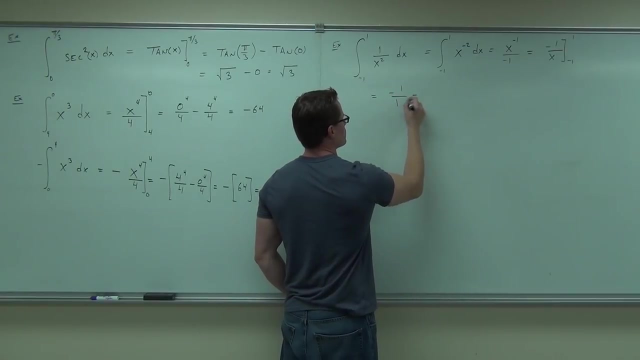 We could bring the x-square to the top. No one. There we go, There we go. Couldn't figure out how to say it, but Okay, all right. All right, So you'd have negative one over one minus negative one over negative one. 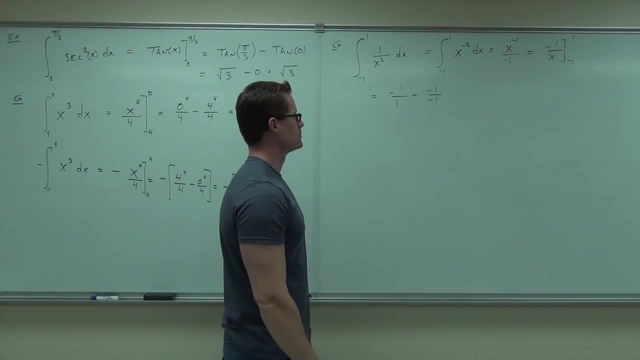 Do you have negative one over one minus negative one over negative one? Yes, No, Hopefully, if I did that right, make sure my signs are correct. I'm looking at that as negative one over one minus negative one over negative one. 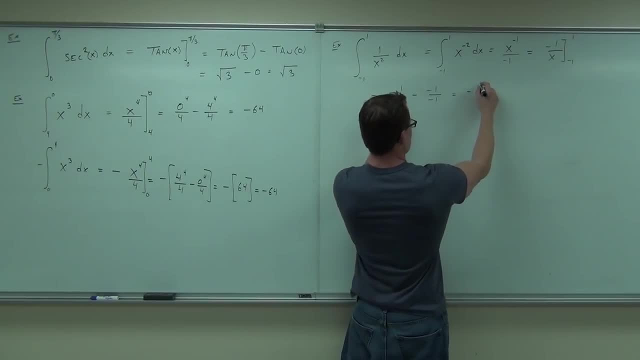 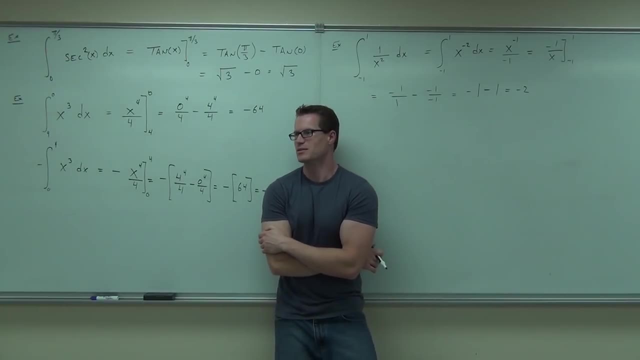 That's negative one. Okay, All right. What's negative? one minus one? Negative two? Yeah, You get an answer. You do, But now think about the answer. I can have a negative area. Well, you can have a negative area. 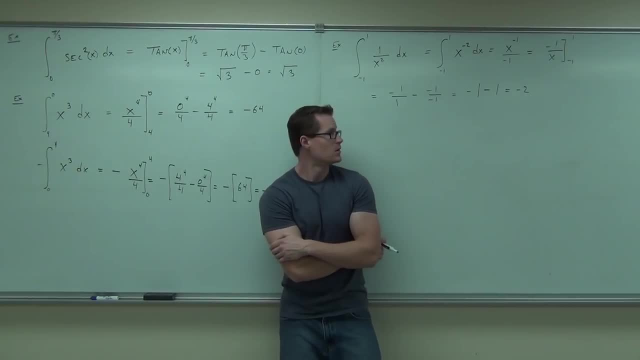 It would mean it's underneath the x-axis. That'd be okay. Think about the function, then Graph it on your graphing calculator. if you can't think of the function, It's a domain. Why? Because it's negative? No, not because it's negative. 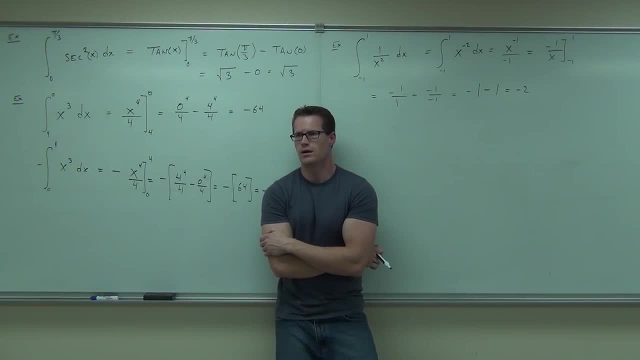 Think about the function. What's the function do? I don't want to draw on a crayon for you. Think about what the function actually does. We have done so much in this class for you not to know this. It has asymptotes. 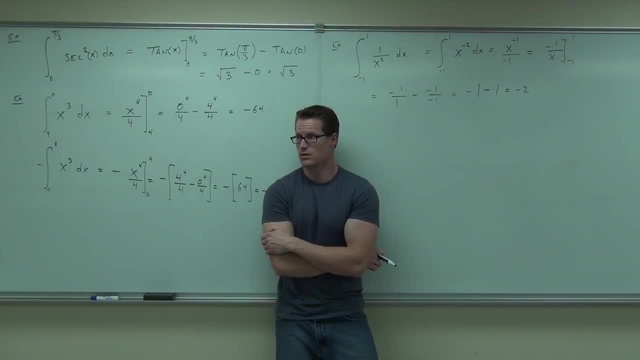 Say what. It has an asymptote. Where does it have an asymptote? That's x-axis and infinity. Okay, it does have those. That's okay, though, because I'm between negative one and one. I'm between them. Draw the graph if you have to. 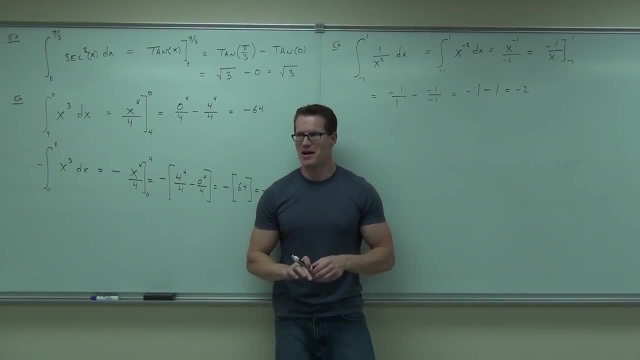 Draw it. You should know the shape of that graph. You really should. Okay, you're gonna make me do it. You're gonna make me, oh my gosh, Plug in zero. Plug in zero. Can you plug in zero? 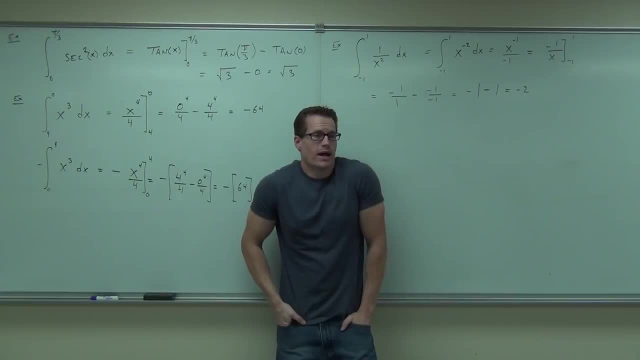 Why not? So what's it tell you: at x equals zero. What do you have? Look at your bounds. Where do they start? Okay, so are you adding up areas that actually are undefined at zero? So it says you're making rectangles. 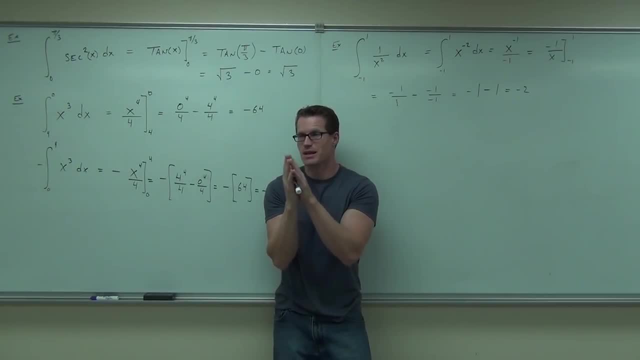 One of those rectangles is going to infinity. Do you see it? It's probably infinitely. many of them are going to infinity because when you go that close you're gonna end up in infinity anyway. So can you actually add the area? Even though you can do the work, that doesn't exist. 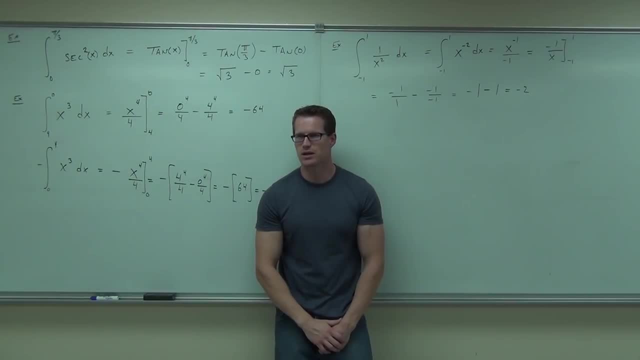 There's a, you can't do it. There's a theorem in calculus. I don't think I get to it, but basically it says that if you're not bounded somewhere, if you're not bounded, you can't add up those areas. 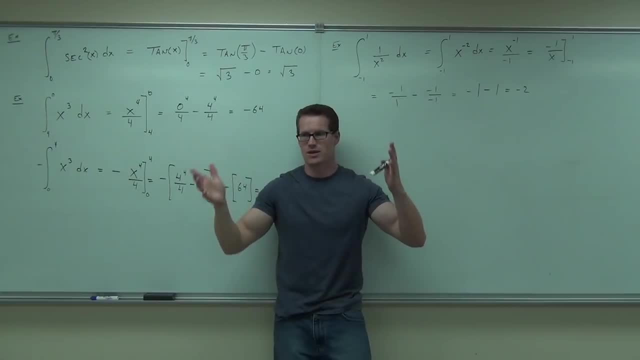 So if it goes on forever in one direction, right, you can't do it, So you have to have that. Here we have an asymptote going to infinity. We're not bounded in any way, shape or form. Therefore, that area cannot exist. 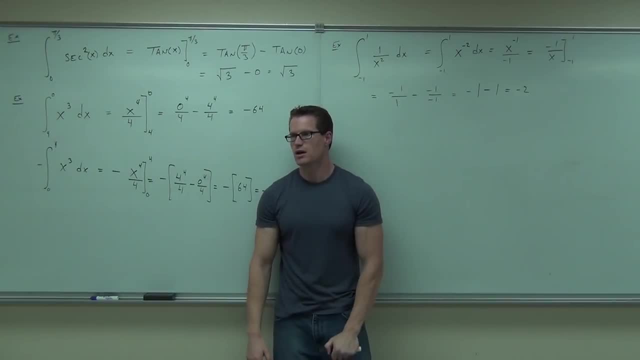 Or it does exist but you can't find it using the methods that we use. There could be something else. I'm not sure if they have a way to do that. I'm not gonna sit through right now, But I for what we know, that doesn't work. 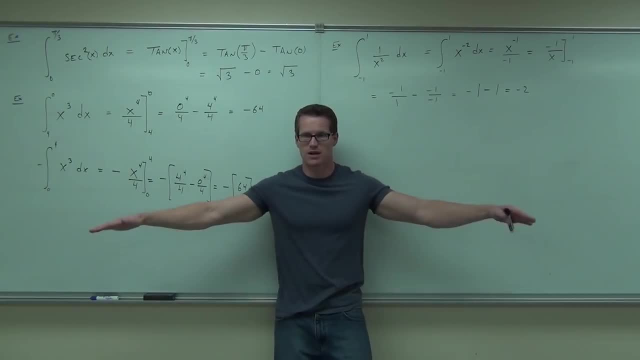 It's not negative. two: If you think about one over x squared, that's positive anyway, isn't it? And if I did my signs wrong it would come out to zero. I don't think I did my. did I do my signs wrong? 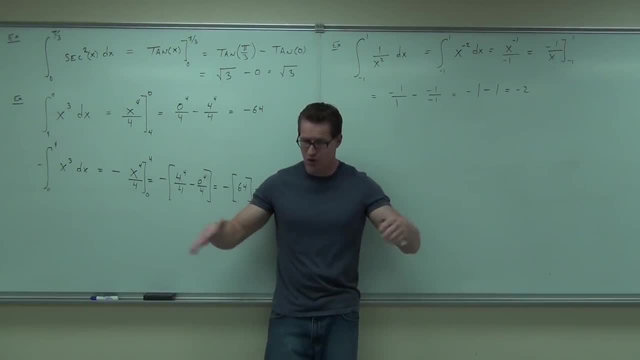 Oh not, I did it real quick, But if you did it would just come out to zero anyway, which you know. there's an area it goes like this: It's a positive area, so that it's not, it makes non-sense. 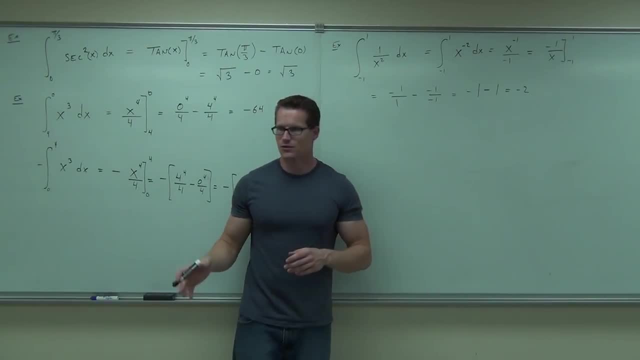 And it's because there's a domain issue. You had it right. it's not the negative, it's the fact that that we start here, we end there and there's a problem between them. That would be the problem. Do you get it? 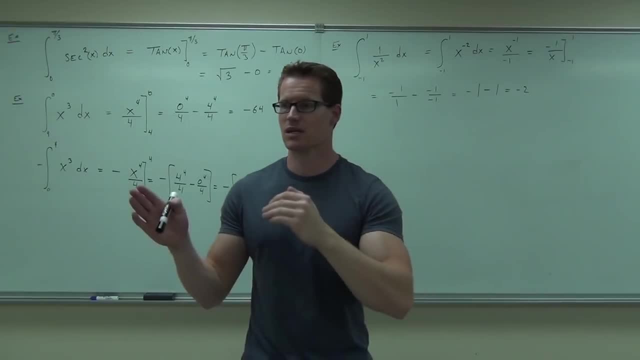 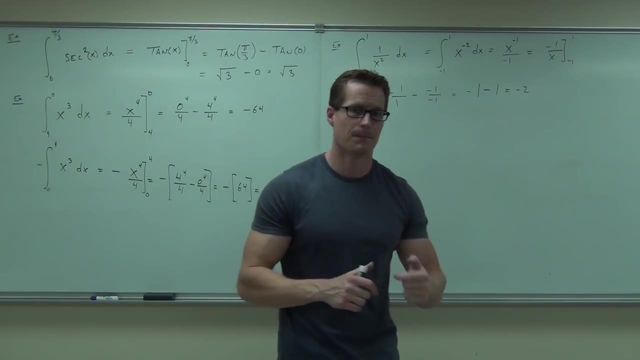 There's a problem at zero. Zero is between negative one and one. You have to be at least bounded between there. Typically you have to be continuous and bounded, and that would make it work. Yeah, even if our bounds were a little bit wider. 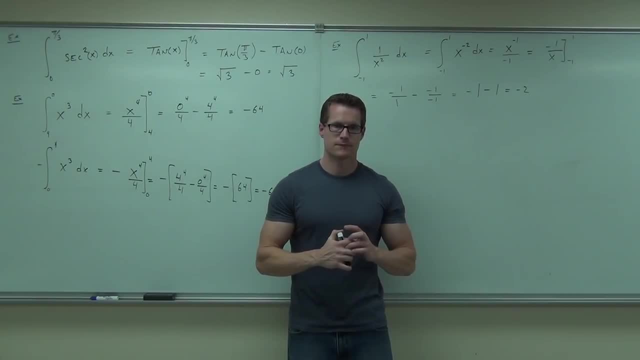 it still wouldn't be undefined, since that you can't measure between. measure at x equals zero. What I mean by bounded isn't this way. I mean this way. You have to have this. Here's a curve between these two points. 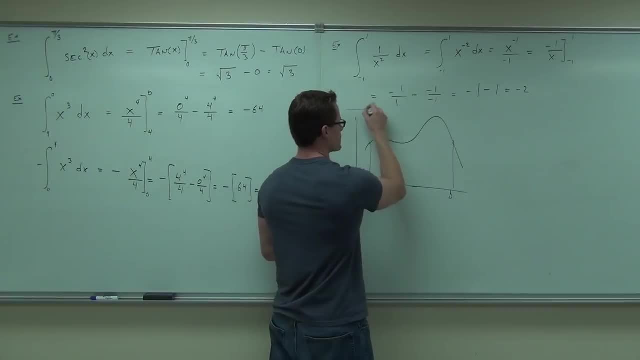 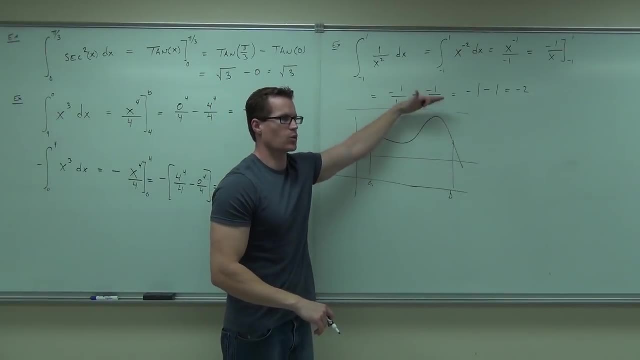 It's gotta have a low point and a high point, which means you can come up with something here and come up with something there. that's between. Actually, really, it's just. if you're just talking about the x-axis is only above, it just has to be bounded above. 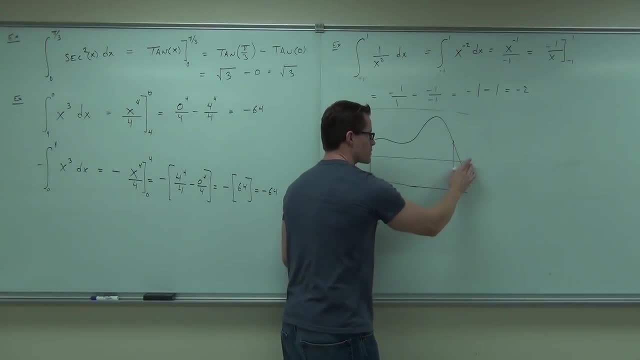 It doesn't go anywhere. If it was below the x-axis, it'd be bounded below, So this one's really irrelevant. when you're talking about the x-axis, That one doesn't matter, But you find an area here. it's gotta at least. 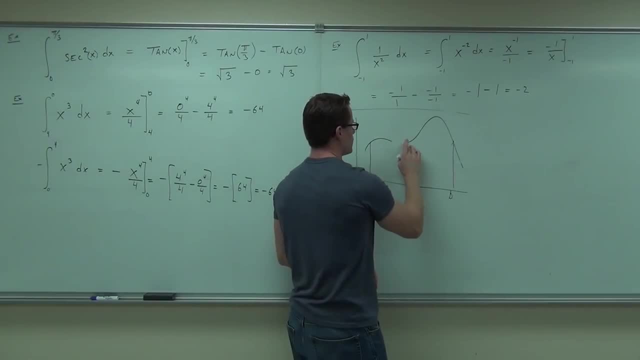 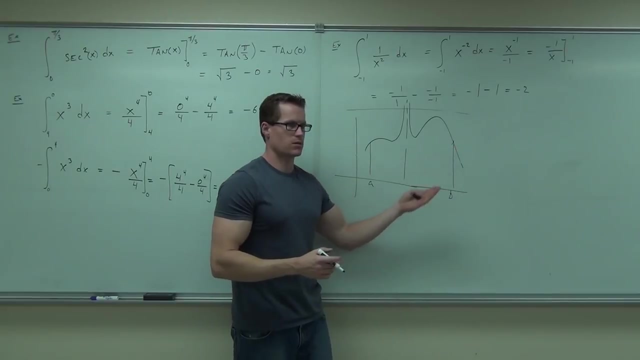 be bounded above. When you do something like this, hopefully you see the problem. Do you see the problem? How are you supposed to add that area up? That goes to infinity? You can't do it, doesn't? I don't know what the area is. 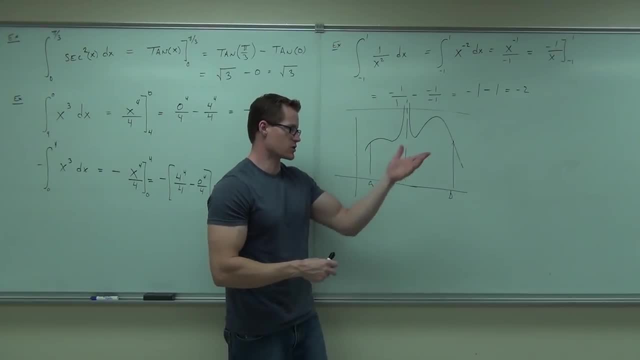 I don't know if you can. if you can say infinite area, I would assume so, because it's going to infinity, But you can't calculate it like this, Like this. How many people understood that? where the problem is, What's the problem? again? 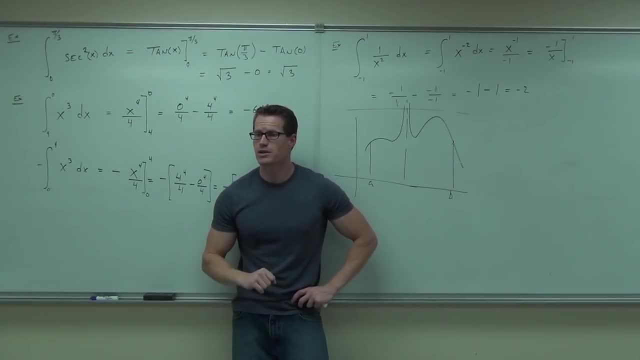 Explain it to me again. What's the problem? Domain issue, Domain issue. Why a domain issue? Someone else Domain issue? Why? Because it's undefined Where, At zero, At zero. And why is zero important? It's in our interval. 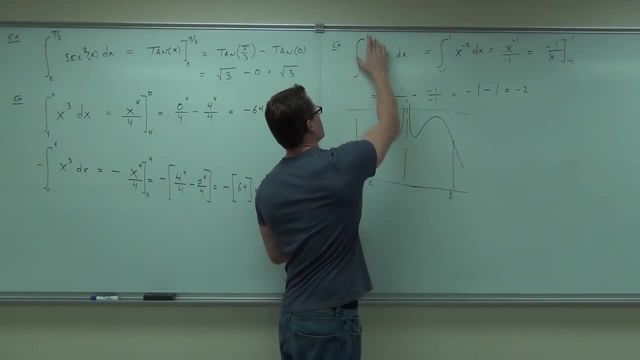 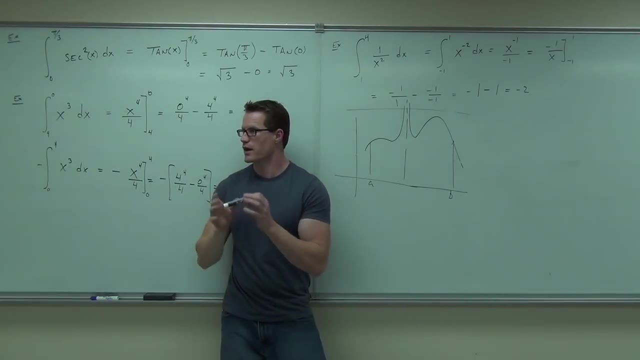 Aha, Aha, It's actually in our interval. If I had done this, would there be a problem? No, Not at all, No. But if I cross over that undefined area, No, Not at all, No, It's something like this: 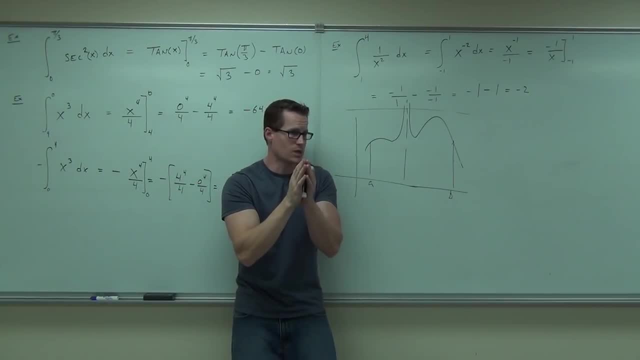 It's an undefined point where we have a domain issue and going to infinity, that's an issue for us. We can't do that Now. is that kind of clear for you? All right, You guys had it Come on. 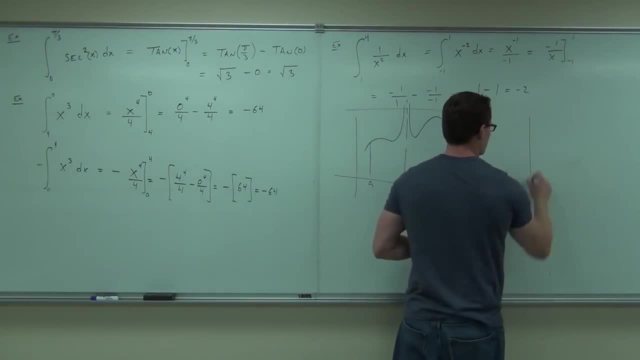 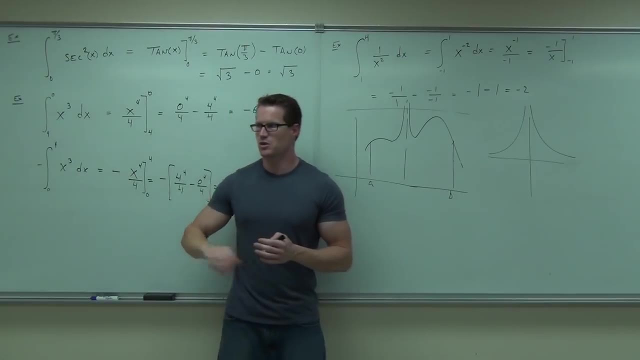 You should have known that. You should have right off the bat. You should know that this picture looks like this too, Like that, Just by thinking about asymptotes. you should know that Asymptote going to infinity is like this: 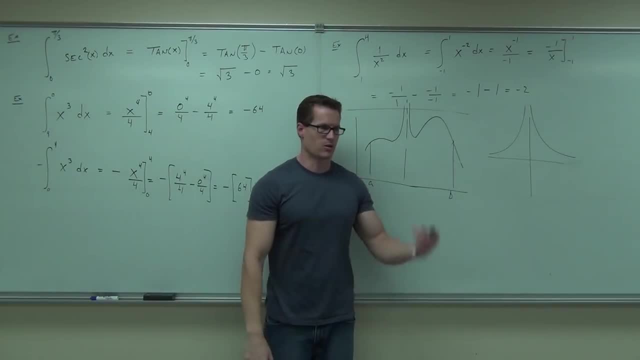 Asymptote in the middle goes like this: Signed analysis says they're both positive. Pulling it into positive: it's positive. Pulling it into negative: it's positive. It goes like that. You should know that, All right. 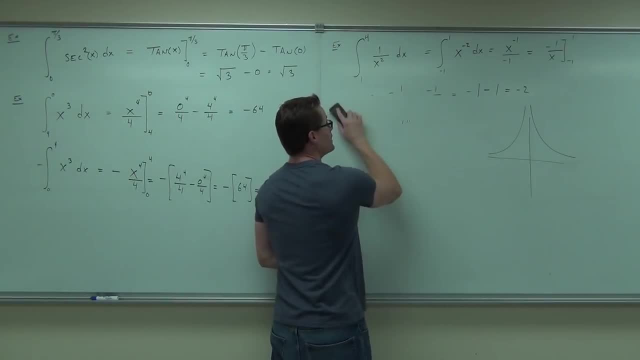 Bye, Anyway, this. none of that works, so we just put undefined for it. Well, this one you would do. Oh yeah, the new one we would do. but the original problem would be to try undefined. or You would explain to me that there's a domain issue and that since our bounds are going, 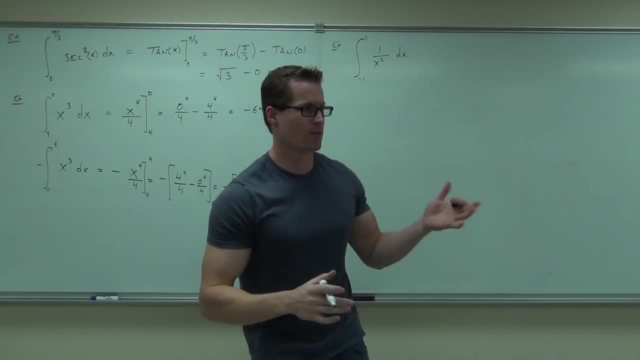 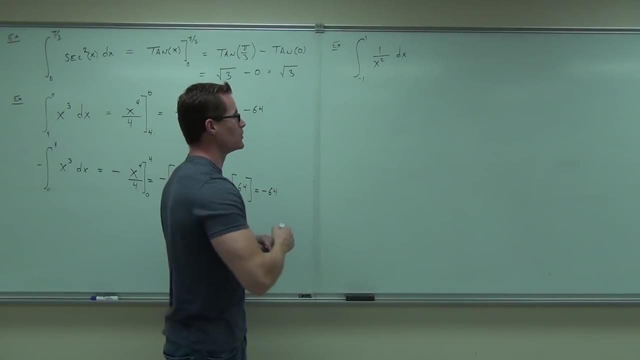 from negative one and cross over somewhere where we have a vertical asymptote. therefore, we in no way can find the area of that curve between those two points. Okay, now let me show you one more thing that we can do. Are you ready for it? 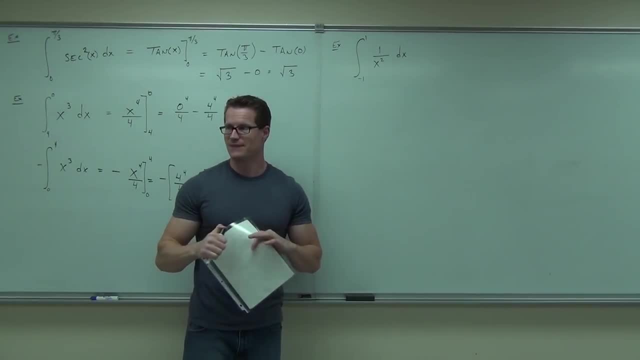 Yeah, Were there any more questions on that one? That was a good one, huh, Because it looks like you can do it and you do it and you go. ah, I win negative two, But you don't think about what the function actually is and it burns you. 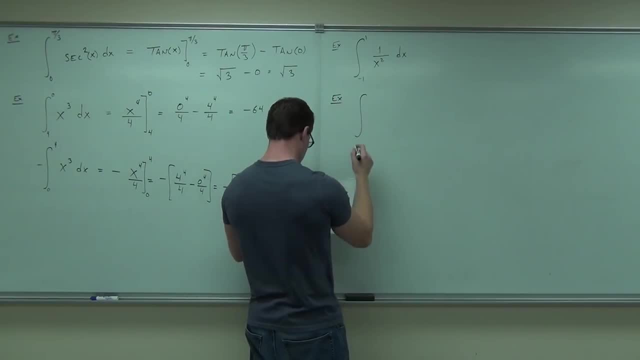 You don't want to do that. By the way, don't assume that all of them are going to be like that on the test. So if all of you go, oh yeah, it's got a domain issue, I can't do it, you're probably mistaken. 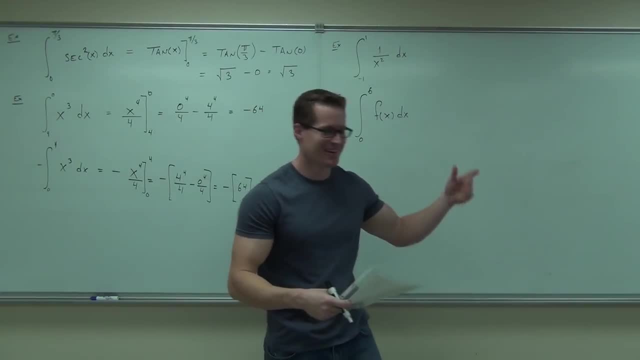 I'm not going to give you 20 in a row. I'm going to give you 20 rules that you can't do. okay, You might get one of those 20, right? Yeah, maybe one, Maybe, Maybe one. I always find that funny. 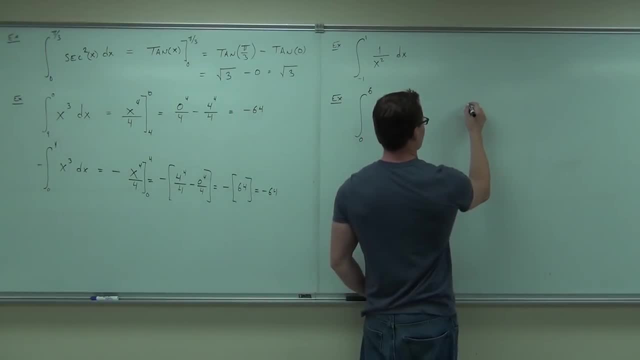 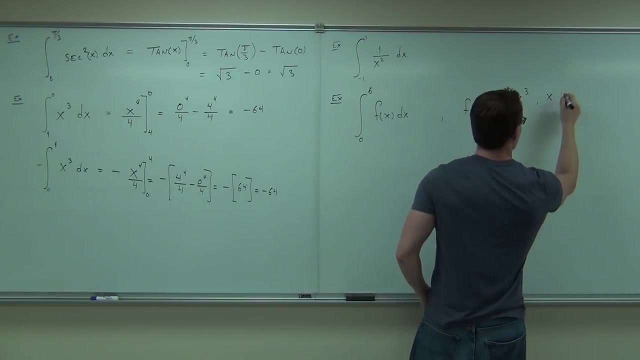 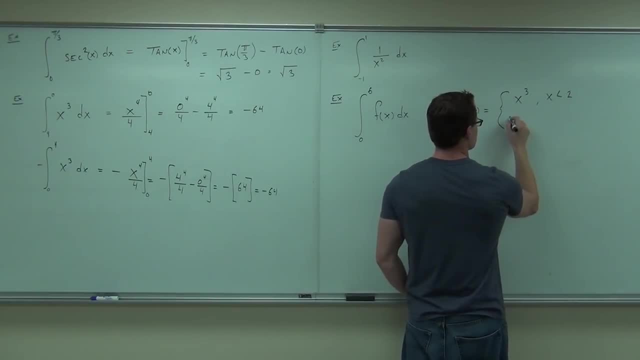 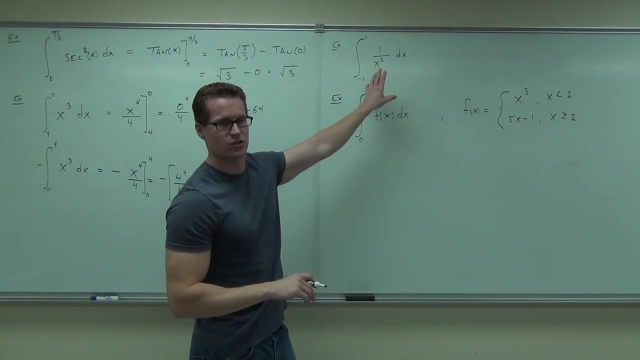 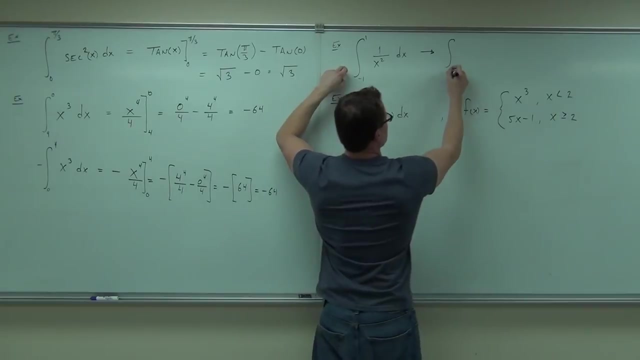 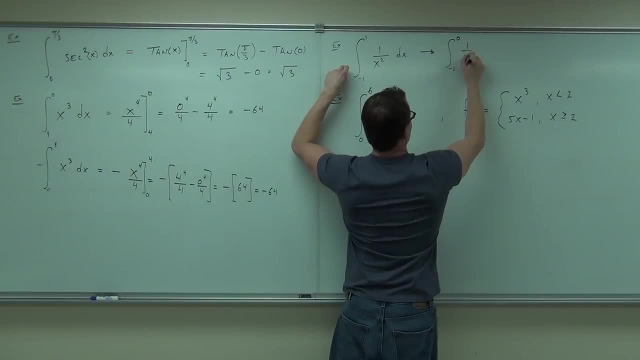 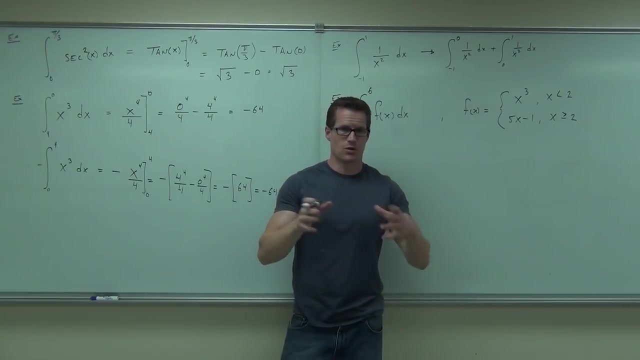 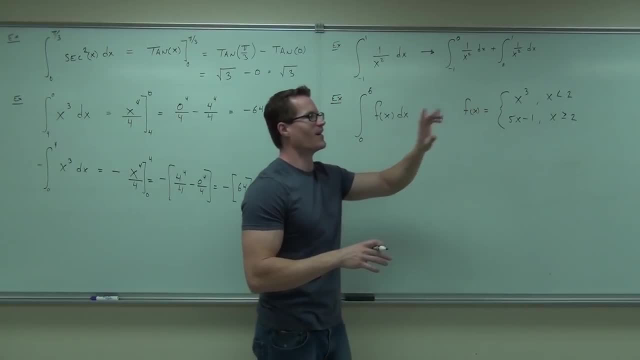 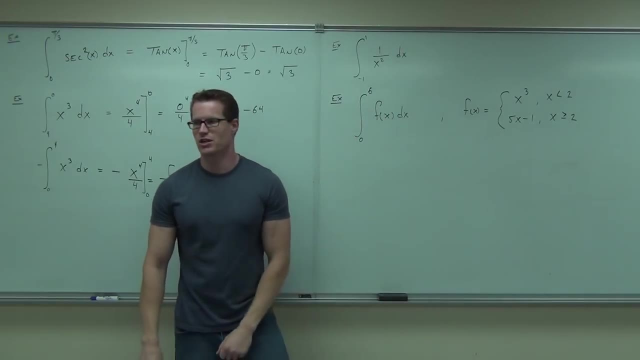 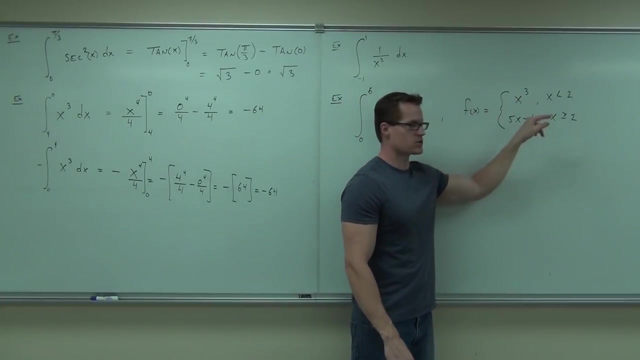 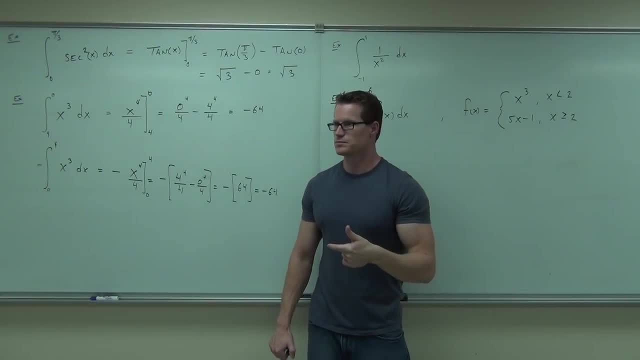 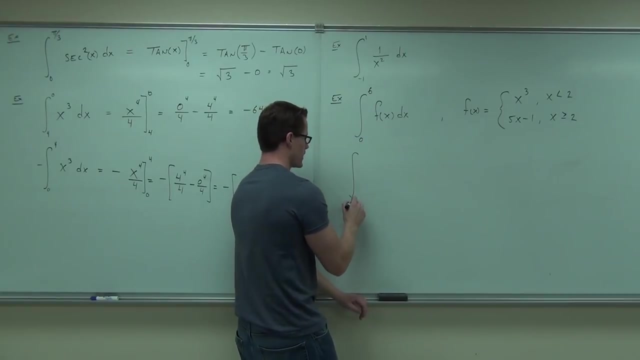 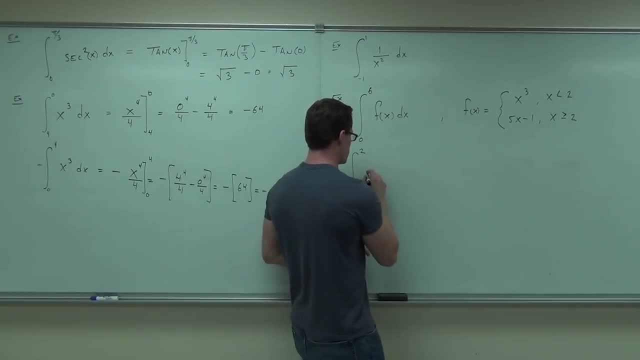 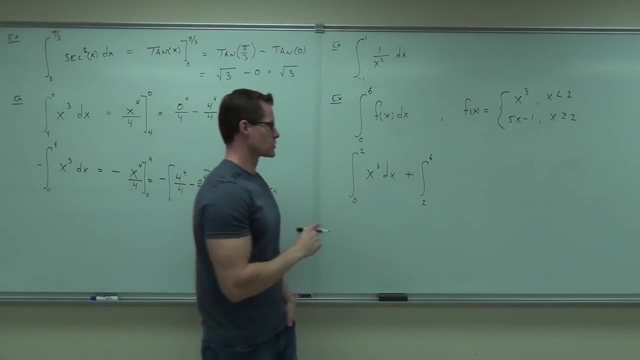 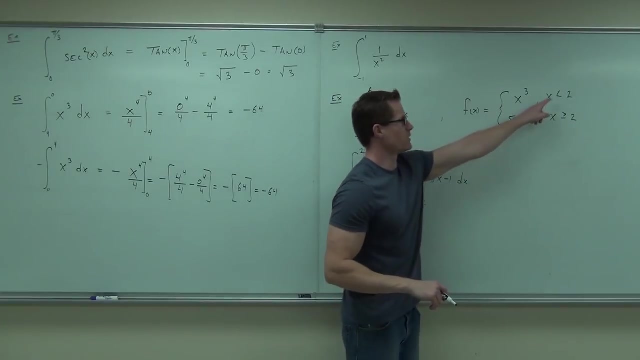 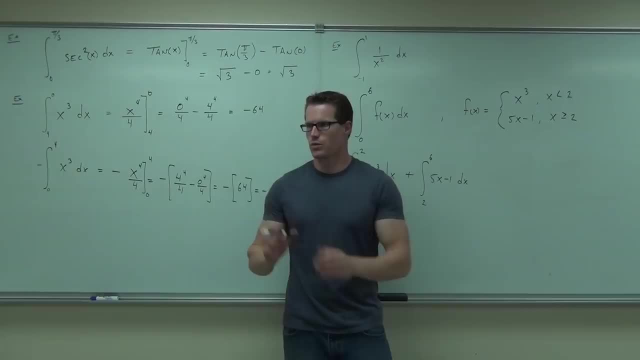 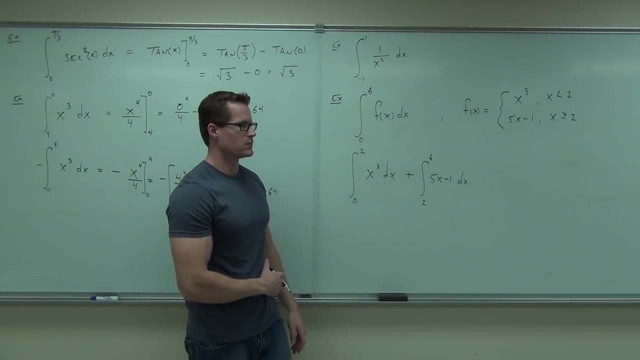 than 2 and this one's greater than or equal to 2? No, not really. We have such small rectangles it doesn't really matter. They're all going to match together anyway. so no, not really. If you had to say that it wasn't greater than or equal to 2, then it would say it was just. 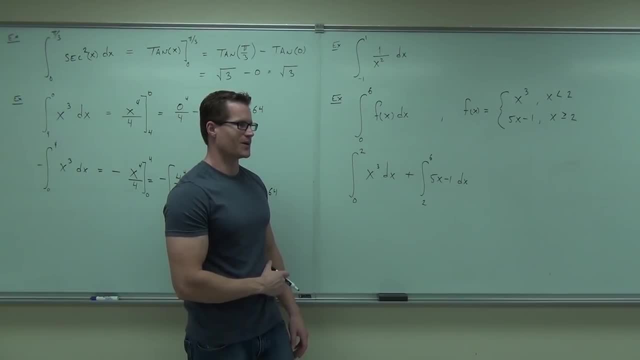 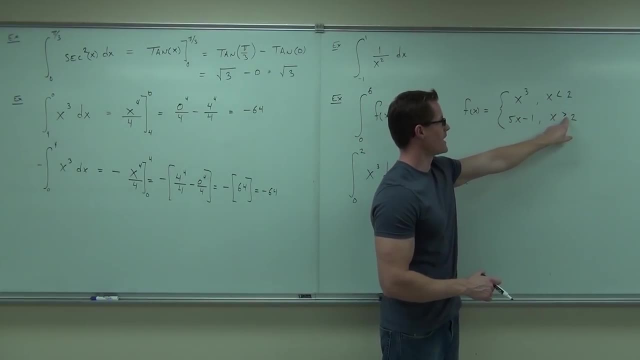 greater than It wouldn't matter, correct, Because you would have a gap right there. No, It'd still do it, Although, wait, wait. Did you say that this one changed? No, the one below. Oh, that didn't have it. 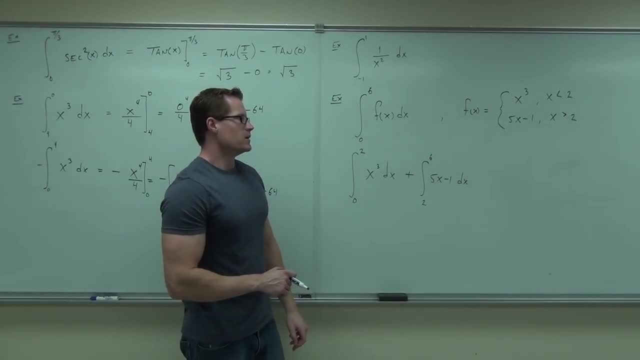 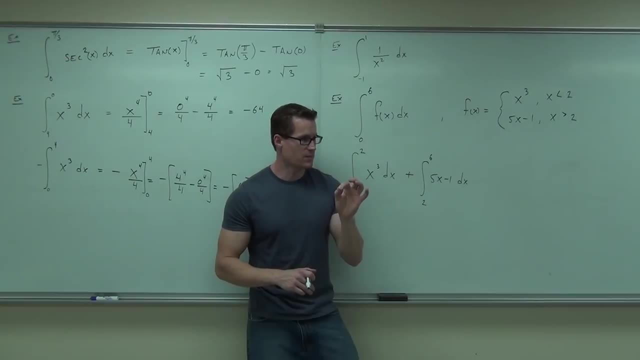 Then you'd have an undefined point. Yeah, I'll say it this way: The area of one point doesn't even exist anyway. So you could technically do it with two different integrals, because the area of that one point doesn't matter. 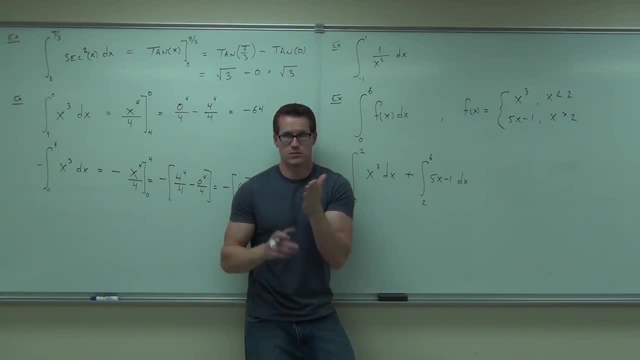 It's one point. The width of one point is 1.. Yeah, You can't do it. There is no width between one point. It's a point, that is, that which has no breadth, which means it does not have a width. 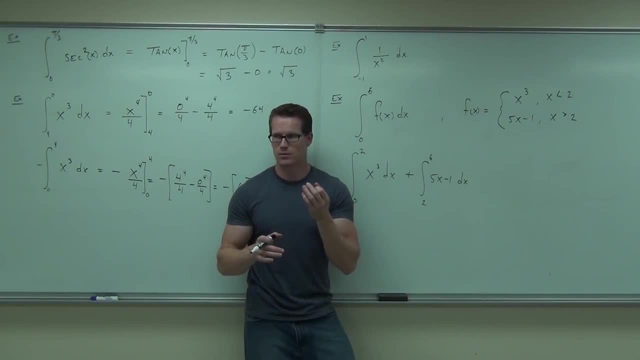 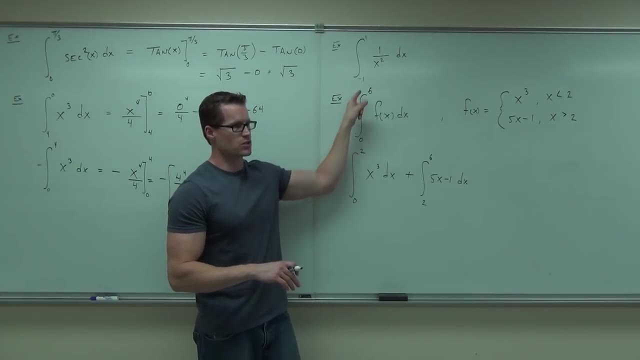 No matter what the height is, the area would be 0 of that single point. However, this wouldn't make sense. from 0 to 6.. This one couldn't be given to you like that, because this says continuously from 0 to 6,. 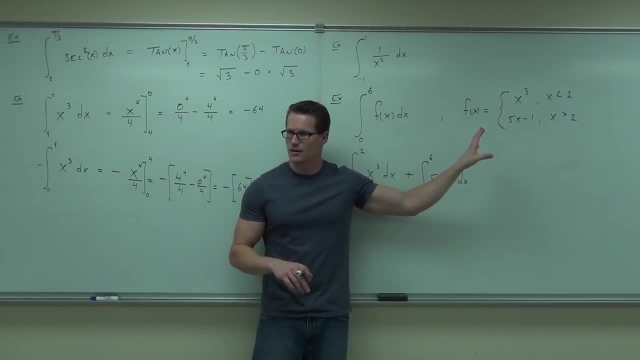 and so that really wouldn't make sense. Does that make sense? I couldn't do that to you because you wouldn't have the ability to do that. Yeah, Yeah, You wouldn't have the ability to break it up, because to break it up, it does have to. 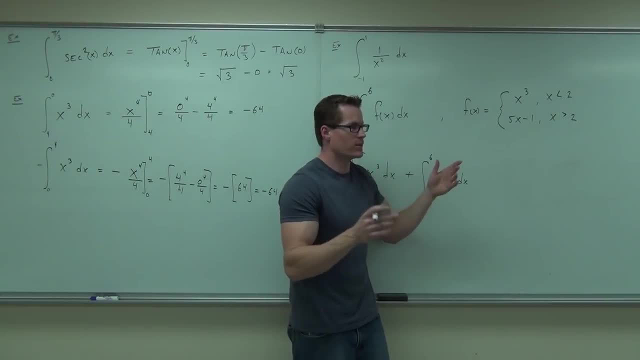 be continuous. I think I gave that to you. I don't know if I stated it word for word, the way the book does- but in order for that property to work- the ability to split up that integral- it's got to be continuous. 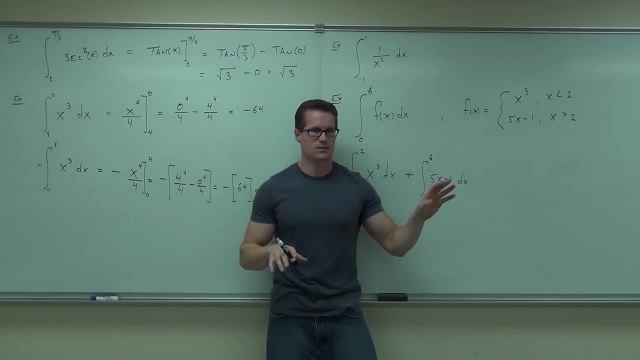 That's another reason why this one would fail. That's not continuous. Do you get that? You couldn't even split it up to begin with. It's got to be there, It's got to all be there and you've got to have the ability to break it up. 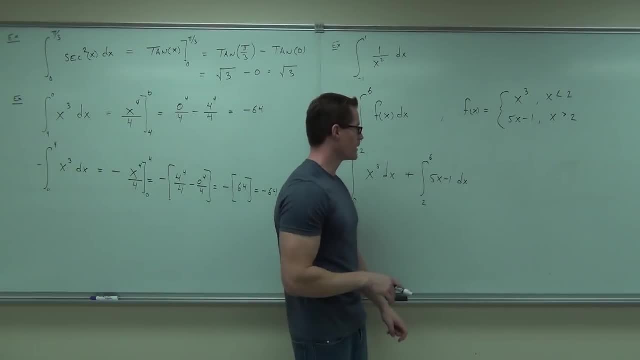 That's the only way this works. Otherwise, you are missing points, like you pointed out. That's a good point. Great question. I talked through that pretty quickly. Are there any questions about what I just said? Were you able to follow it? 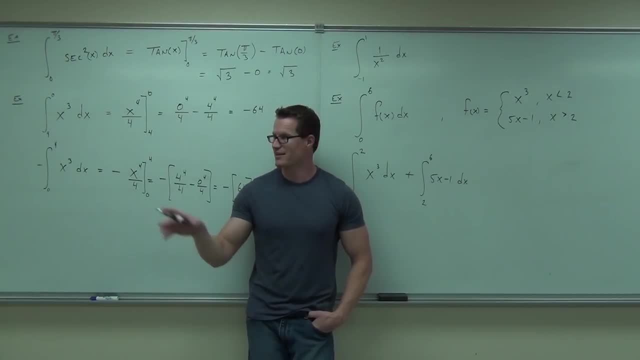 Yes, So same thing if it was, if the bottom function was 5x minus 2 or something and there was a jump, then you wouldn't be able to do it either. Or If they didn't actually match. Oh, that's a good question. 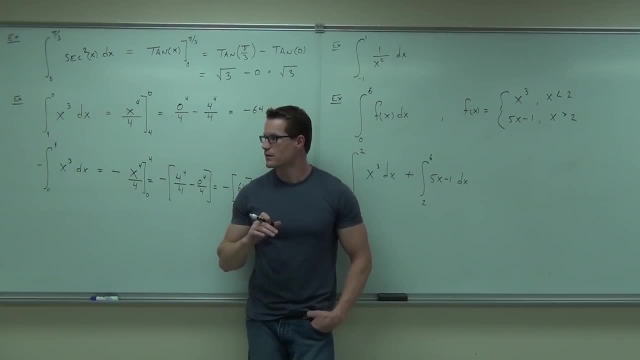 You mean if there's an actual gap, like if you plug in 2 and it doesn't Right, like they're not the same for both functions? Yeah, they're not in this case. Yeah, Yeah, Yeah, Yeah, Yeah. 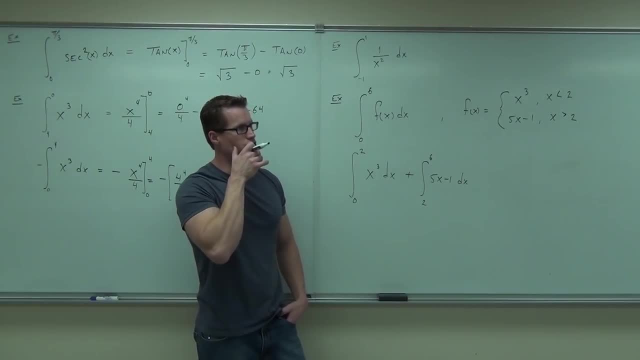 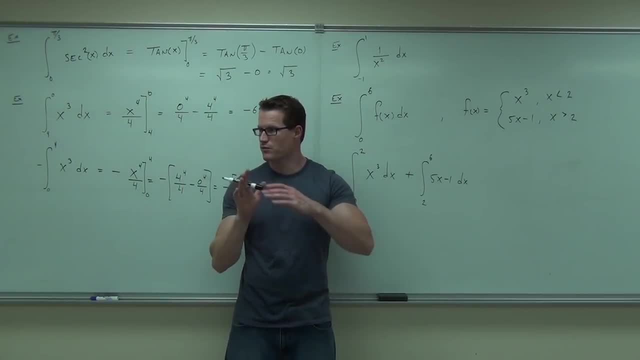 Oh, you're right, They're not. Yeah, they're not in that case. No, it doesn't matter. Just, it means that you're defined for every point from, In this case, from 0 to 6, that you have something for every one of those points. 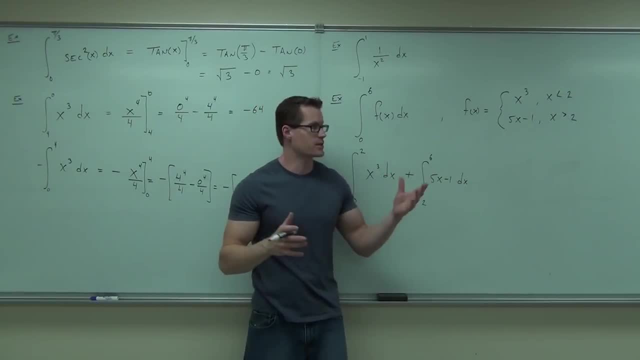 Okay, That's the ability to break that out. Now, in practicality, is that if you add those areas or you add What was it here? If you add those areas, it's going to be the same. You just can't do this if you don't have that. 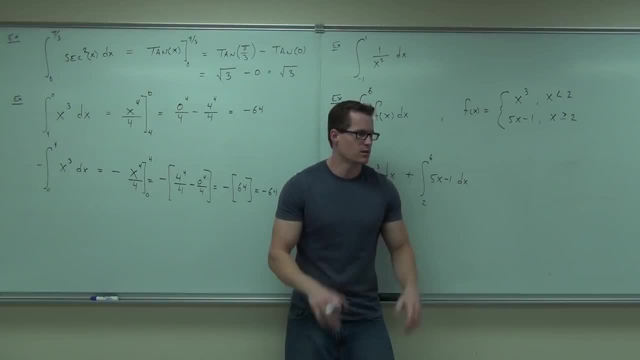 That's the point. Does that make sense? You just can't do it Legally. legally speaking, you can't do it. Yeah, Theoretically it would make no difference, though Theoretically it does make a difference. 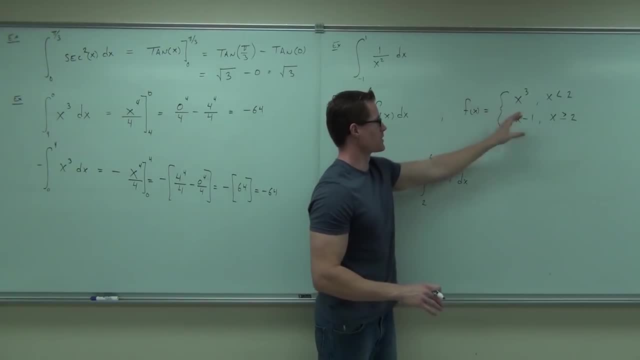 You cannot actually do it. Practically, this area plus this area will equal this area. Yes, Sorry, This area plus this area. This area plus this area. I should do it this way: This area plus this area, even like that. 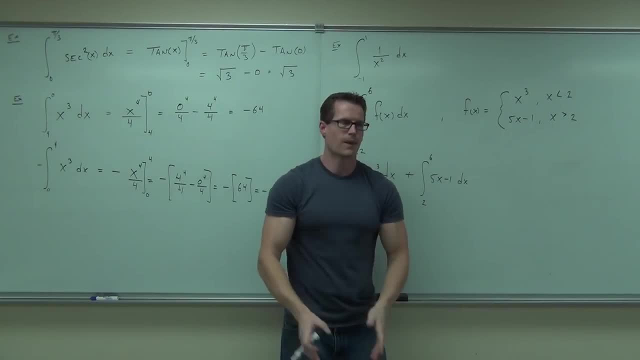 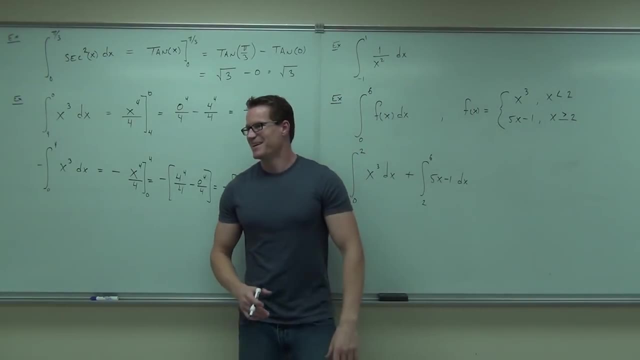 will equal that area, because the area under the point is 0. But you can't do this unless you have this. That's the point, Dang Good questions. You're making me work for my money today. That's why they pay me the big bucks. 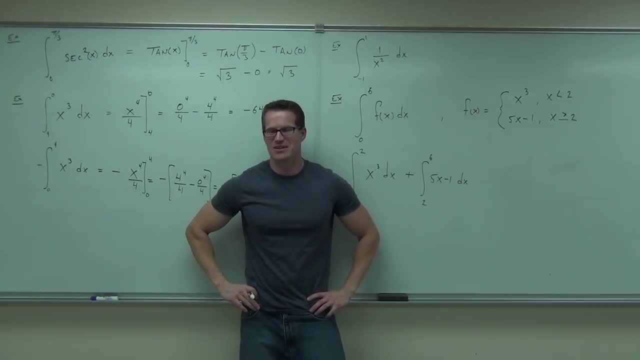 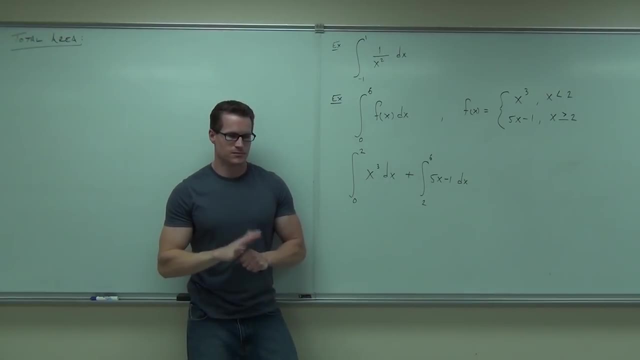 You know that right, I'm going to explain all this junk to you. I don't get paid big bucks. The Audi I drive is a 01.. Integrals aren't actually that hard. It's plugging the numbers and getting that right, huh. 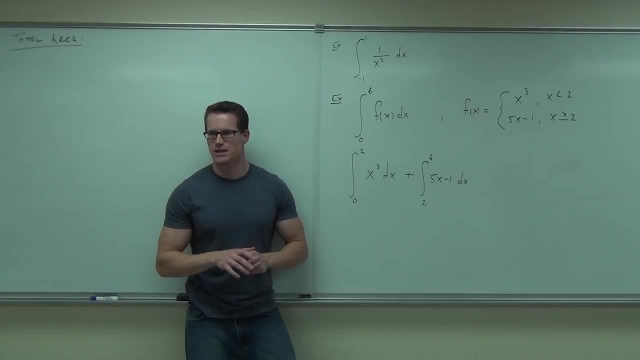 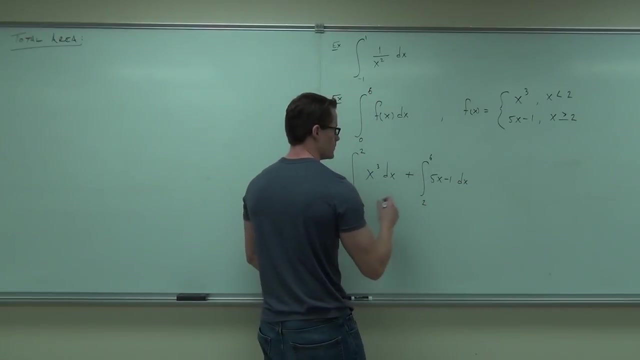 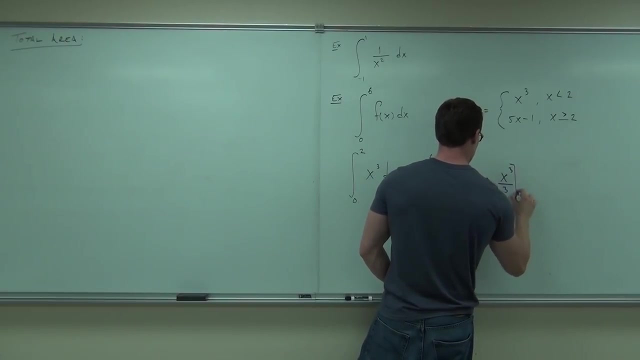 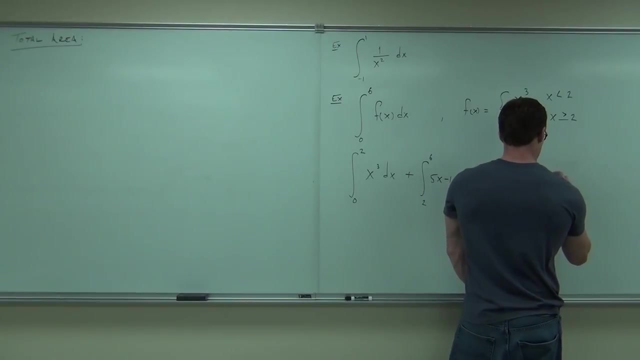 That's the biggest problem in math is the small stuff. My gosh, Don't forget any signs. Don't lose anything. Keep track of all your numbers. That's right. Why is that x2?? Oh, 4.. Sorry. 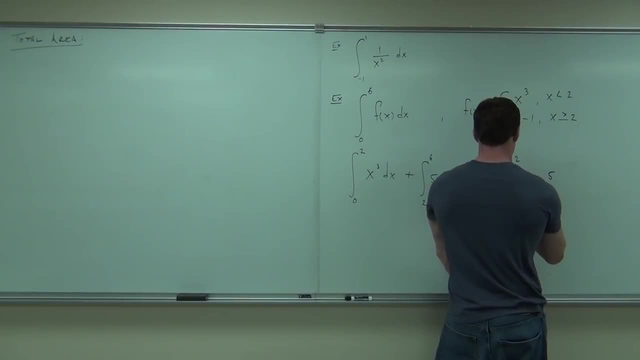 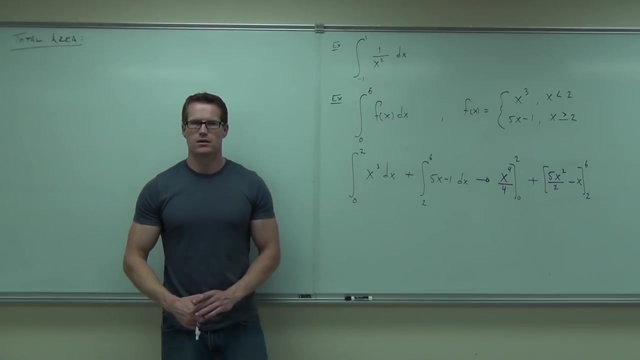 Yeah, New math, New math. Come on, It's a government policy. Did you all get your integrals correct? You got x to the fourth over 4 from 0 to 2.. You got 5x squared over 2 minus x. 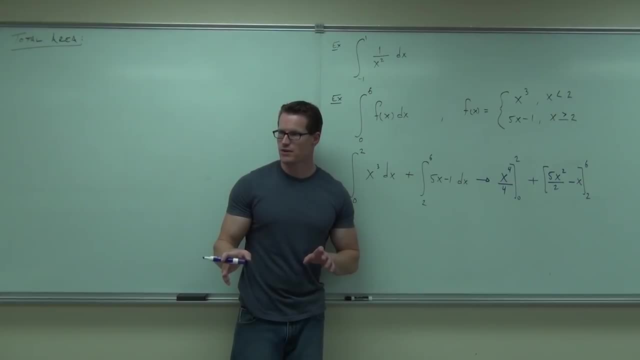 You didn't forget the minus 1, right From 2 to 6.. Did you get that far? Now we plug the numbers in. I'm probably. I don't know if I should count on you guys on that one. No, I don't understand what that is. no. 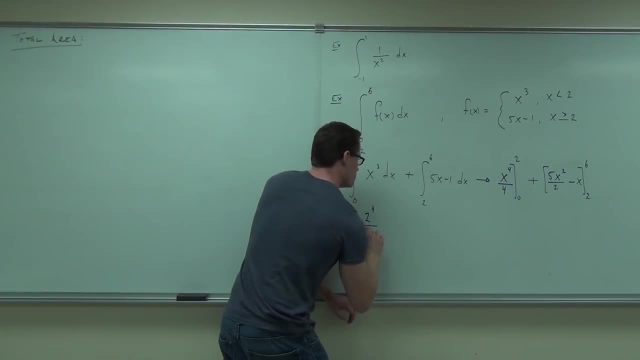 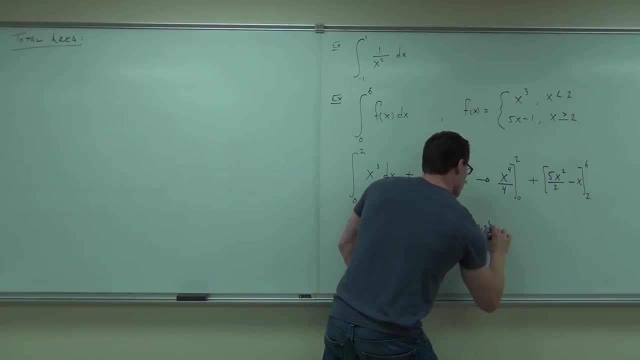 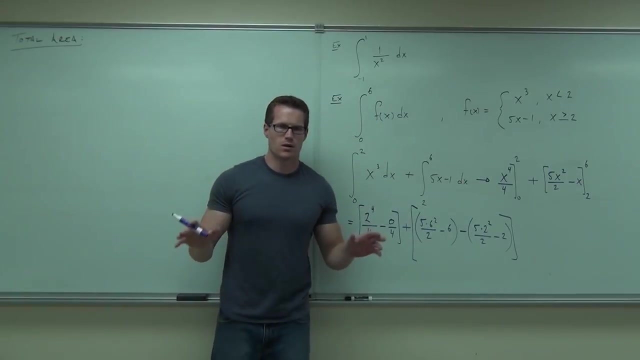 OK, So you can just give us some more trade and we'll get back, Right, OK, Oh, OK, You know you're going to need some brackets and parentheses on this thing, because you've got stuff going all over the place. 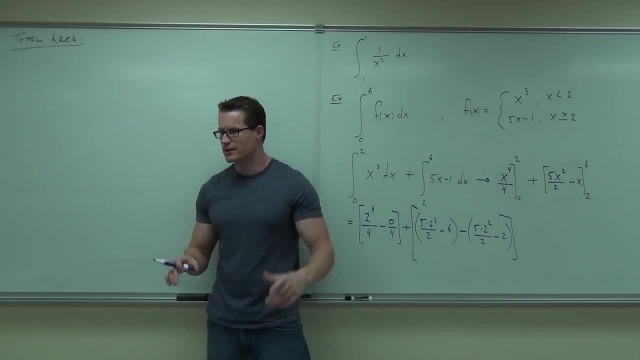 especially when you have those multiple terms being added or subtracted. This one's pretty easy. This one: you just plug in the 2 and you plug in the 0, and that's very straightforward. You get 2 to the fourth over 4, minus 0 over 4.. 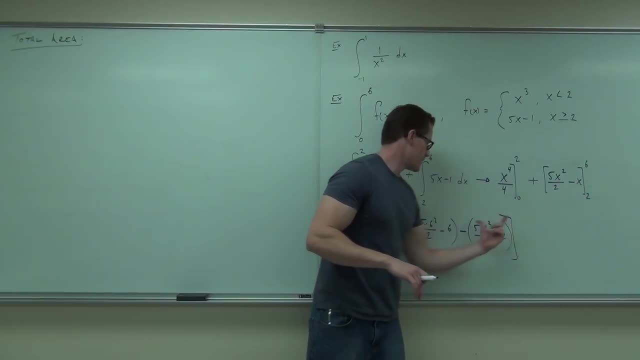 This next one. you've got some things going on. Notice how you have to plug in the 6. That's giving you the 5 times 6 squared over 2 minus 6. Then you plug in the 2, but you're subtracting. 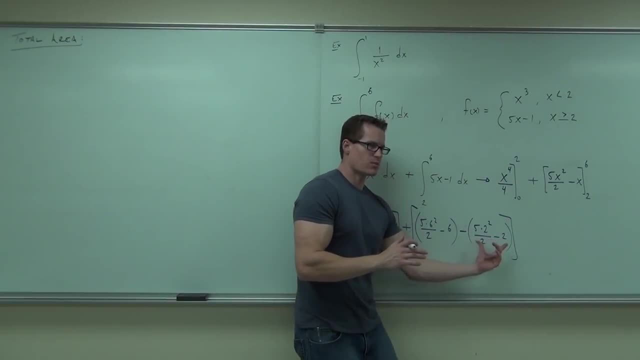 Remember it's f of b minus f of a. The whole thing. Do you see why the parentheses are important here? OK, If you wanted to distribute, you're distributing that sign with a chain. Typically order operations say you add all that up together. 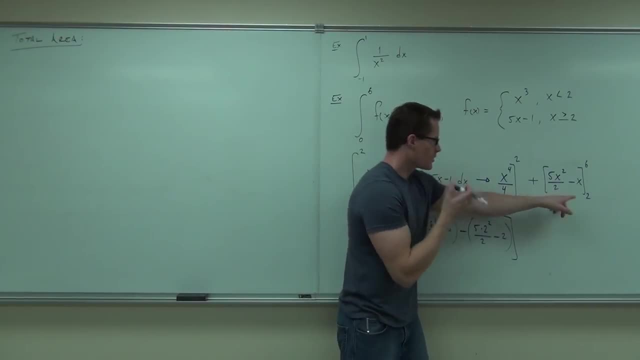 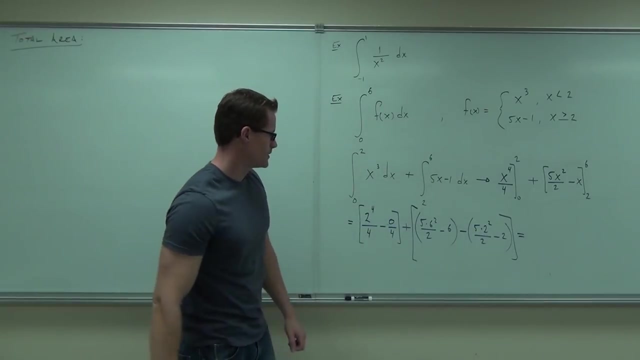 before you subtract anyway, but it's important that you know that. So we plug it in the 2.. We got all that down. You want to help me with the math? That should be what, 4?? Yeah, Yeah. 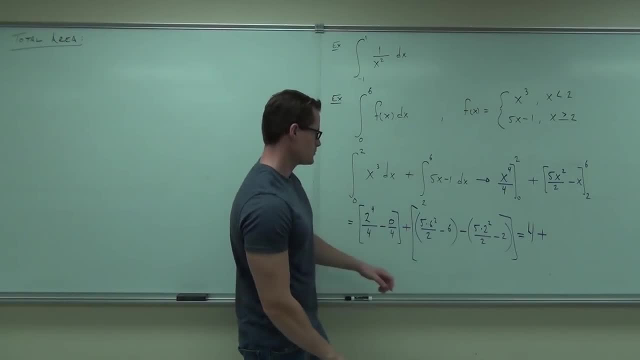 4 plus, So that's 4.. 90.. 84., 36.. That's 90.. 90.. 90 minus 6. 84. 84.. OK, So that's 84.. 8? Minus 8, right. 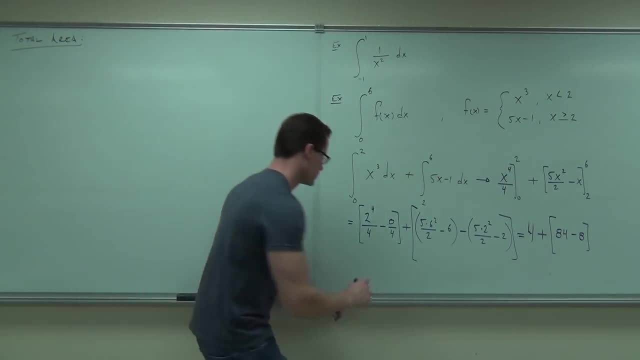 Looking like 80 to me. Did you get 80?? Yeah, Uh-huh Cool. How many people were able to find the 80?? Did you feel OK with it If you weren't able to actually do it on your own? 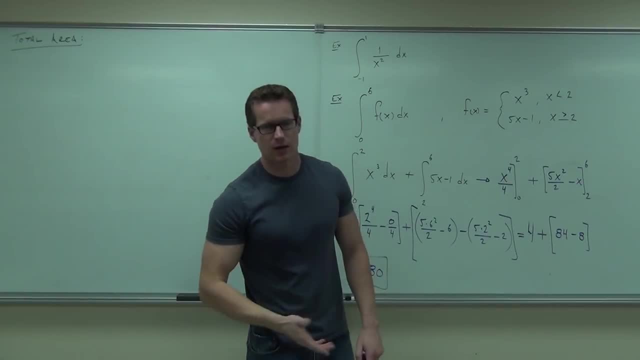 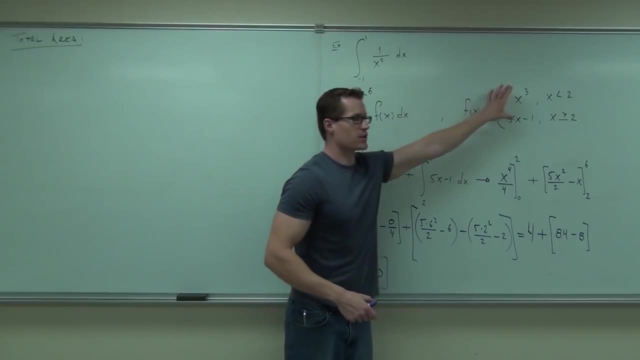 were you OK with it. Now, what's it represent? What did we just find? The area of, what A piece of it, Yeah, Of this, when it's defined this way: between 0 and 6, you found the area under that curve. 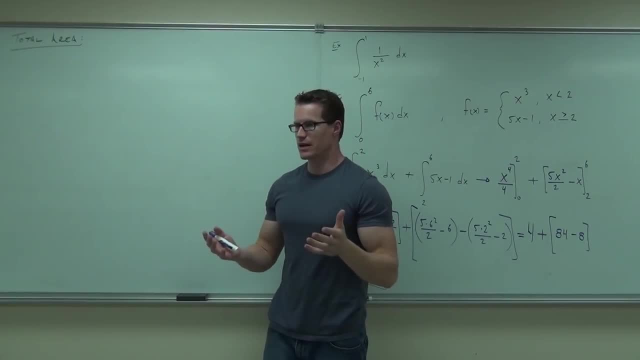 Or actually the area, the net signed area. If this thing went below the x-axis I'd can't see the net, But it does. But if it did go below the x-axis then we would actually have the area that takes the difference between the area above. 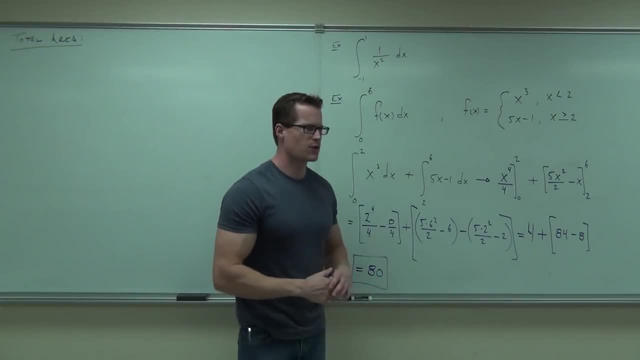 and the area below, And that would be net signed area. Do you feel OK with this example? Do you have any other questions? It's: whenever we have multiple terms in one, we just take the first one, put in for all the x's solved. 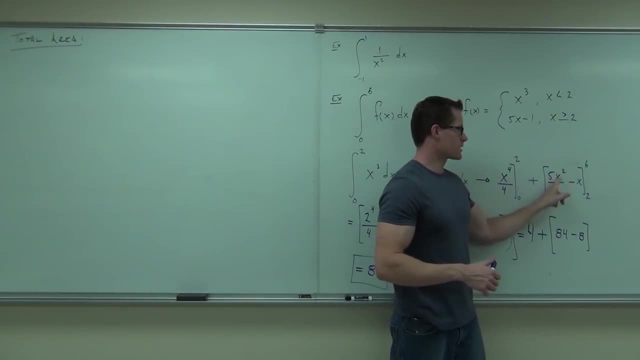 and then take the bottom. Absolutely, What this says to do is you plug in the 6 the whole way through. you figure it out. That's the area from 0 to 6 of this function. Then you subtract From 0 to 2.. 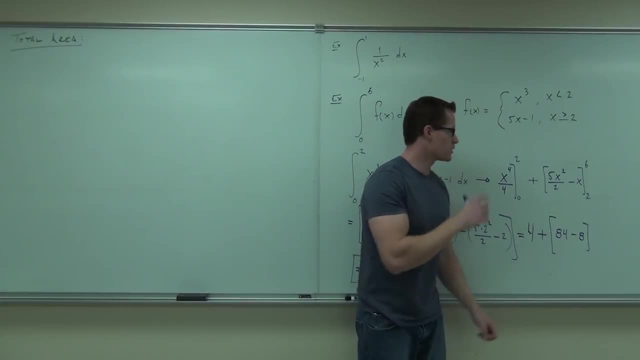 And that's what that's going to give you. And so, no matter how many terms we would have, Plug them all in, Then subtract And then plug them all in, And that's what you do. You've got to plug them into everything. 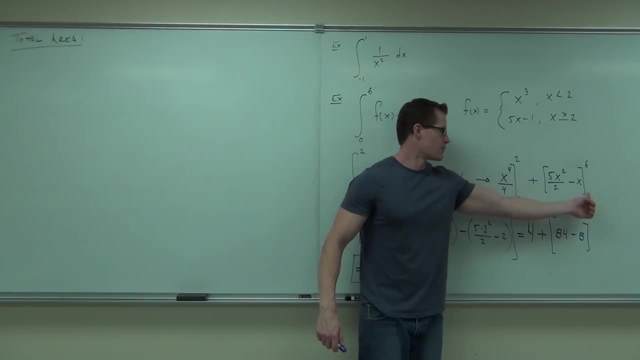 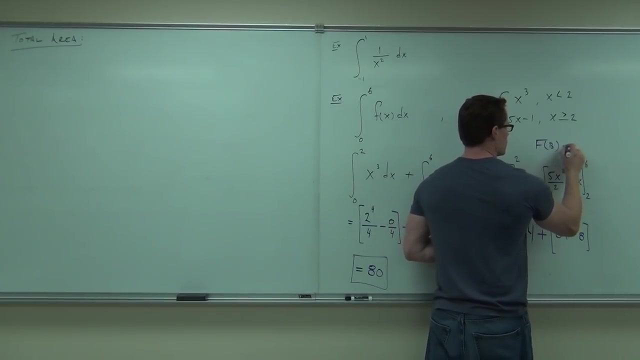 And for this instance, your x becomes 6, every cx. For this instance, your x becomes 2, wherever you see x, And then you subtract, And that's what this meant: f of b minus f of a. That's what that meant. 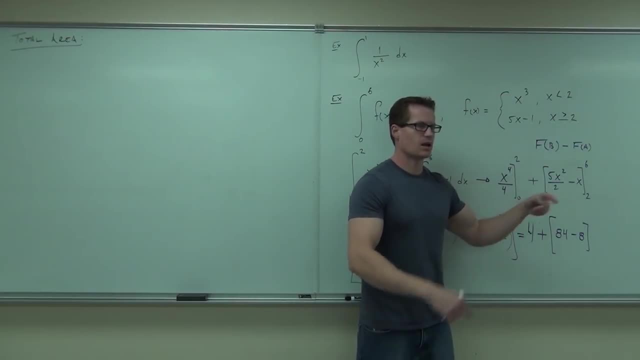 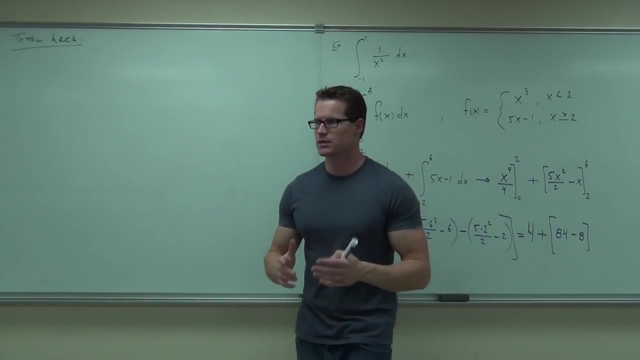 You take your b, You plug it in, You take your a, You plug it in, And then you subtract And that's what you get. Now, what we've been talking about this entire time is something called net signed area. I gave you net signed area before. 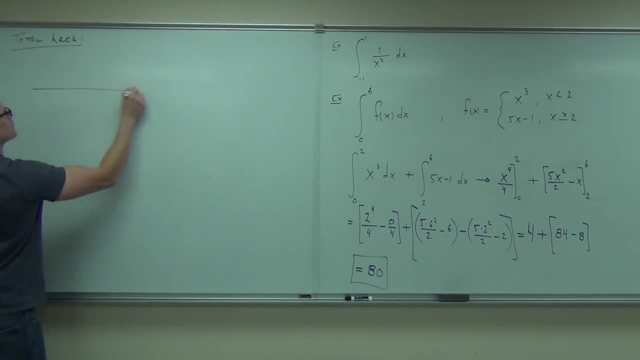 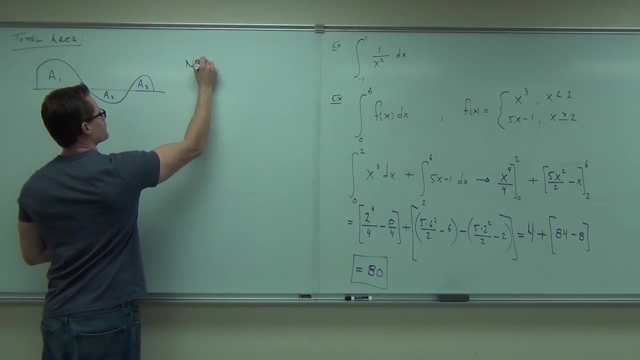 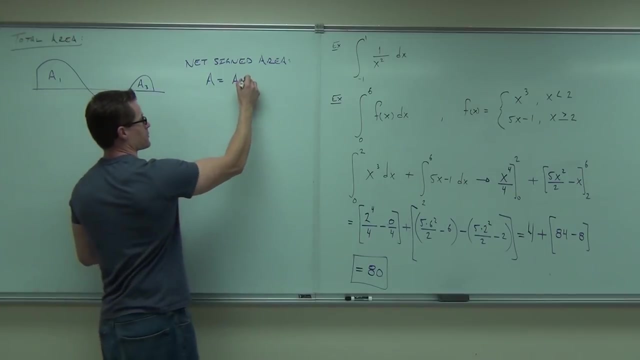 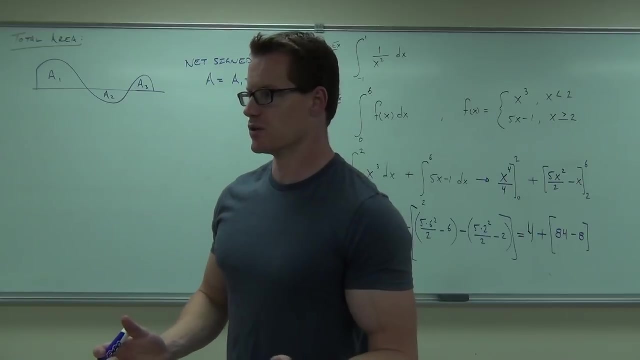 What net signed area was was this: You took the area 1.. You took the area 3 because it was above the x-axis And you subtracted area 2 because it was below. That is what your definite integral will do automatically. 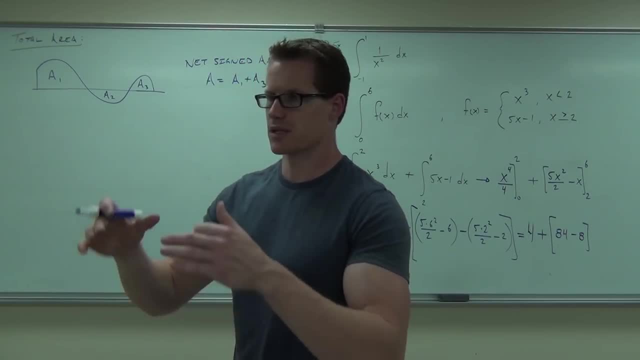 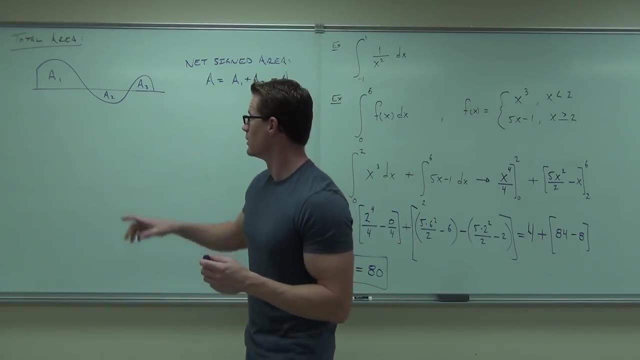 Without asking you, it will do that. Why does it do that? Because it will count as negative area for a definite integral. That's actually one of the things that we saw with our switching of signs. That's another reason why that comes out negative is because when you go from whatever, this point 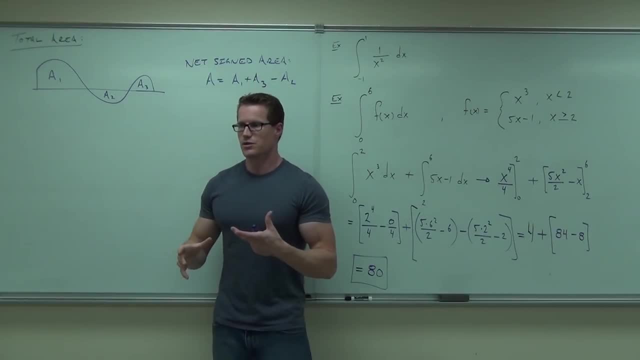 to. whatever this point is that is below, it's going to be subtracting those areas and thereby causing them to be negative. So this counts against your total area. Now, in order to count total area, what you do is this: You say: I want to count up the area that's between the two curves. 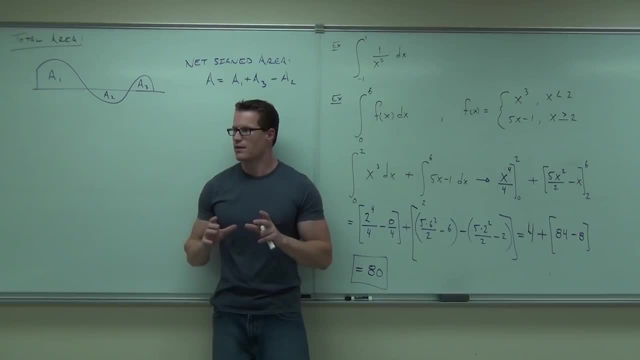 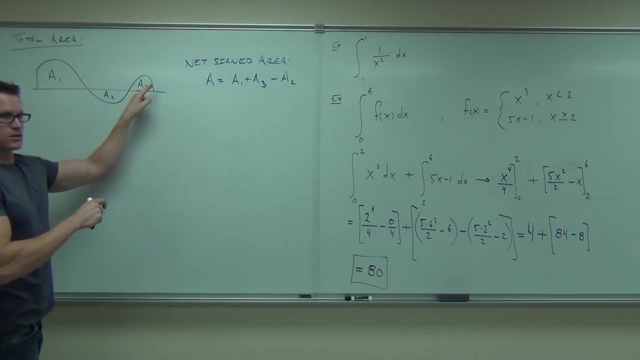 I don't care which one's on top or which one's on bottom. I want to find out the actual area between them. So find the area that's here and here and here That would be total area. This is net signed area. 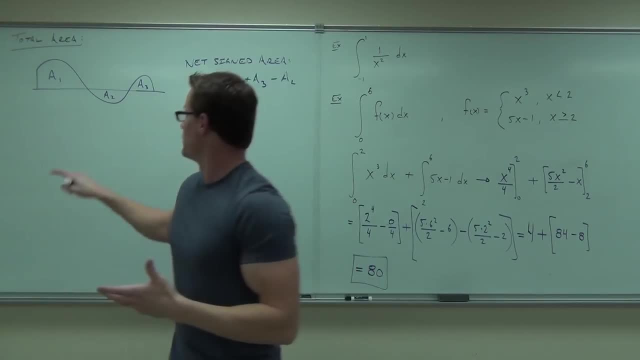 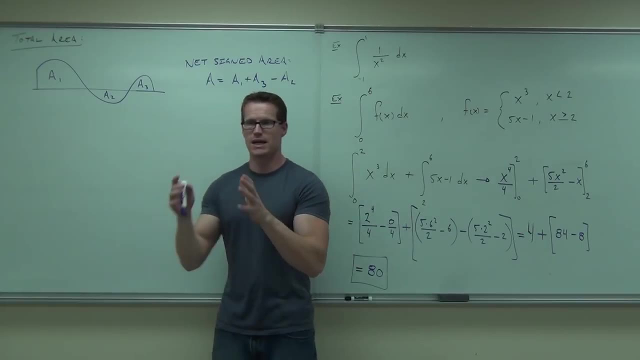 So one question I have for you is: how in the world can we get this area to become positive? How would you do that? Absolute value, Say it louder. Absolute value. Absolute value will absolutely take any negative thing and make it positive whenever you see it. 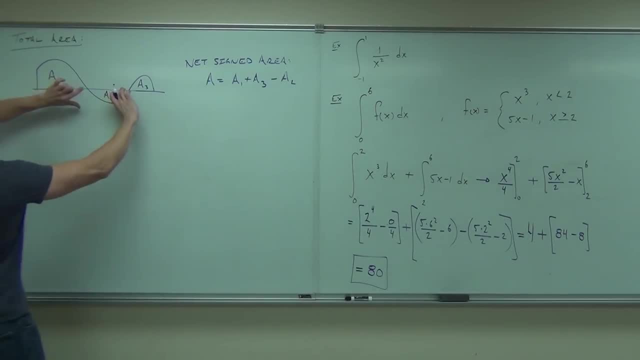 So what we're going to try to do is this: We're going to try to take this one, We're going to take this one and flip it over and say, all right, well, total area then should become area one, area three. 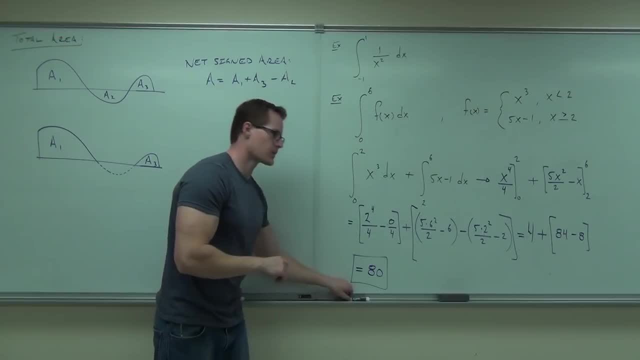 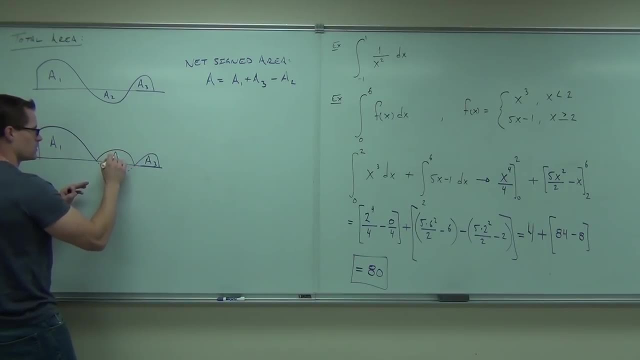 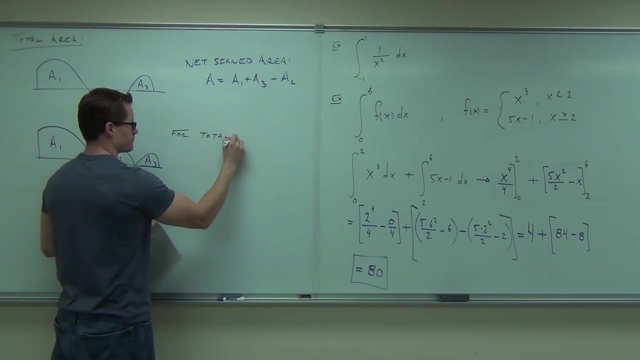 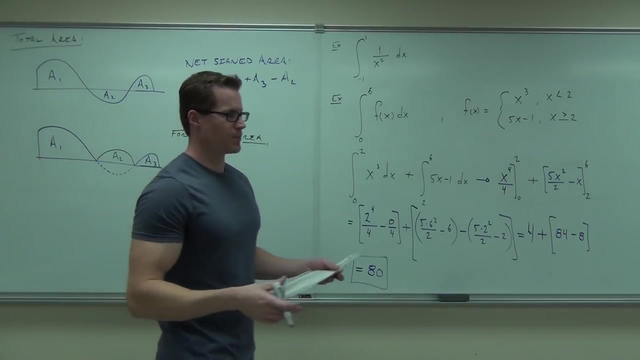 Not that We don't want that. That's going to count as negative area. What we want to do is find a way to flip it over here And make it count for us. That would be total area. For total area, we need to change the sign of area two. 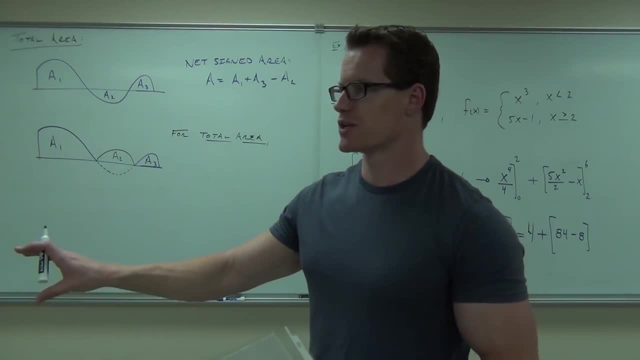 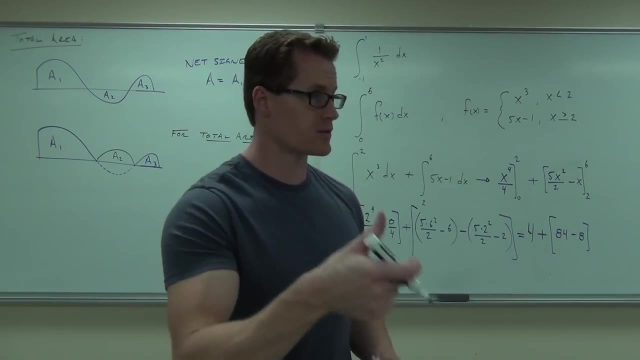 In other words, if you kind of go on further than this, you say: well, I want to change the sign of any area that's below the x-axis. If I can do that, then that negative area actually counts as positive area. 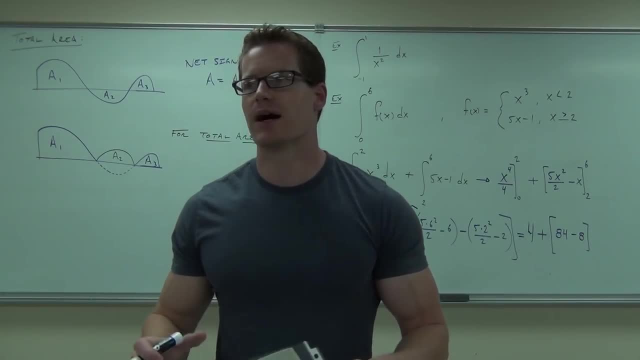 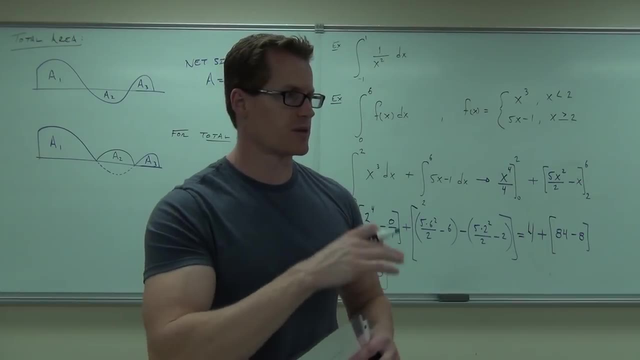 And we add it up together And what we end up doing is we end up finding the area between two curves. One of the curves is the function, The other curve is simply the x-axis. Now, in section 5.1, we go further. 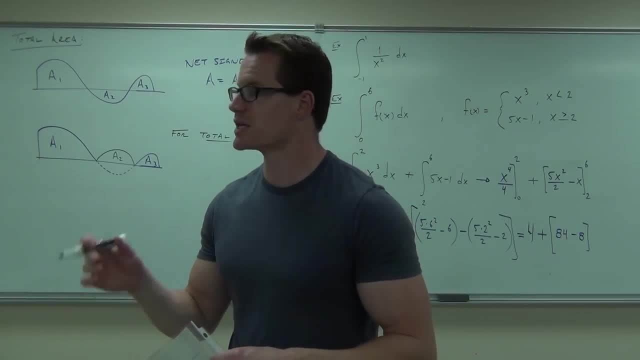 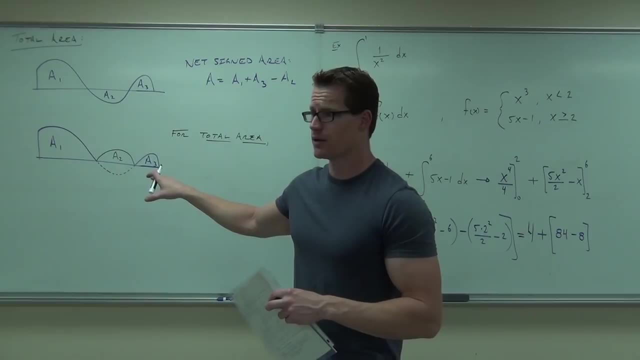 And we actually do legit two curves, not just the x-axis, But keep in mind that this is exactly what we are doing is finding the area between two curves. So I'm going to draw on this later, You understand. So this is one curve. 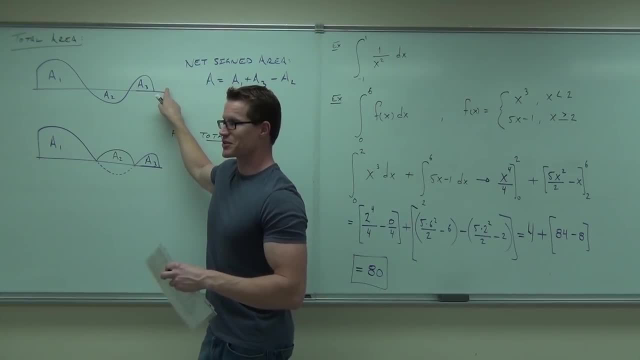 This is the other curve. It's a very simple curve, It's just x equals 0. But what we're doing is finding the area that's bounded between two curves. That's what we're doing, literally, In order to do that. that's positive. that's positive, that's negative. 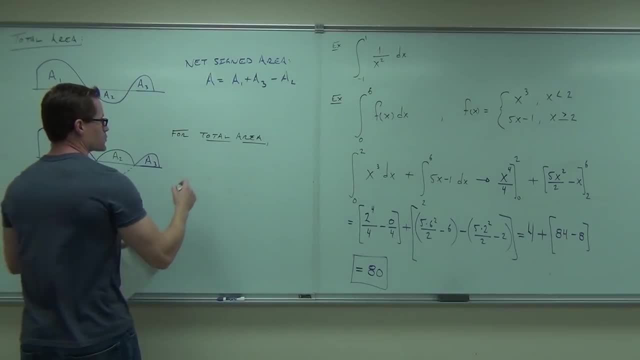 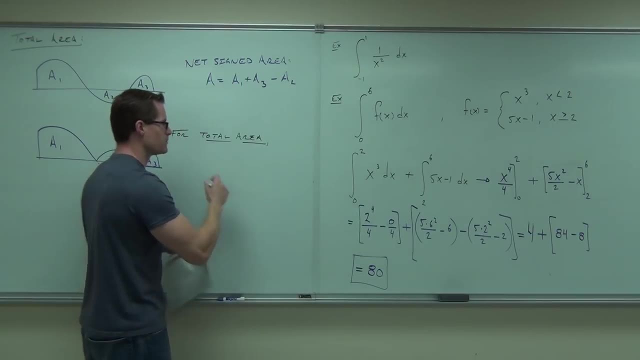 We have to change the sign of that for the x-axis. That's the idea. So for total area, we need to change the sign of area two, Or in other words the area of any piece of the region that is negative In this context, that's, the area that's below the x-axis. 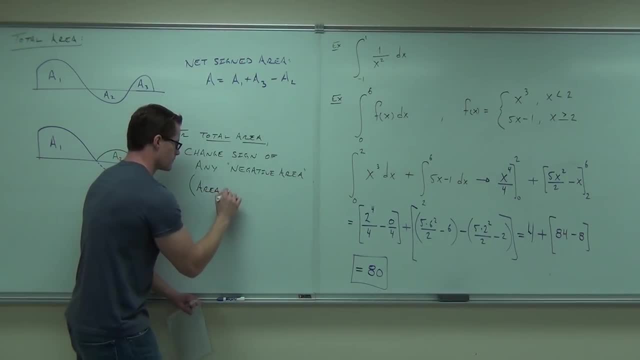 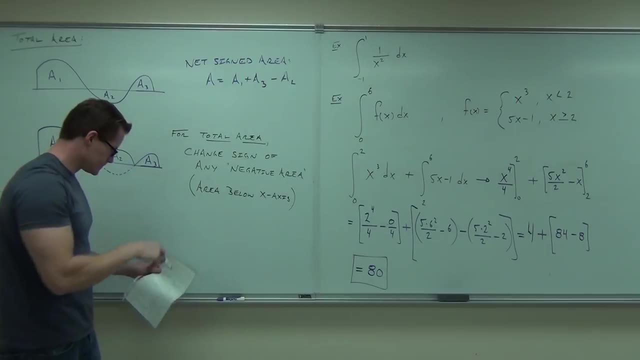 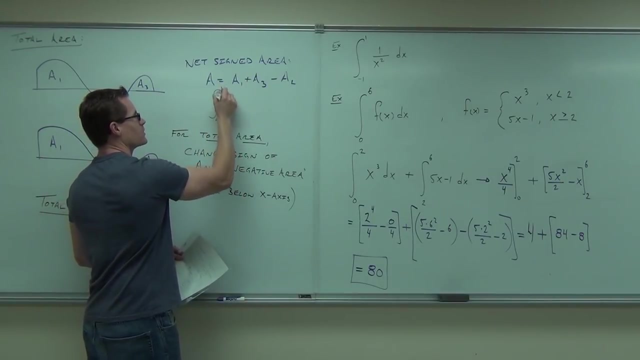 No, I want to show you how to do it right now. OK, now check it out. Here is net signed area. Net signed area says you start at a, you go to b, you just take the integral of whatever function you have. 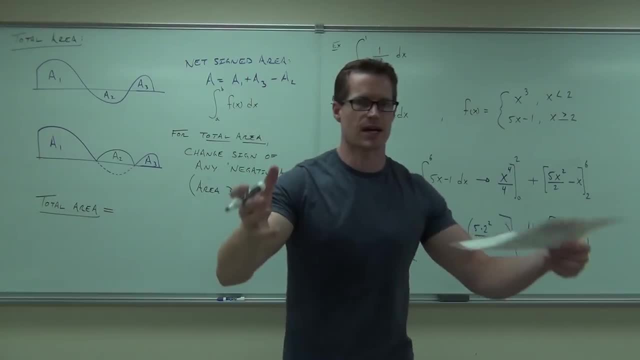 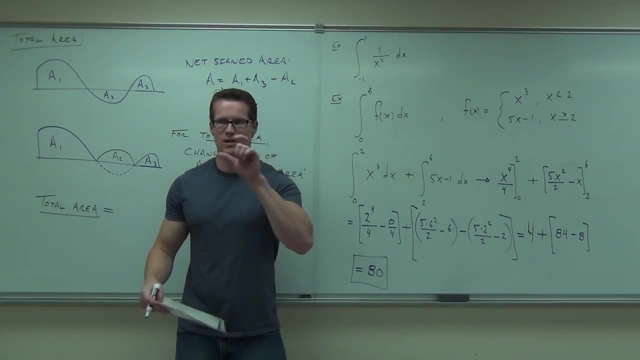 and whatever happens happens. Positive area means most of it's above the x-axis. Negative area means most of it's below the x-axis. Even if we cross over, it just basically says: your net change what is mostly happening, whether you have more positive than negative. 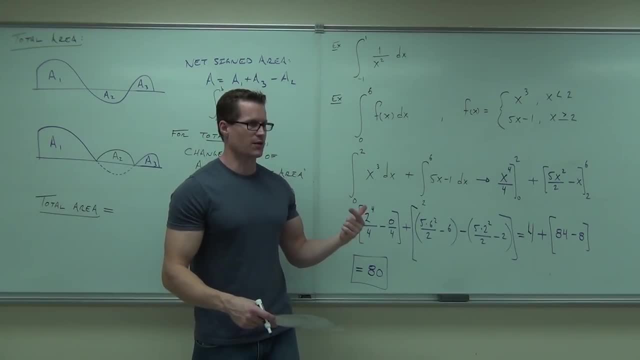 or more negative than positive, no matter what it actually is on your graph. Does that make sense to you? Now, total area says no, no, no, no, no. We're gonna take all the negatives and we're gonna make them positives. 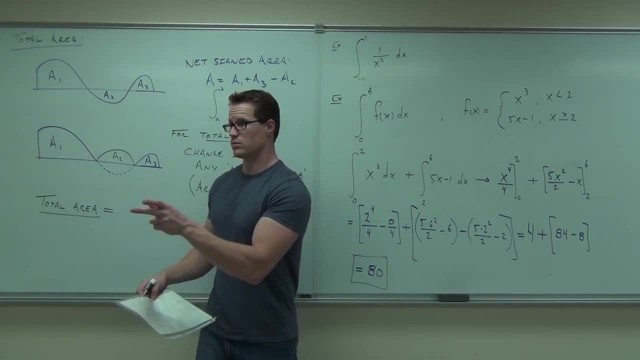 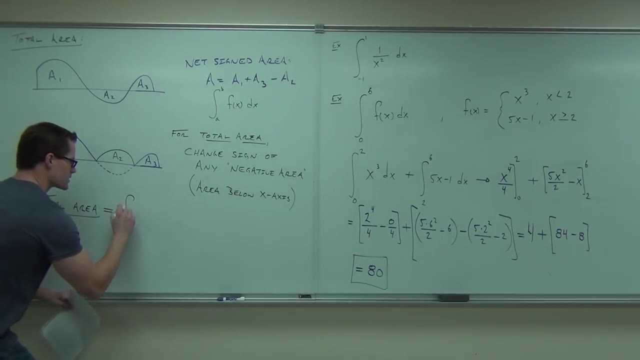 What do you do with the positives? Leave them alone. The thing that leaves positives alone and changes negatives to positives is, of course, absolute value, like you said. So total area says: all right, we're still going from a to b. 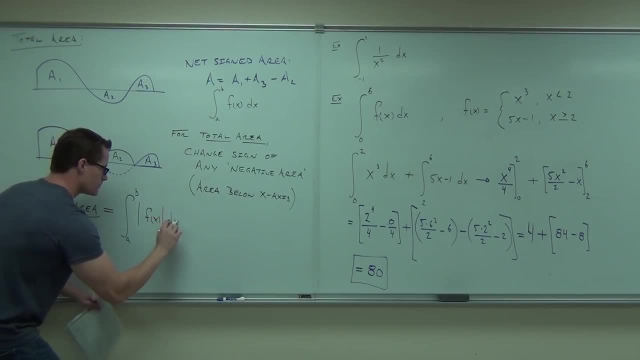 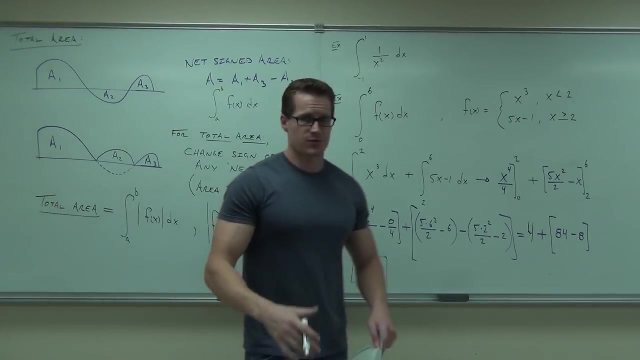 but now we have the absolute value of f of x. Just remember one thing: The absolute value of f of x, so the absolute value of any function, is actually piecewise. So it's gonna look kinda like this is why we did this first. 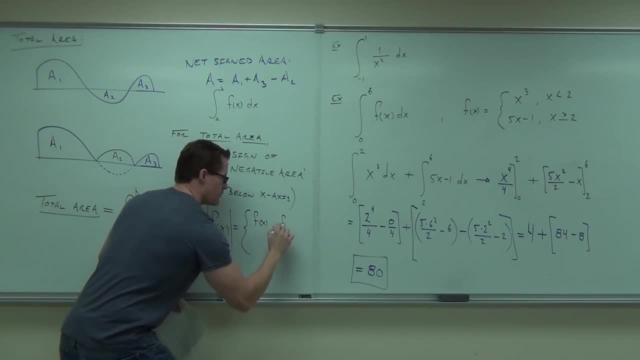 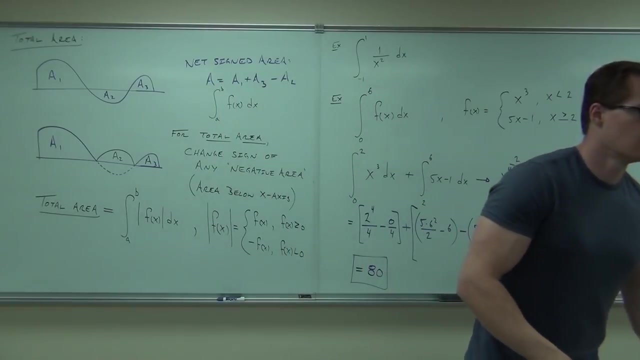 It says: you keep f of x if f of x is positive, You make it negative f of x if f of x is negative. That's the way you do absolute value. It says: shoot man, if your function's positive, why are you gonna change it? 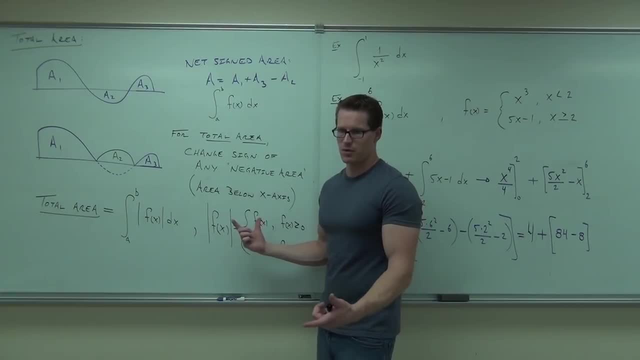 That's gonna be a positive area. In fact, we know it's gonna be a positive area from one of the properties that I taught you before: Whenever your function is completely above the x-axis- hopefully you're listening to this- whenever your function's completely above the x-axis. 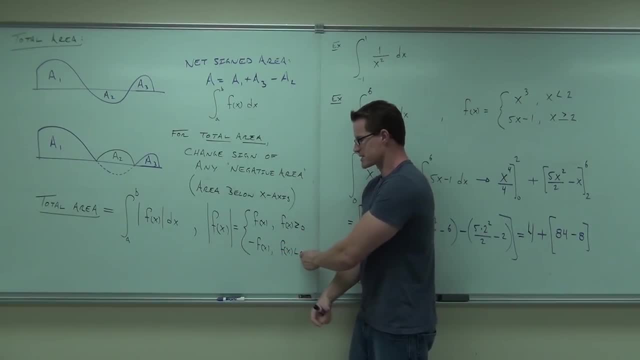 your area would be positive. Remember that Whenever your function's completely below the x-axis, your area would be negative. If we make an area, a negative area, negative, that's changing the sign of your negative area. it would become positive. 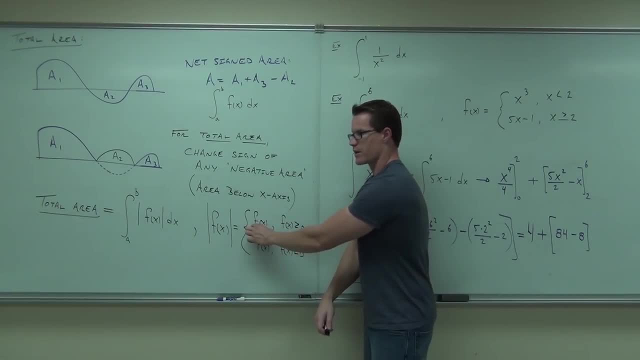 So here's what this says: This area will be positive. This area, this area, will be negative. So we're going to change the sign, thereby making it positive. Are you clear on this? Did that blow your mind like a grenade? 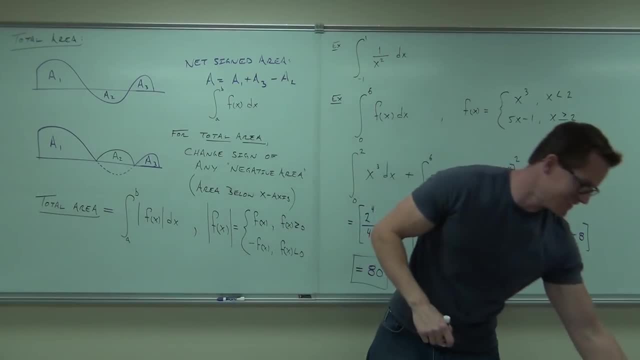 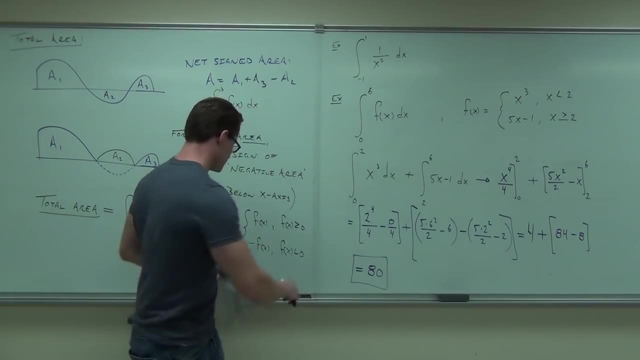 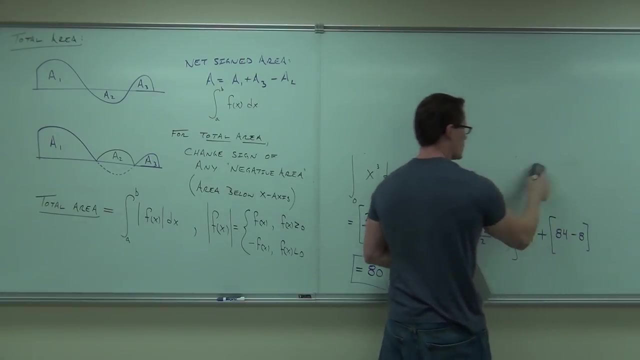 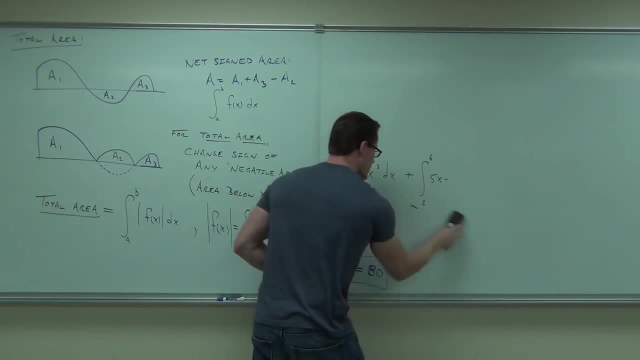 There's just one more step to be able to figure out where you separate it. You see, we just did this piecewise function. only in this piecewise function I gave you the separating mark right. I said you go from zero, two and two to six. 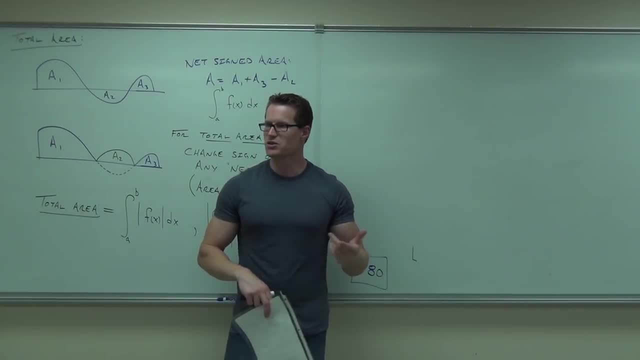 All you're gonna have to do is figure out where that mark is for yourself. What that's called is a sign analysis test. Bam Told you this was exciting, Exciting stuff here, ride. How can you not get excited before a sign analysis test? 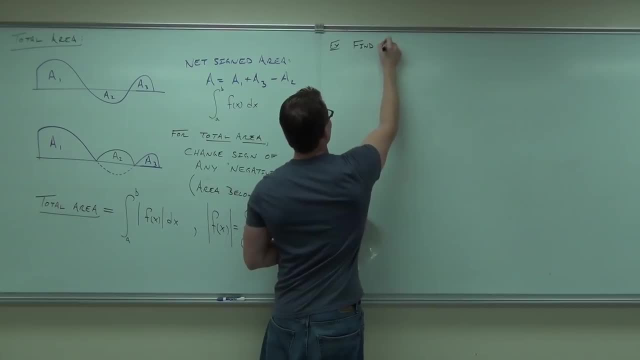 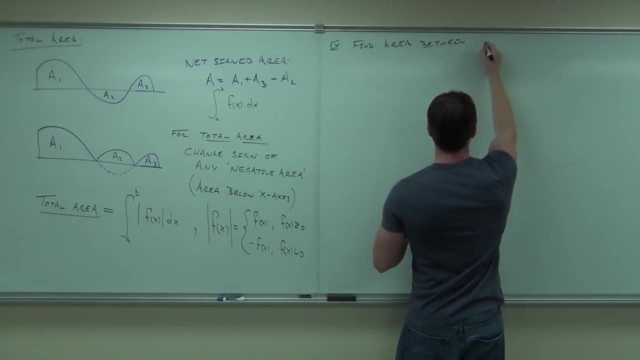 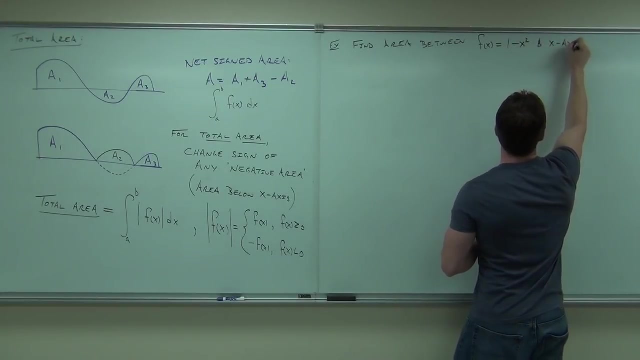 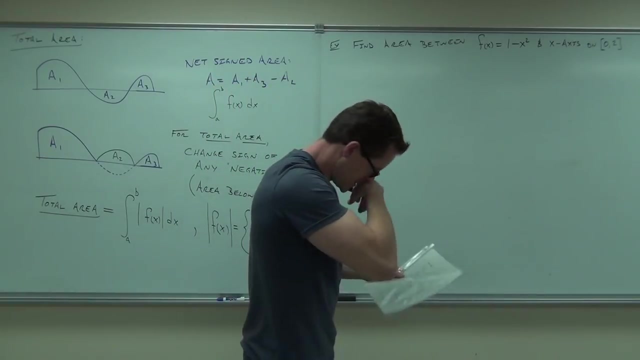 Find the area between f of x equals 1 minus x squared and the x-axis on 0, too. Well, what we mean is total area. Let me insert that right here. Find total area, Total area between that, Because net signed area would be very easy. 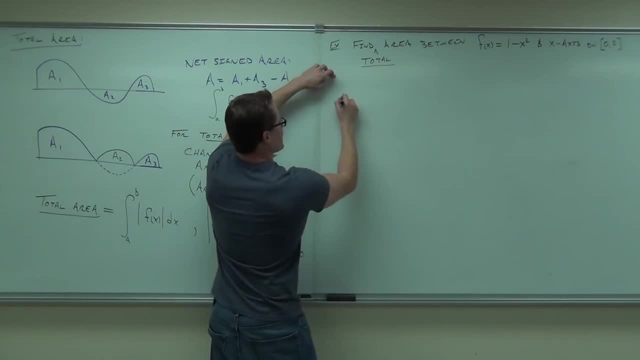 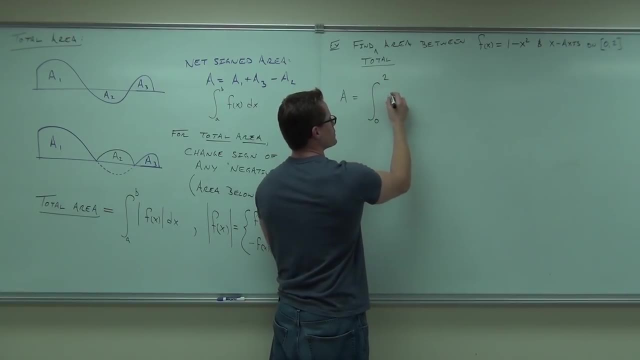 Net signed area. you would just take the integral. Look it Here would be net signed area. It would be: from where would your integral start, ladies and gentlemen? Where? Where would it end? Your function is 1 minus x squared. 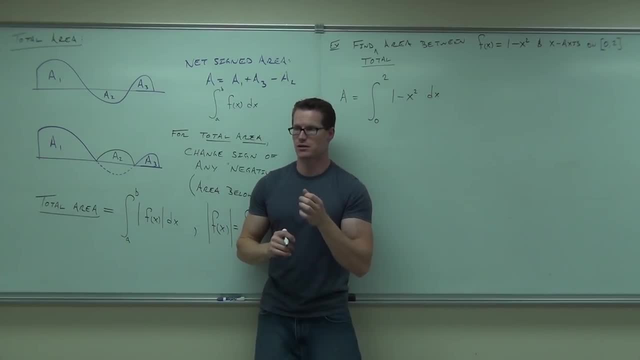 Yeah, This right here is net signed area. Do you understand? It would take the area above the x-axis, subtract the area below the x-axis, because it would be negative and that would be your net gain, your net change in area. 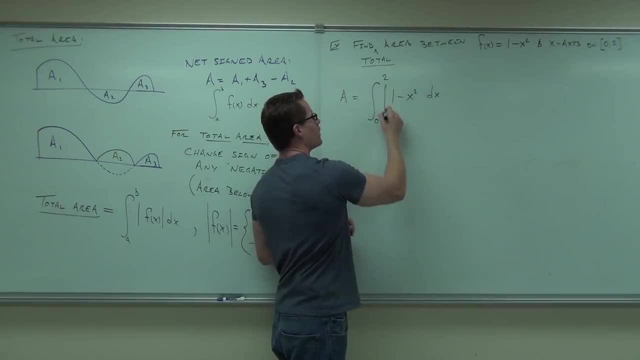 That's what that would be. This says: ah, no, total area. The total area will do this. It will take the negative area, It will flip it above the x-axis, or at least it will change the sign of it. 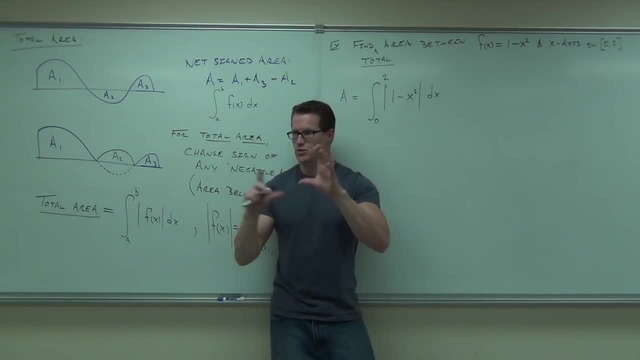 and that would count as positive area. It would say: I want to find the area between them. Take all of it and add it up. Take all of it and add it all together, no matter what the sign is. add it together because the absolute value will change it to a positive. 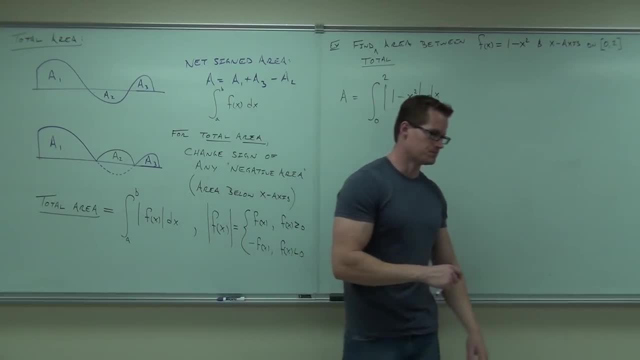 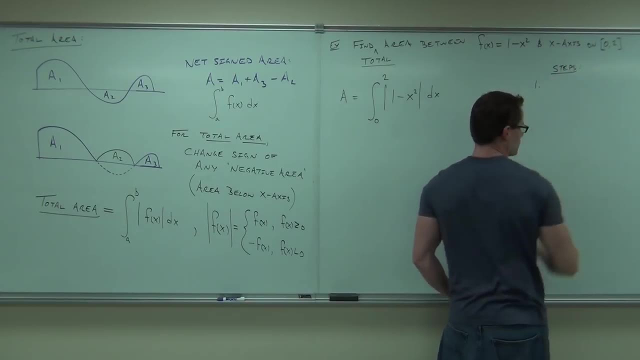 Are you following that? Okay, So how do we actually do it? Well, here's your steps. Step 1. You've got to set your function equal to 0.. Do you know why you've got to set your function equal to 0?? Why not? 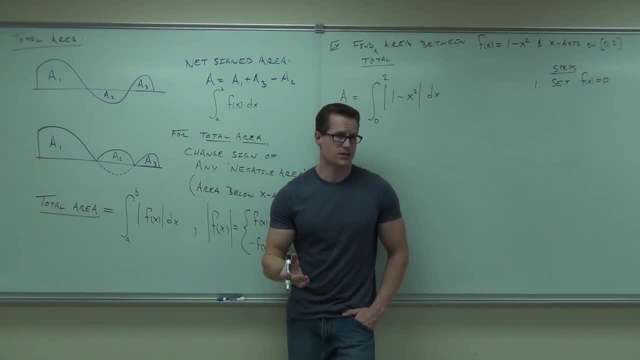 x-axis, x-axis, x-axis. That makes sense to me. Does it make sense to you? If you know where it crosses x-axis, then you can perform a sign analysis test, plug in some numbers easily and say: oh, it's above, it's below. 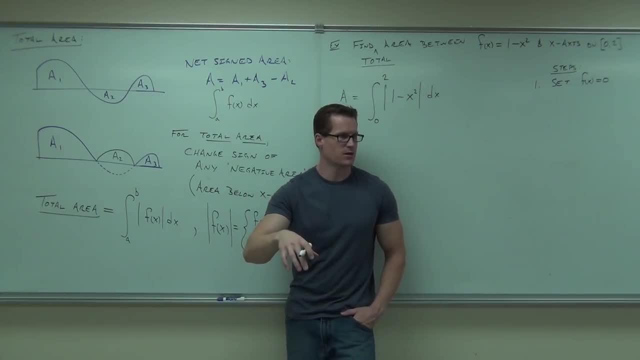 therefore, I know when the area's gonna be positive, when it's gonna be negative. You get me Okay, So set the function equal to zero and solve So for us. I'll do that in purple, so you see the work over here. 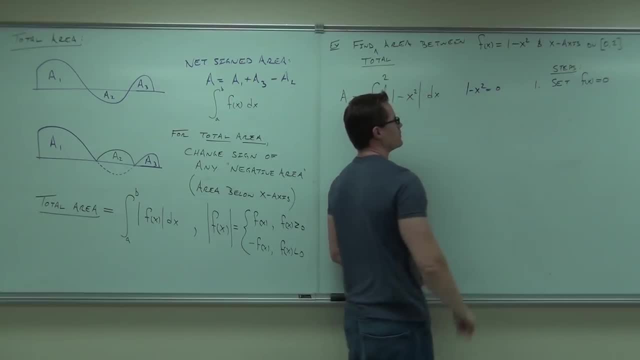 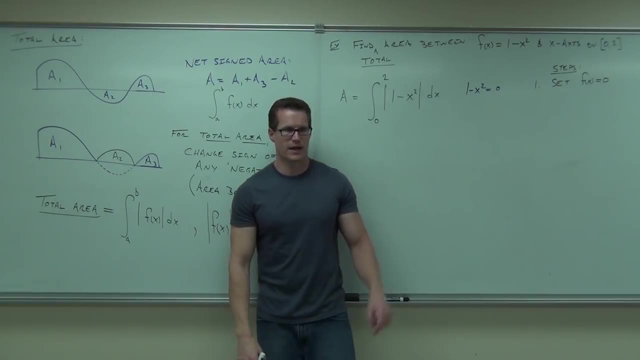 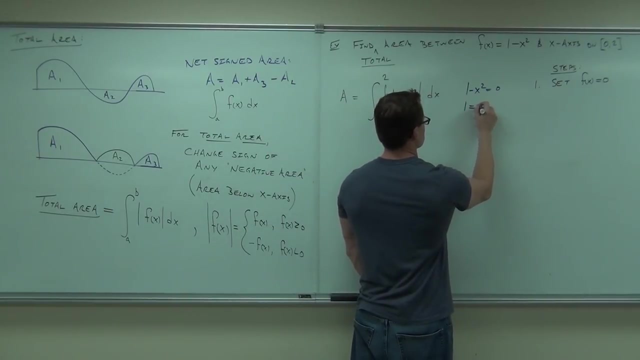 We're just gonna get one minus x squared equals zero. Well, there's only like two more steps. What are you gonna do with this? Probably, add x, squared, yeah, And then you're gonna Square root, Yeah, sure, square root plus or minus. 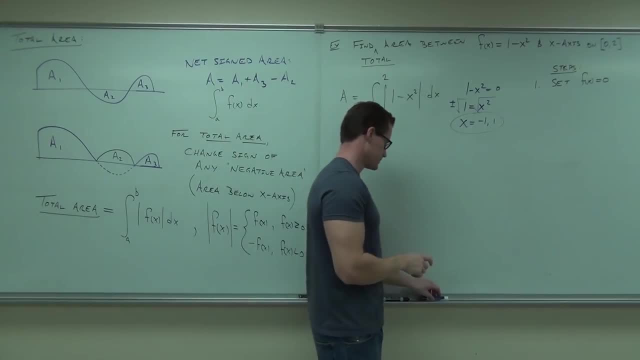 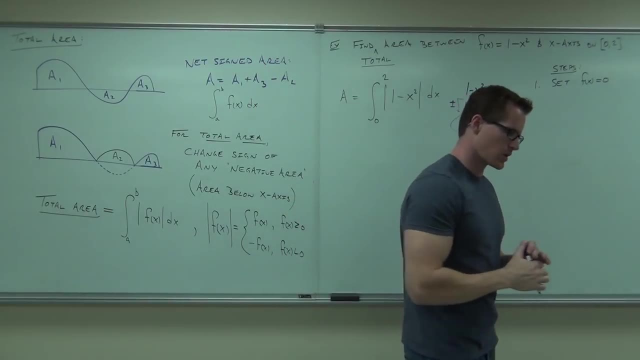 x equals negative one and one. Raise your hand if you feel okay with this. so far, Okay, now the next step. You gotta set this up correctly. What you're gonna do is you're gonna do a sign analysis test, Sign analysis. 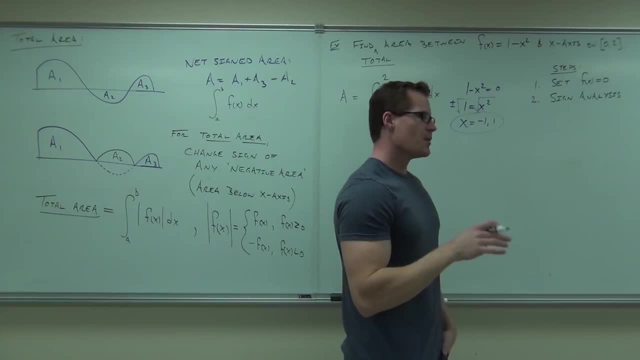 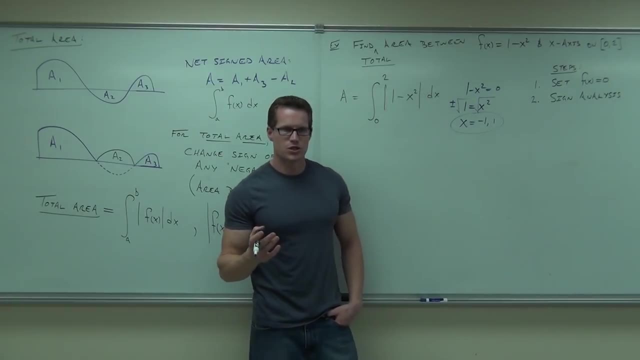 Sign analysis. But you only need a few of these points. What points do you need? Well, let's see. Do you need the zero? Yeah. Do you need the two, Of course. Do you need the one? Yes. Do you need the negative one? 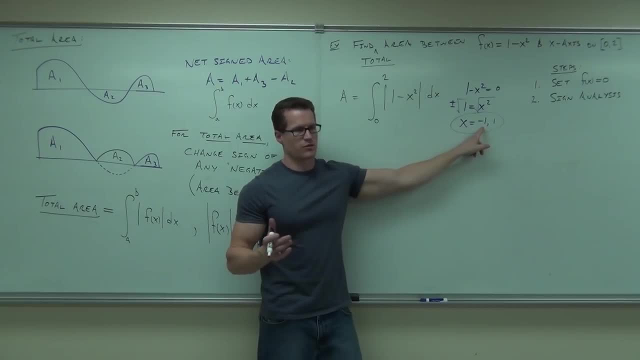 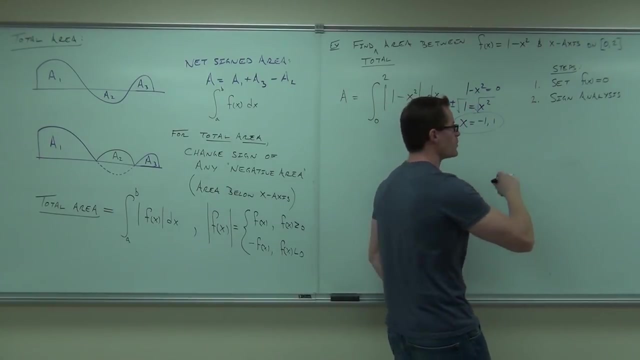 No, No, you don't need that one. Why not? It's not So really. you're going to make a side analysis, with your endpoints, of your interval, your bounds of integration and whatever points fall between them. That's it. So make it with your endpoints and your x-intercept that fall within those endpoints. 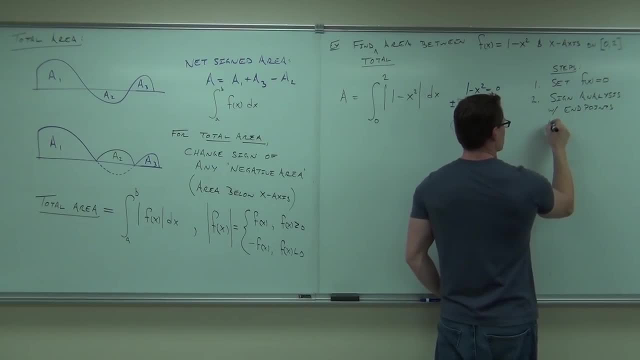 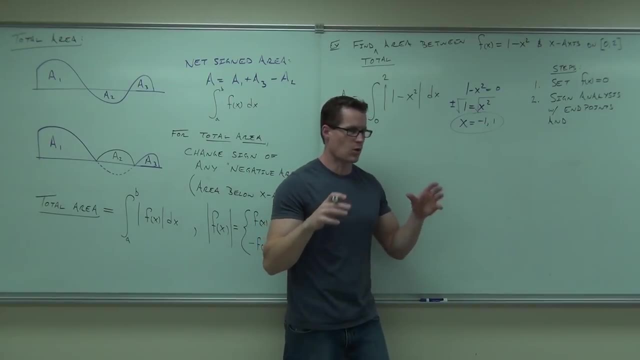 Now, if you had no points of intersection within your bound, you'd just use your two endpoints. Then you know what. You wouldn't even need that, Because it's either all going to be positive or all going to be negative. So you just test one and go with it. 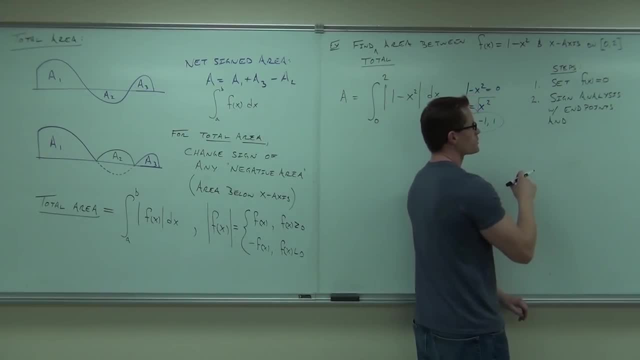 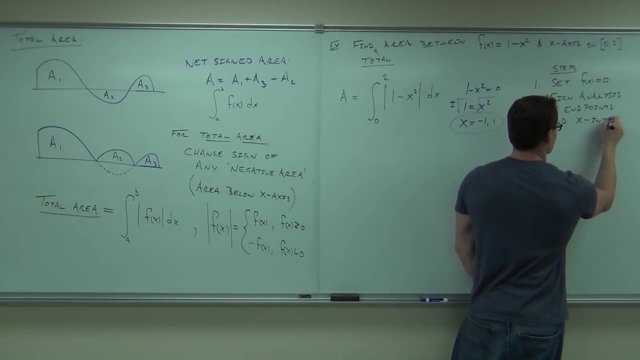 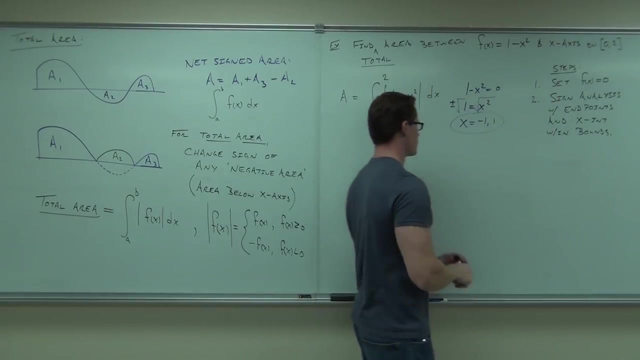 Yeah, So side analysis with endpoints and any x-intercepts that happen to be within your bounds of integration. Well, let's go ahead and do that now. So we're going to make a side analysis test. Here's how side analysis works. 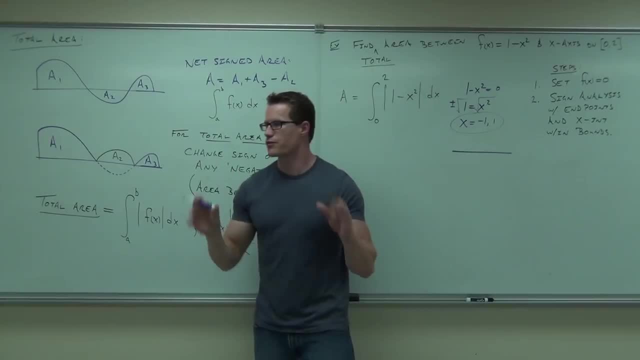 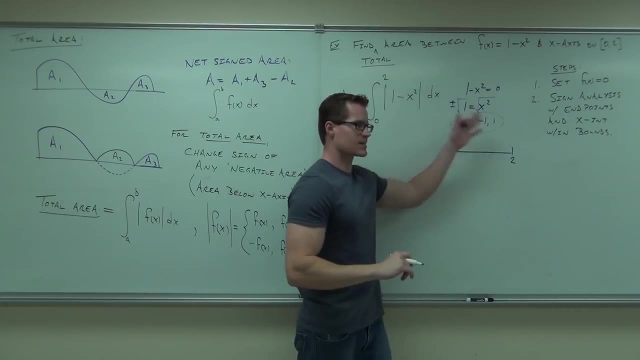 We're going to make a side analysis test in case you forgot. What you do is: you take your bounds of integration first. The bounds of integration start at 0 and they end at 2.. You take any of those x-intercepts that you have. 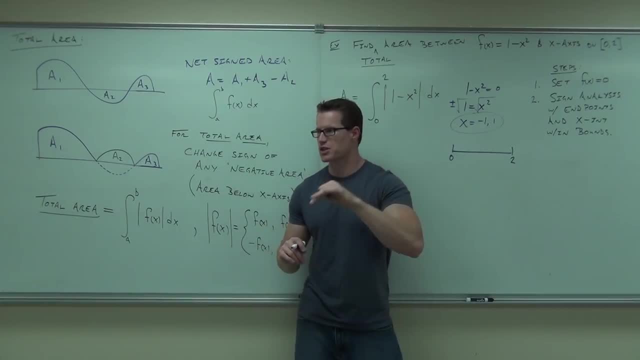 Those are the places where you're crossing the x-axis and therefore that's the places where your signs could possibly change. Well, only one of them, That's one. Feel okay with your side analysis so far. After that, after you make that number line, you just determine when f is above 0 and f is below 0.. 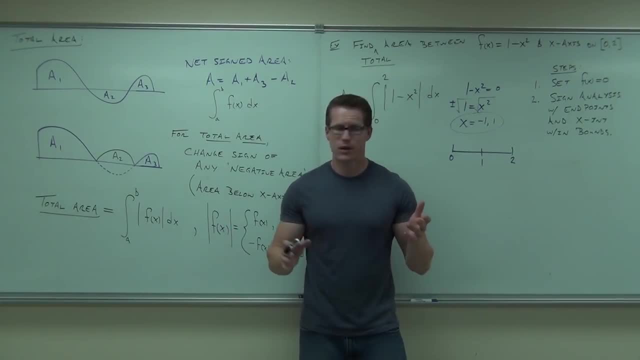 Okay, That's just plugging in a point. Plug in one point for each of these intervals. That's only two. You don't have to go over here. I don't care. I don't care about that one either. I care about these two intervals. 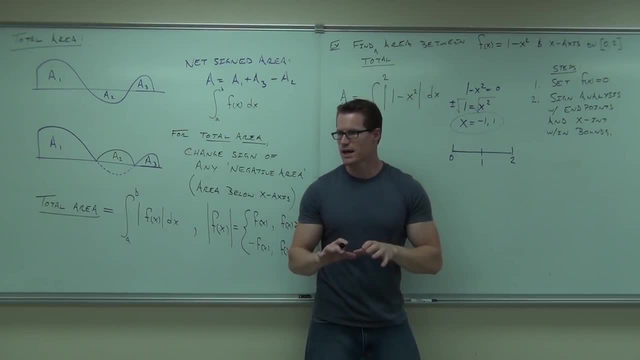 Plug in one point to see whether it's above or below the x-axis. Recall that if it's above the x-axis, the area has to be positive. If it's below the x-axis, the area will be negative, And this is the separating point between those two areas. 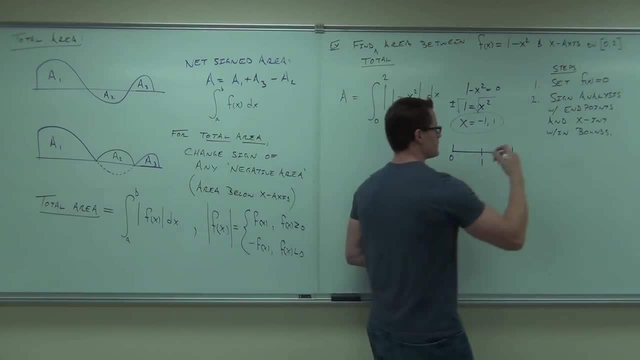 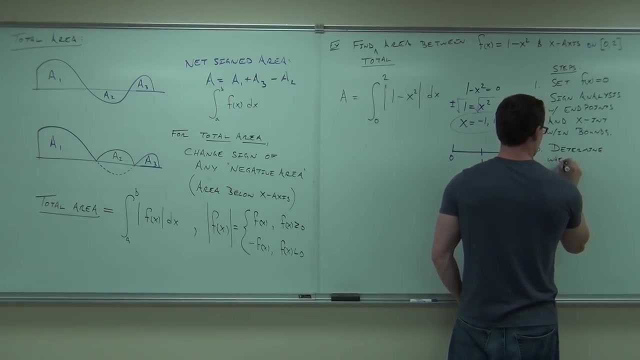 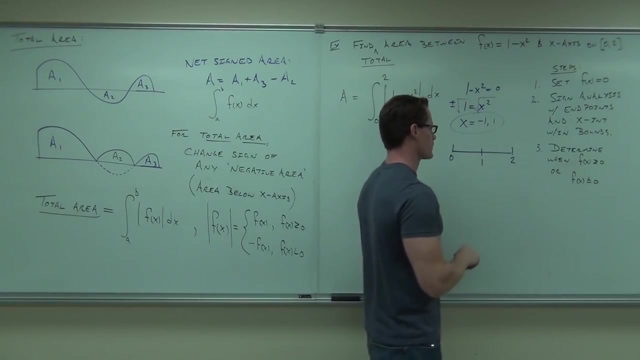 That's why we said it equal to 0. So we're going to determine when f is greater than 0. That would be above the x-axis or less than 0, below the x-axis. Have you done it already? You plug in probably one-half. 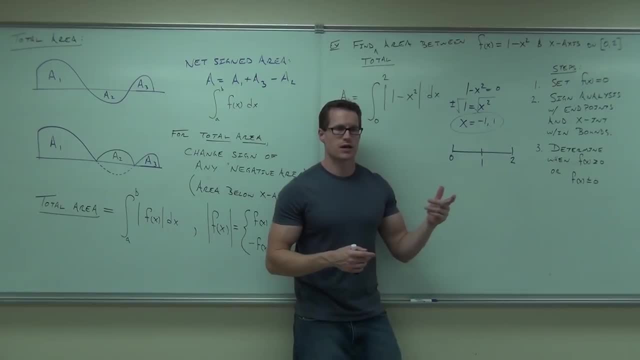 Where are we plugging this in, by the way, To our original function. Yeah, plug in the function. It's going to tell you: I don't care about the number, I care about the sign of the number. Which one's one-half. 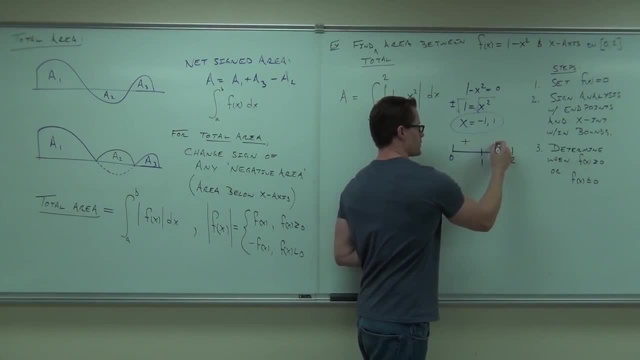 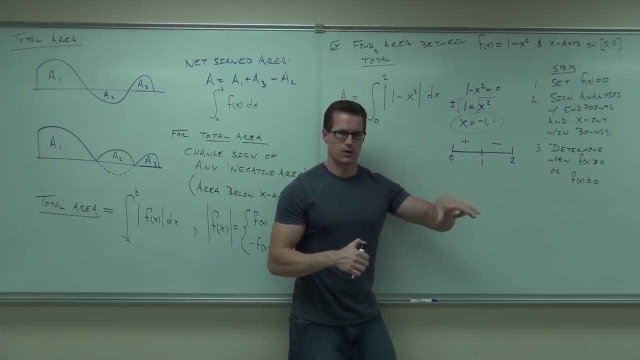 Positive. Okay, So this is positive and this one's negative. Cool, What this says is that from 0 to 1, I'm above the x-axis. From 1 to 2, I'm below the x-axis. We're going to have to come up with that sign change. 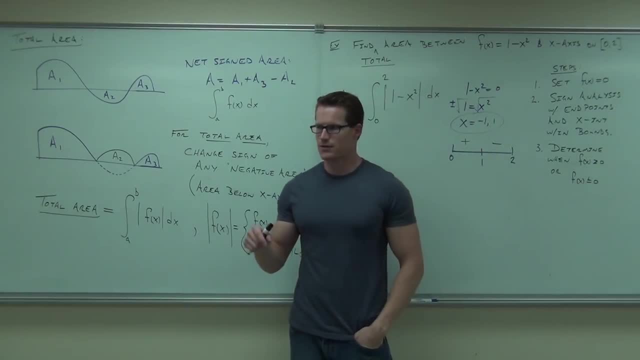 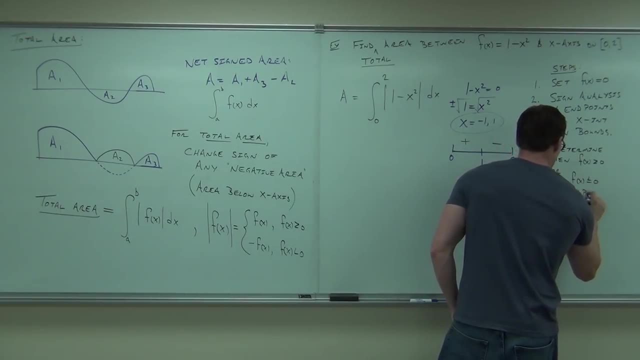 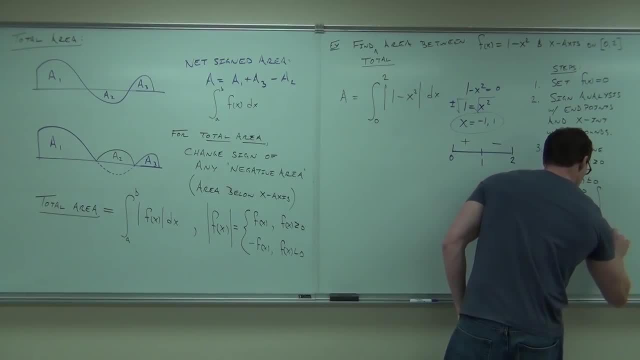 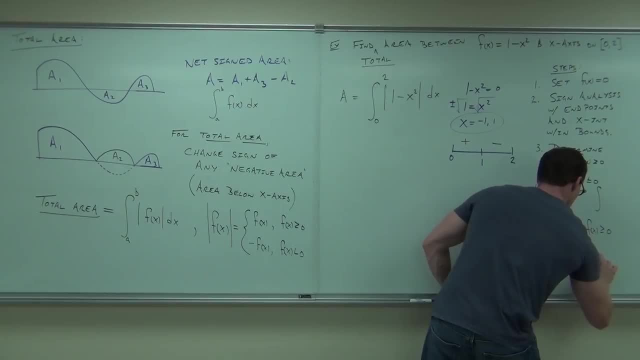 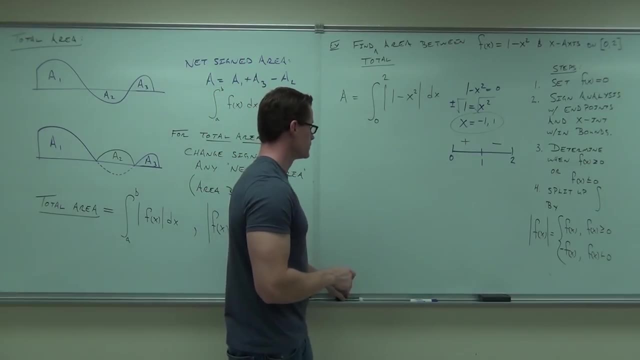 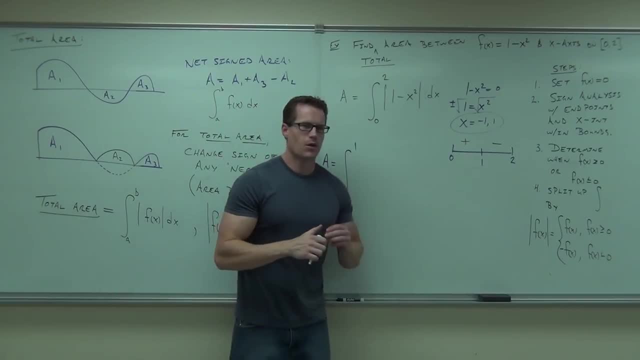 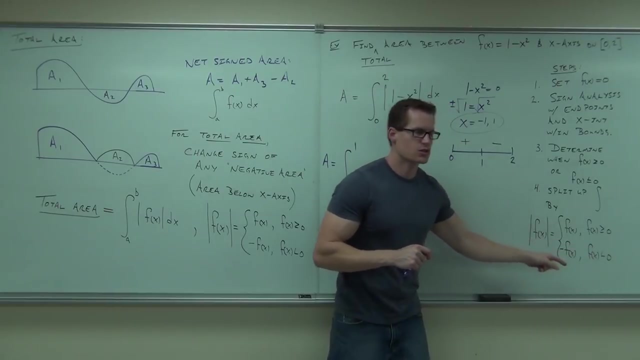 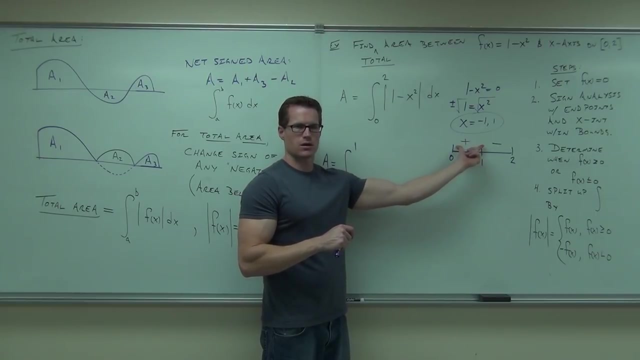 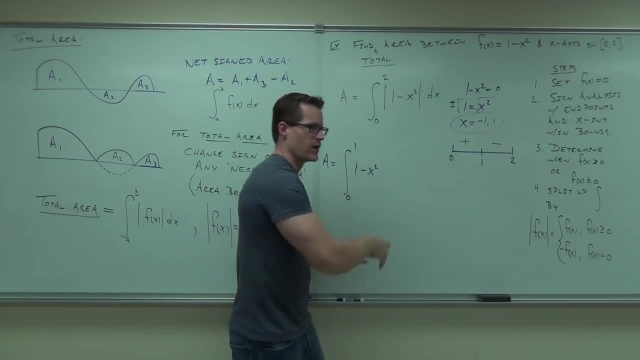 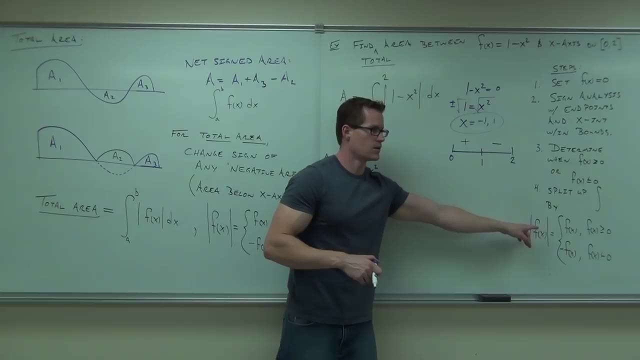 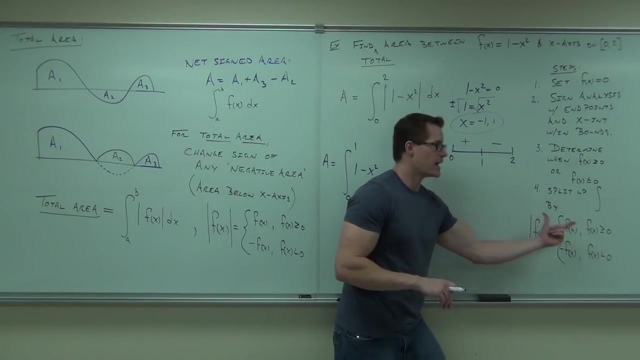 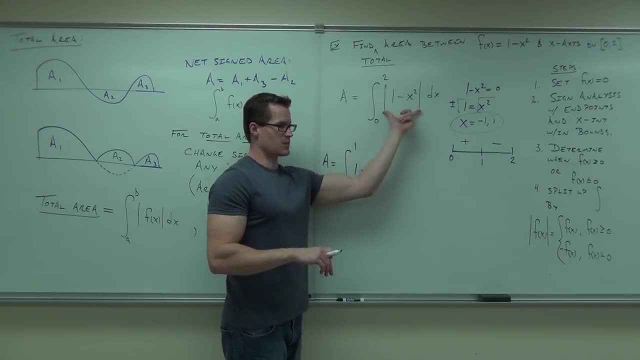 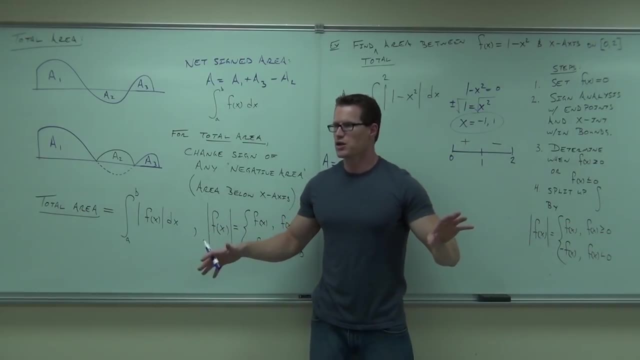 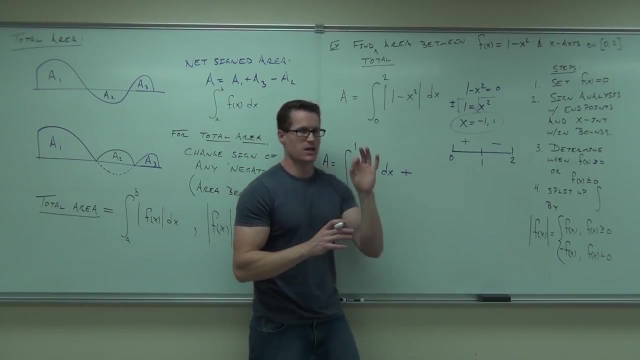 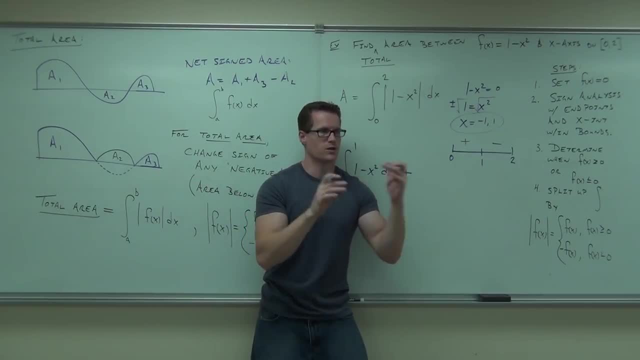 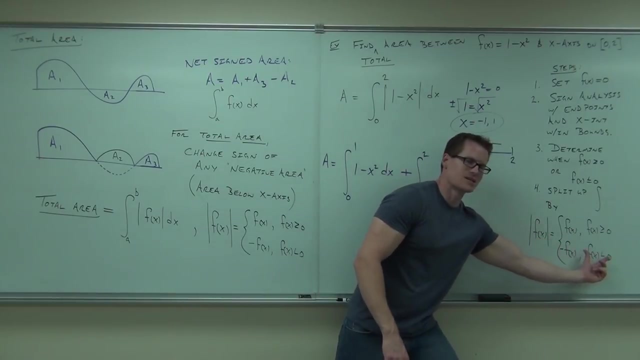 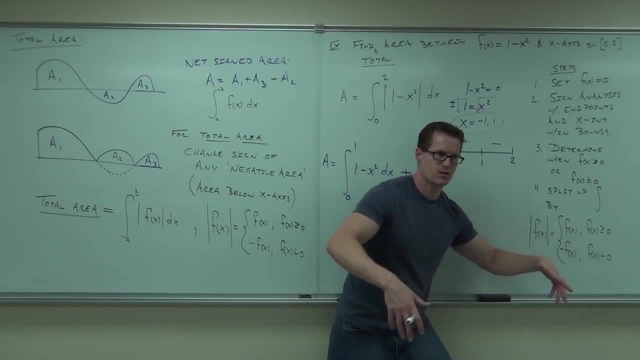 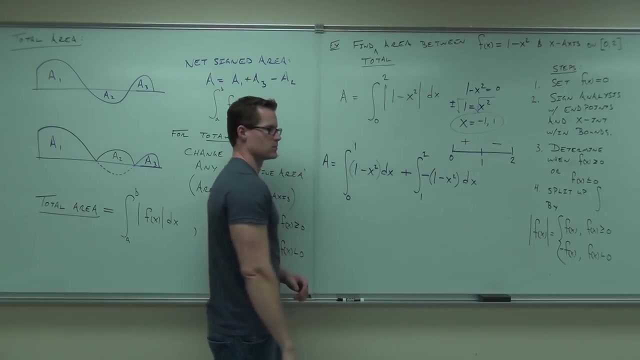 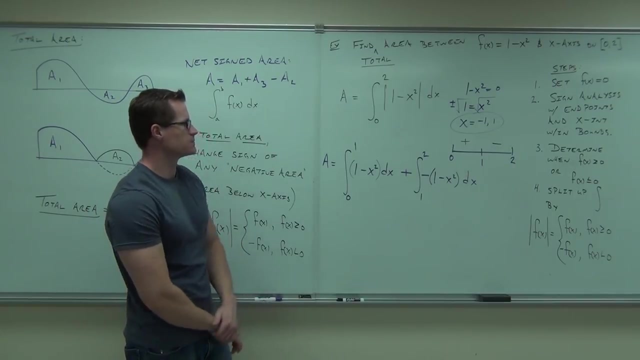 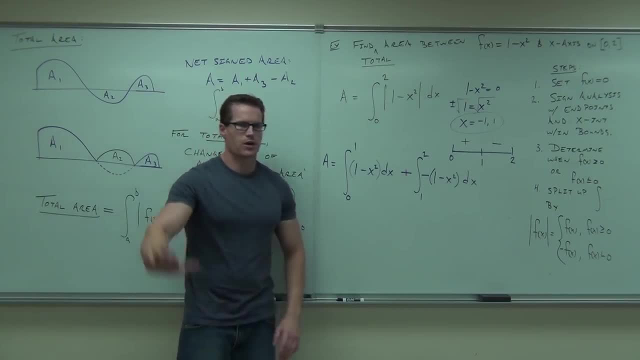 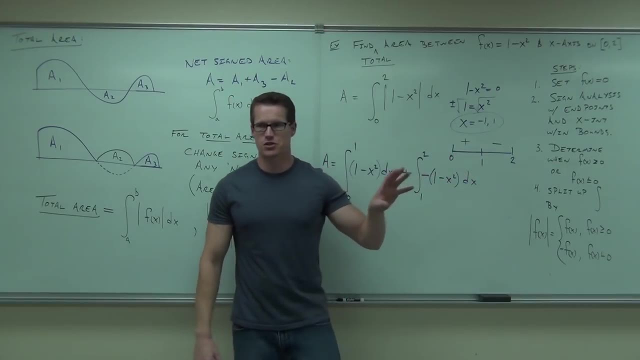 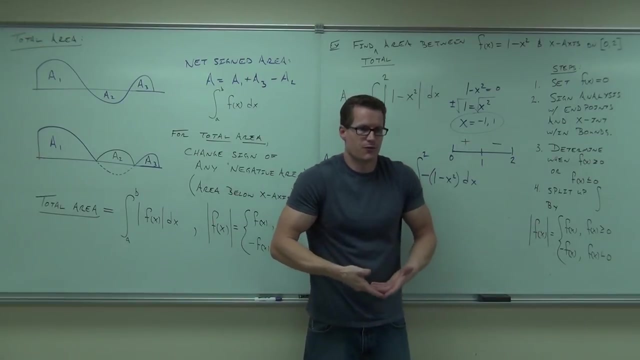 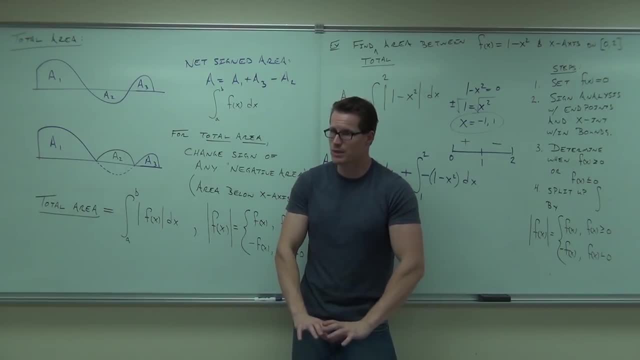 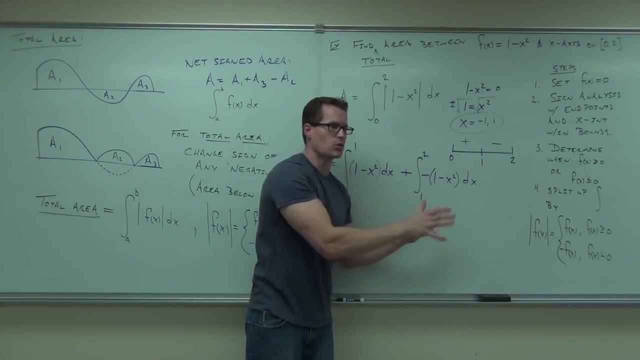 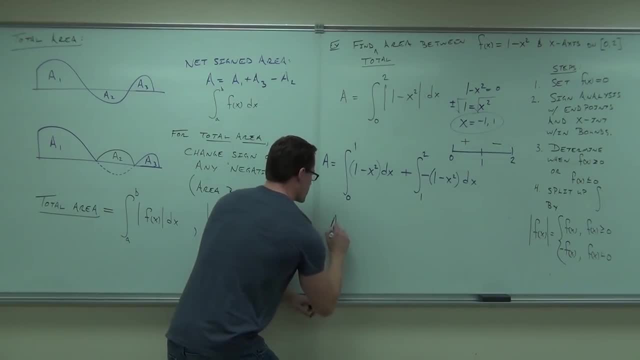 Okay, Okay. Okay means that the area is zero to one of one minus x squared dx, minus one to two: one minus x squared dx. I'm doing this just so you can see this part of it. Check it out. You know this area's positive right. 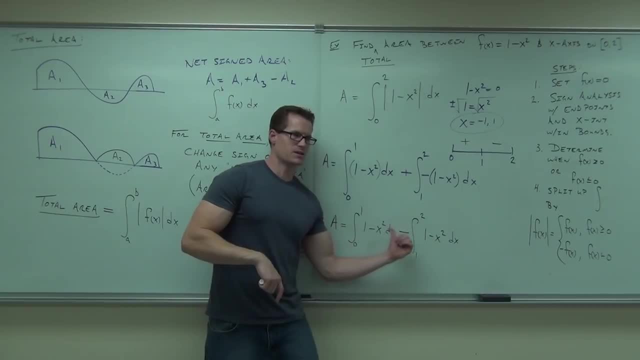 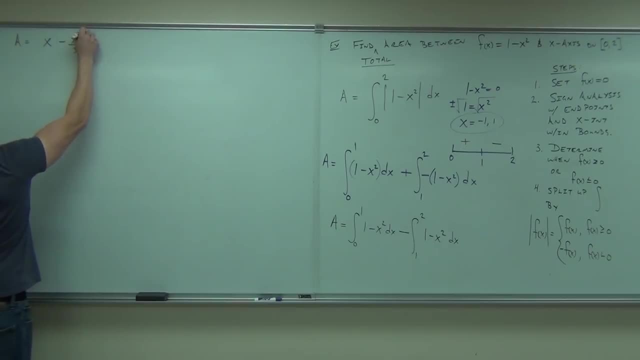 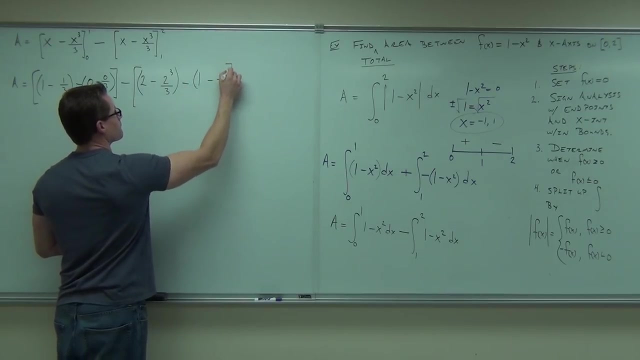 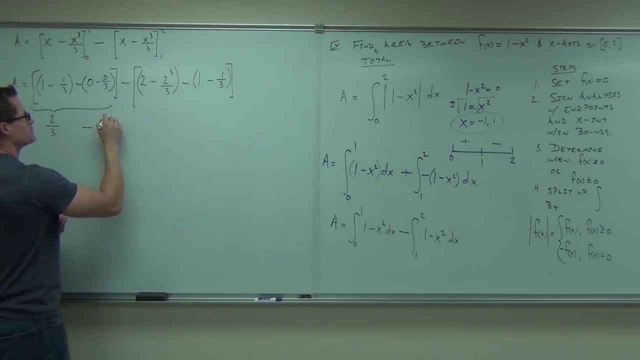 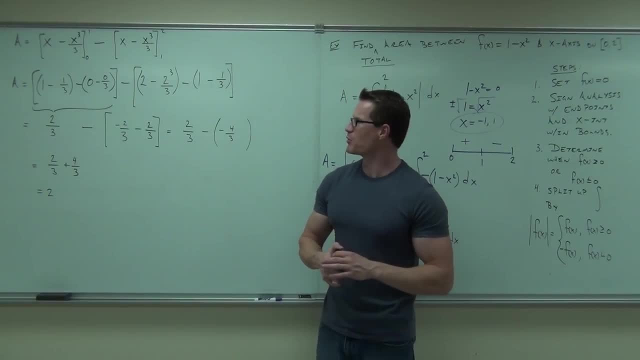 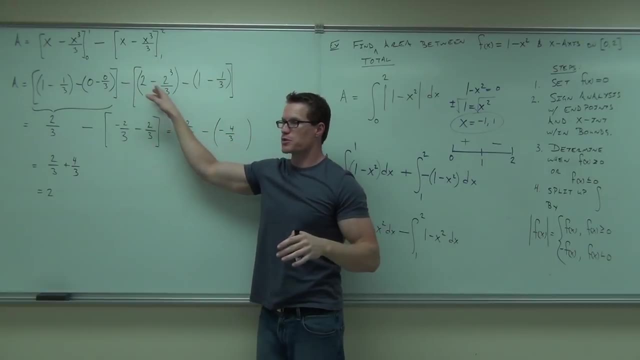 but hopefully you got two. How many people were able to make it down to to this part right there, that part integral? Did you get that part Good? Did you plug in all the numbers? at least this far? From here on out it's just fraction work. 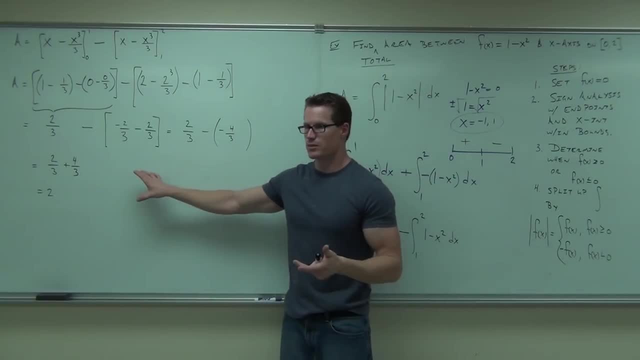 Calculators are fine. I don't care, As long as you're able to get the right answer down here. be able to do that. Can someone please double check my work to make sure that I am correct on that? Make sure all my signs are right. 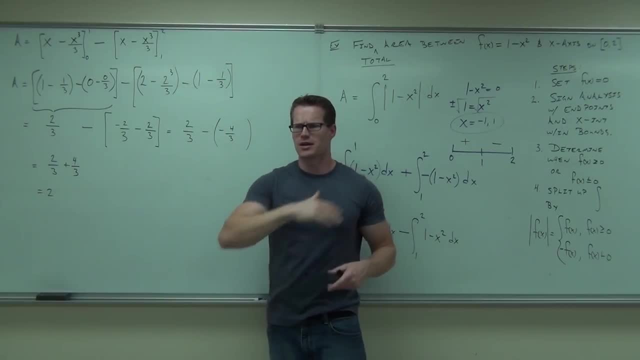 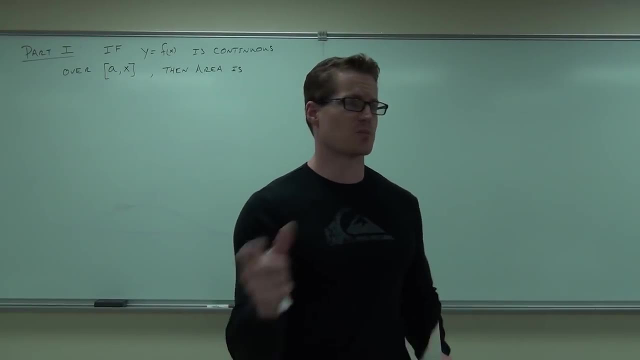 You did. How many double checks do they have? that got two. Good for you, Good for me. actually, I did a lot Shoot, Alright. well, we're ready to tackle the fundamental theorem of calculus, part one. The first part we did was actually part two. 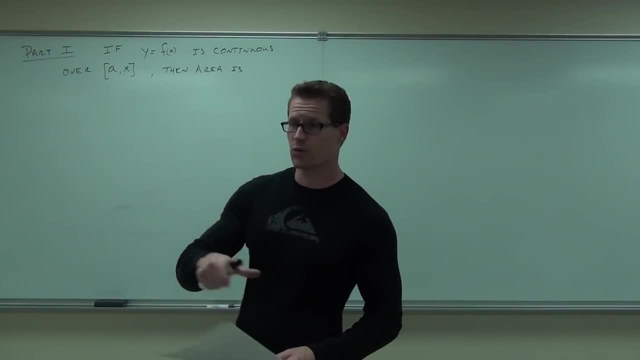 That was all the area things and being able to calculate a definite integral, which means an area, by doing that whole subtraction: Find the antiderivative plug in B, find the antiderivative plug in A and subtract the two. 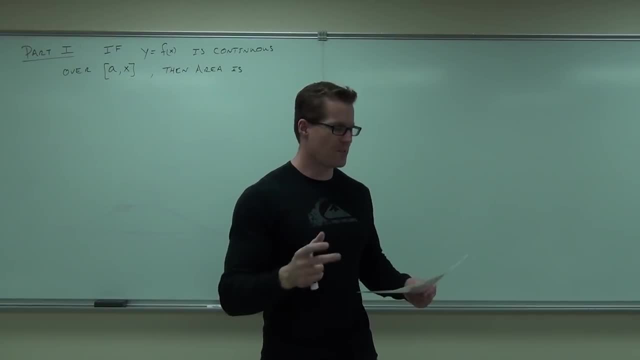 That's the fundamental theorem of calculus, part two. The part one basically says this: It says that derivatives and integrals are inverses. It says one undoes the other. That's basically the idea in the most small sense I can make it. 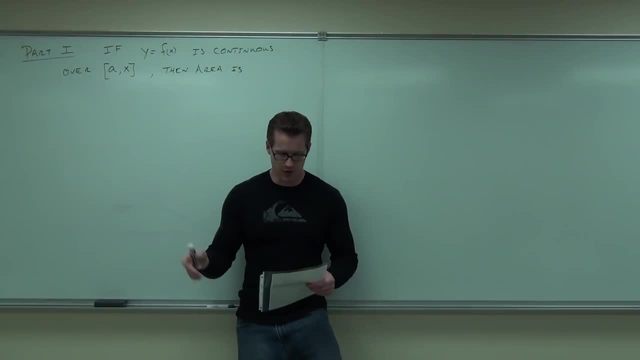 So let's suppose we have this function: y equals f of x is some function and it's continuous over a certain interval, Starts at A, a point, and ends wherever we want. Ends at some x, down the way. You get me on that. 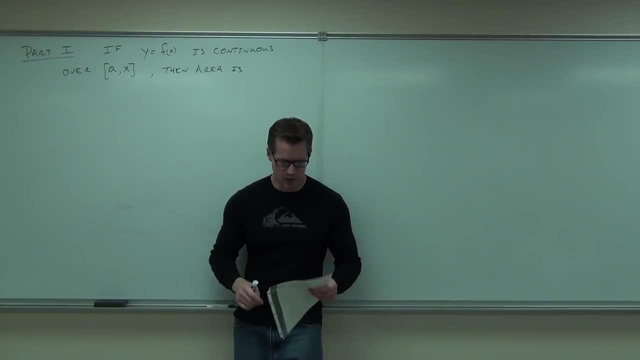 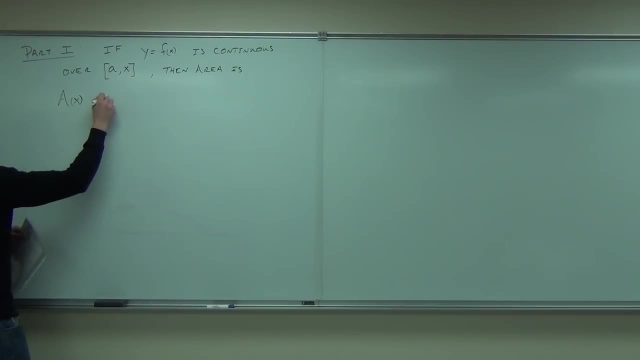 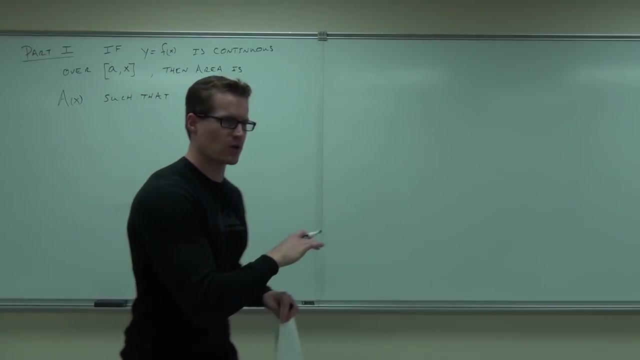 Some x, even changeables, provides continuous up to that point. Then the area is A of x. We already know that Area is gonna be some area function, such that when I take the first derivative of my area, what does it have to give me in this case? 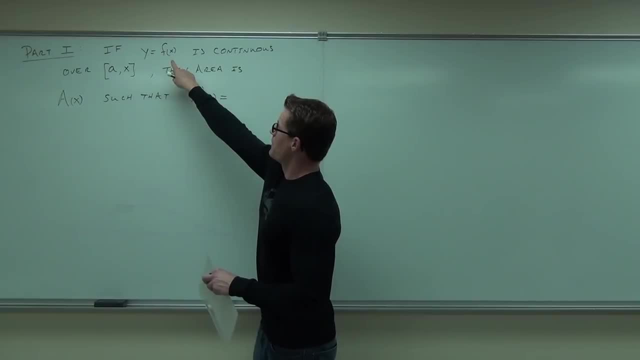 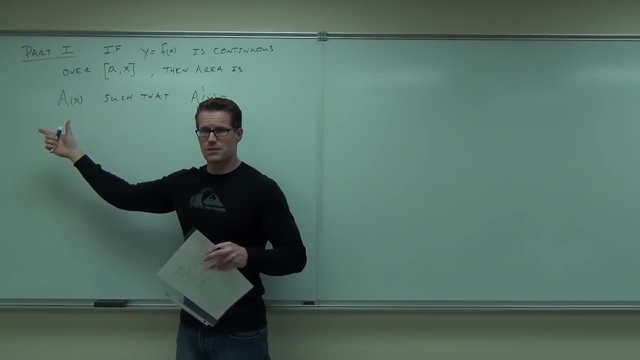 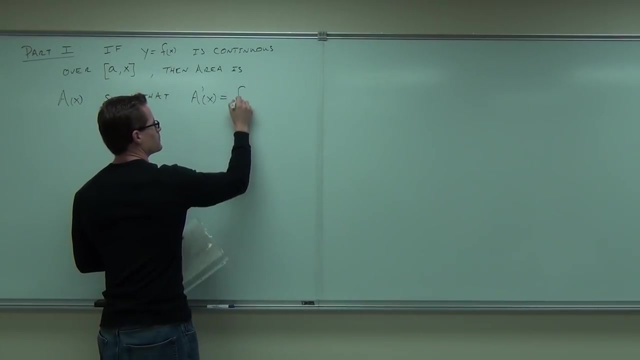 Say it again: Very good, So if f of x is continuous over this, then the area is A of x. Some area function and the derivative of the area function must give me back my function, my original function. That was the antiderivative thing. 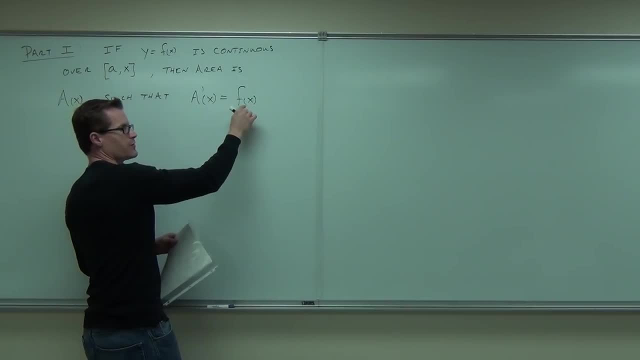 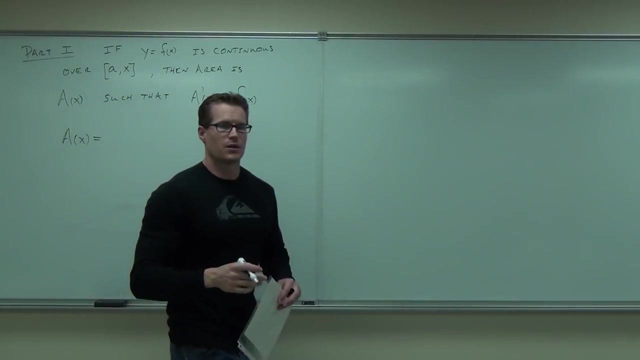 Saying that this is the antiderivative. This is the anti-derivative of that, treating this like a derivative and going backwards. Well, I could write that a different way. I could write that also, as the area then should be the integral of f of x. 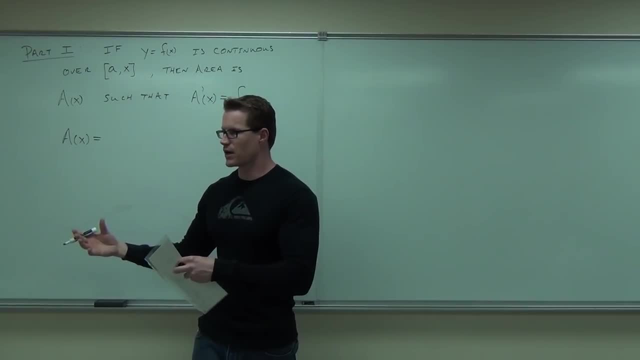 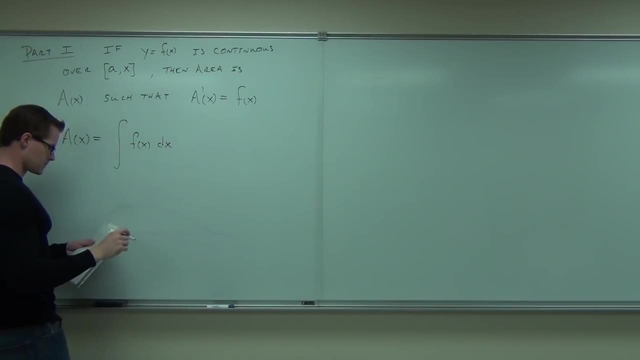 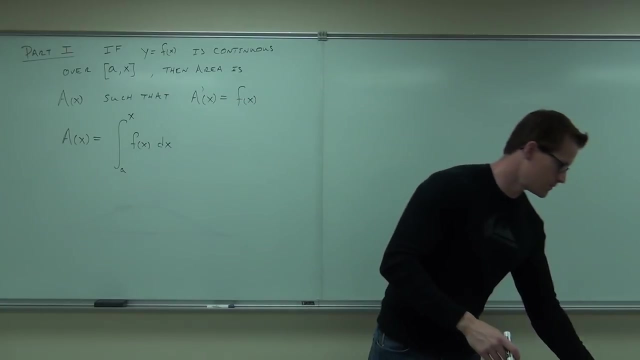 We also had that from the, from what we've been studying right. It says that if I want to find the area, it should be the integral of f, of x, dx, from a to x. You okay with that as well. 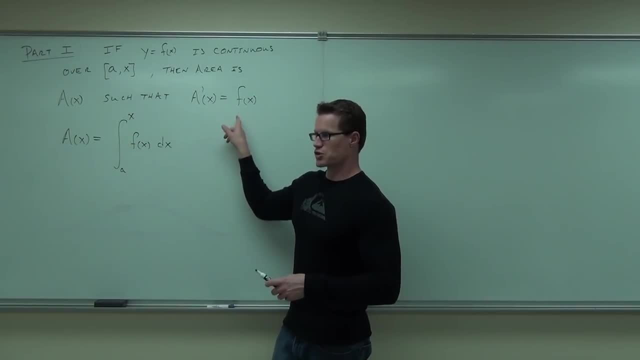 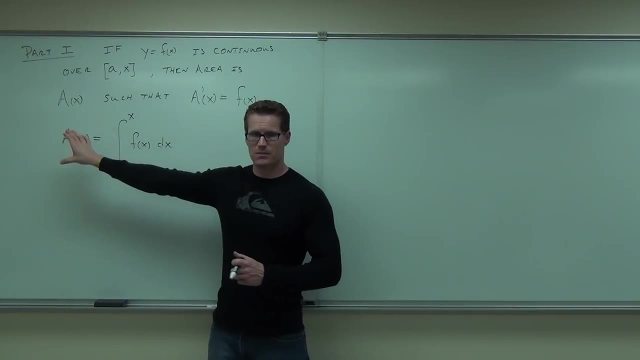 It says that the first derivative of the area is going to give me my function back. Therefore, the anti-derivative of my function between my two bounds, whatever they happen to be, should give me my actual area, should give me the area. 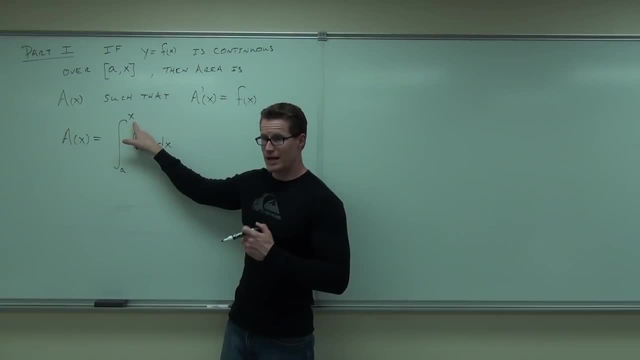 Now this is in terms of not a b but an x, so as to give me the a of x, Not the actual area. Does that make sense? It would be a function of the area. That's what it's saying there. 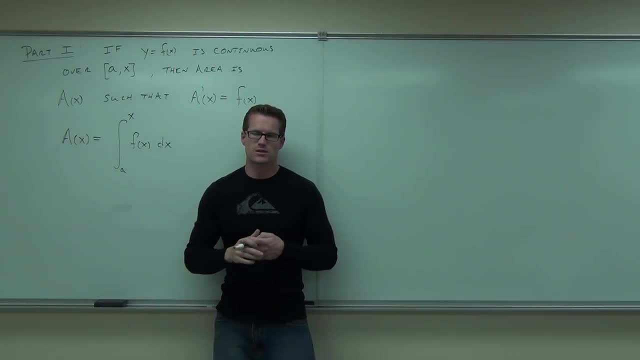 How many of you feel okay with that so far? Now I'm going to do one thing so that we don't get a little bit confused, because it's kind of awkward to have a function in terms of x and then have a bound of x. 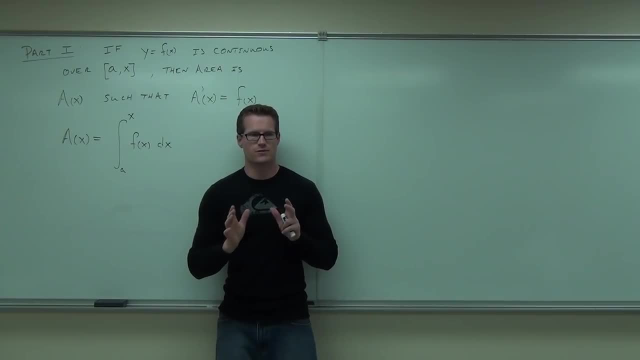 What we use here is called a dummy variable. It really doesn't matter. It's just a variable that we're going to be integrating because you're going to be plugging in x later anyway, so the x's will appear. So typically what people do at this point is they go. you know what? let's not call it f of x. 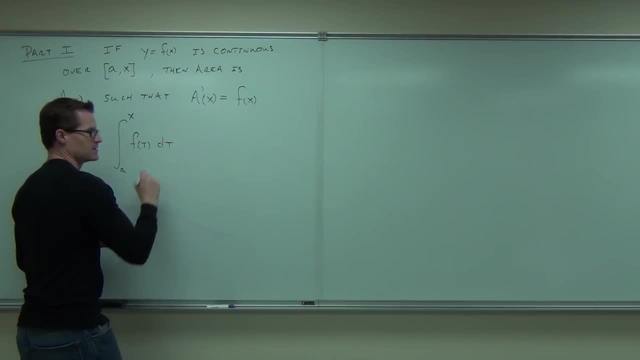 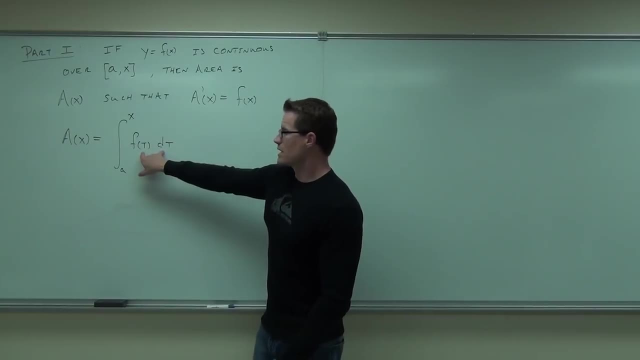 Let's call it f of x. Let's call it f of x, Let's call it f of t dt. They make it a dummy variable. Now, why the dummy variable doesn't matter is because, when you think about it, when you take the integral of this, you're going to have a function in terms of t, correct? 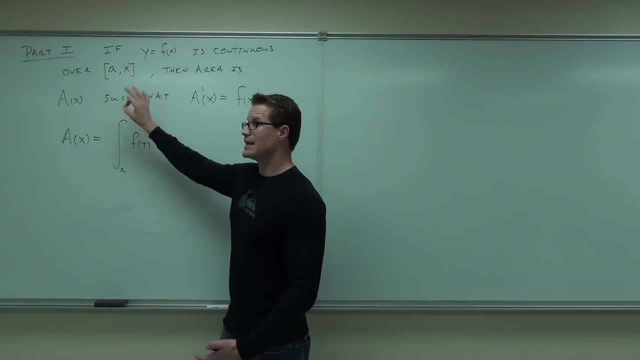 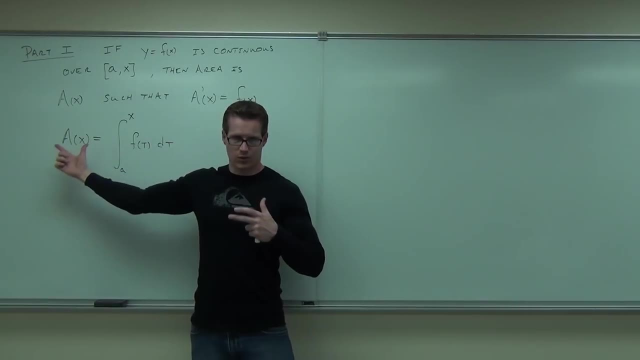 But look at your bounds of integration. You're going to go from a to x. You'll be plugging in the x's somewhere for your t's. You'll reinsert them into your equation. That would give you an area function in terms of x, like we're looking for. 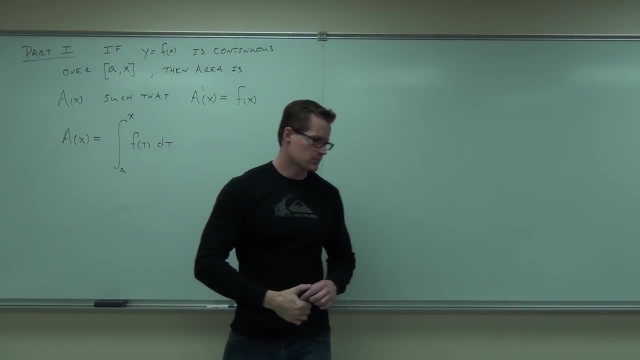 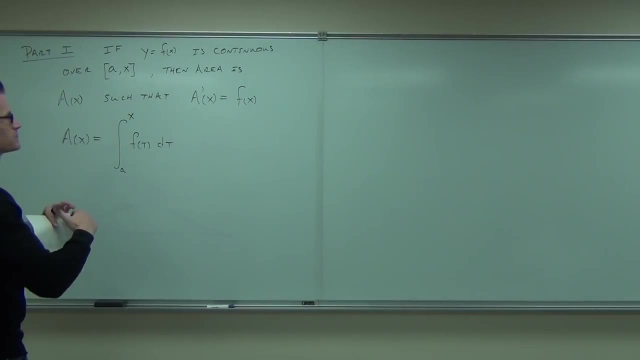 How many of you feel okay with this so far? Okay, Well, here's the basic idea. I'm going to try to tie all this together for you, real nice and neat. I'm going to try. I'm going to try to try. 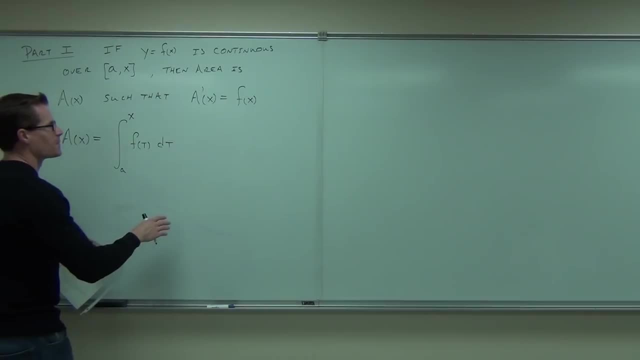 I really will try to make it neat. Would you agree that this equals? I'm going to try to try to make it neat. Would you agree that this equals f of x? Yes, Uh-huh, For sure You believe that. 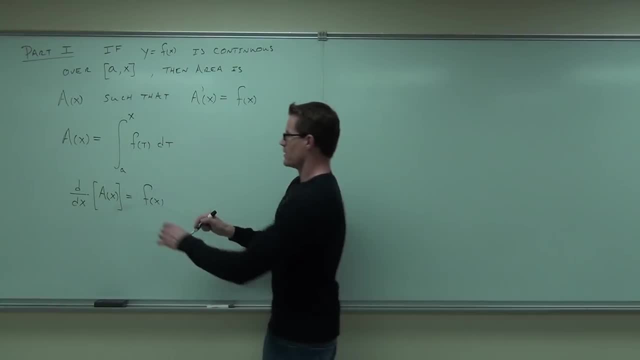 Yeah, Oh, then we're almost done. That's fantastic, Very good, Because this means a derivative right, That means a derivative. So the first derivative equals f of x. The first derivative equals f of x. However, we also have this statement right here: 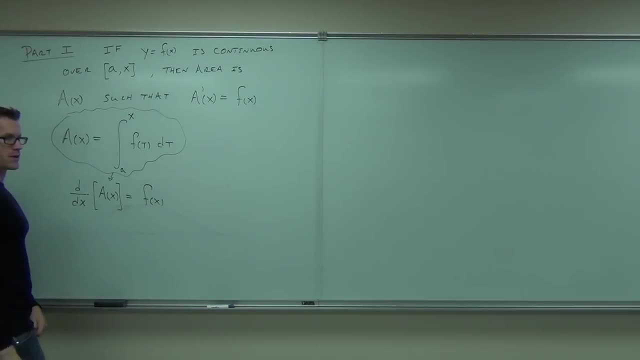 What I'm going to do is make a little substitution right there. So what this says is: the derivative is equal to f of x. Okay, So what this says is: the derivative is equal to f of x. Okay, So what this says is: the derivative is equal to f of x. 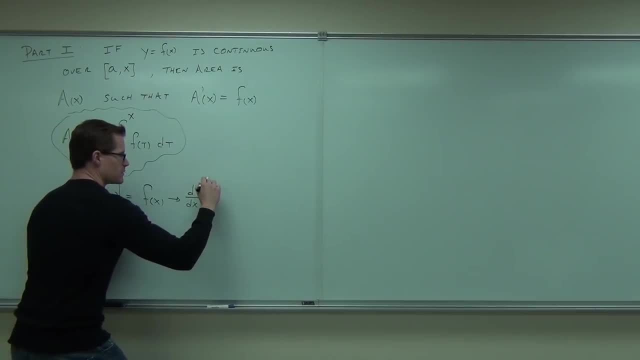 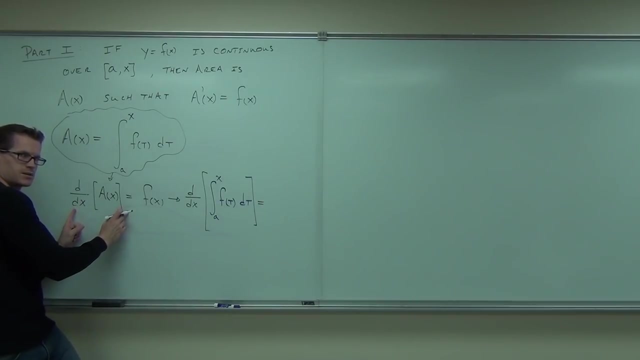 Okay, Okay, Okay, Okay, Okay, Okay. of a of x. Here's another interpretation of a of x. What's it have to equal? What did this equal? Are you seeing that this is the same thing as this, Yes or no? 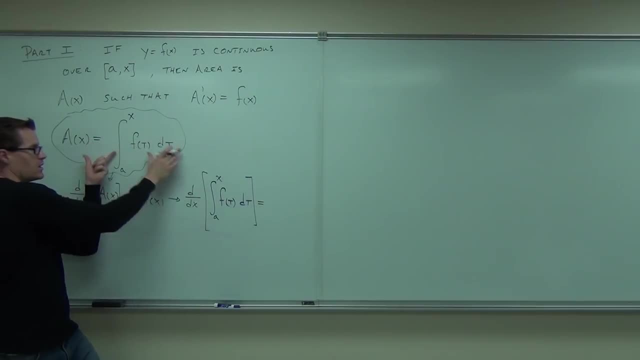 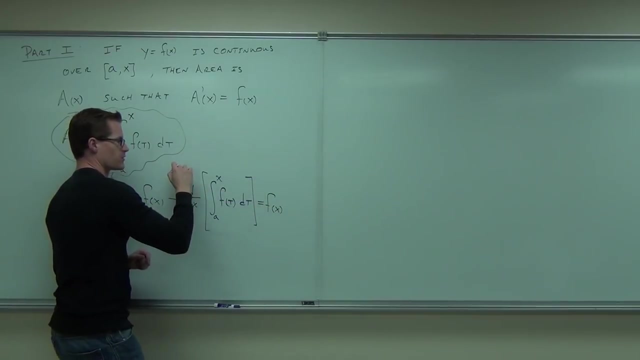 This is a of x, so is that from right here? I just went this way, I made a of x. that way That has to equal f of x as well. This right here is the fundamental theorem of calculus, part one. Yeah, because we talked about this first. 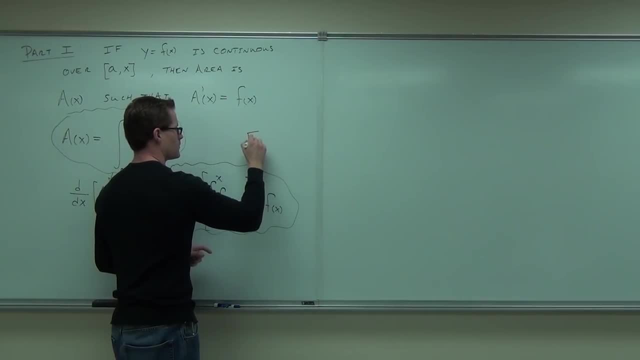 And does it, And so you have the f of t. because of the way you do the integral, you're just swapping it out and reinserting your x to make it come out with f of x, not f of t. Right, We use the t here so you don't get confused with x, with x. 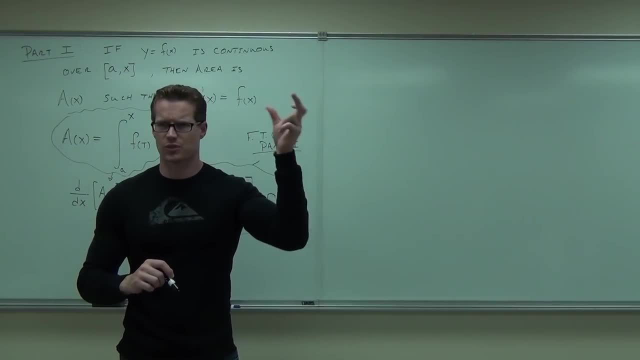 because it's hard to think about. oh, I'm going to plug an x in for an x. That's weird. Why do we do that? So what we do is we use a t and say: I'm plugging in both x and a for my t. 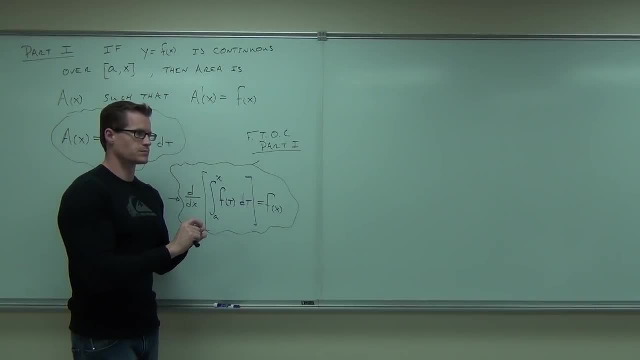 Or you could use x subscript one, x subscript two to keep them separated. Or does it matter what we use besides t? Yeah, No, You could use an h there if you really want. t is a dummy variable. It doesn't really matter. 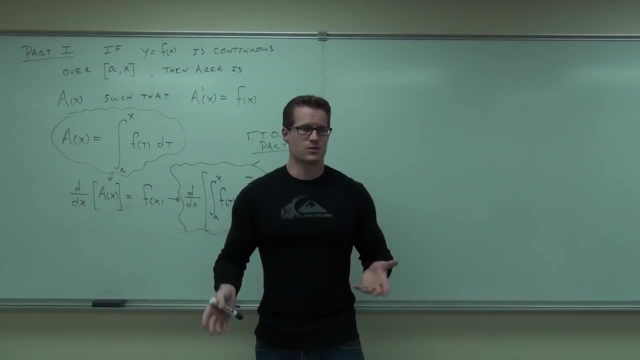 You're going to be integrating some variables, right. For those variables, you'll be plugging in x's. That's the idea. Did you follow? a of x equals this. Derivative of a of x equals this. Therefore, derivative of this equals f of x. 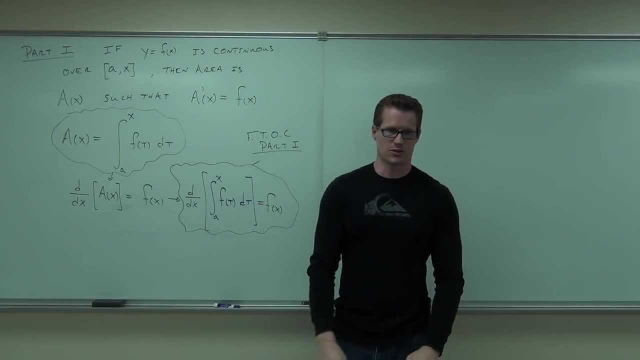 That's the fundamental theorem of calculus part one. Here's what it says in plain English. It says: if you take a what's this stand for A derivative Of a what's this stand for Integral, It will give you back your. 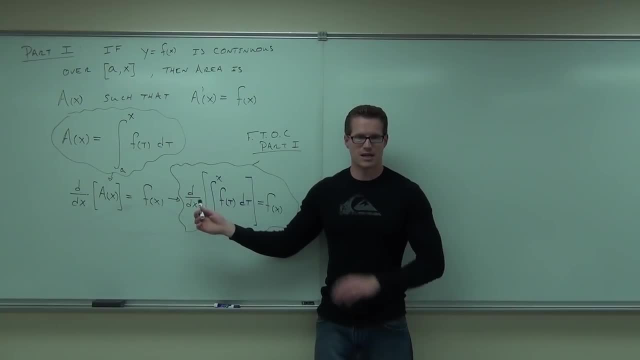 Function. That's it. If you take a derivative of an integral, basically it undoes everything. It essentially says they're inverses. It says a derivative undoes an integral. An integral of your function gives you something right, An area function, as it were. 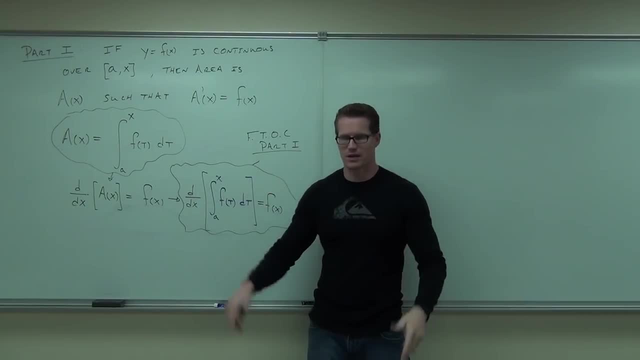 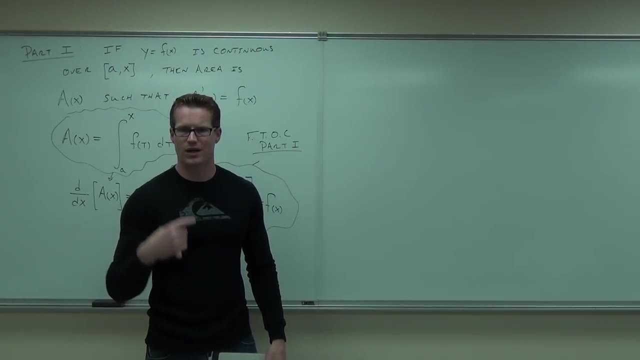 Then you take a derivative of that, gives you it right back, Gives you your original function back. Now, why, Why, Why is this important? Because that seems pretty common sense, doesn't it? We've already kind of thought that, well, I mean shoot. 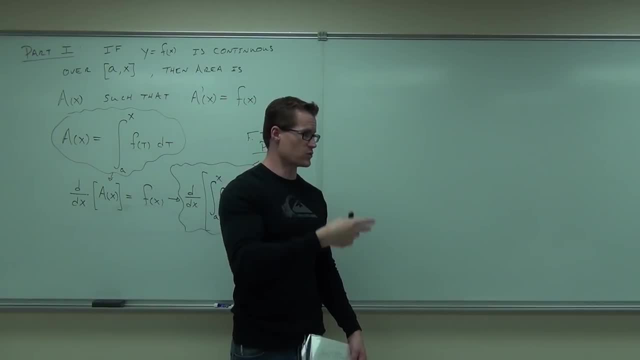 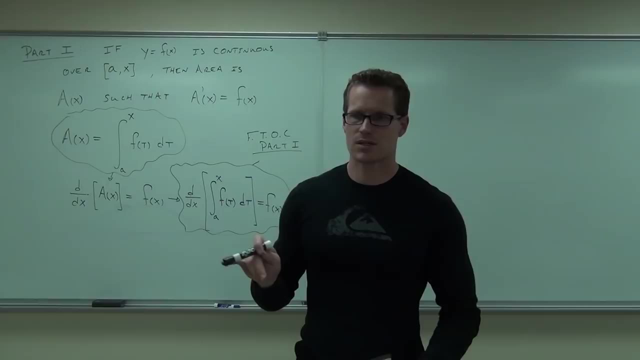 If an integral is undoing a derivative, it should be the inverse of a derivative. This proves it that a derivative is the inverse of an integral. But how? why we do? it is because sometimes it makes certain integrals very easy to do. 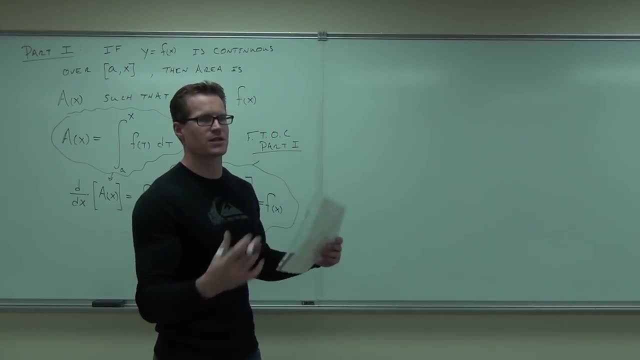 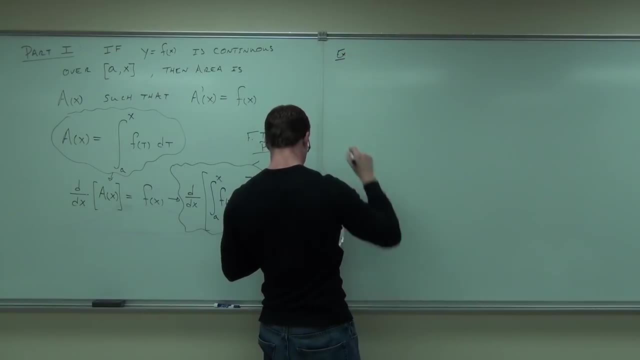 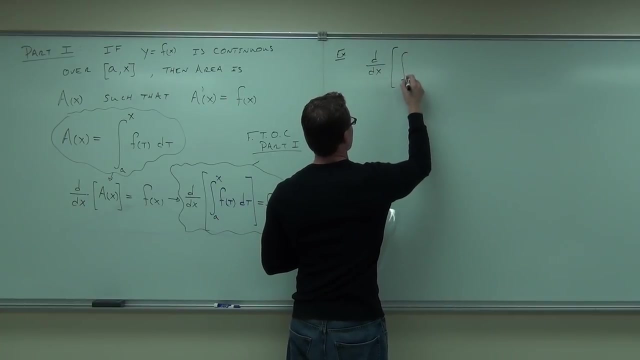 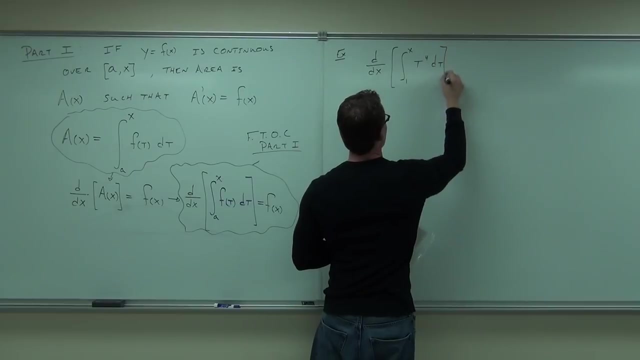 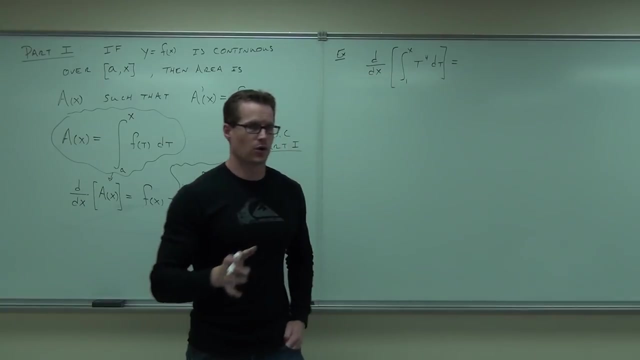 Now here's why. Maybe not certain integrals, but certain computation is very easy to do Without doing any work. any work. you can tell me what this is Actually. say what T to the fourth, Not T to the fourth. you're very close. 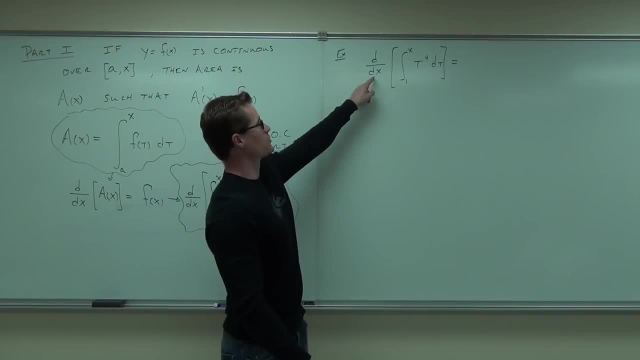 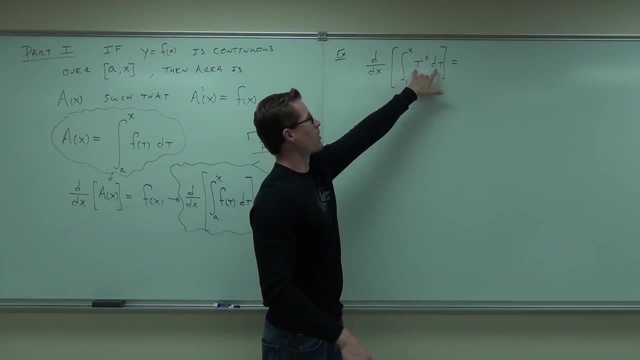 X to the fourth Without doing any work. Why? Well, because you have a derivative of an integral. The integral starts, I don't care, but it ends at X, wherever it is. That means that this is going to be, whatever our dummy variable is. 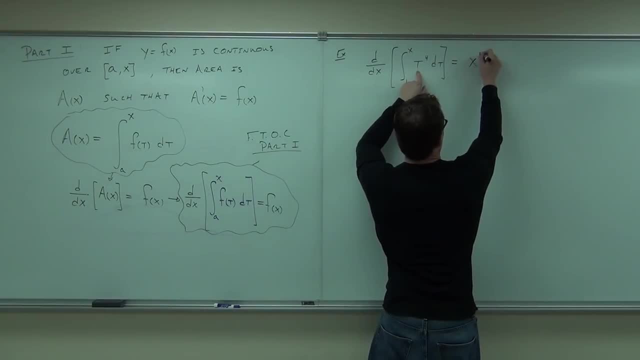 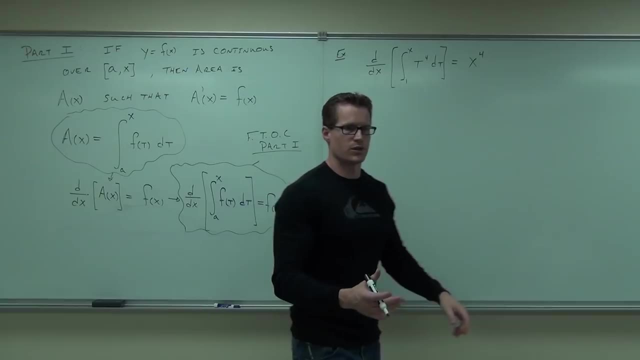 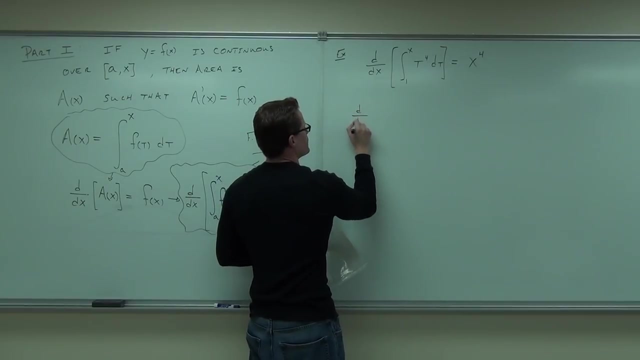 but with an X instead. So this becomes X to the fourth, By this, by this theorem, by that theorem. If you want to see it proved out which we can do that directly, I'll show it to you right now. that would be a derivative. 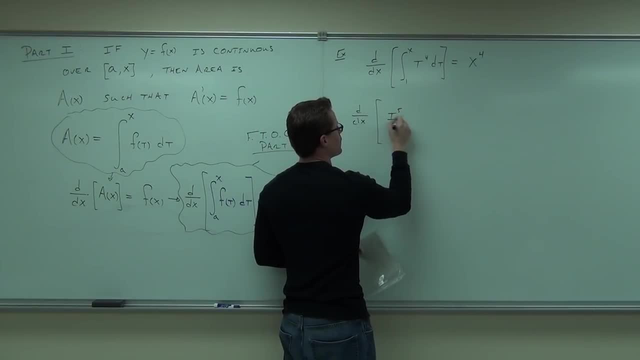 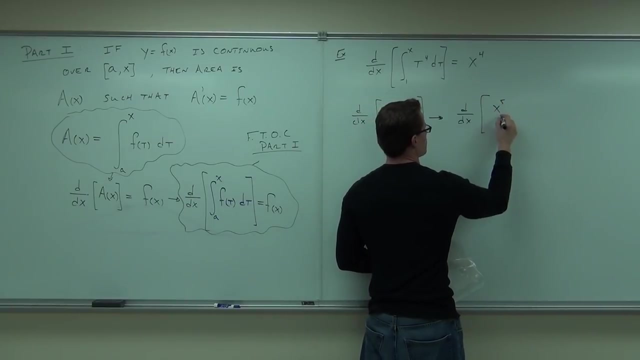 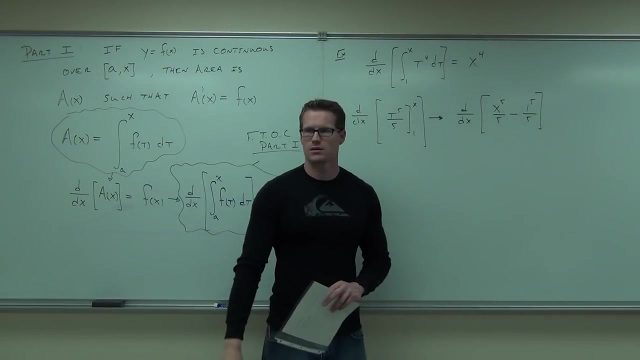 You have an X and a dome. If you did the integral, you're going to get T to the fifth over five From one to X. True, What that would give you is a derivative of X to the fifth over five, Minus one to the fifth over five. 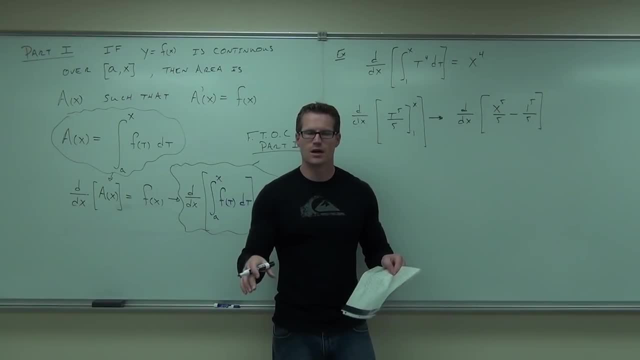 Do you see where the X is coming in? Do you see why we have a dummy variable Doesn't really matter, You're plugging in X for it anyway. Okay, Do you see why this number doesn't matter? When you plug in a number to that, you're going to get all constants. 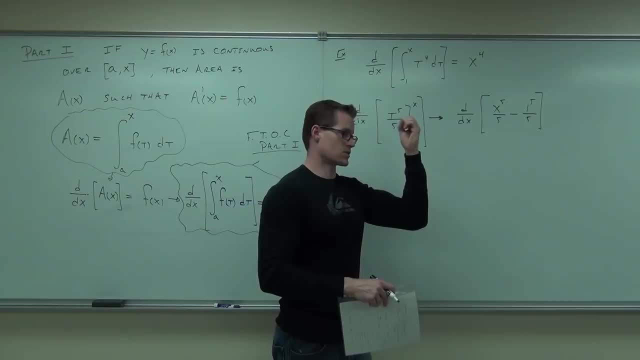 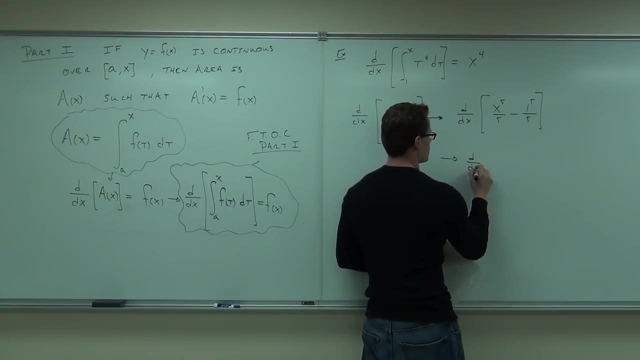 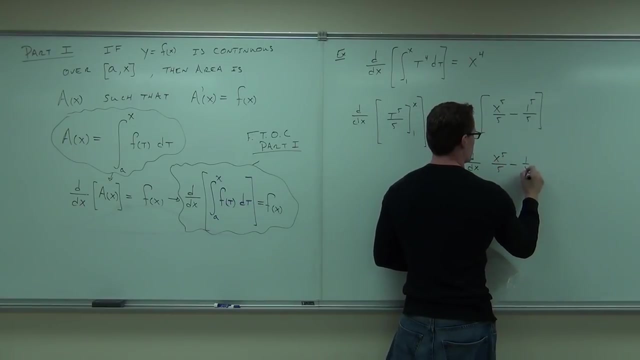 What happens when you take a derivative of constants Zero, Zero, So really only that matters. So you're going to get a derivative x to the 5th over 5 minus 1 5th. What's the derivative of x to the 5th over 5 minus 1 5th? 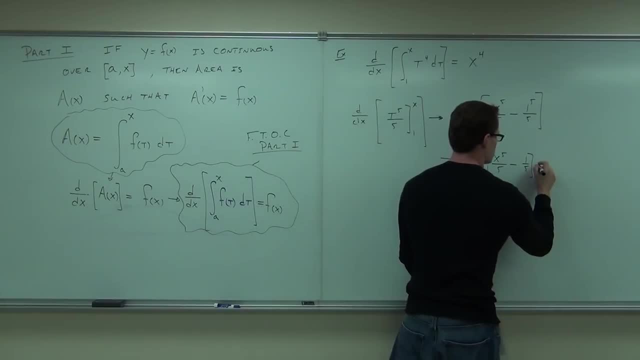 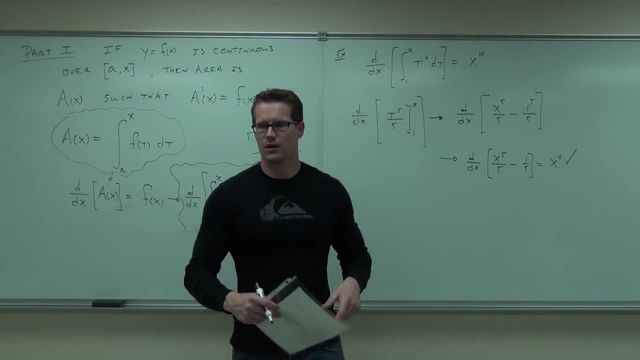 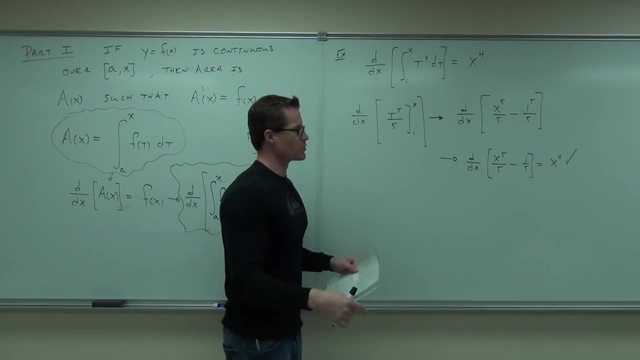 Ladies and gentlemen, which proves it Well, at least for this example. I basically kind of proved it here with this statement. here It's done. There's some more serious proof to it, if you really want, but that's basic enough for us. 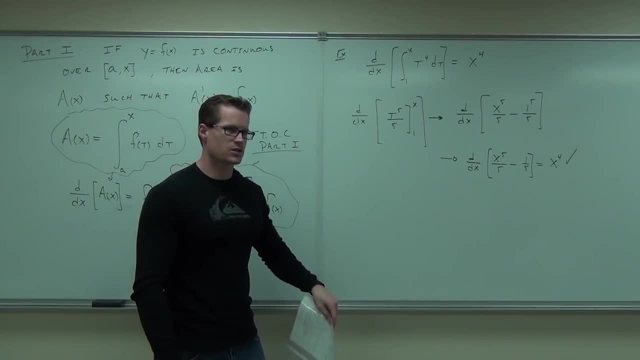 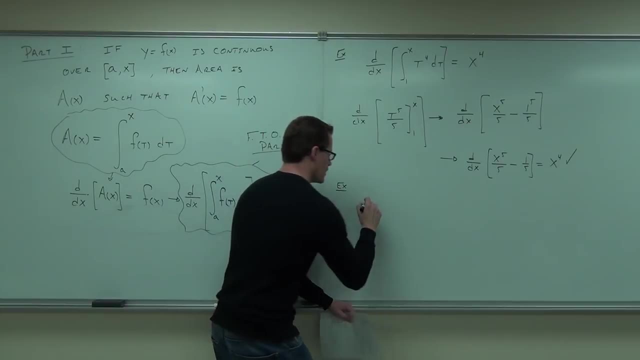 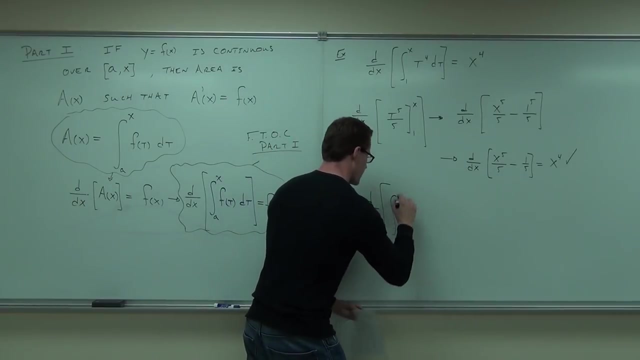 Now that you can do directly, Some of them you can't. So when you get to this integral like this, I don't want you to spend too much time on it because there's no way you can do this integral In this particular class. let's say you had something from 1 to x, sine of t over t, dt. 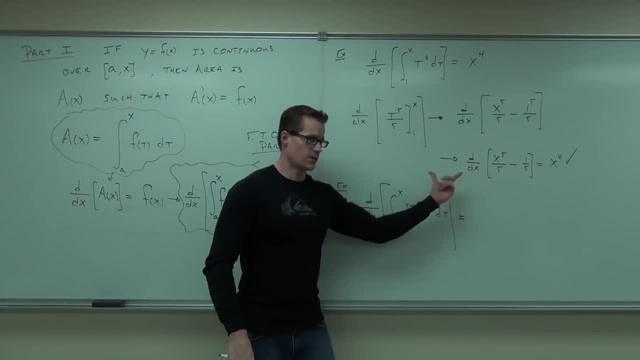 You can't do that integral directly. You can't do it the same way I did it. all right, It's not. you can't just hammer at it, Not in your integration table. you can't do it, However, because you have a derivative of an integral from 1 to x. 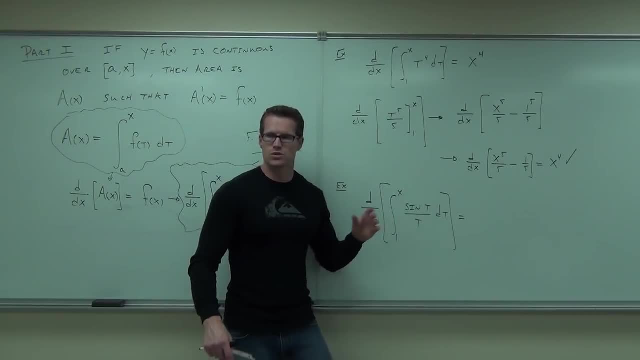 from a, any a to x, you can use the same property right here. So how much is this going to be equal to Sine of x over h? Sine of x over h is right. That's exactly correct. Now one thing does have to be defined for the entire, just like remember how we found. 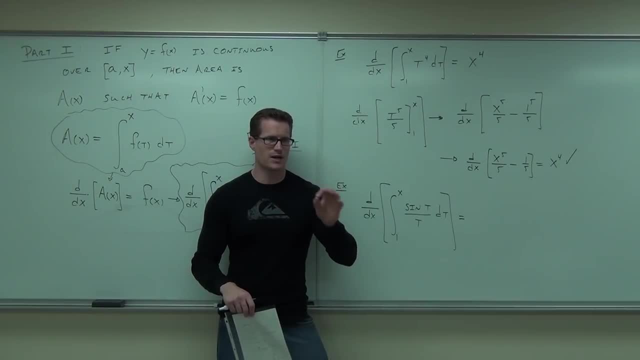 out last time. it's got to be defined, You can't. it's got to be continuous. It's got to be very nice. You can't have the undefined points. It has to be bound somewhere, Are we okay here? 1 to x. Remember, this is a small number, so it can't go backwards. 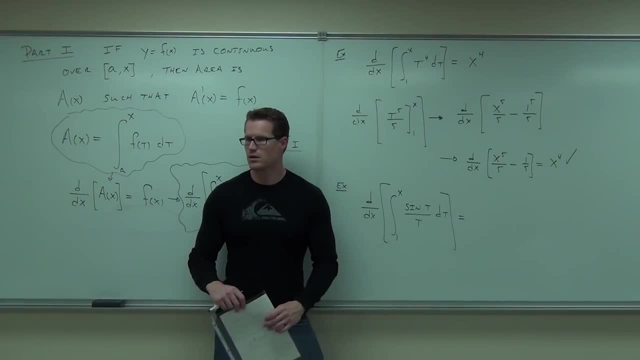 Are we okay? What's the one number? that's not okay. We missed a zero, so we're okay. If this had gone from like negative 1 to x, we'd probably have a problem because we couldn't evaluate that integral. Yeah, that's it. 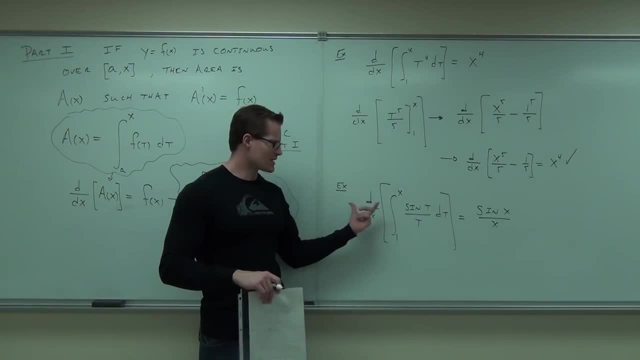 So when you get to some of your homework, some of it's going to be kind of easy If it looks like this: a derivative of an integral, and you're going from a to x and it's defined for that whole region. I mean it starts higher than any problems. 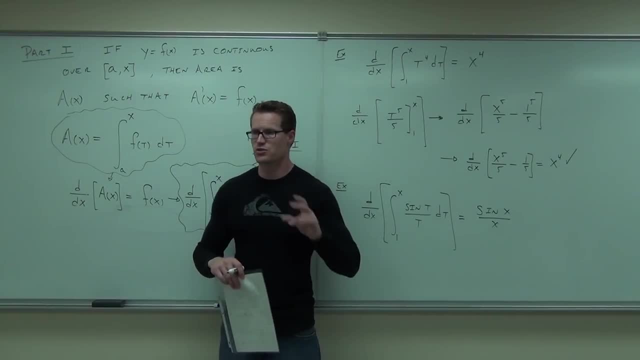 that you have. that's all you got to do. Plug in your x's and your e's, You're done. A derivative will undo an integral. That's the fundamental theorem of calculus. part two, Part one. Part one: What did I say? 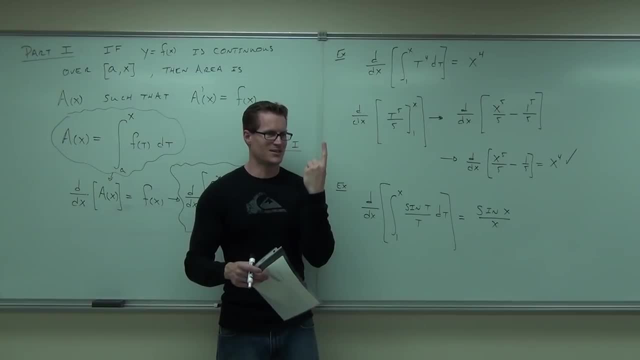 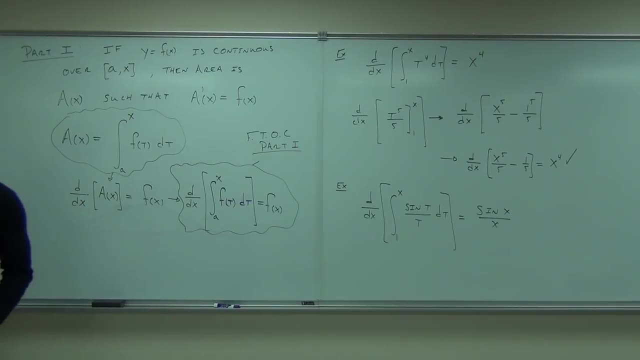 Two, Part one. That's it. I hope you understood that. Good for you. That's fantastic. I wish all integrals were like that. I know right. Well, the thing is, we don't always take derivatives of integrals right next to each other. 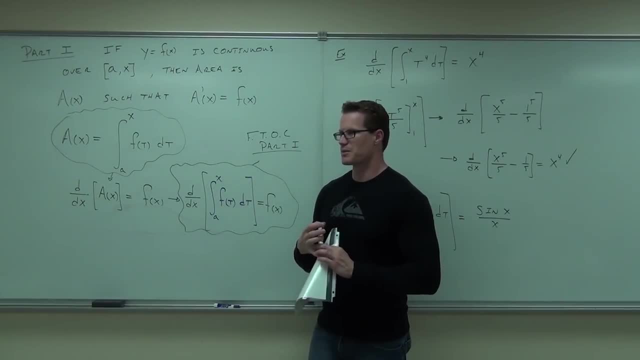 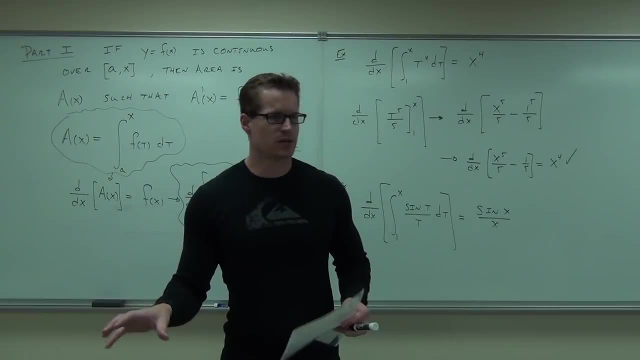 It's not. it doesn't happen very often, but it's a statement that says it is true. It's proving that they are inverses. Now we're going to move on. This is technical. It's typically a different section than most other books. 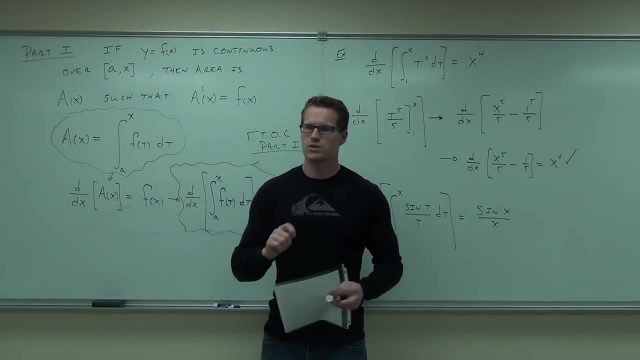 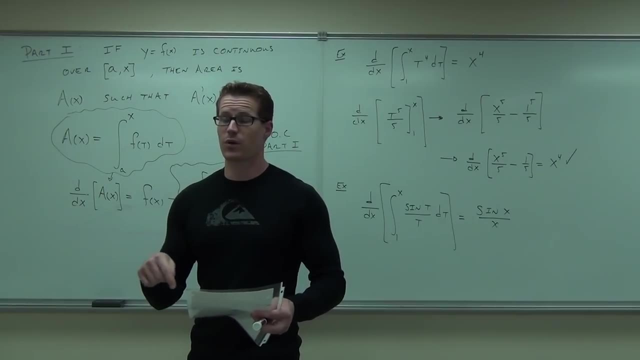 but this book ties it all together with this. We're going to continue doing definite integrals, only we're going to do some more, I guess tricky ones. They're not super tricky, but they're going to incorporate something you've already learned in this class. 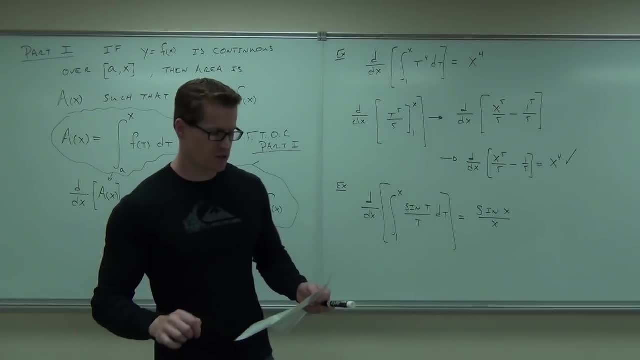 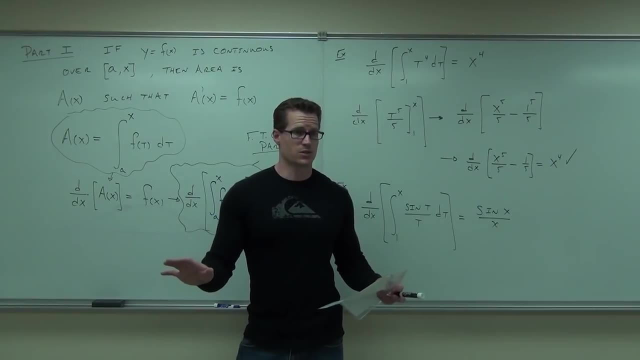 which I guess is kind of nice, but we haven't dealt with it yet. We're going to start talking about how to do definite integrals that might involve a substitution. You ready to learn how to do that? It's not hard. You've already learned substitution, right. 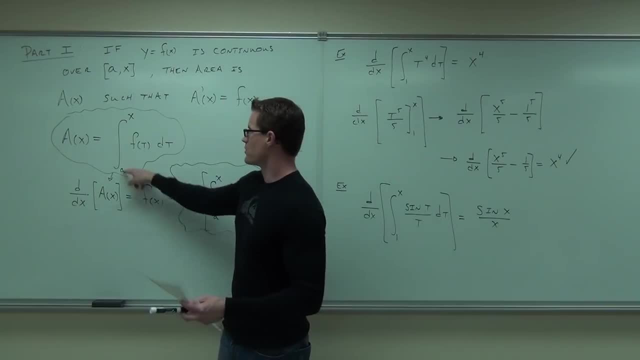 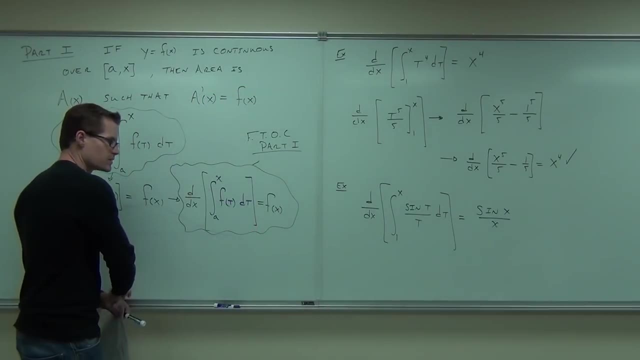 So if you've already learned substitution, I just have to tell you what to do with the bounds, The bounds of integration. after that, everything falls into place. So same idea: Let's look at how we deal with bounds, and that will be our the rest of our lesson. 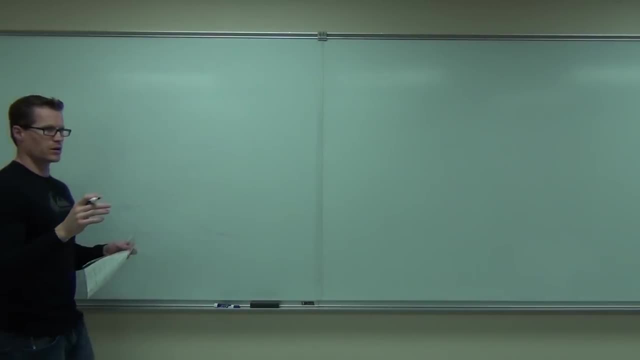 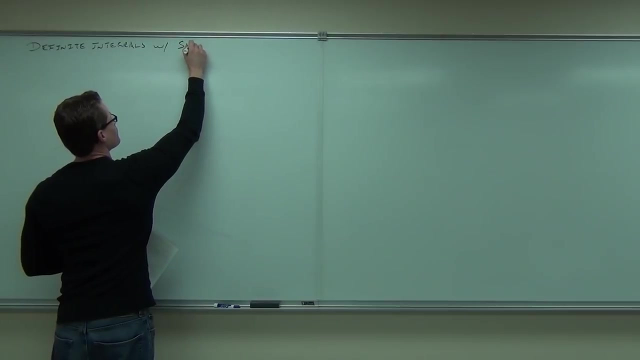 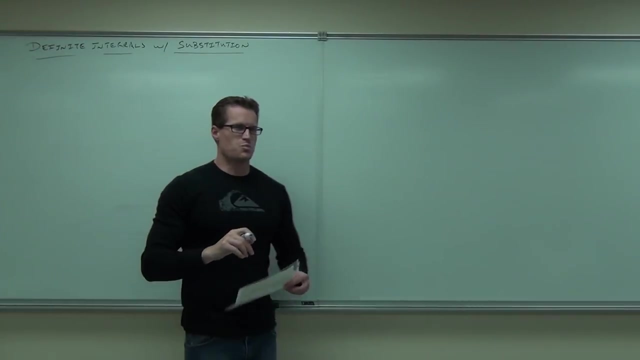 Okay, So, Oh, what are we on? We're still on 4.5.. It's still an extension of that, So we'll talk about definite integrals, But this time we might have some substitution. It's It's still in your best interest on your homework to check. 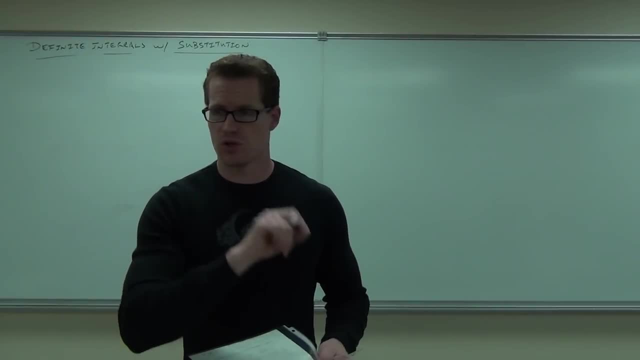 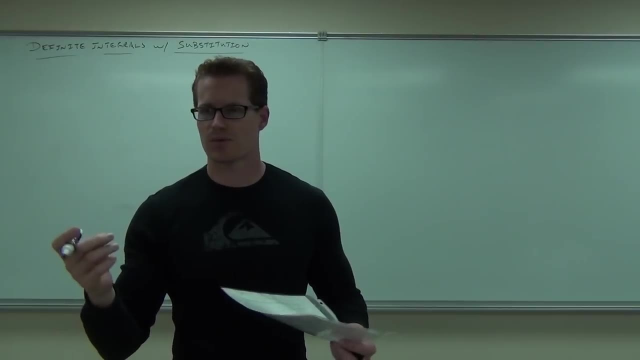 if you can do the integral without substitution, If it's just a simple distribution or a simple change. you know some exponents from square roots into one half, So I think we had one of those last time, right, And you combine them. that's probably easier than substitution. 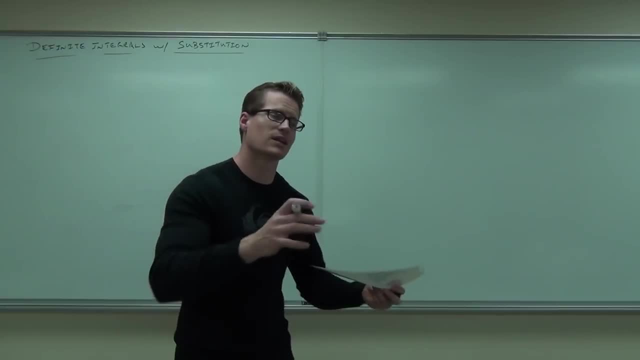 because substitution might even work in that case. But if you have to use a substitution, at least you know how to do it already. There's basically two methods. I'll show you method one first, and then I'll show you method two. 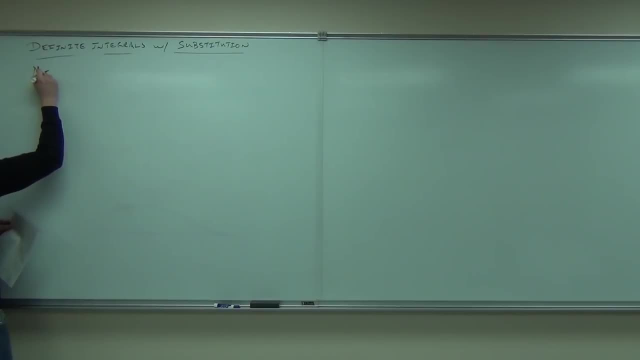 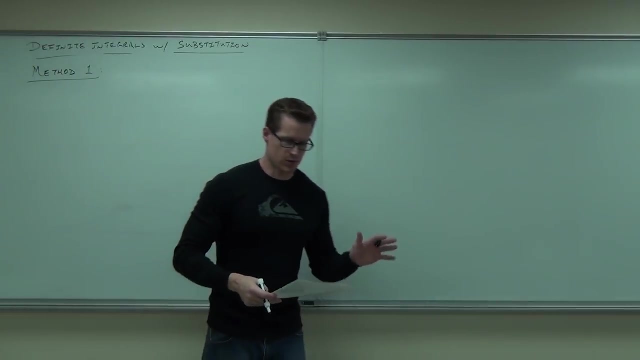 Method one says this. It says you're not going to change your bounds. You're going to do the same exact thing as before, but you're going to be sure to substitute back in for u before you evaluate. So method number one is: don't change bounds, sub in for u at the end. 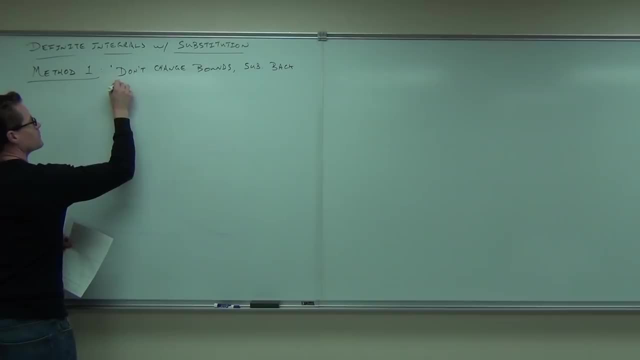 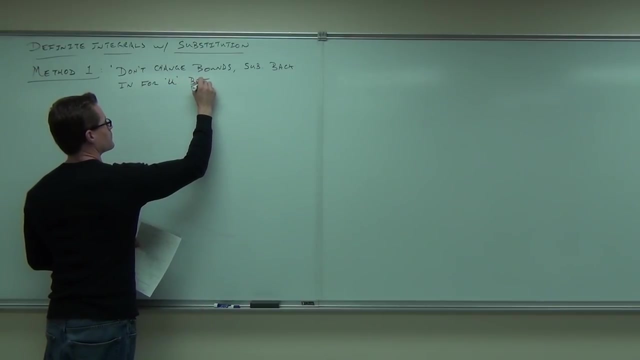 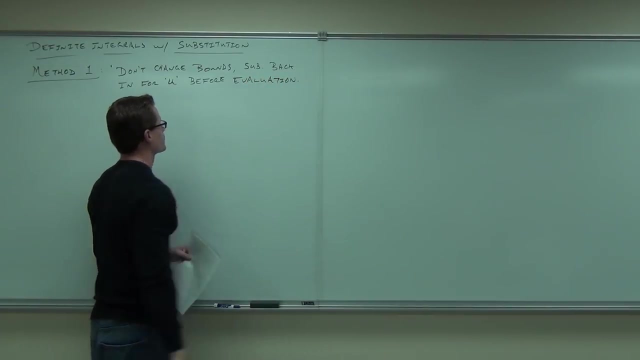 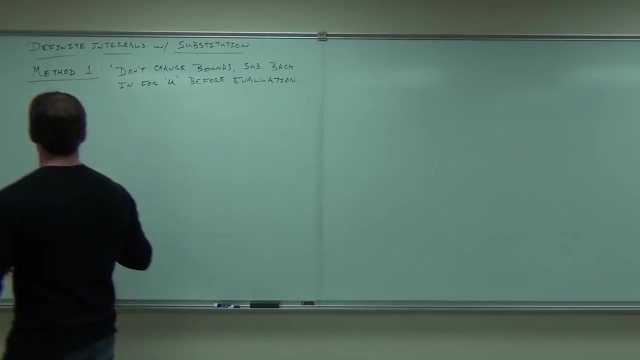 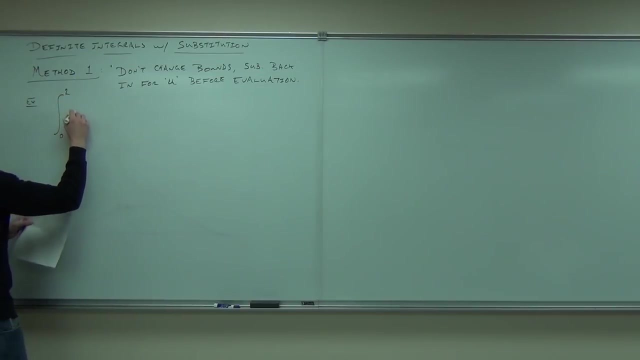 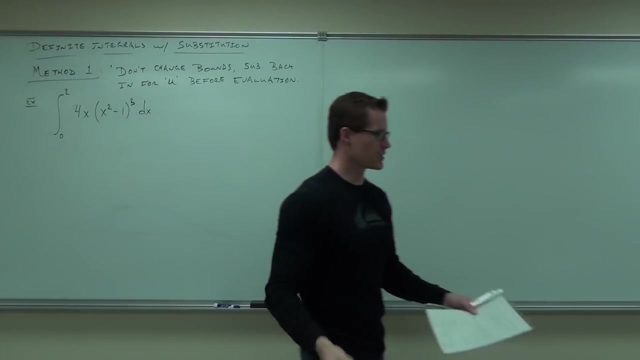 Don't change bounds. Substitute back in for u before you evaluate, And you'll see exactly what I mean on this example. There you go. Okay, let's look at the integral. This is the first time we've had like an honest to goodness integral with some numbers up there. 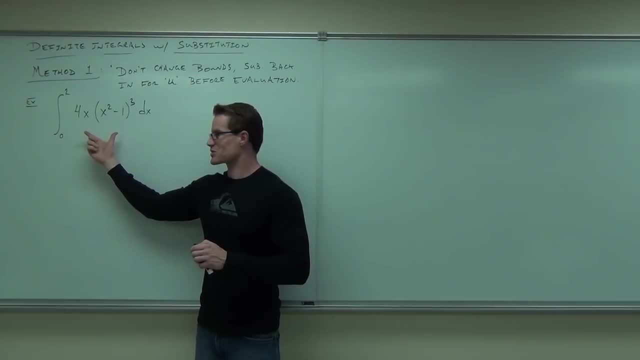 and something that wasn't just super, super basic, So this looks like a real integral, with some real numbers and some honest work to do. First thing: Could you distribute everything out? You could, You really could in this example. You probably wouldn't want to, though, because that's a power of three. 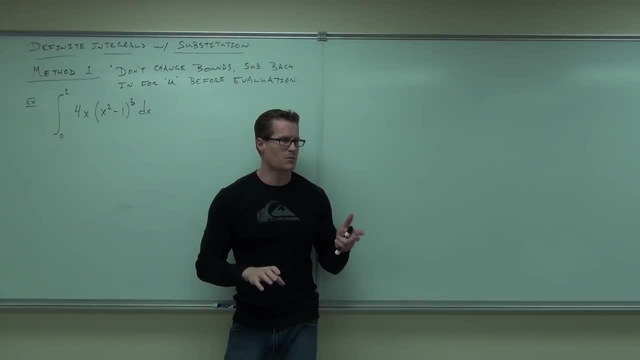 It's going to take you a long time, So substitution in this case would probably be your best bet. Ignore the bounds when you're picking your substitution. It's just a basic integral, just like you do with indefinite integrals. Pick the correct substitution. 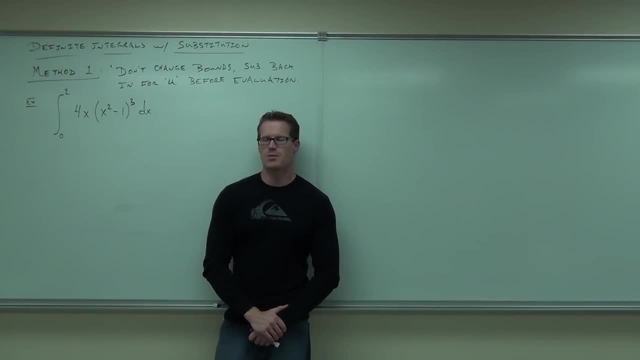 Why don't you do that now? At this point, I'm hoping that most of the substitutions are pretty obvious. The only times they might be, maybe wouldn't be, is with some of the square roots- Sometimes people forget about that- Or the trig functions. 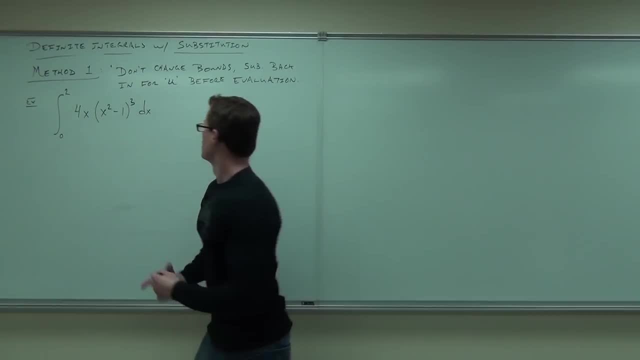 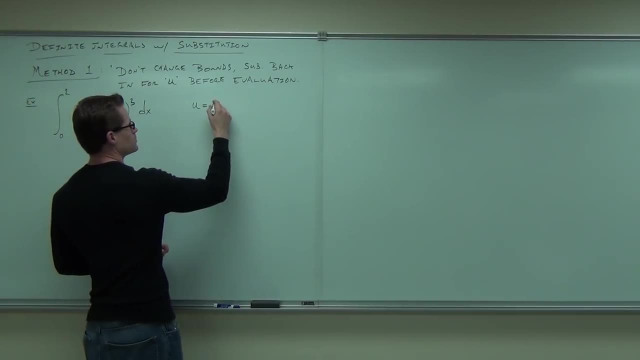 Sometimes they're not obvious. You have to guess and check. So u What's u? Good What's du? Don't forget the dx. You need the dx. And then how I've taught you how to do this is: I've had you solve for dx. 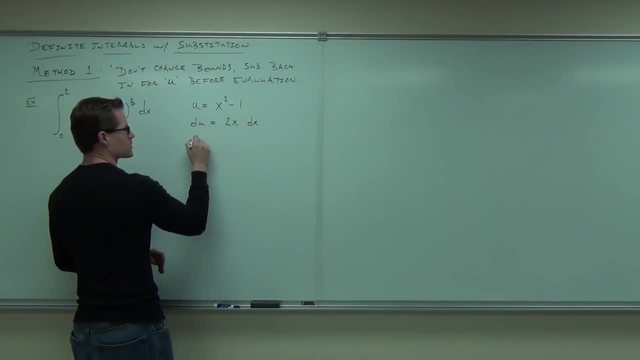 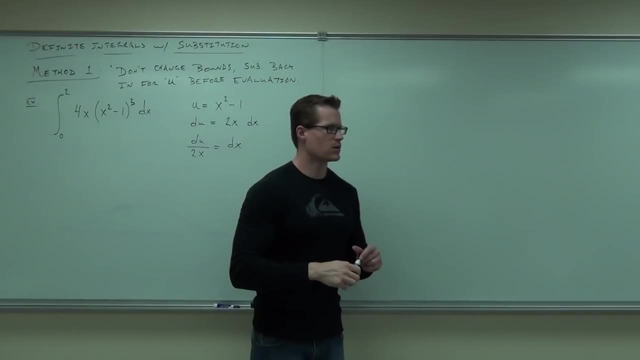 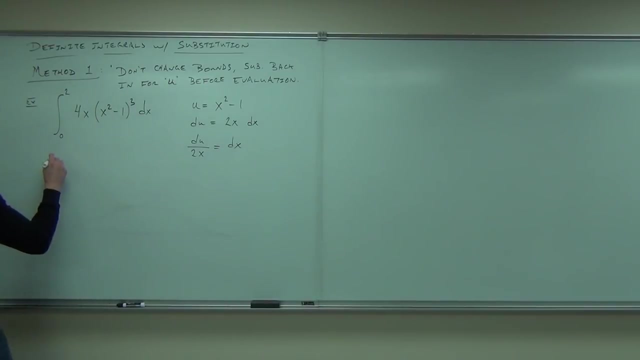 That makes a substitution nice and neat. So solve for dx. You're going to get du over 2x Equals dx. You okay with this. so far, Everybody Okay. Now what do we do? So we're going to have. what are we going to have? 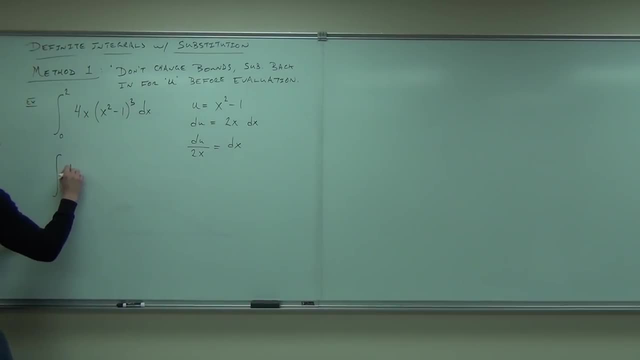 Why don't you tell me exactly 4x? u 2a- Okay, I heard 4x. What did you say after that: U 2. Perfect, And then what? And then du over 2x, Excellent. 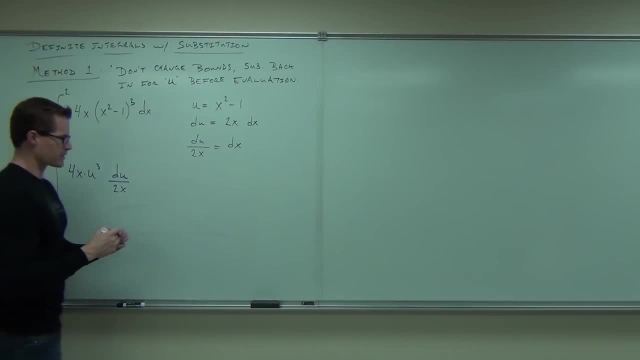 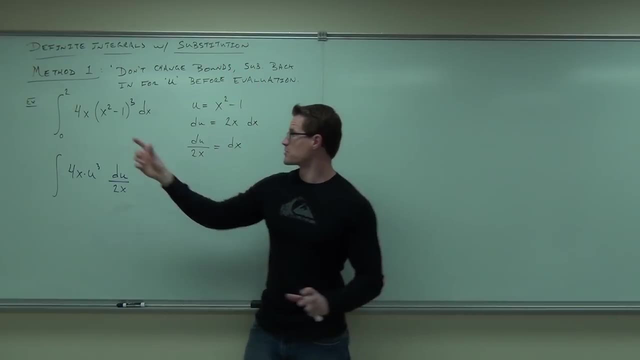 From 2 to 0.. Can we talk about that in a second? Firstly, how many of you feel okay with our substitution? 4x is still there. for right now, The? u cubed comes from u cubed dx. No, no, no. 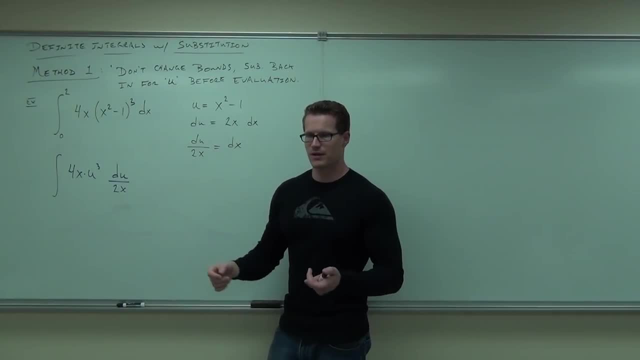 Not dx anymore, Du over 2x. And then we start simplifying things. And then Michael said something interesting: from 0 to 2.. Yes, and kind of no, Yes and no, We're going to put it there. But I want to show you why method 2 can do something different for you. 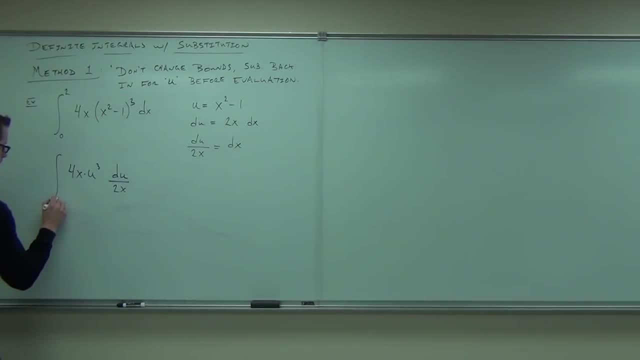 Because as soon as you do this, From 0 to 2.. As soon as you do that, from 0 to 2.. Look what's going to happen. Sure, you're going to eliminate this 2 and that's going to become a 2, yeah. 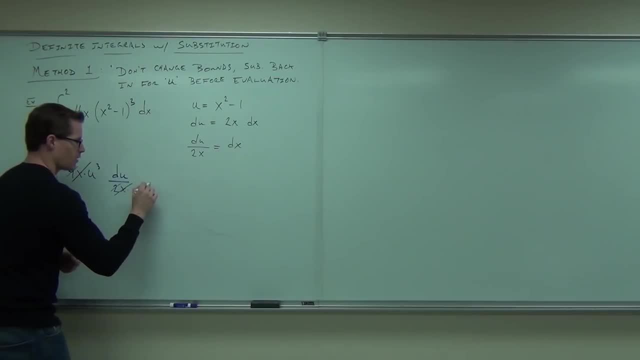 Mm-hmm, And you're going to eliminate this x and this x And what you would get is 0 to 2 with a 2 out in front of it. You see where the 2 out in front of it's coming from. 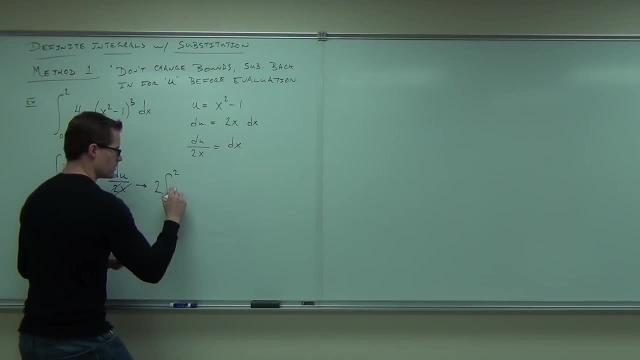 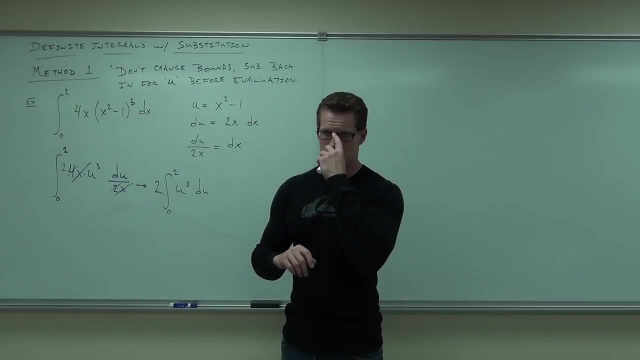 Mm-hmm, That 2 pull up front. You could use it. U cubed DU. which variable U? Which variable U U? Yes, it's U, not U U It's U. What were these bounds originally in? 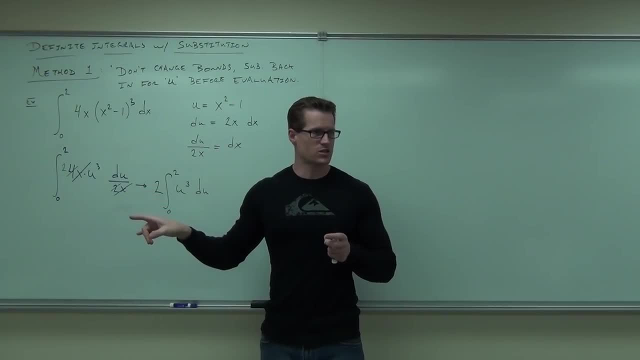 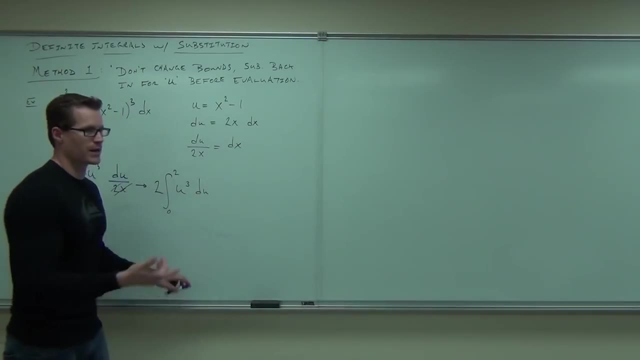 So we kind of have bounds that don't match our integral right now, which is sometimes leads to problems, because what people do often is: they'll do this, They'll go okay. hey, I know how to take an integral. It's very easy. 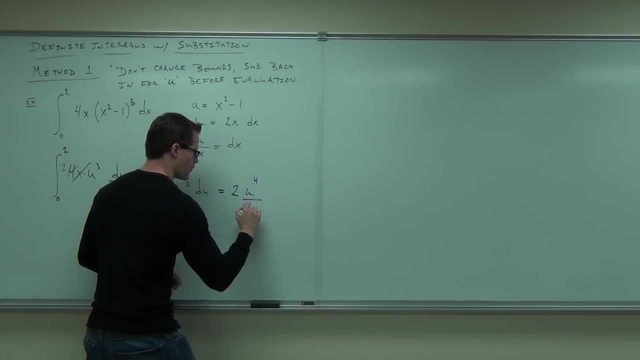 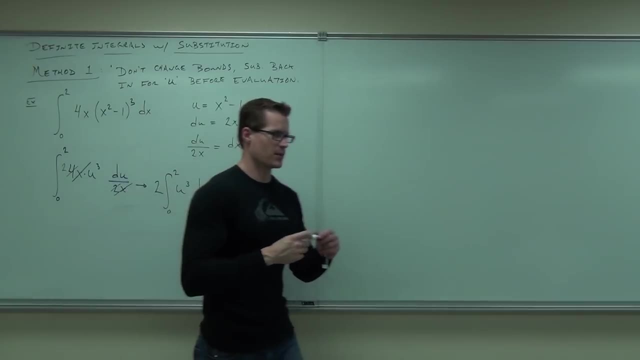 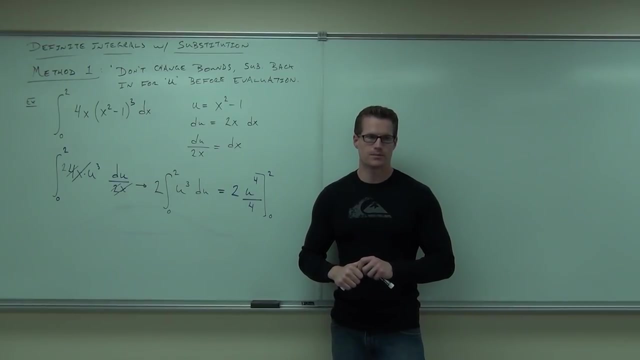 I'm going to have 2U to the 4th, over 4, and then they do this. Explain to me why that might be incorrect. Right, These are in terms of X, right, But the integral makes it seem like you're plugging them in for U. 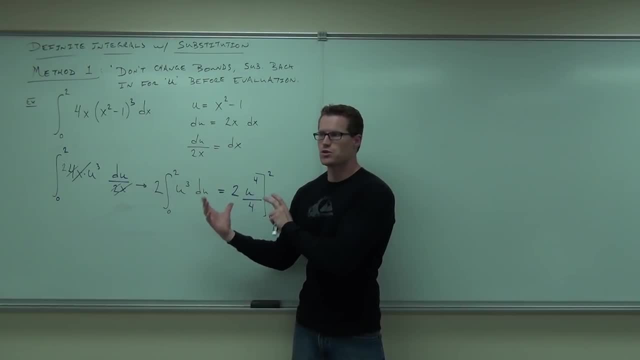 Now you can do it this way. You can, You really can, provided that you do one thing. provided that you do this, You're going to substitute back in for U Don't change the bounds. We didn't change the bounds. 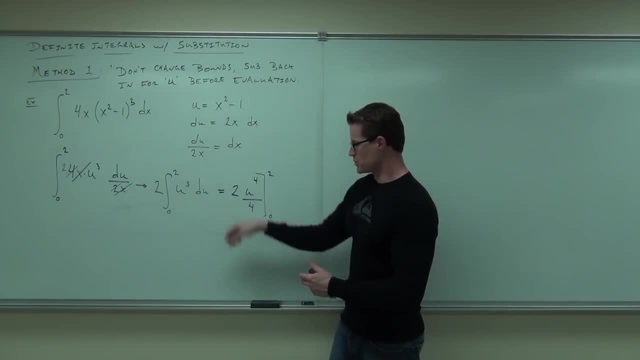 And substitute back in for U before evaluating. so not here. This would be the wrong way to go. Do you see why it's the wrong way to go? Honestly, do you see it? You're trying to plug in X's for U's. 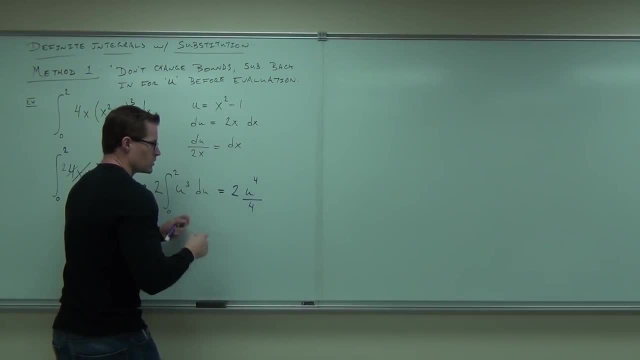 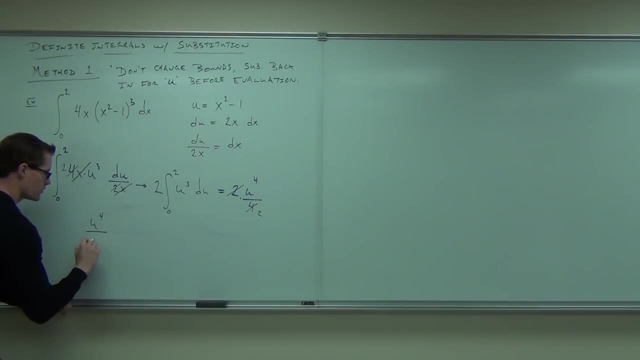 That's not going to happen. So instead we're going to do a little bit of simplification. still, We're going to get U to the 4th over 2, and you all said that you're going to substitute back in for U. 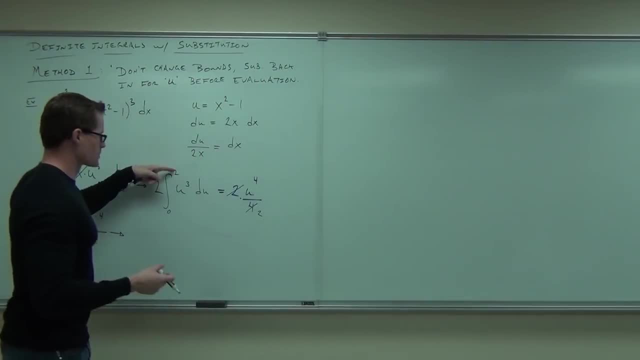 In terms of X before you plug this in. You see, if these are in terms of X, I want my function to be in terms of X, my integral to be in terms of X, what I got to be in terms of X before I evaluate. 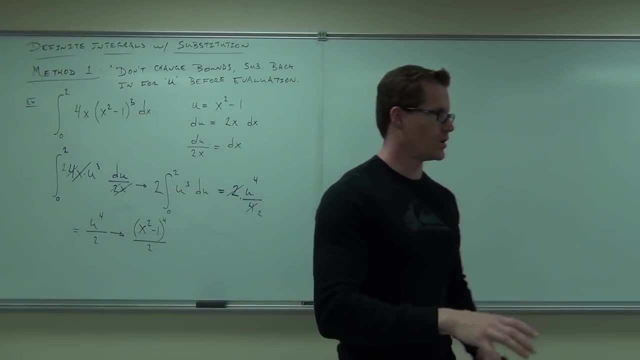 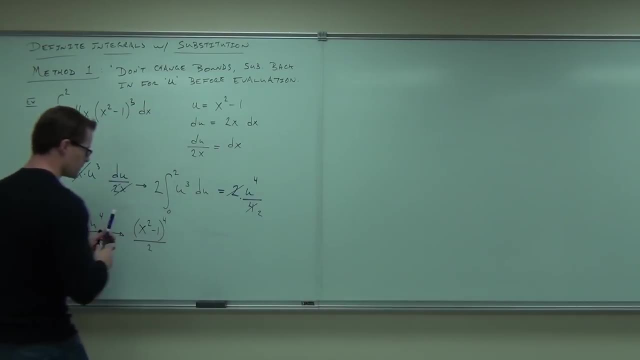 So we'll substitute back in for the U, We'll get our X to the 2nd minus 1, all to the 4th, power then over 2, and at this point this is where I should evaluate. So right here, all right, let's get a little bit of craft up there. 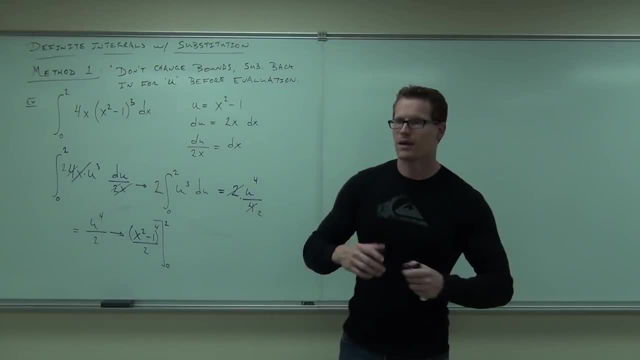 Now we get to go from 0 to 2.. That's okay. That says, now that we have this in terms of X- great, They match up with our X bounds that we started with. Now plug in the 2,, plug in the 0.. 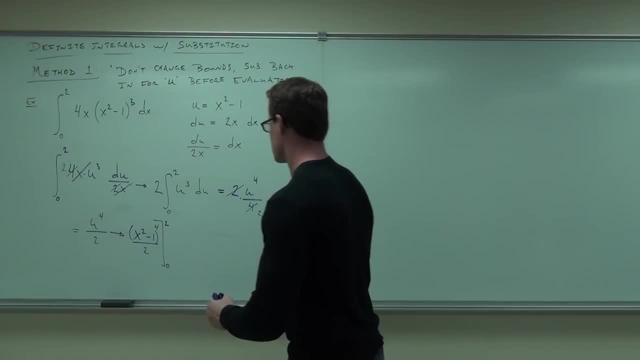 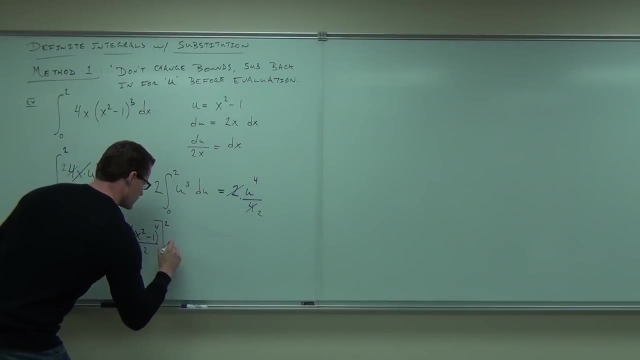 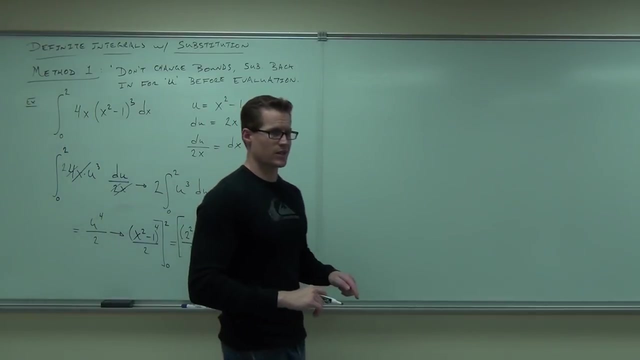 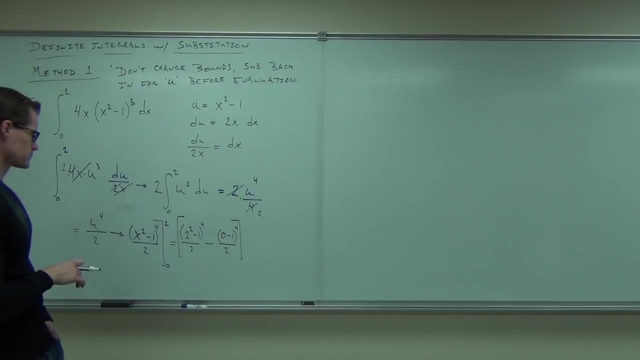 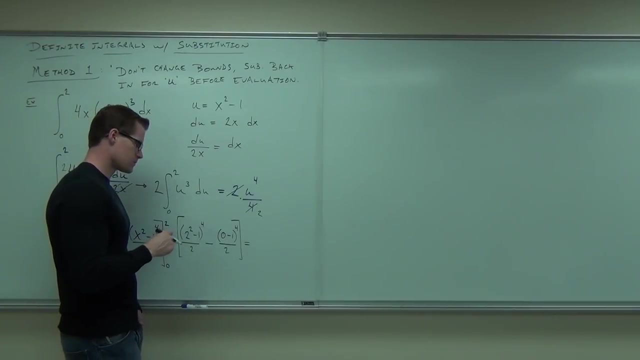 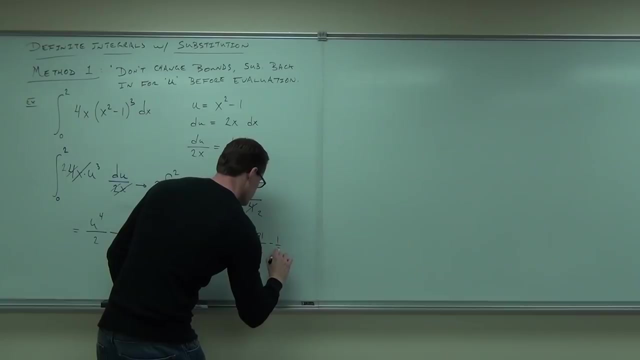 Why don't you do that and see what you get? Don't neglect that 0.. 0 squared minus 1 isn't 0, so you're going to get something over there. All right, I got that. Did you get that? 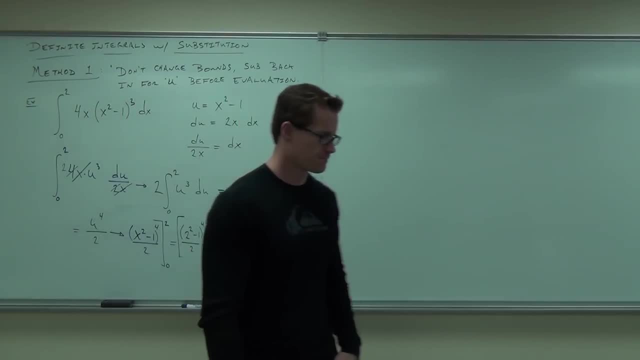 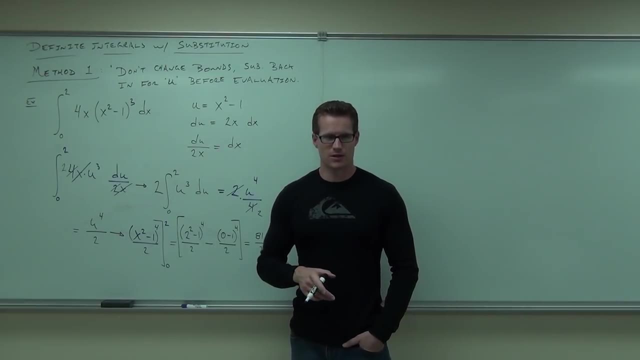 Mm-hmm. Cool. Okay, What's it mean? It's an area, It's an area. What type of an area? Is it total area or net signed area? Net signed- Good, We haven't talked about absolute value or anything. 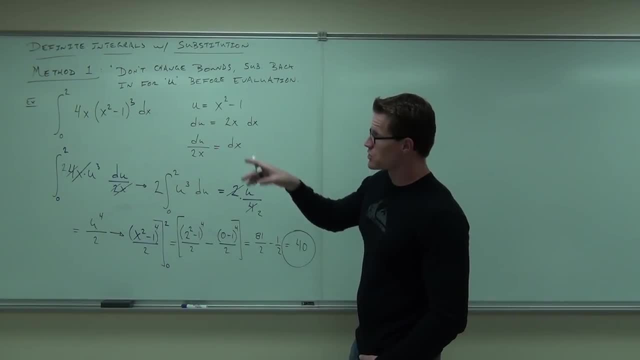 I'm not sure if that one's going to have any negative area. If you graphed on a graphic calculator, you can tell. Or if you wanted to find out total area, what you would have to do is find out whether that's above or below the X axis. for all of those points, 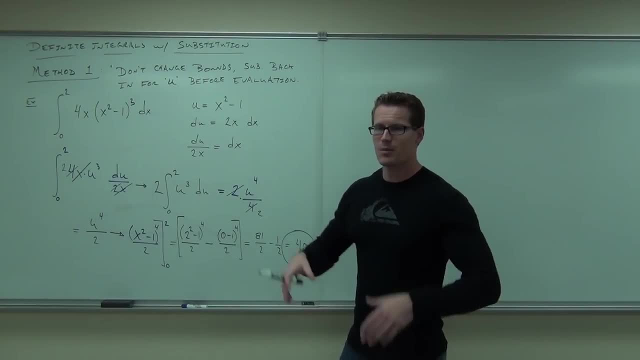 I'm not sure. in either case, Maybe you can look at that, But you'd have the absolute value for total area. You remember doing that from last time. The absolute value, you'd take this, you'd set it equal to 0.. 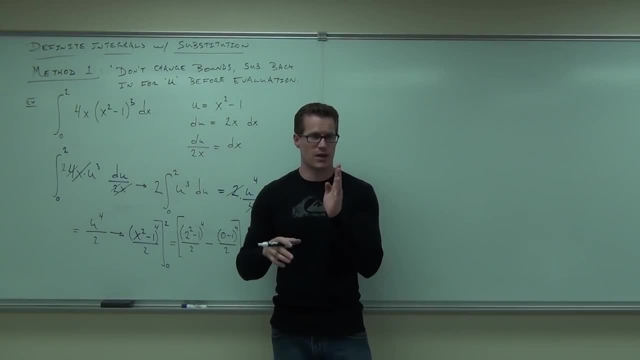 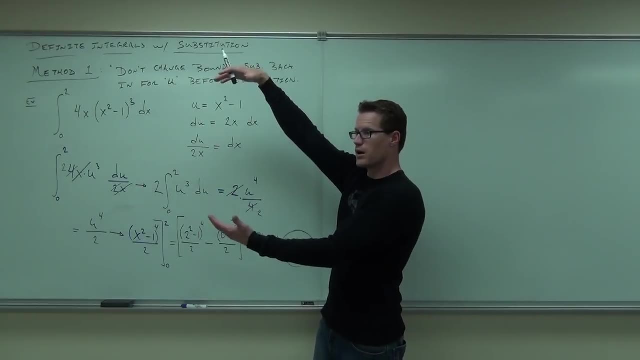 You'd have your end points and any points in between there. that would change the sign of that thing and you'd separate those two angles And that's how you do that problem. So this actually is net signed area, whether or not we have it all above or below. 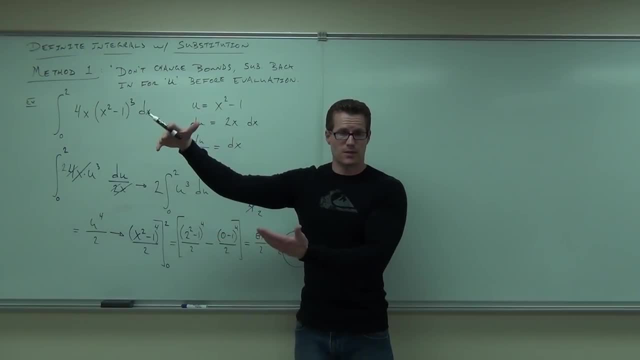 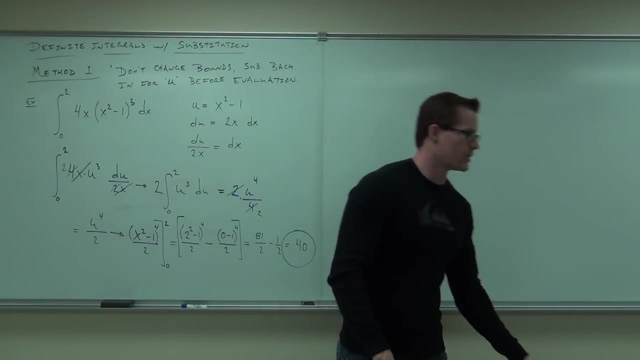 And if it was all above the X axis, net signed area would be total area, But if there's any area below the X axis, it would have automatically subtracted enough for us. So that's the case. By the way, has anyone graphed that? 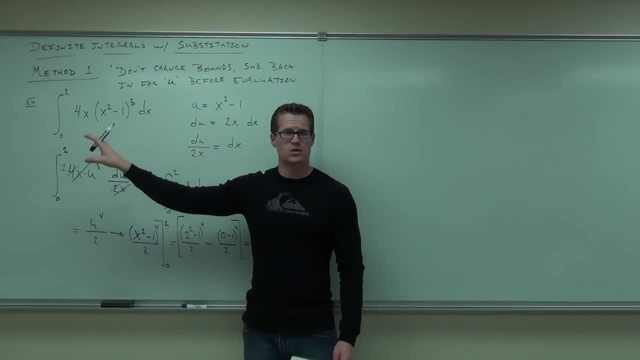 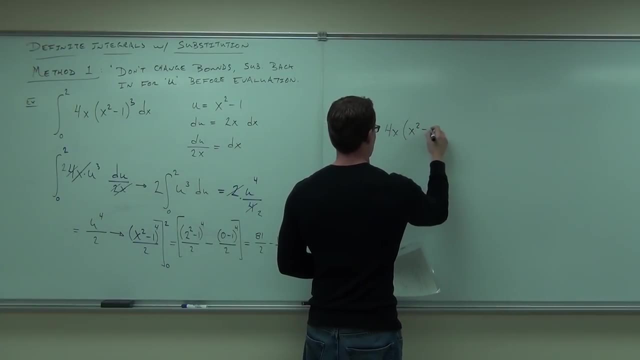 Do you know if there is any area below the X axis between 0 and 2?? I guess we could find out real quick Between 0 and 2,. yes, there is. Yeah, there is Between 0 and 1, it looks like. 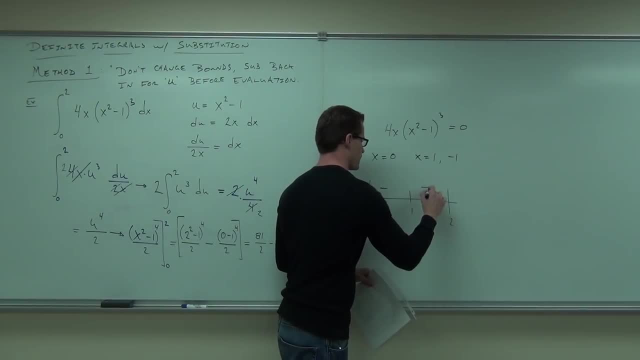 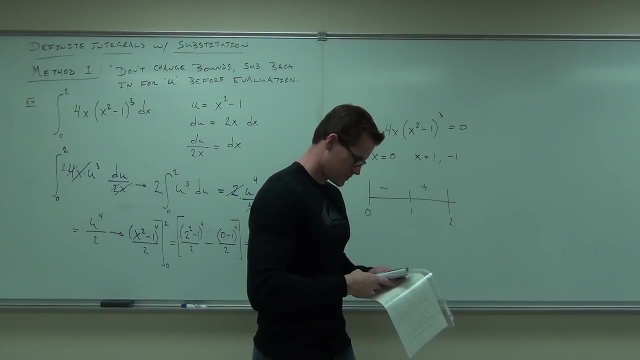 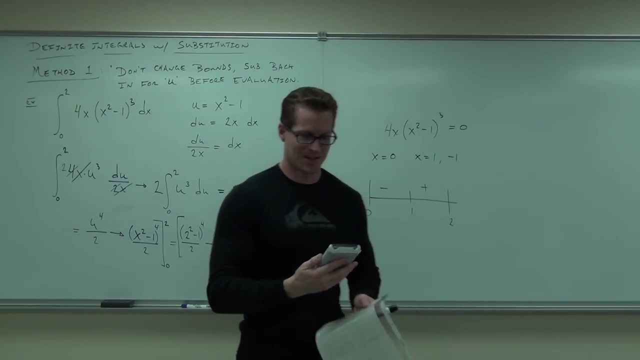 This is negative. Yeah, Okay. So it looks like I mean, there's a little portion Like that, Just a little bit, on the side of 0, it looks like, Well See, You can see, Yeah, we have a little bit below the X axis. 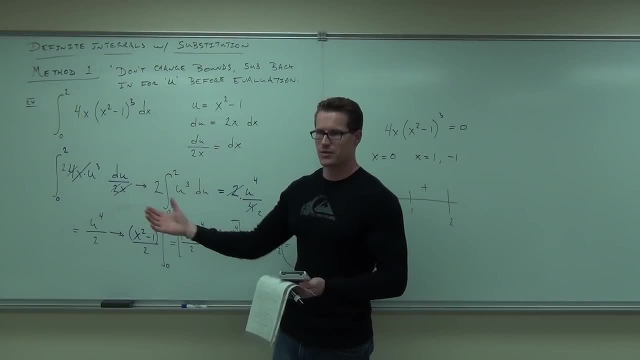 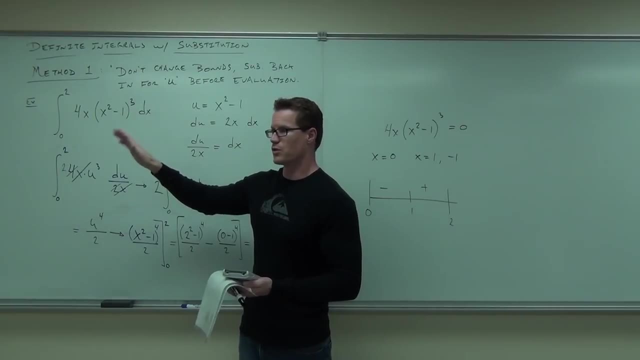 Between 0 and 2.. So that's going to be counted against our area right here. So this is actually total, not total area. This is net signed area. It's discounting the part between 0 and 1. And then we have from 1 to 2. that would actually be positive. 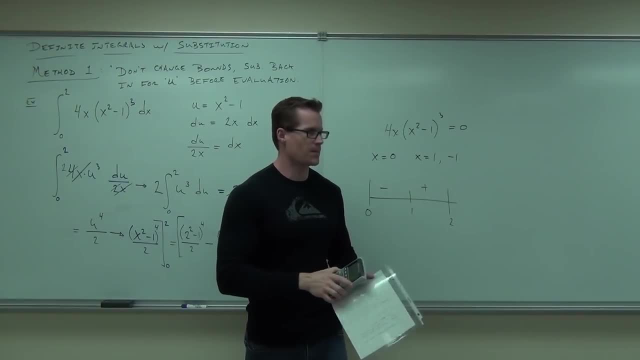 But it's greater than the negative area. That's why we have a positive 40 out of that. I mean we'll be okay with that so far. All right, cool. Would it be substantially harder to do that? Substantially harder to break them up? 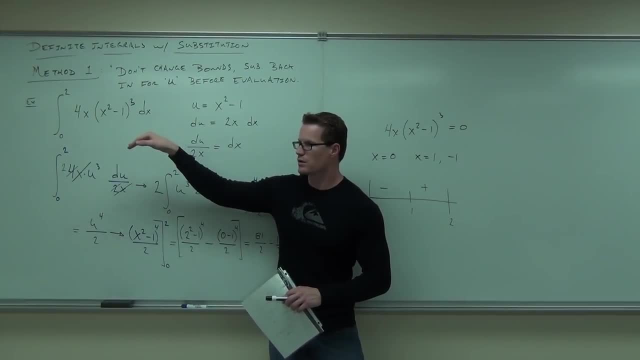 Not really. It's actually just a matter of separating them. We're going from 0 to 1 and having a negative in front of that, and then going from 1 to 2 and doing it just like we just did. We just plug in some different numbers. 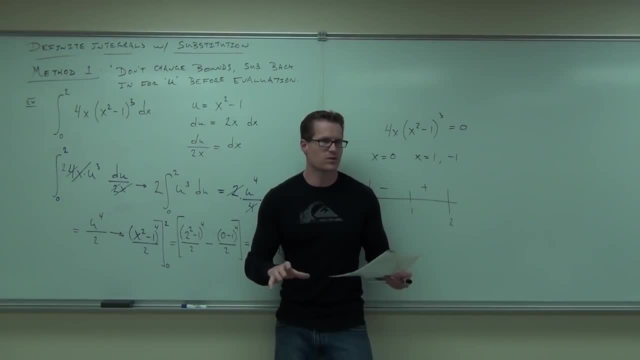 So it's not that much harder. You just have to do the integral twice. So I don't want to do that right here because we'd have to change bounds a lot in the next example. but that would be something to talk about. Are you okay with this first example? 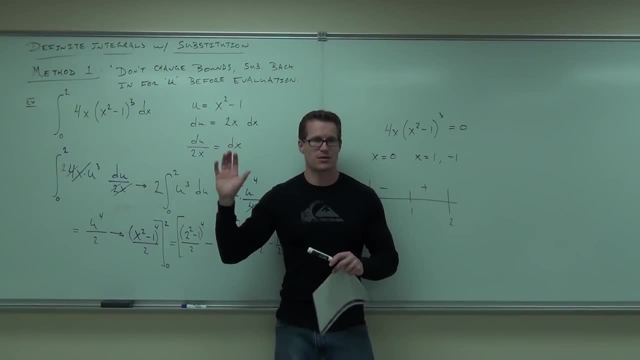 Do you understand the idea of not changing bounds? Basically the same exact thing you do for every example. You just don't change the bounds. You do the integral, like you normally would, change it back into x, like you normally would, and then plug the numbers in. 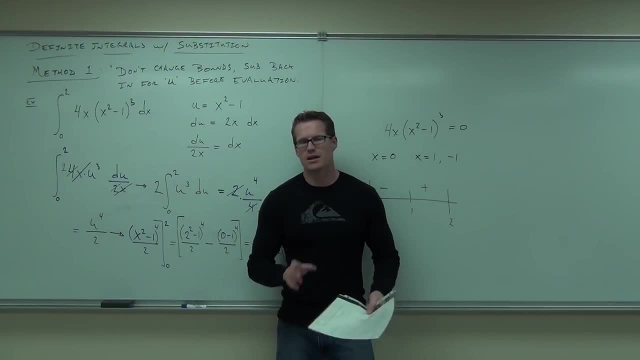 That's the first method. Second method says: well, maybe not necessarily a quicker way, It's not quicker, Maybe we can just do it a different way. In either way, notice that you're going to be plugging these numbers in. 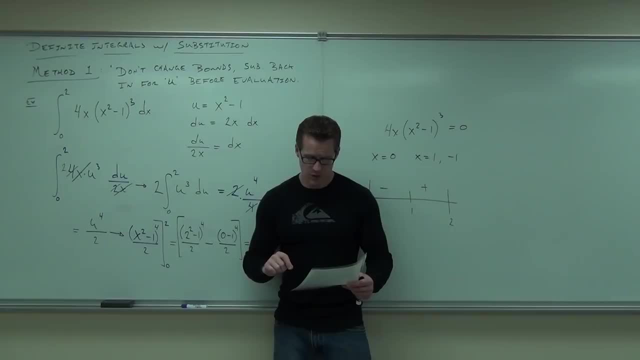 You will be plugging in 0 and you will be plugging in 2.. You should do it at a different time. So we're going to talk about method 2.. I'll show you how that works. I'll tell you which method to use on the test. 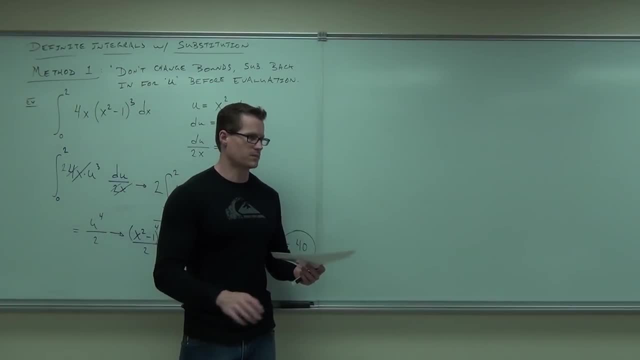 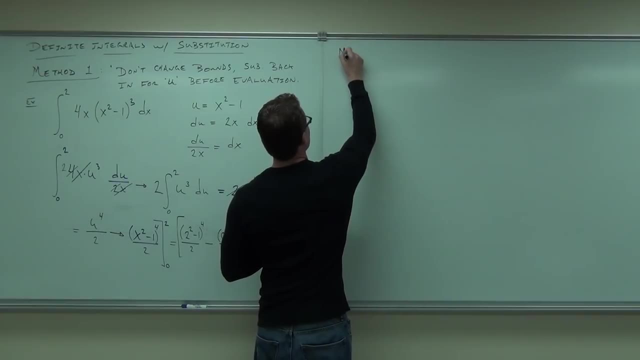 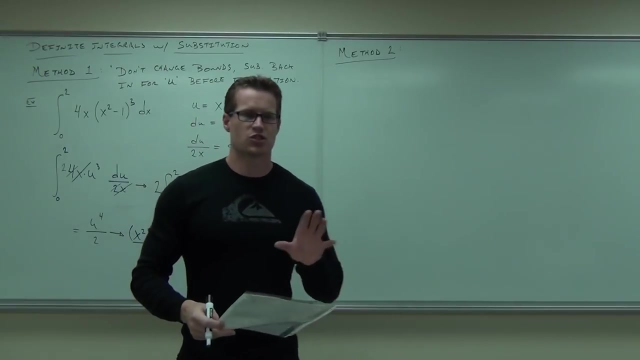 When I want you to use it. If I don't tell you a method, you do whatever method you want. Okay, So we should learn both methods. You must learn both methods. yeah, Okay, method 2.. Method 2 is: you change bounds. 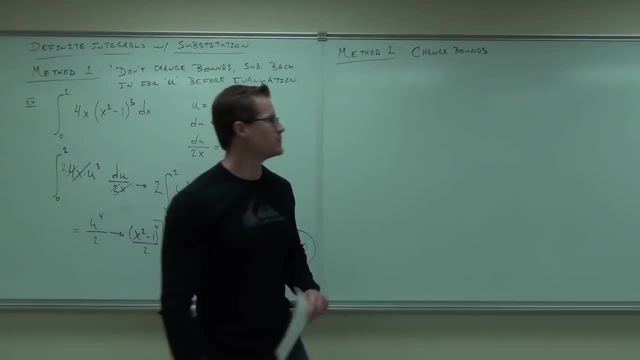 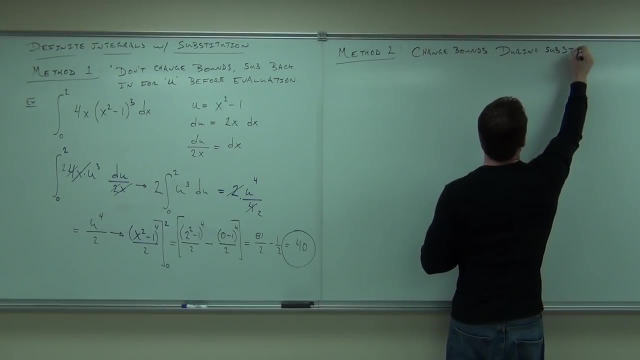 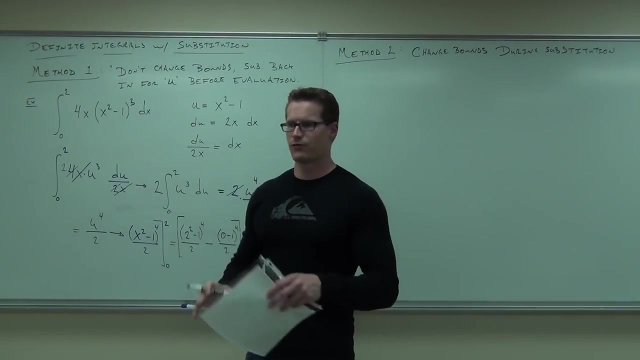 You change bounds during your first substitution. If that's the case, I'll give you like a little foreshadowing of what's going to happen. You're going to change your bounds from x's into terms of u using your substitution. 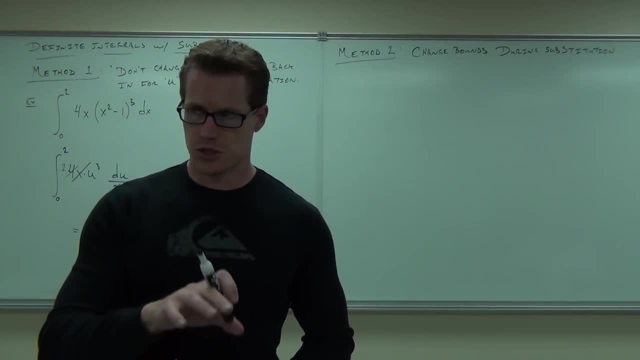 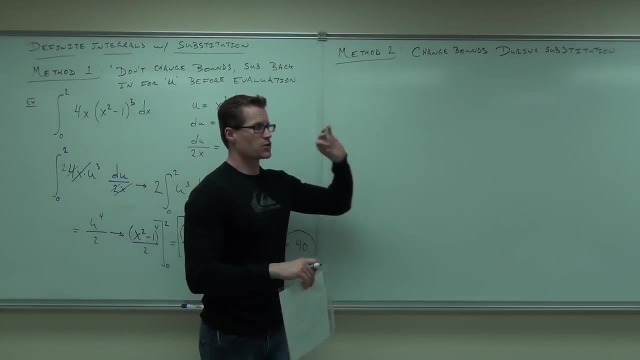 If you change your bounds into terms of u, do you need to substitute back in at this point for x? No, because they'll be in terms of u. So if you do that, you're going to have to substitute back in. So if you do method 2, you change your bounds and then you do not substitute back in. before evaluation: 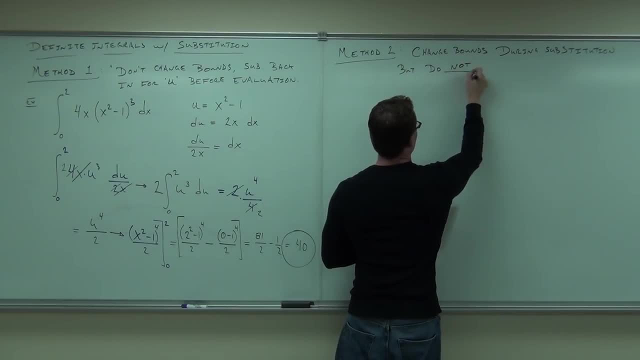 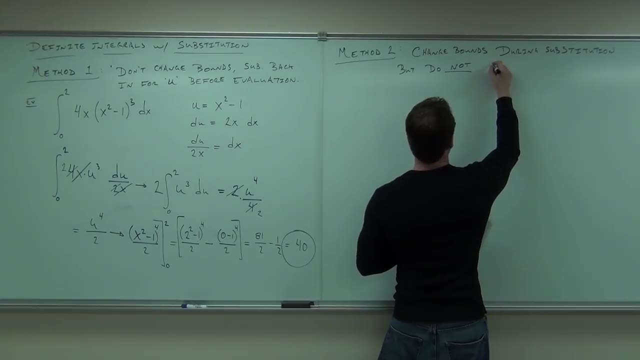 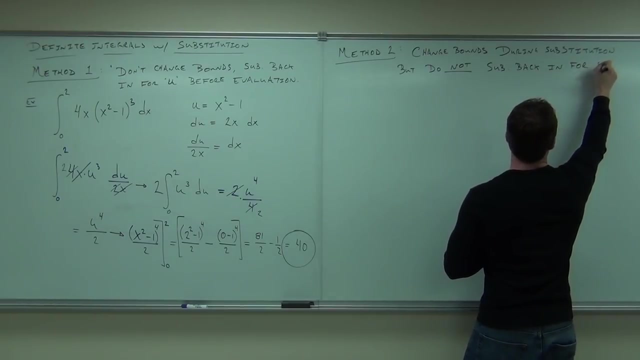 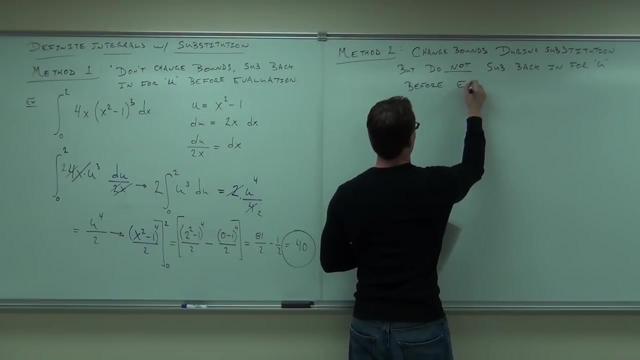 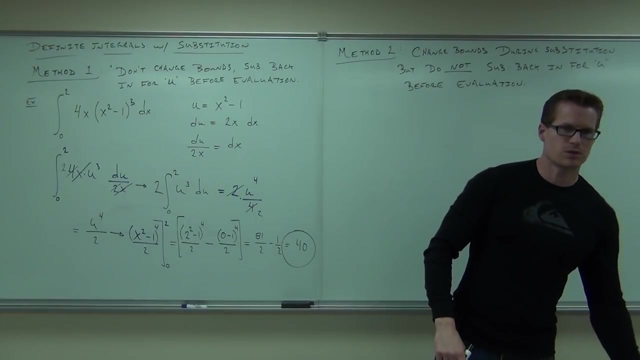 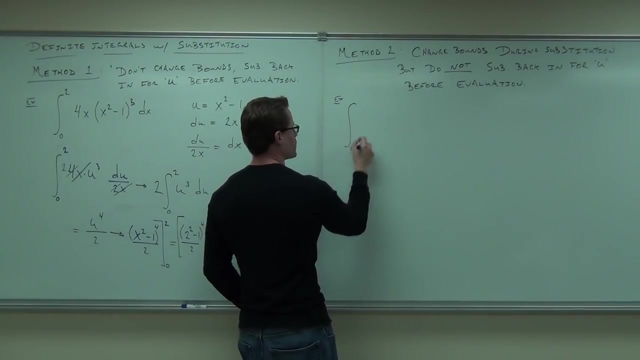 It's the same. It's. you Tell you what let's do. the same example. Can we do the same example, just do it a different way? So you see I'm not full of smoke here. It really does work out. 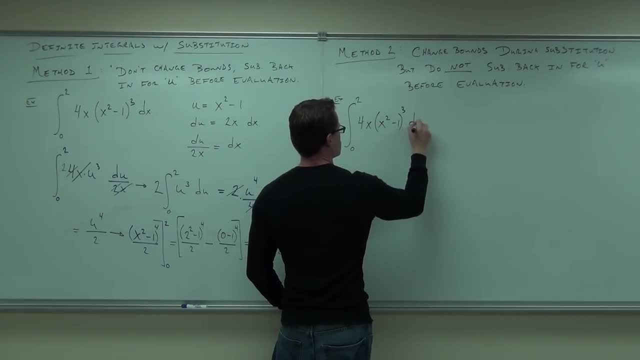 I'm not here to reteach you how to do substitution. I've already taught you everything that you need to know about substitution, that you need to know. that doesn't change, so that's nice. You can still use the same substitutions, no matter what. 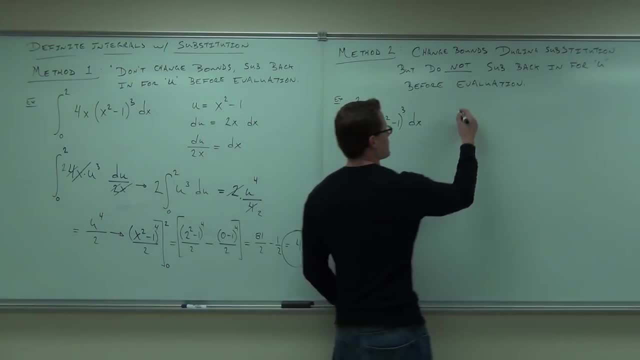 What I'm here to tell you is there's a slightly different way to do it. So if we pick the same substitution, u? u is still x squared minus 1, and, hey, du is still 2x dx. and sure enough, du over 2x is still going to equal dx. 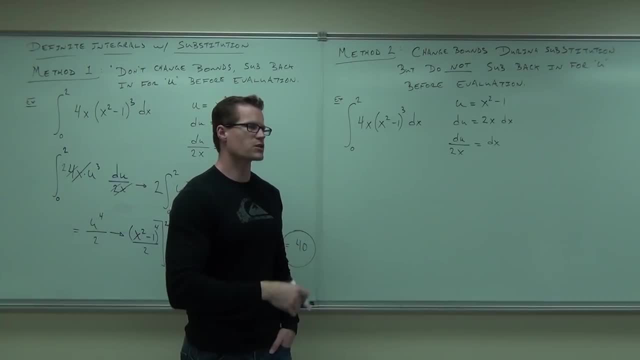 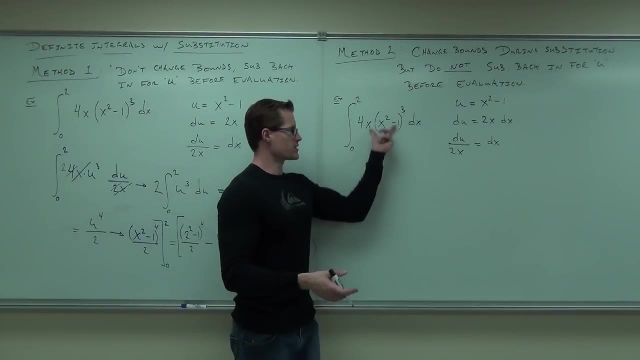 That doesn't change at all. You still okay with that? Here's the change. The change says: well, since we're substituting everything anyway, I mean we're substituting this for u, this x part for u and this x part for u. 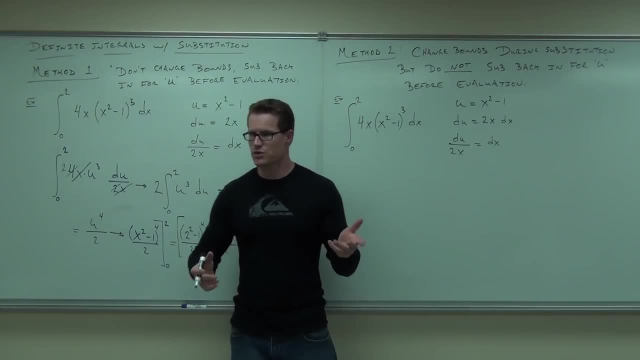 why not just do the bounds as well? Why don't we substitute those things for u as well? And here's how to do it. All right. well, that's a good idea, Mr Leonard. Let's try, Boy. here's the point. 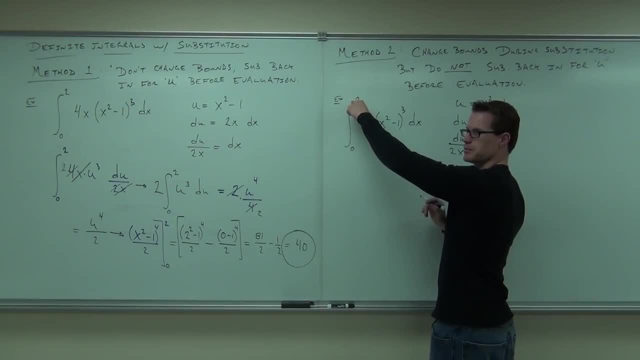 When you look at that, that says x is going to become 2.. That says x is going to become 0. Why? Why don't you find out what u would be when x becomes 2 and u becomes 0?? And that's the question. 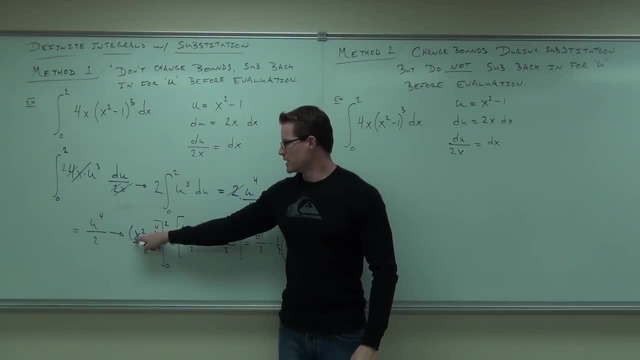 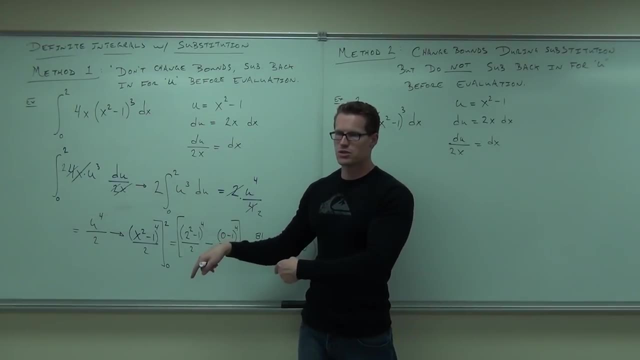 Notice how we're actually doing that right here. We're plugging in 2, 2.. We're plugging in 0, 0.. It's just within the evaluation process Here. you just do it beforehand so that when you get your bounds it's in terms of u. 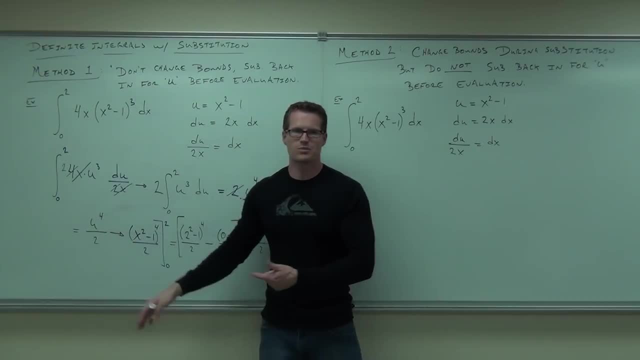 so you don't have to do this step, You just go directly from here. It's basically: do you want to do the work beforehand or do you want to do the work after? It doesn't matter, You can do the work either way. 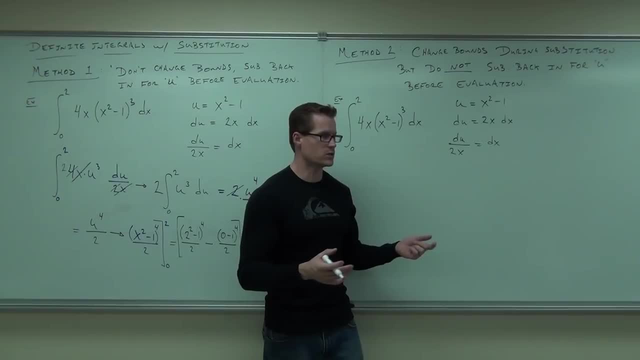 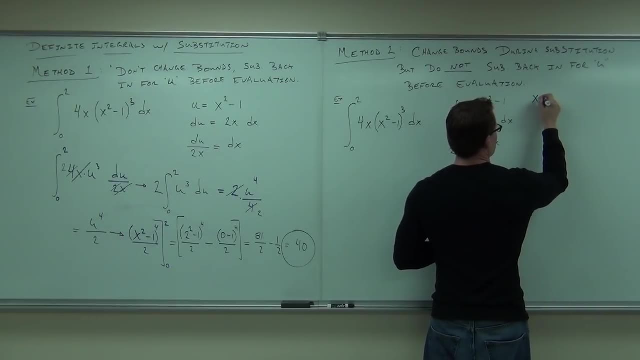 So it's really up to you. Now I'm going to make it a little bold. I'm going to tell you what to do, but it's an option for you. You got it Okay. So we'll say: if x equals 2 and if x equals 0, this is the whole process of changing bounds. 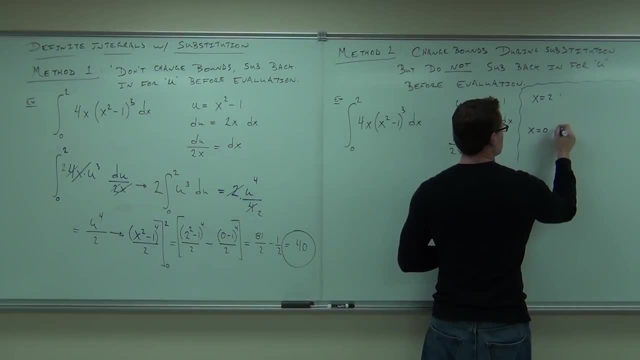 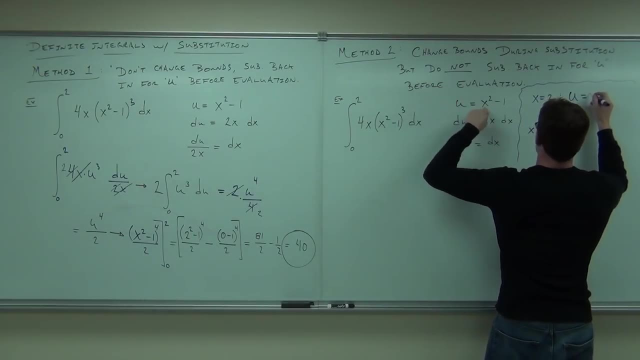 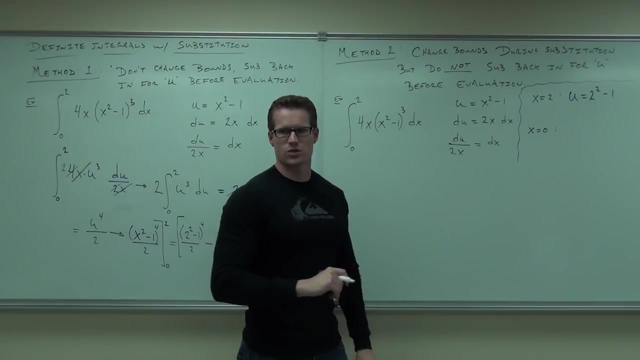 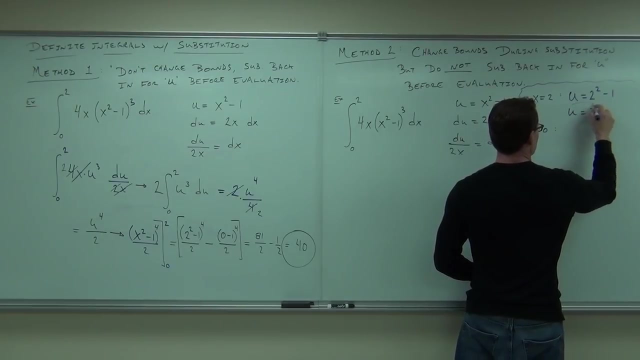 Let's do this: If x equals 2, then u equals 2 squared minus 1.. See where the 2 is coming from right, And u is going to equal what 4 root. Okay, If x equals 0, u equals 0 squared minus 1.. 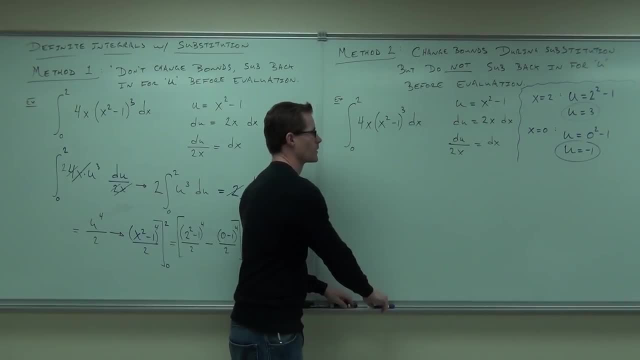 Very good. Well, now we can make a substitution with everything, and the bounds will match this. So we're going to use the variable, which is nice. So let's do it. Do we still have the 4x? Of course, 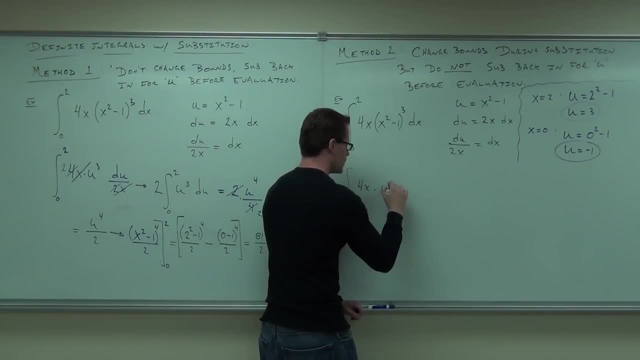 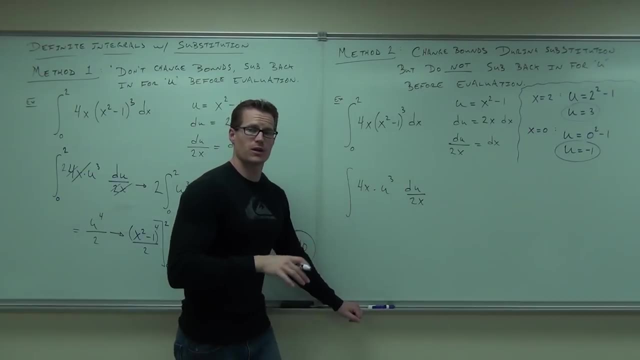 Do we still have x squared minus 1?? Of course not. That was our. u Notice how it's going to look. exactly the same as the previous problem: du over 2x. The only thing that's going to be different is what. 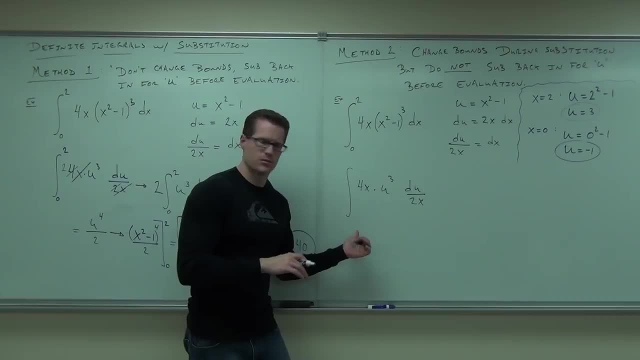 Our balance. What is the? what did the 0 become? The 0 became 1.. What did the 2 become 3.. It's going to be done the same What It's going to be done the same way. 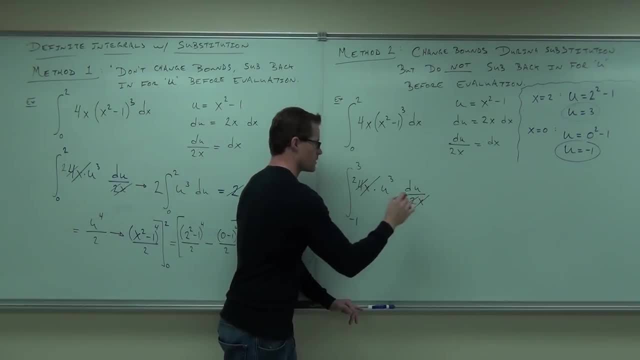 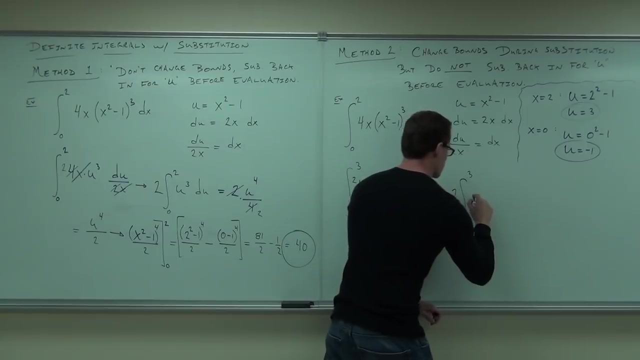 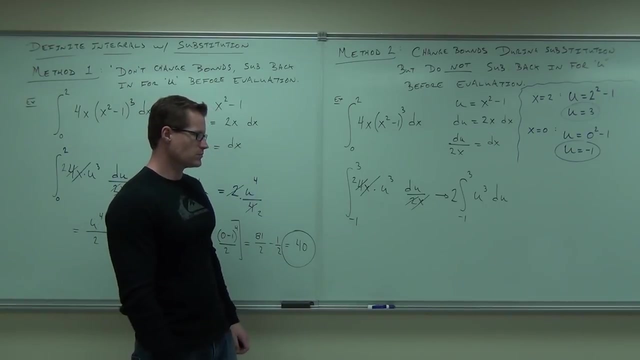 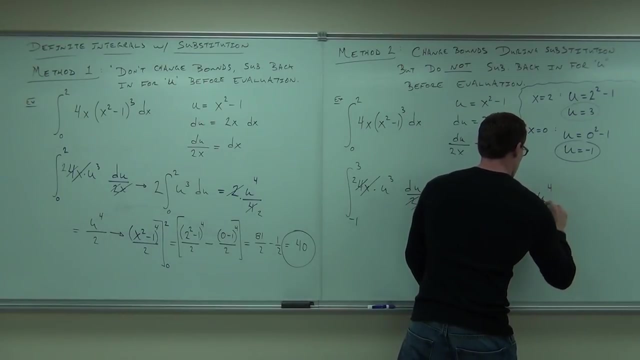 2 is gone, x is gone, So negative 1 to 3 will still pull the 2 outside. u to the third: du Hey, we can do the integral the same way. We're going to get 2.. u to the fourth over 4, and we'll simplify that. 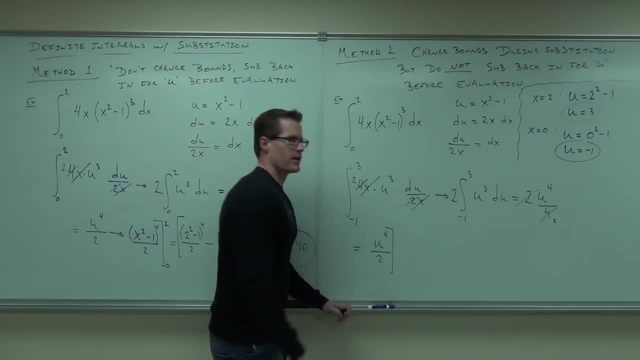 u to the fourth over 2.. But now, when I do my evaluation, do I have to substitute back in for the u? No, because we did our bounds And that's the only reason why we had to here, because the bounds were in terms of x. 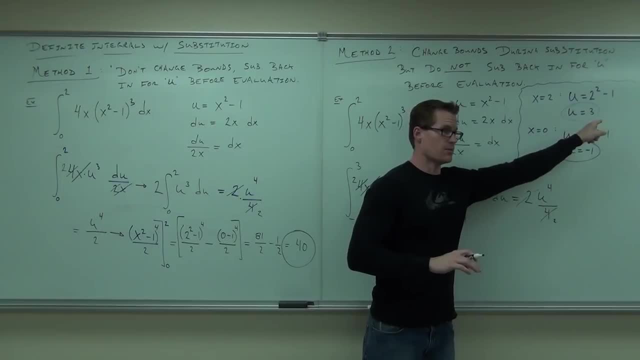 Here you've already, You've changed them, You've taken x's and you made u's out of them. Once you make u's out of them, you can u's it right here. Get it, You can u's it here. 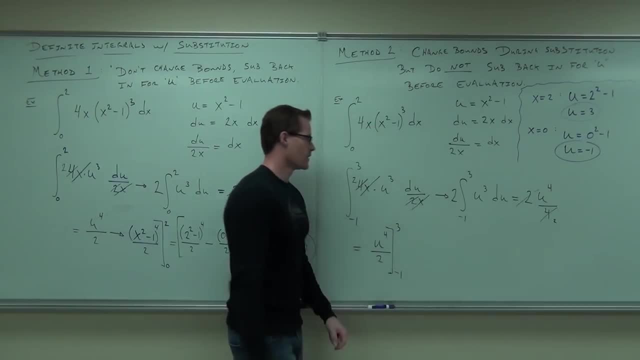 Negative 1 to 3. Because those are in terms of u Plug them in, you're going to get the same answer. So let's try that. Hopefully you get the same answer. It makes it so your evaluation is just a little bit simpler. 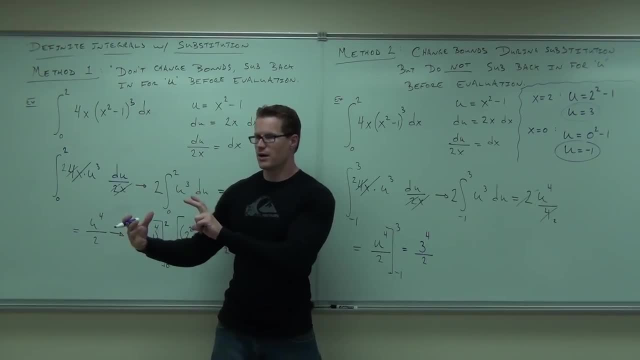 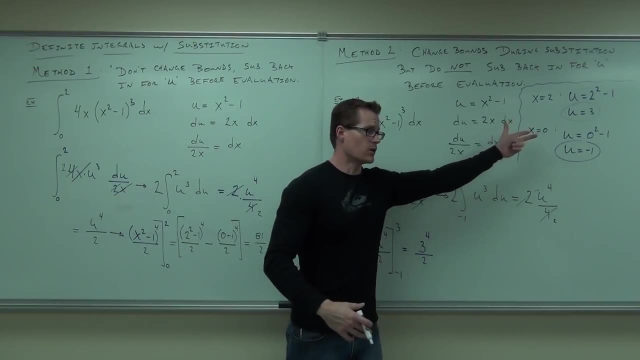 By the way, because you typically, because you have this function's gone right now, You don't have to plug that in and then do all the math. Basically, you just do it ahead of time. You're still doing it though, You're still doing it. 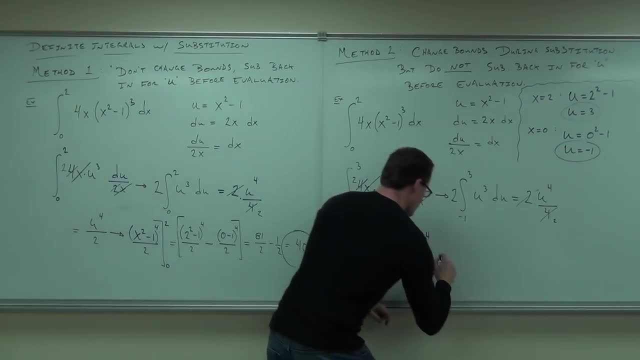 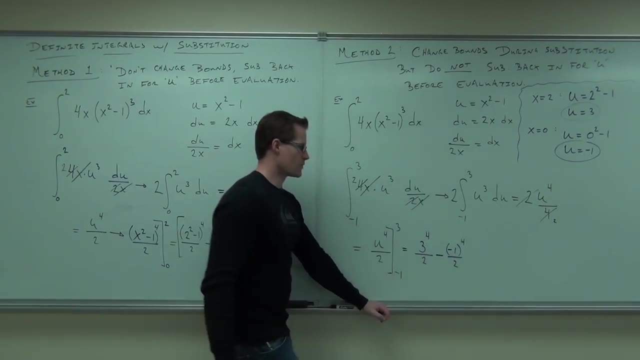 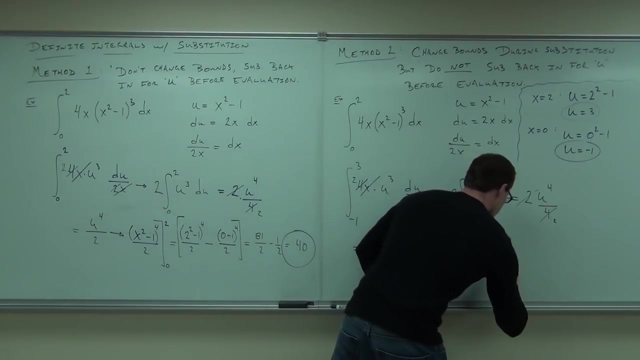 It just kind of set aside for you up here, which I suppose is nice: Minus negative, 1 to the fourth over 2.. Well, what that's going to be is 81 over 2 minus 1 half, And again that's 40.. 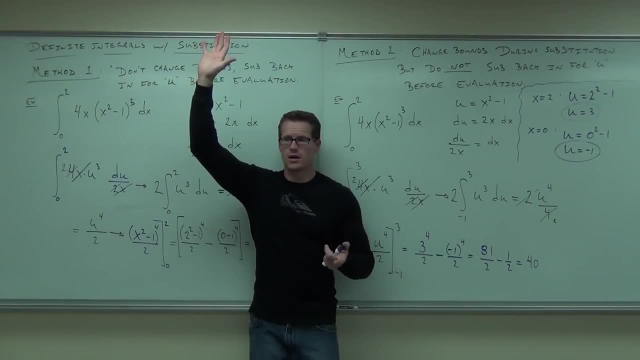 Show of hands. how many people feel okay about the both methods? How many people prefer method 1? Method 1.. Okay, that's cool, You can, It's fine. How many people prefer method 2?? People seem to like that a little bit better, for some reason. 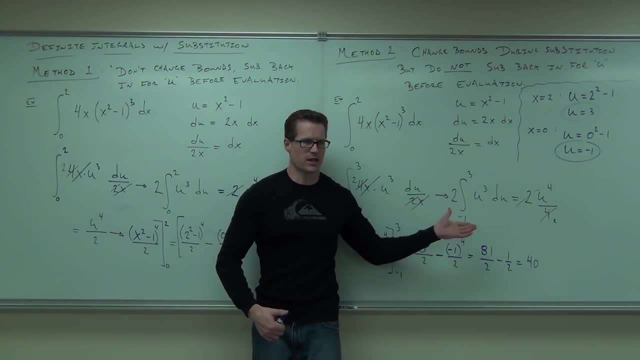 Simply because you're doing the work ahead of time. You don't have to worry about this later on. The two mistakes I see are this: I see because integration's not that bad. I see people making mistakes here. They either forget to substitute. 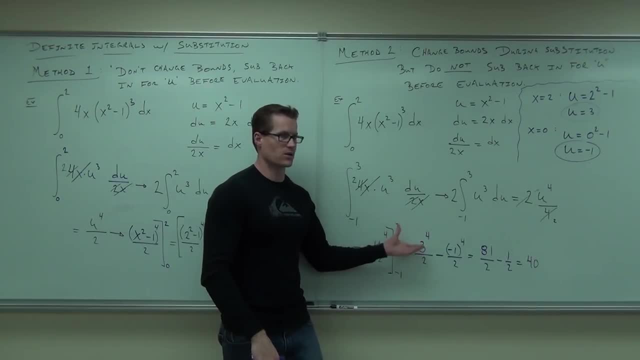 They either forget to substitute. They either forget to substitute. They either go back in X here, or they accidentally do it here again and they get something way off. You see what I'm saying? That's where the mistakes happen. So do one or the other. 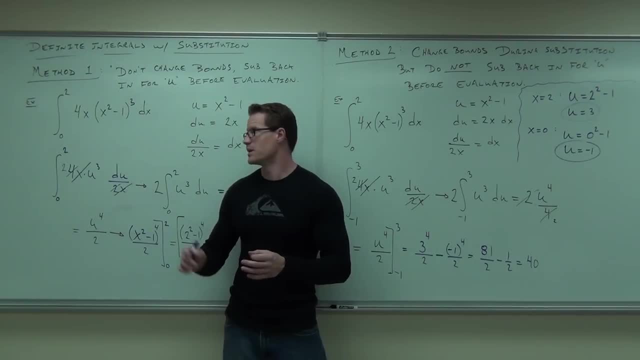 Now, of course, on the test, I will ask you for both. Maybe not even that one. I'll say: do this if you want, But I'll give you some. where you have to change bounds, I say I want to see you changing bounds. 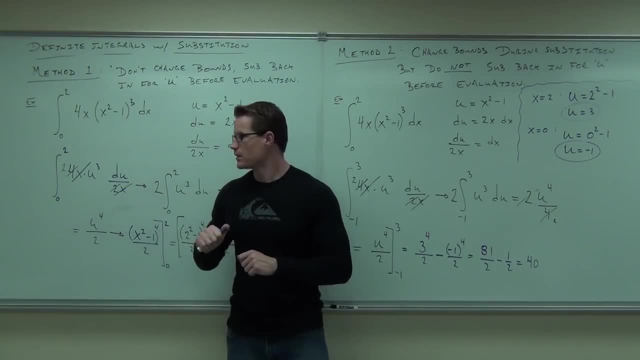 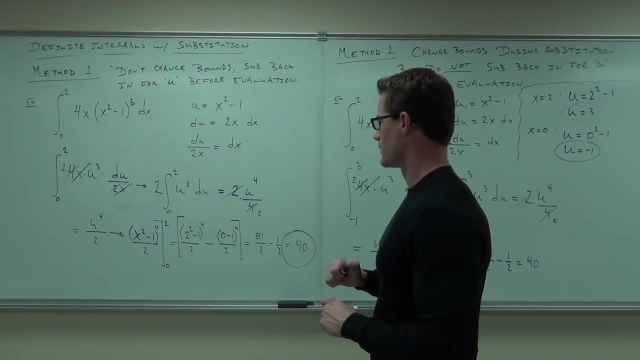 So you do need to learn that method either way. So those intermediate sets though, would you have to use a different notation than method 1? Since, like, where it says 2 times the integral of your k, 2,, 2, 0,, 2, 2, that's not actually true, right? 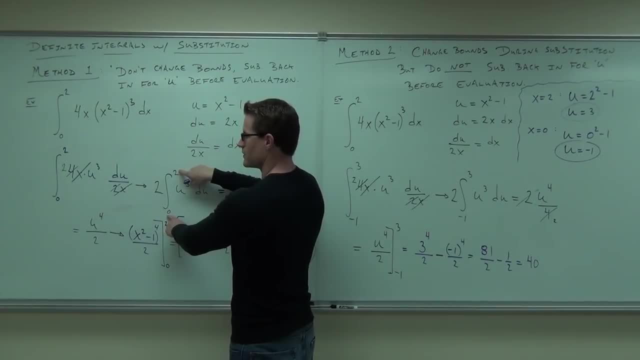 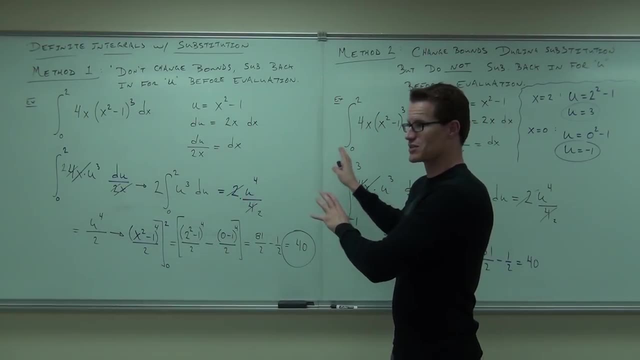 This is slightly off, Right? So how would you actually write that if you were Still write it? Oh, OK, You'd like? Yeah, you'd still write it. But this is one of the reasons why we have that, Because you go, oh, these bounds don't really match. 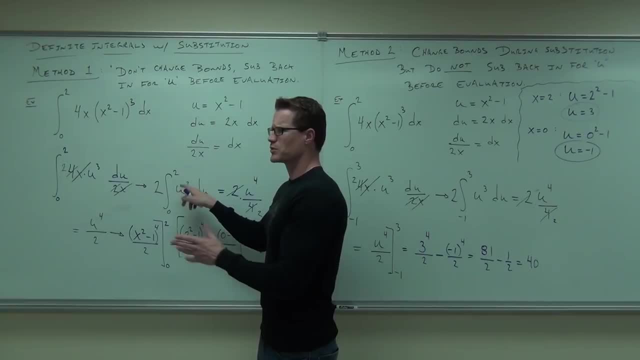 up with that letter. Now you could say: well, maybe we'll just treat like a dummy variable. It's really not, because it's substitution, But we know in our head that we're just going to plug back in for X, So it still works. 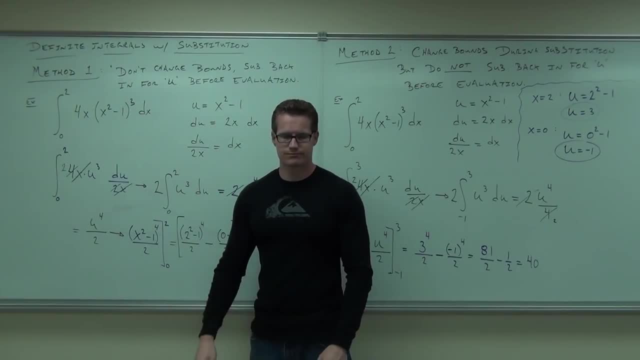 But those really don't match up all that well Because they actually don't. They're X's and that's a U Good question. Any other questions before we go on? So then, as a method of check, you can actually do both methods. 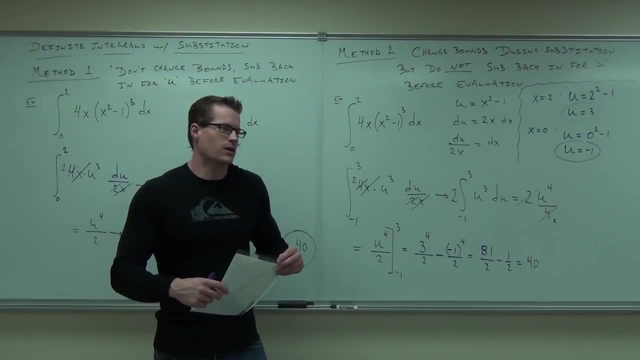 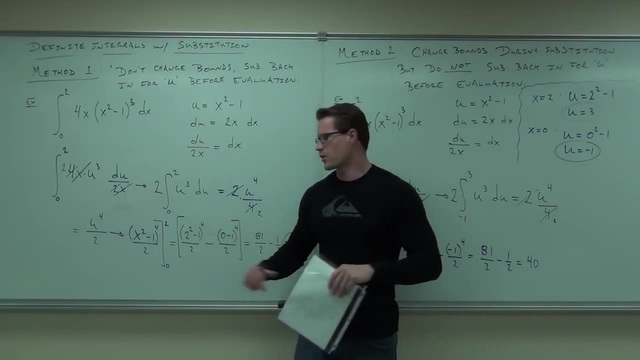 and you should. It has to be the same thing. It is the same thing. You're just doing one part here and you're doing one part here. One part before evaluation, before even integral, and another part after the integral, during evaluation. 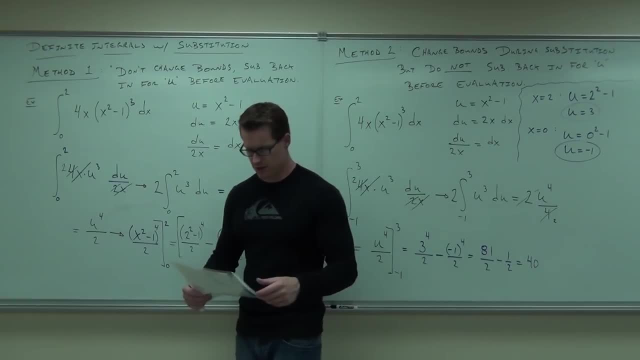 That's really it. You're doing the same work, Same work. It's two different places. Good questions. Any other questions before we go on? Why does that work when you change the range of the bounds? Why does it work? Yeah, 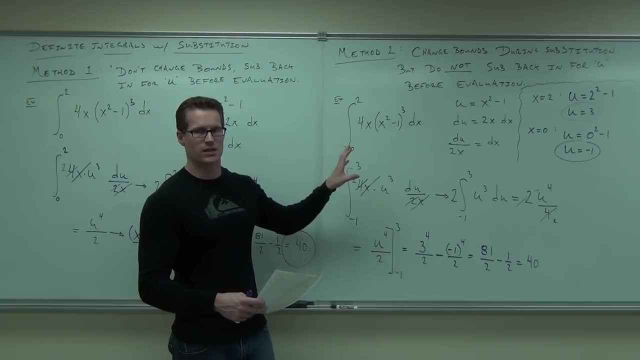 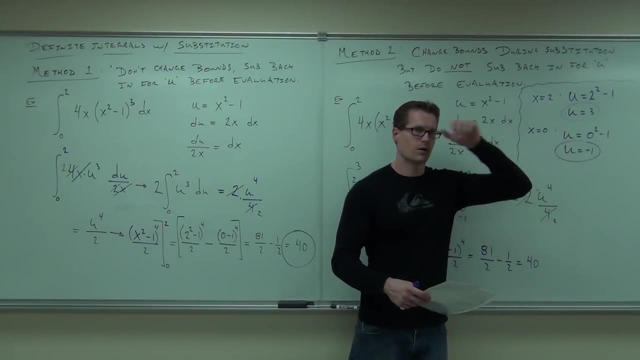 Well, it's taking a function and make it something else, Basically translating Into a different variable. Yeah, And then you have to change your X variable into your U variable to make it work. Okay, So right now this is 0 and 2, but it's regarding the X function. 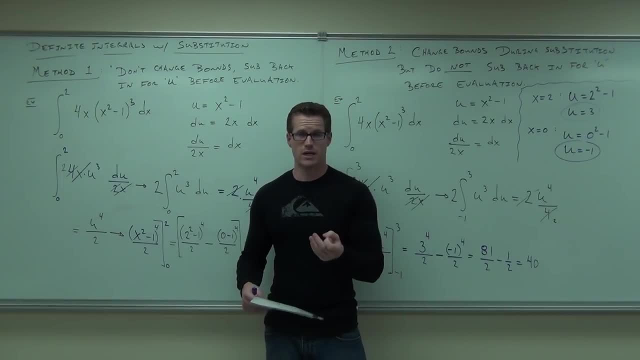 This is negative 1 and 3, but it's regarding the U function that you just created. Does that mean that the integral that we're translating into is within that family of integral? Is that why it comes out to be in the same area? 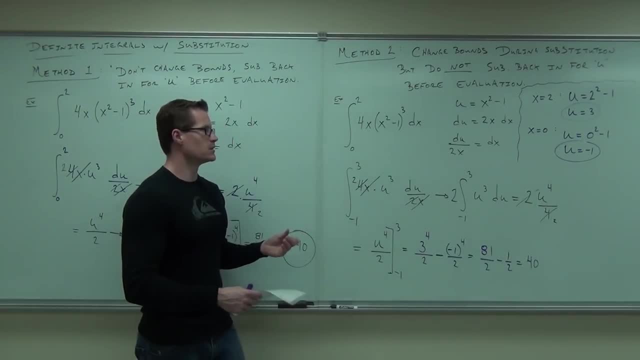 Well, that's a good question. You're completely changing the function when you do this. Right, You really are, And so you're just making it. It's almost magical that it works, It's kind of cool. But you're making a different function and saying the areas will be the same. 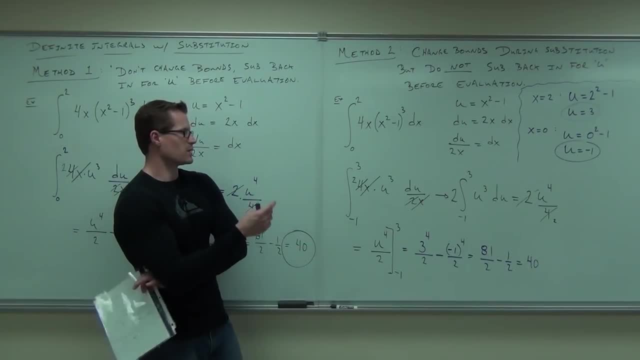 because I'm working with different bounds in that function. If you try to do it graphically, I have a hard time believing that 2U cubed is going to look anything like 4XX squared minus 1 to the 3rd. 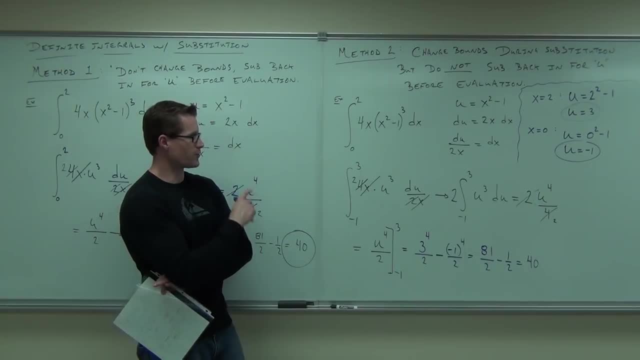 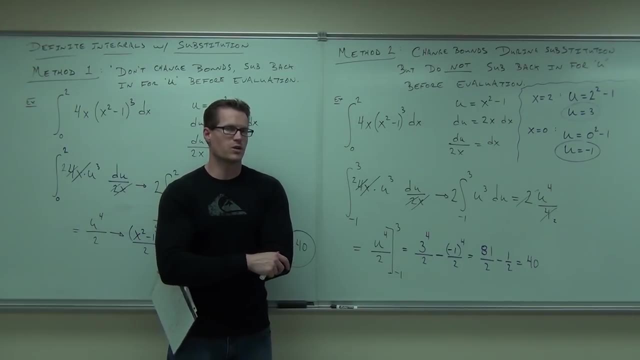 In fact, I know that because a cubic just goes like this: right 4XX squared minus 1 to the 3rd does what we saw. I showed you the graph. It doesn't look the same. So you're changing functions, but you're only talking about the areas. 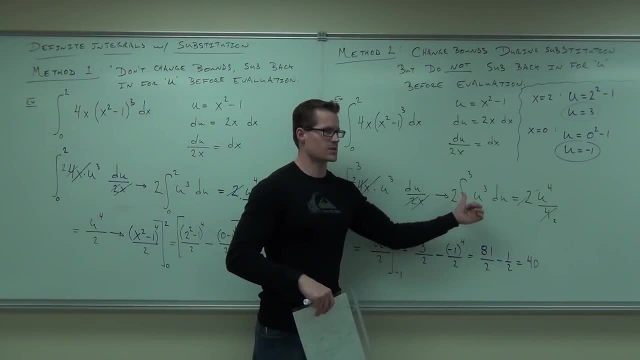 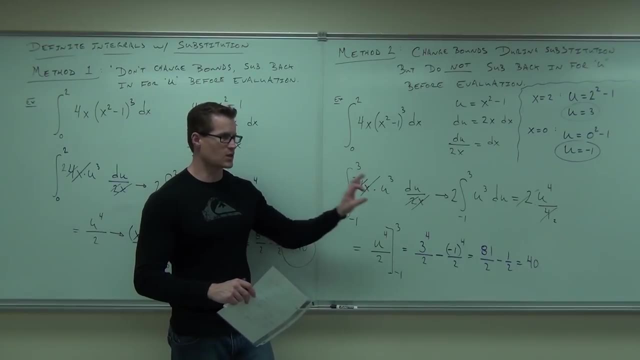 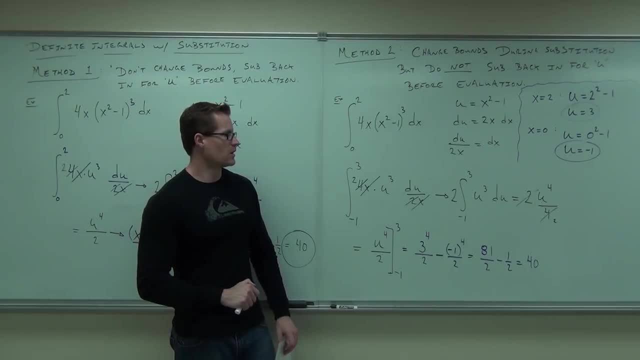 Portion would be a better way to make an analogy there, But something similar to that idea. It's very cool. Now you need to know that substitution doesn't always work right, So you can't always use this. It's only very special cases. 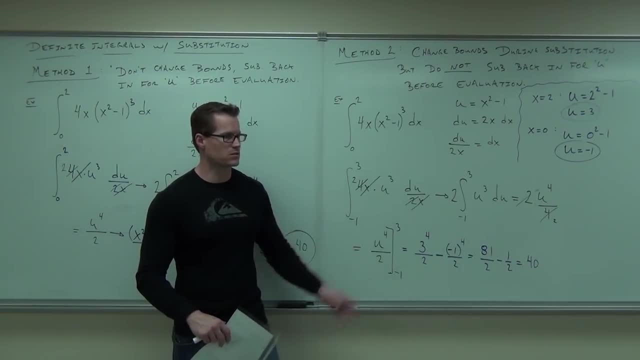 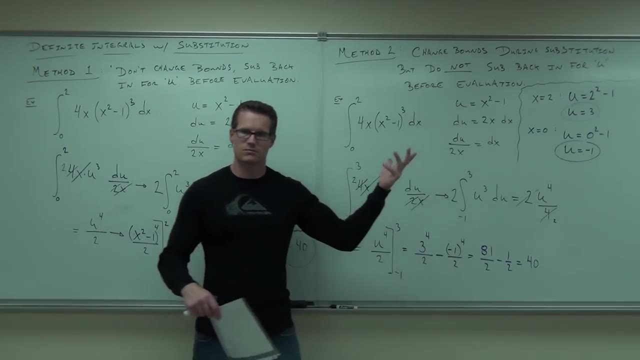 I can give you lots of integrals where you can't use a substitution. In fact, most you can't use a substitution. That's special. Everyone that you can do substitution with the derivative has to be in there somewhere, right, It's got to work that way. 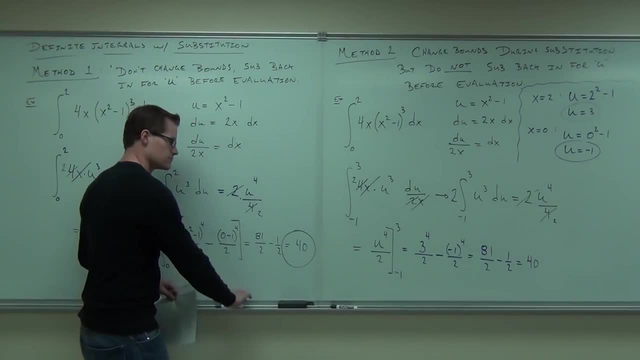 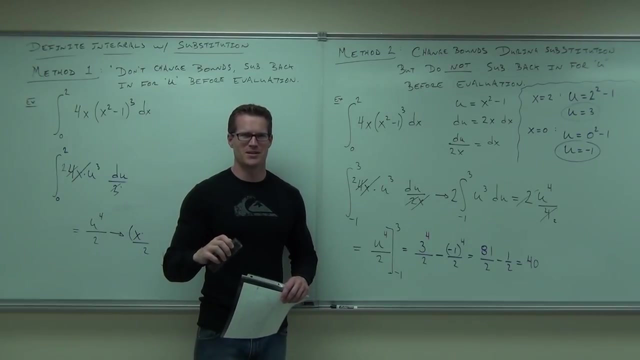 Are we going to deal with the integrals beyond, So that we can't use substitution? It's not in this class, but it's next semester, In your next semester, which I'll be teaching in fall, no, spring, spring of 013, a year from now. 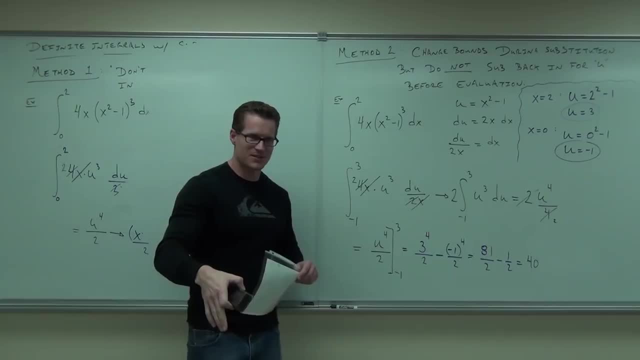 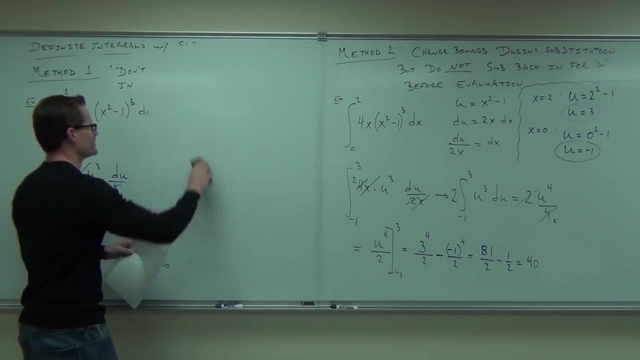 A year from now. So just go ahead and fail this class or something, take it next semester, pass it with some other teacher and then come and see me. I hear I'm down to four B and four C. Just four B for now. 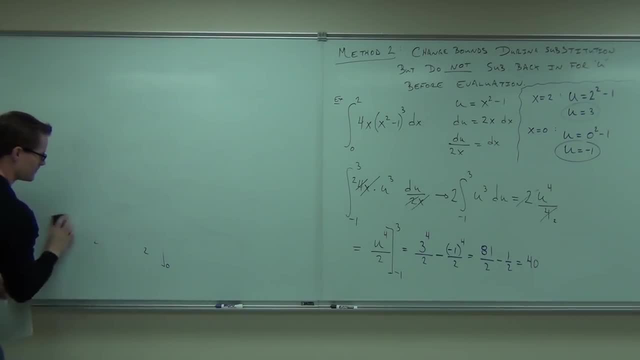 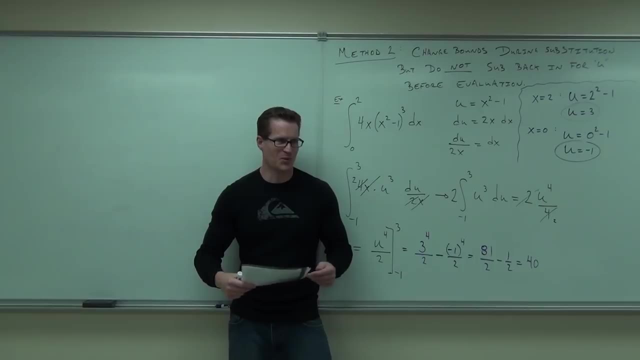 You need to skip up to four C. No, Then my videos won't be in order. See, It just wouldn't work. They're going to be in order, All right. what do you say? we practice a couple more, Would you like that? 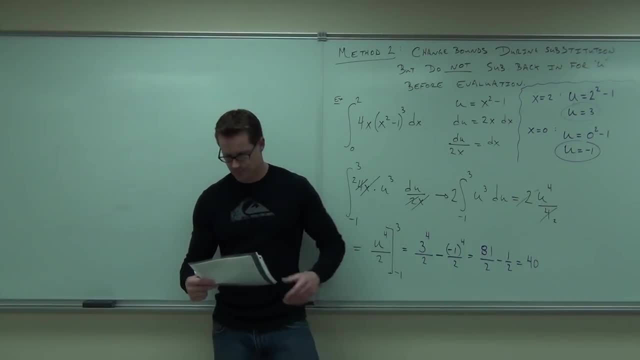 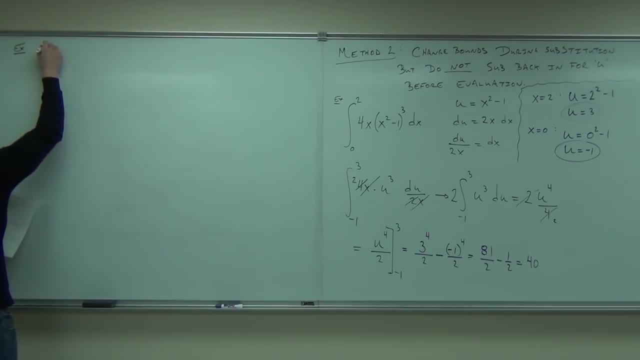 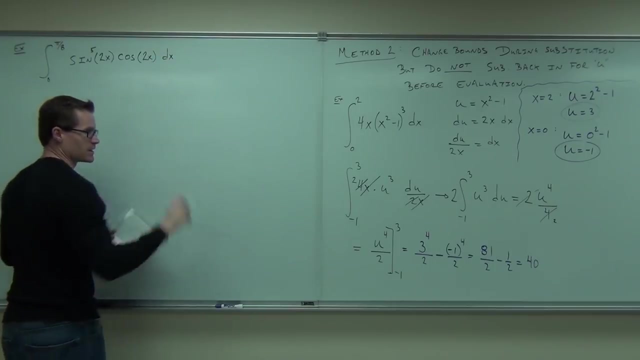 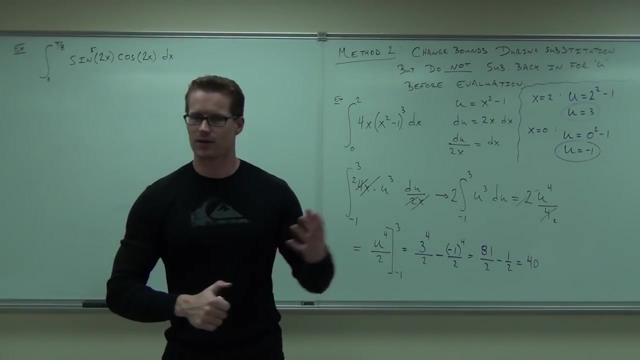 Yes, Oh yeah. I don't want to practice that Hm. That's sticky enough. Some of you always complain I give you stuff that's too easy in class and doesn't look like your homework. Well, here, deal with that thing. 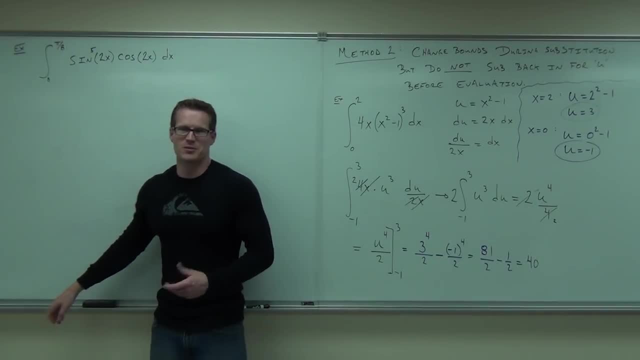 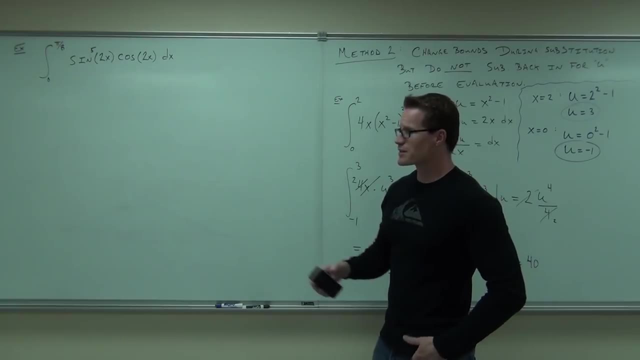 Huh, Actually, it kind of does look like your homework Most of the time. I would say Some of them are harder, Would you not say? I wouldn't say, Except for the most part. Anyway, that's fairly difficult. 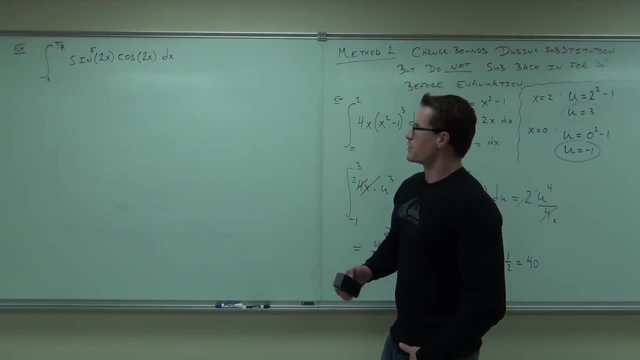 Looks like something that would throw some people for a loop. Let's talk about it. Firstly, is it going to fit your integration table directly just like that? Oh, not at all. So it's going to probably involve a substitution. If we can do it, it will involve a substitution. 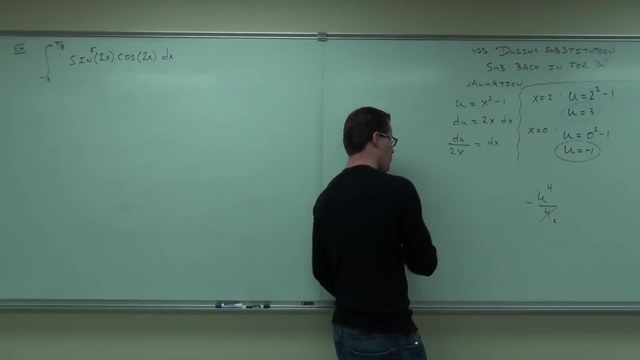 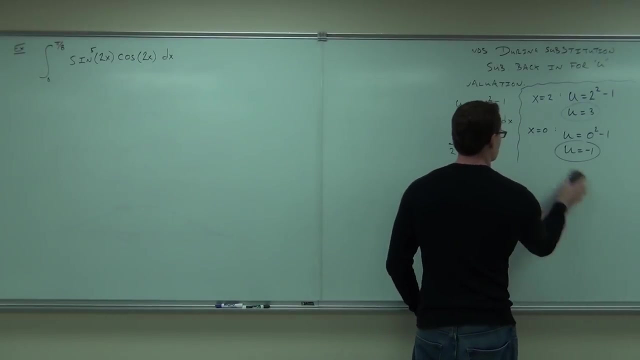 Watch and think through. Don't say it out loud. Just think about what a proper substitution would be. What a proper substitution would be in this case, Think. Don't say it out loud. Some of you might be asking: well, could it be 2x? 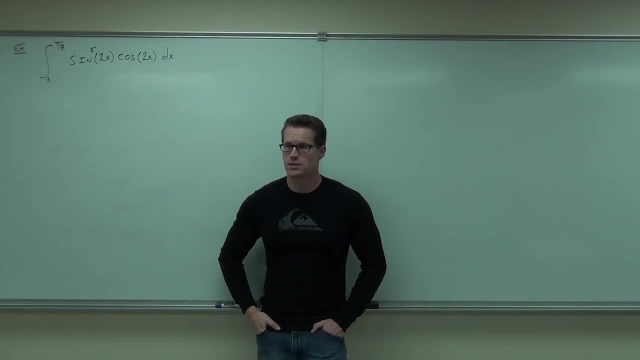 Could it be 2x? If it was 2x, it'd be sine of u to the fifth times cosine of u. Sine of u to the fifth times cosine of u does not fall in your integration table, So that doesn't really help you at all. 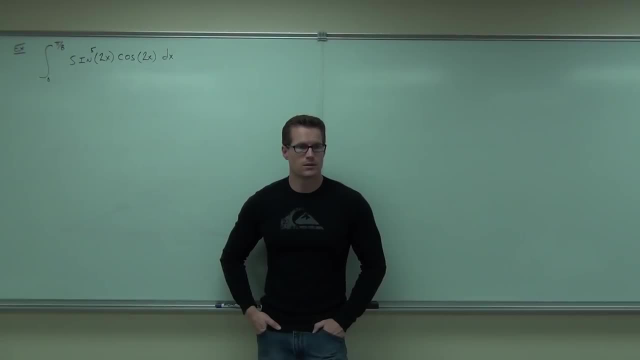 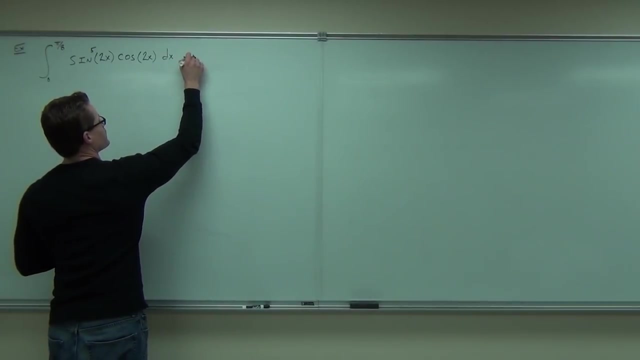 Assign 2x and then change it to parentheses to the fifth power. OK, Let me change it And then you'll get to your cosine. Let me see if I know what you're saying. You're saying that, if I change it to this, 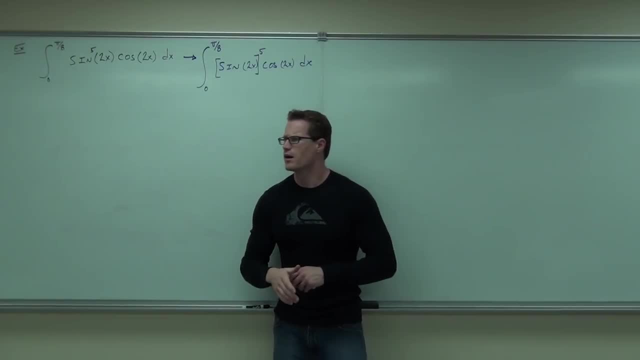 Change it like that. OK, That's good. Why don't you change it to that? What do you think It's easier to see? It really is easier to see, isn't it? Your u should not be 2x. 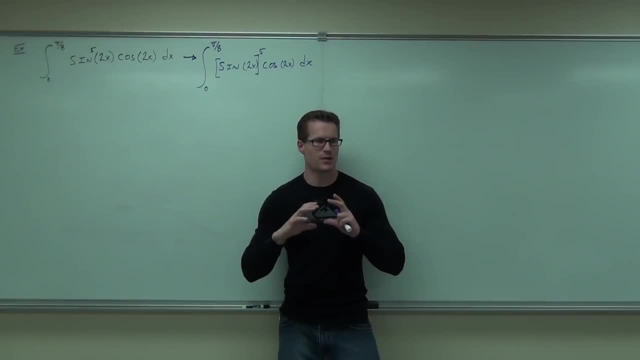 Not 2x. That's not going to work for you. I know I said it's supposed to be the inside thing. This is an inside thing. However, if you take the 2x, the derivative of 2x is only 2.. 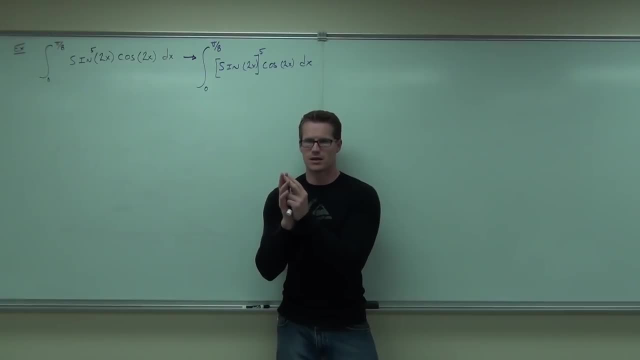 That's just a constant. It's not going to eliminate the cosine. It's not going to eliminate the sine. You're still going to have sine and cosine. That would be a bad choice. But you'd see that bad choice within a minute, right? 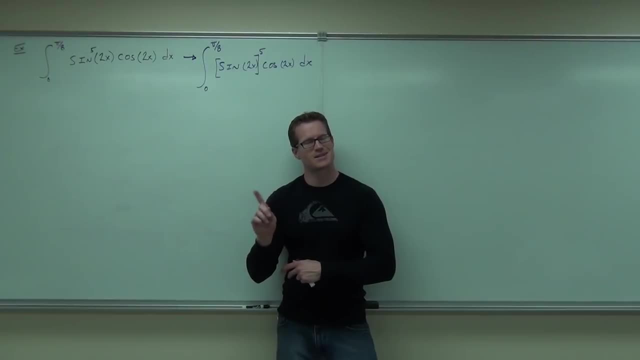 At least I would hope so, Because you'd go through the process your way to saying, eh, something's not right here, Mr Leonard, Change this thing, And then you change it. Then you look back at your integral and say, well, 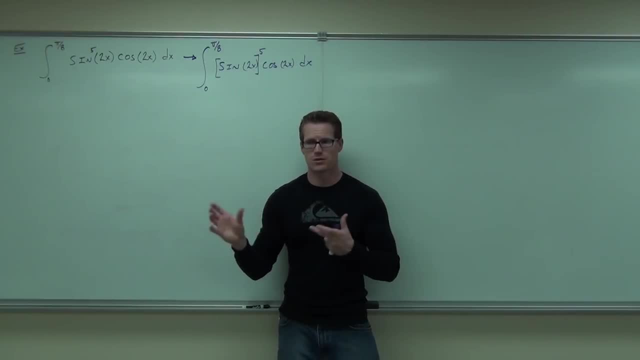 do I pick sine of 2x or cosine of 2x? Because that's the only other thing I'm going to do. I'm definitely not going to pick to the fifth power. Fifth power- you'd have some sort of a chain rule or general. 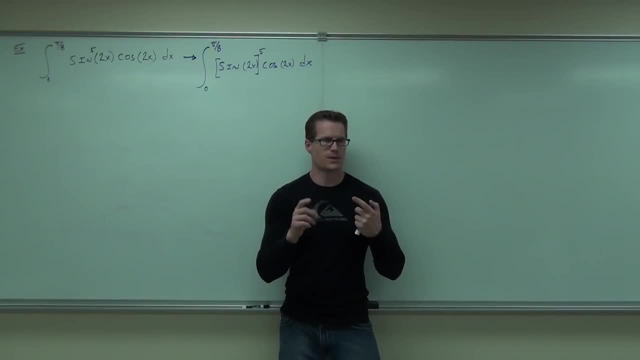 power rule if you want. That's going to make things a little messy Because you're going to have sine and cosine. It's not going to simplify out for you very nicely. You typically pick the inside of something without the power, So we're going to pick sine of 2x. 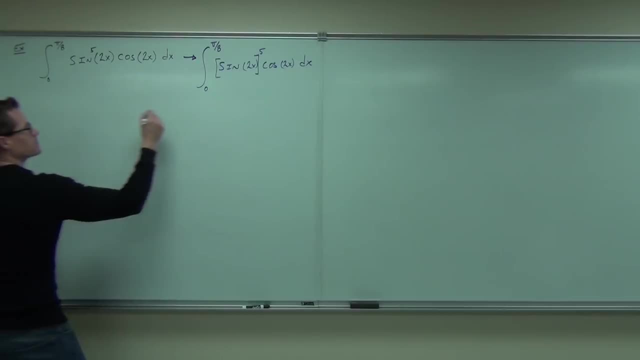 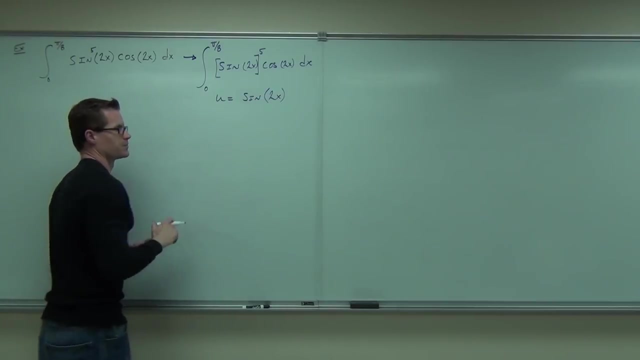 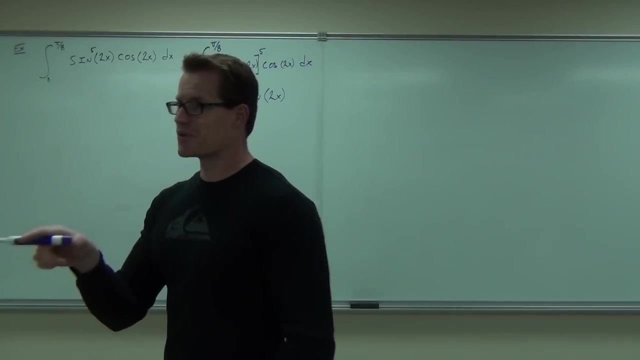 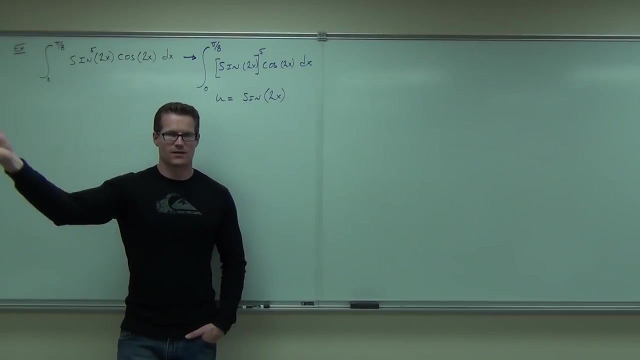 Now you've got to kind of remember how to take derivatives of sine of 2x, Because a lot of people here forget one thing about this: Do you see that sine of 2x is actually a Negative? No, it's not a negative. 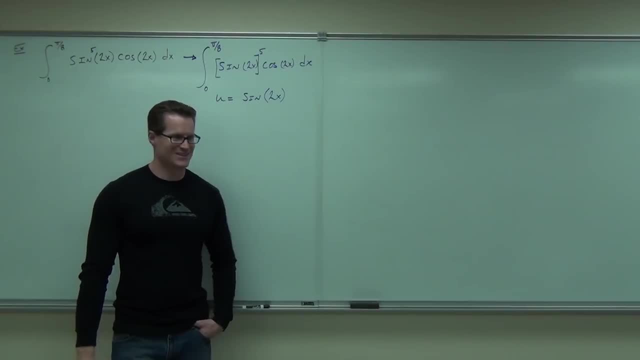 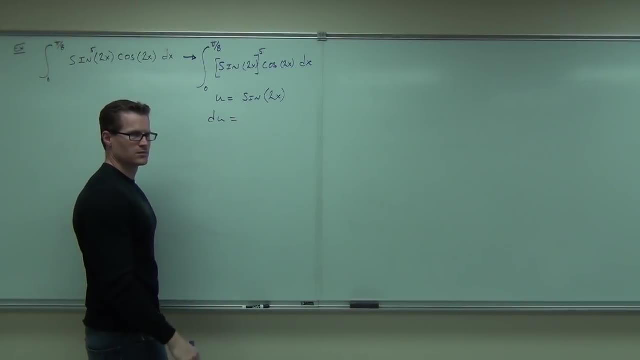 It's a chain rule. It's a chain rule, It's a general power rule or whatever du equals. Here's how you do a chain rule. How do you do a chain rule? You take your sine and flip it to cosine of 2x. 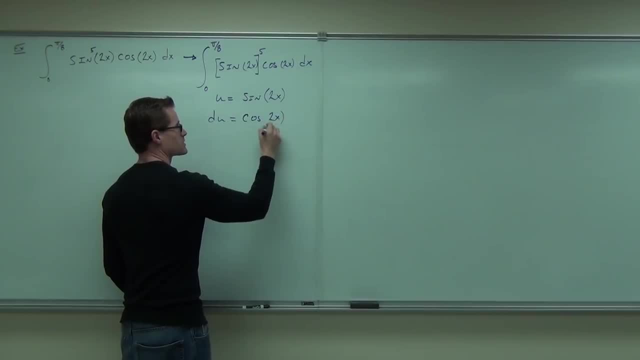 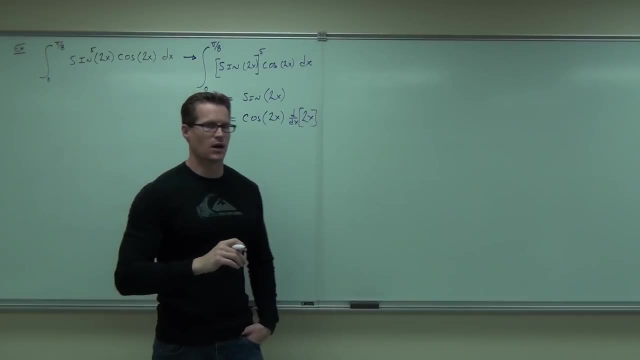 multiplied by dd of x of 2x. OK, Cosine 2x absolutely. But then the derivative of the inside must also be there. You see, when people do this a lot of times they're off by a factor of 2.. 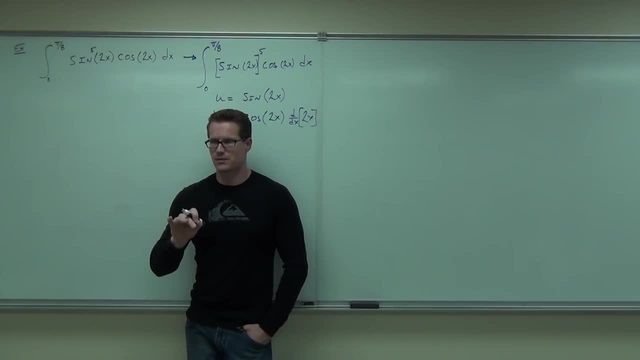 Actually a factor of 1 half, because when you divide it's 1 half, But they're off by that, They're off by a factor of 2. Because they forget all about the 2.. Do you see the 2?? 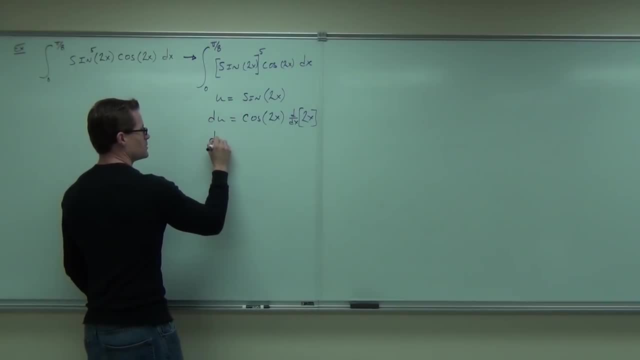 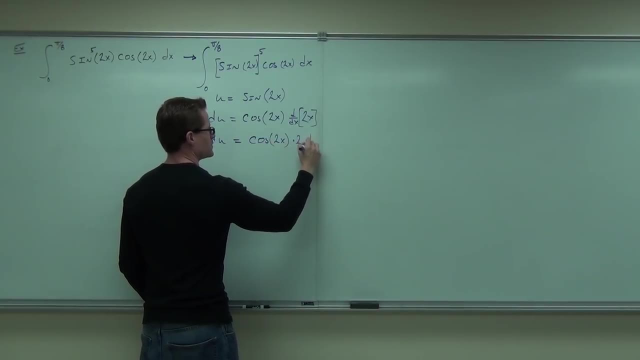 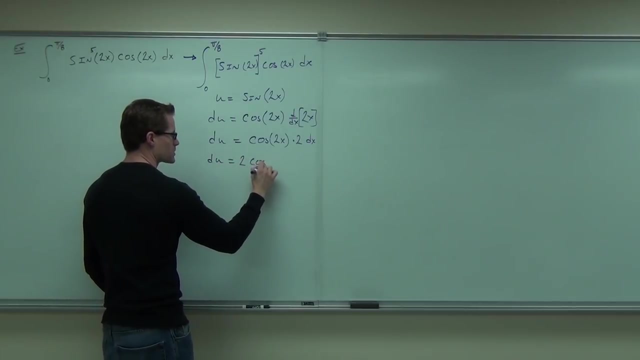 Don't lose the 2.. OK, So we're going to have du equals cosine 2x times 2dx. Otherwise I'd probably write it as 2 cosine 2x dx. That's the appropriate way to write that. 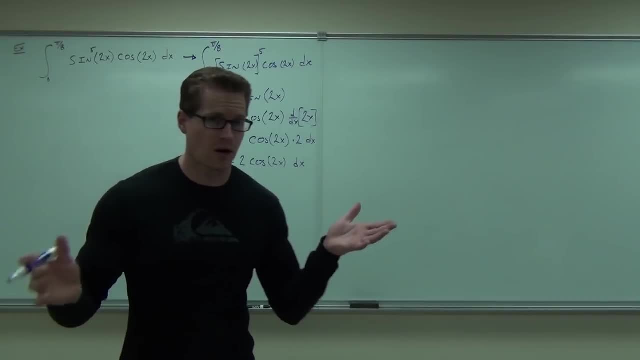 Just don't lose the 2. It's a chain rule. You don't have the derivative of 2x somewhere. The derivative of 2x is the 2. Move it out in front of your cosine. So what we're going to get is du. 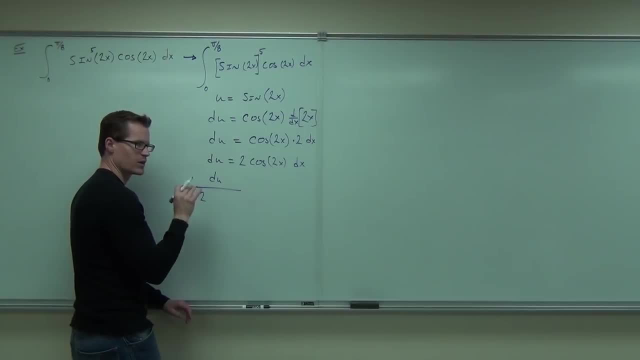 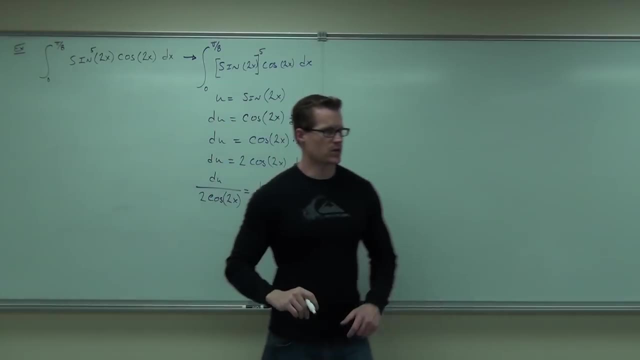 Once we solve for dx, it's going to be kind of obvious that we picked the right choice, And here's where you'd make that judgment. By the way, you're getting more practice on substitution right now, too right. It's kind of nice. 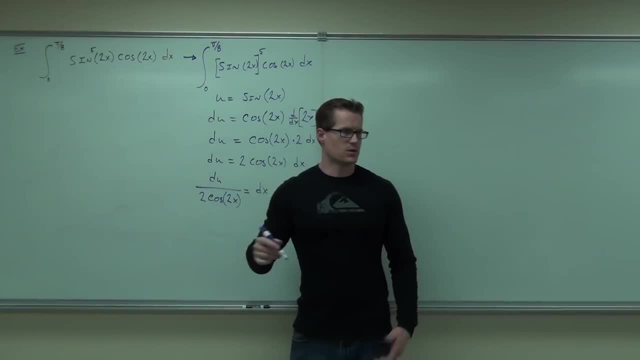 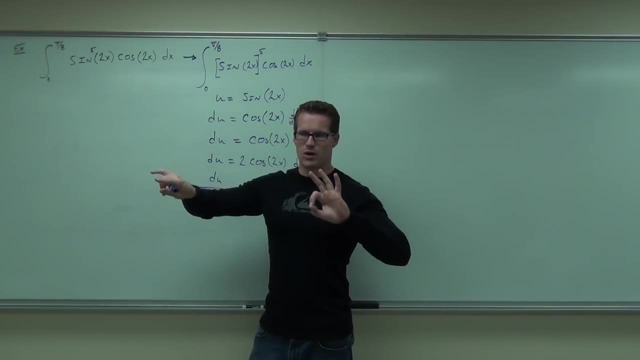 Do you see anything that's going to cross out? That's where you make your judgment. You go OK. If this becomes a? u, I'm good to go. If this gets crossed out, that's fantastic, And I'm going to be left with no more x's. 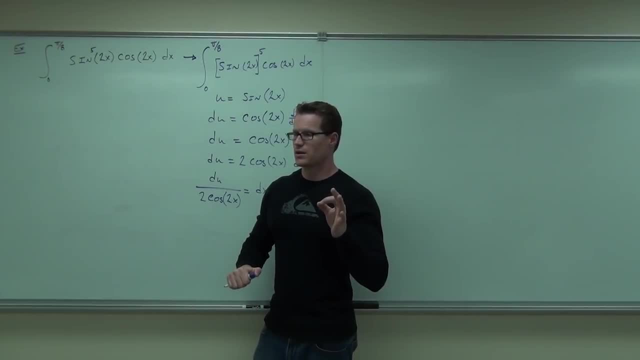 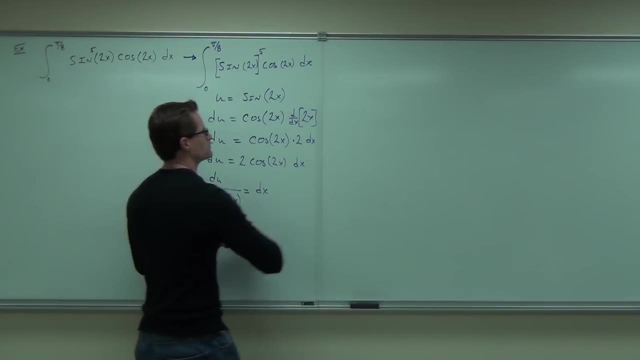 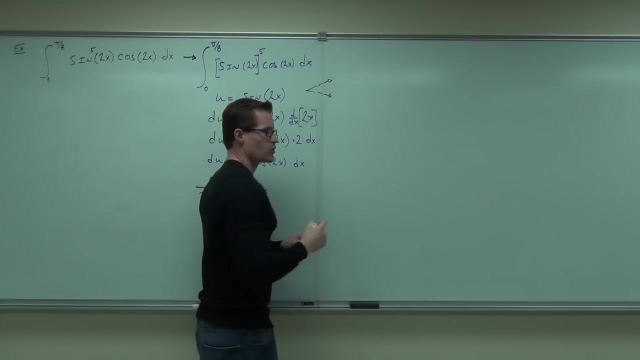 And that's exactly what we want. Feel OK with this so far. Now, at this point, we're also going to change our bounds. We're going to change our bounds Because I don't know about you, but I'd rather deal with the bound changes now. 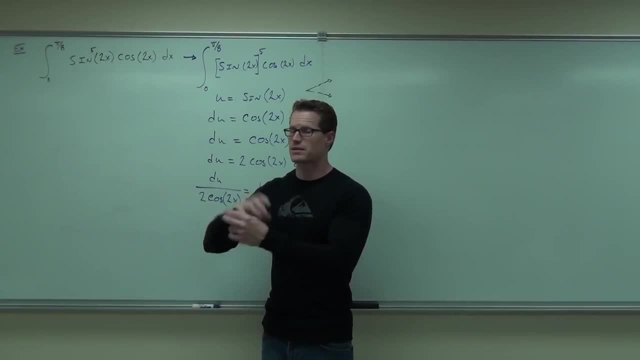 and then just have to plug in some numbers, rather than change everything back to sine of 2x and then have to plug in numbers and then figure out the sine of that again. You follow me, I don't want to have to do that. 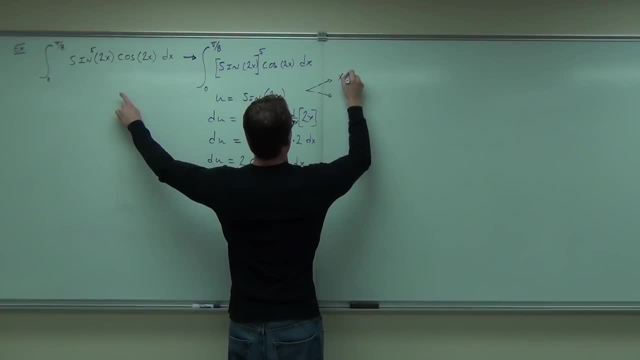 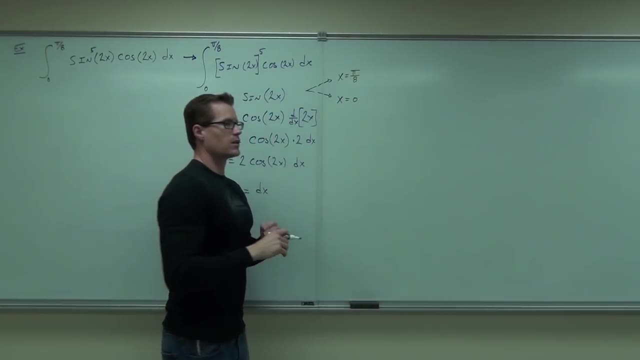 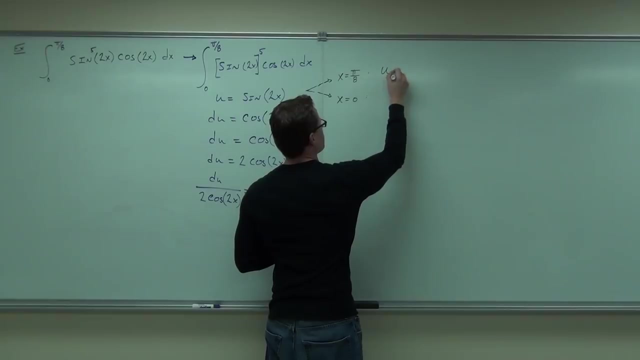 So when we have x equals pi over 8 and x equals 0, let's figure out what those things are. Some of you guys are zoning out. Don't zone out, Stick with me here. You use your u substitution, You plug your x in and you figure out what u's value is. 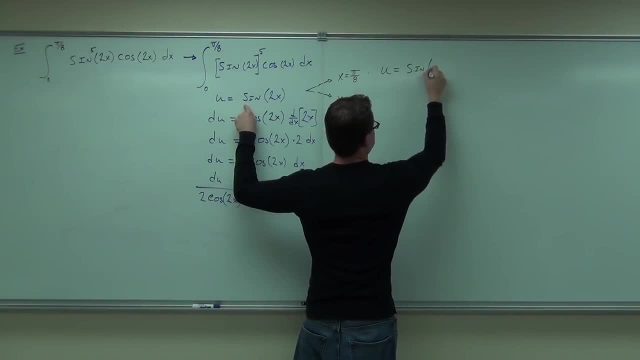 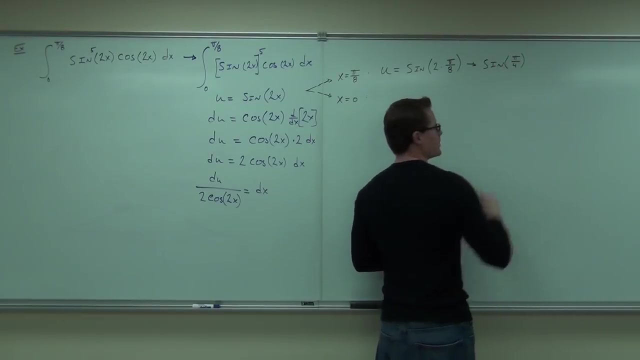 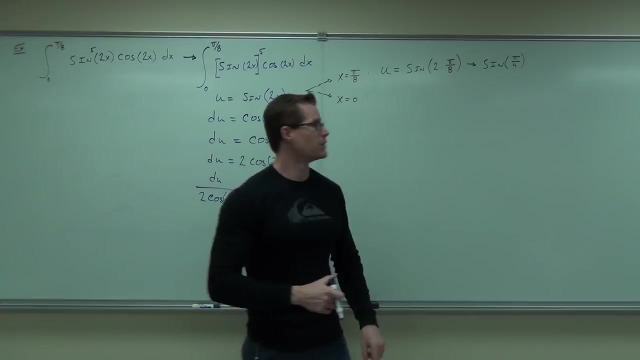 So here we'll have sine of 2 times x. Well, x in this case is pi over 8.. How much is sine of pi over 4?? 2. Square root of 2 divided by 2.. Very good, Absolutely right. 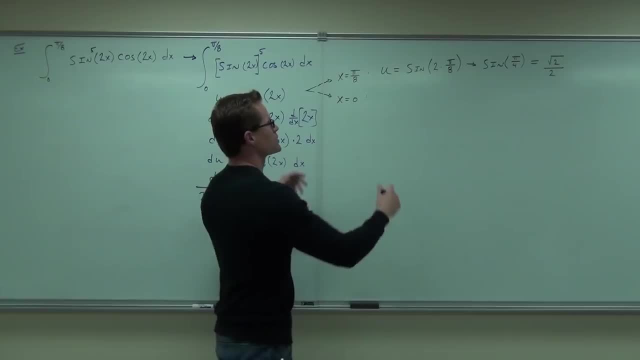 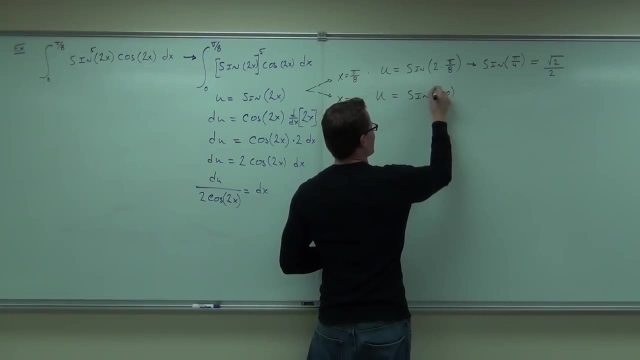 You guys OK with the root. 2 over 2? Awesome, Let's do the 0.. I'll take care of the 0 for you. Sine of 2 times 0.. I love this one. That's sine of 0.. 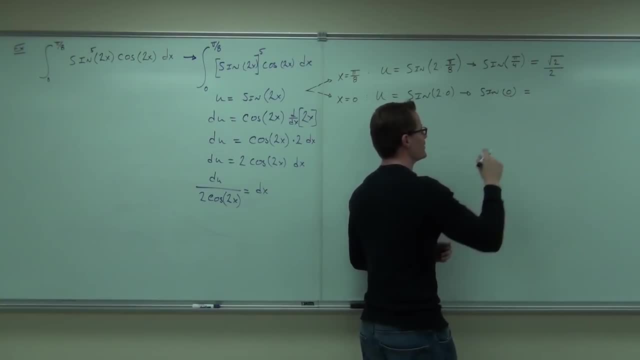 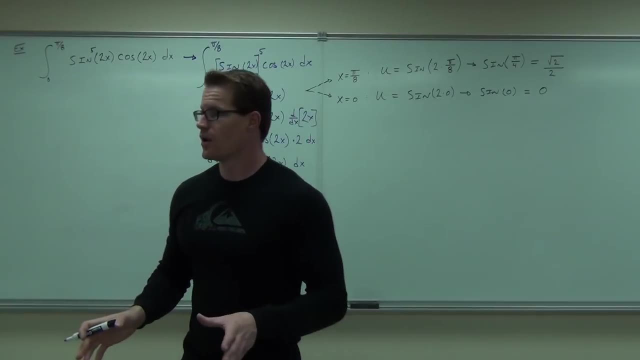 Sine of 0 is 1, right, Good, Just checking, I was really checking there. Yeah and 0.. Sine of 0 is 0.. So do you know your new bounds? Let's do the substitution. 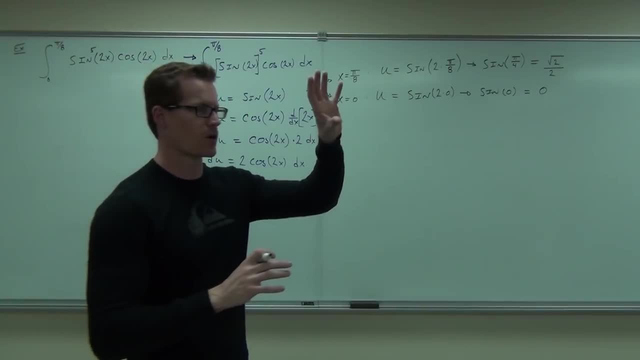 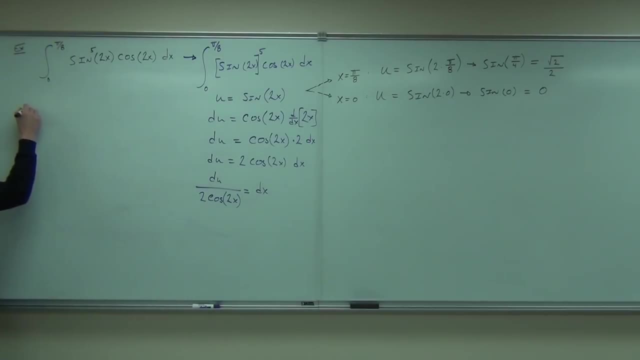 Let's do it correctly. Let's substitute everything we can. We'll substitute for dx, We'll substitute for the sine of 2x, We'll also substitute for bounds. So here's how the integral looks when we're done all our substitution. 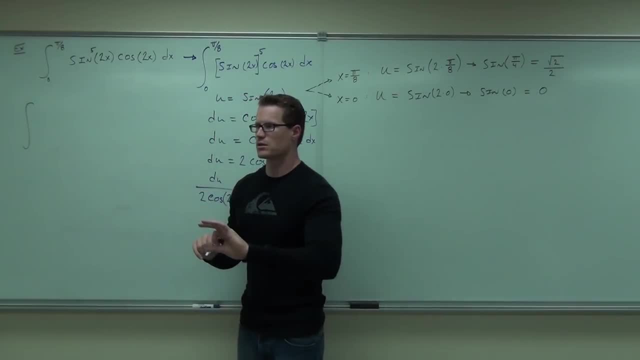 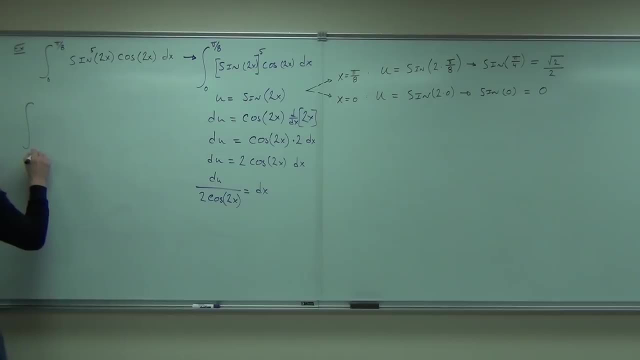 We go from where to where. now, Where do we start? 0. 0 to where 2 over 2.. That's because we're going to change all this stuff in terms of u. That's why we did our changing bounds. 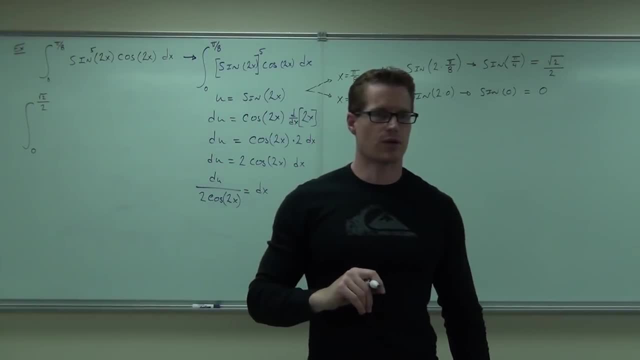 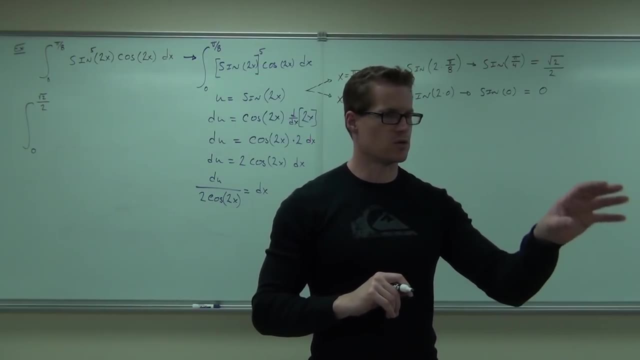 OK, Is the sine of 2x to the fifth power still there? Can you please tell me what I have instead, A little left. u to the fifth, u to the fifth. Not just u, but u to the fifth. That became a u. 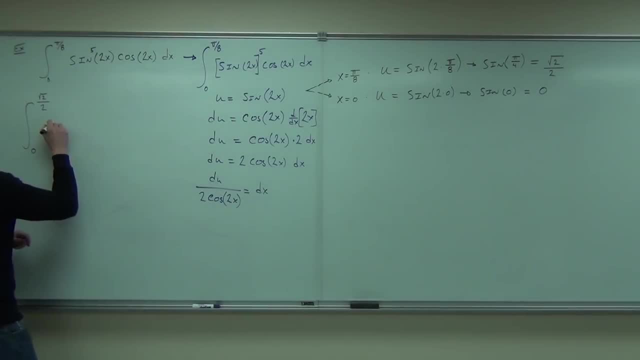 Yes? u to the fifth. Do I still have the cosine of 2x there? Yes, As of right now. Yes. Do I still have the dx there? No, No, That's our substitution right here. We're going to do du over 2 cosine 2x. 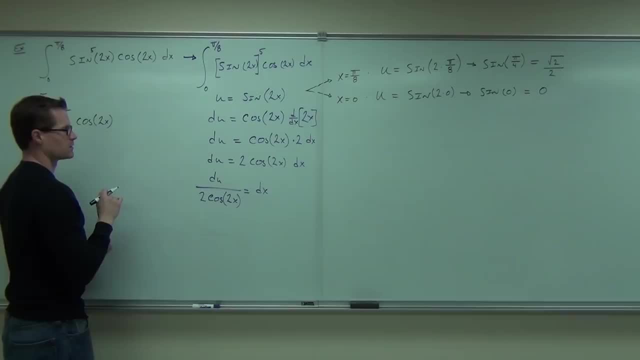 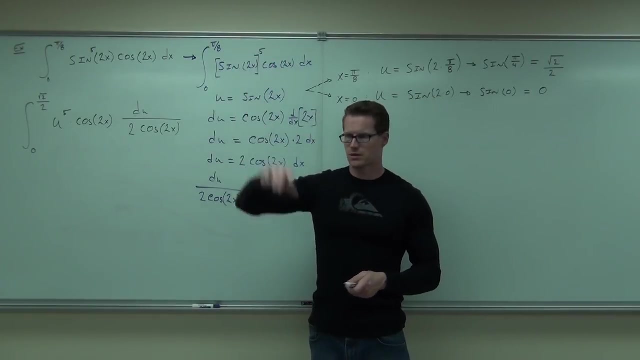 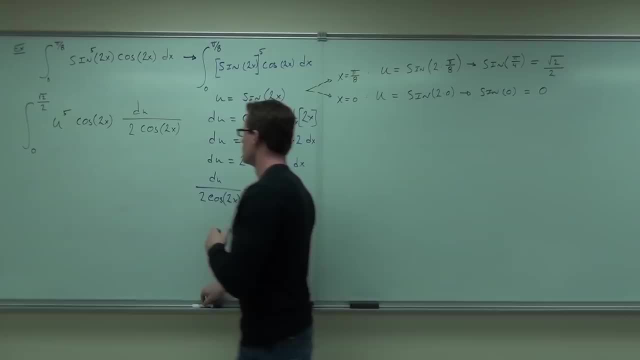 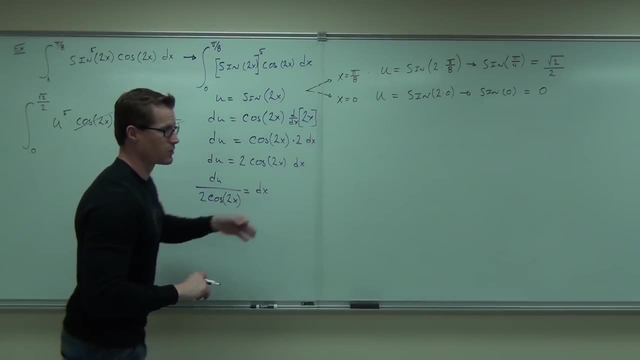 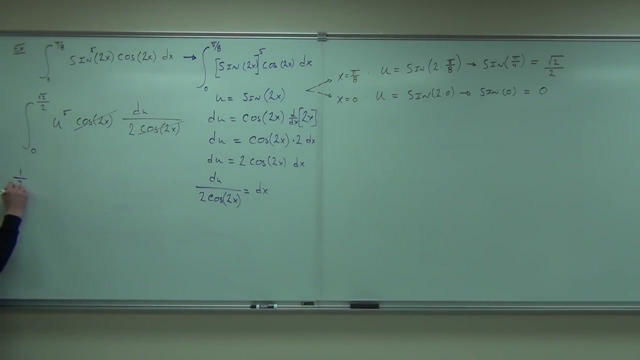 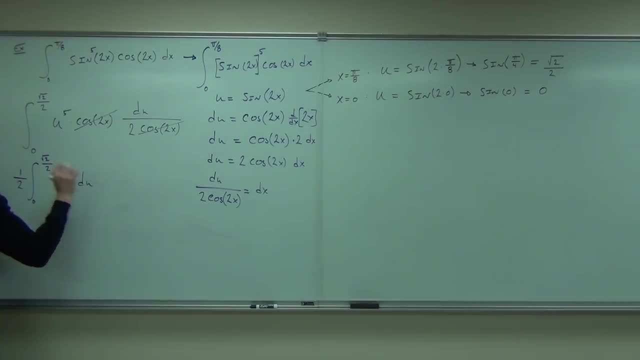 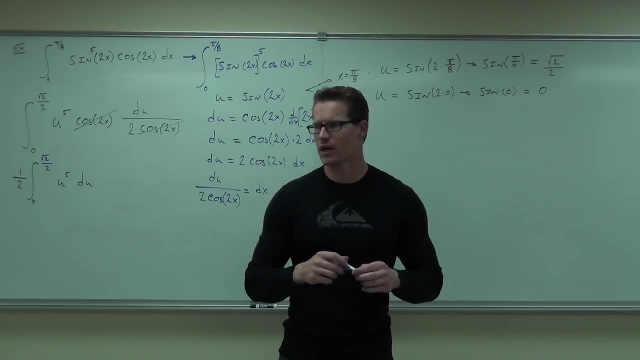 What's the cosine? All cosine plus du. Now that is a nice easy integral. The numbers you have to plug in aren't all great, but that's okay, Just plug them in. So take our integral, we're gonna get. 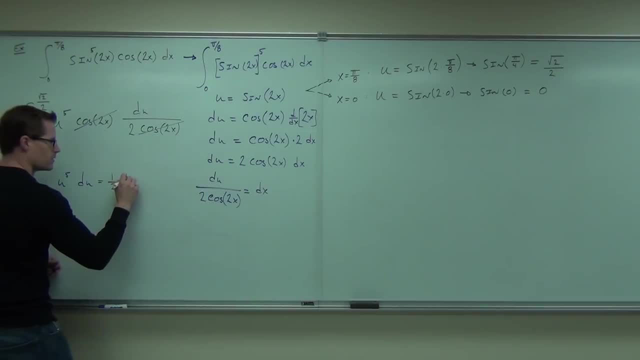 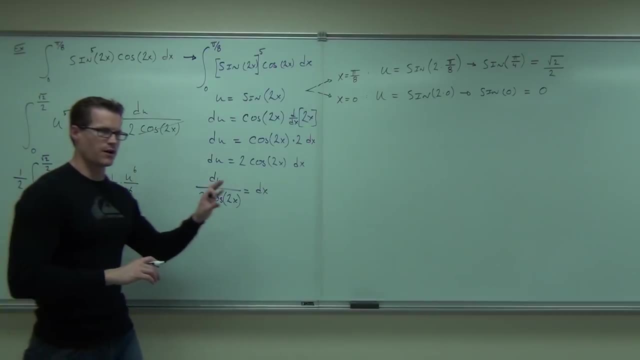 don't forget about that. 1 1⁄2.. 1 1⁄2? u to the sixth over six. I'm gonna make this nice and neat before I evaluate. I'm gonna get u to the sixth over 12.. 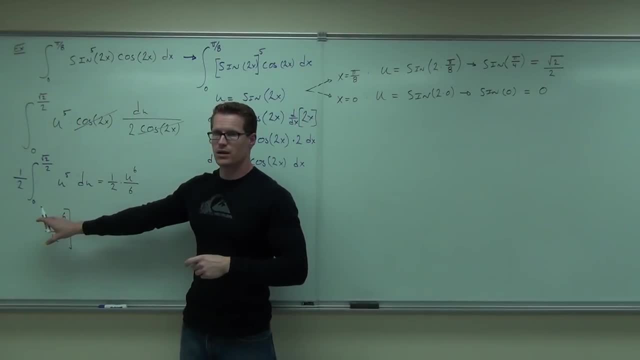 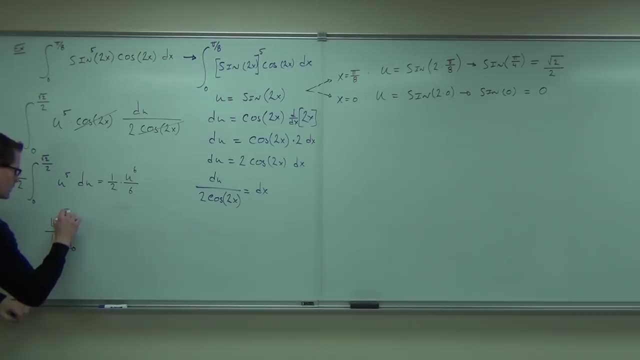 And do I have to plug in the x back into this thing before I evaluate? Why not, Because you've already taken care of it. I've already changed my balance. That's exactly right. Okay, so root two over two. we're gonna plug that in first. 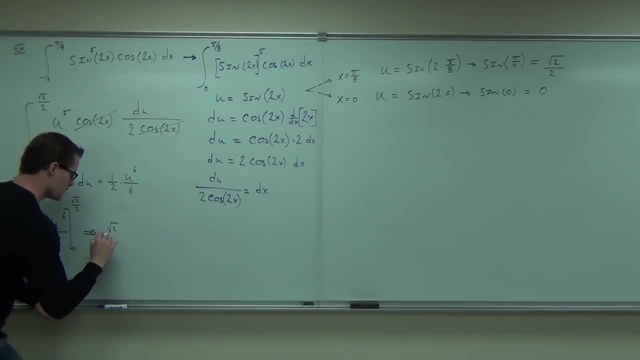 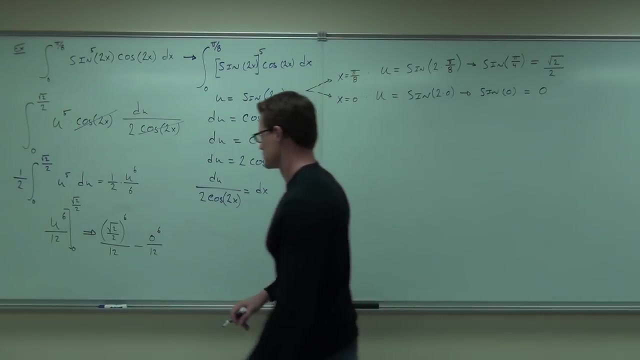 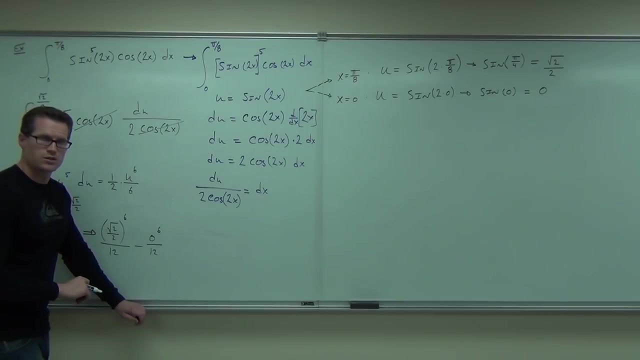 then we'll subtract and plug in zero. So root two over two to the sixth, power over 12, minus zero to the sixth, power over 12.. What's two to the sixth? It's how much? Two to the sixth is 64?. 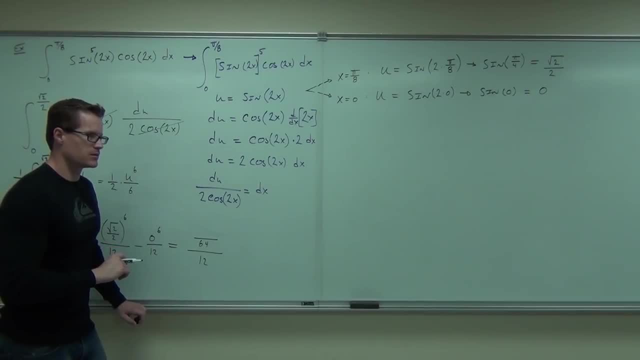 Now root two to the sixth. power is two to the fifth. power One-third should be eight. So you've got eight 64ths there as well. It's what? two to the fourth? Yeah, root two to the sixth: Eight, because it's eight. 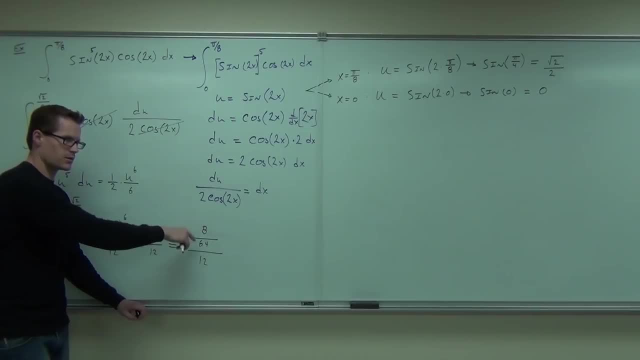 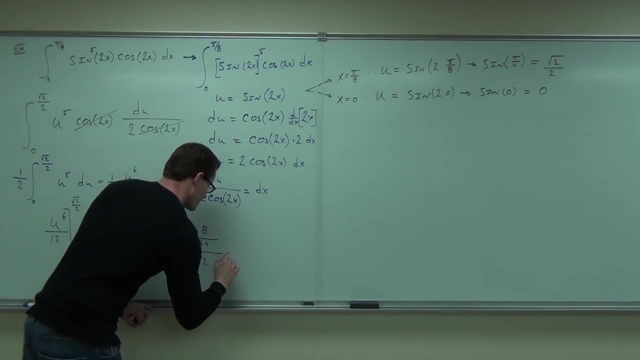 It is eight, right? Yeah, That's gonna be one-eighth. Yeah, one-eighth. Am I way off or am I okay? No, you can try it, You're good, Just making sure. One-eighth and then minus, yeah. 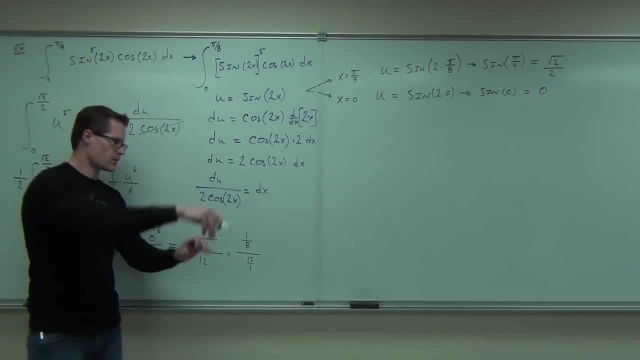 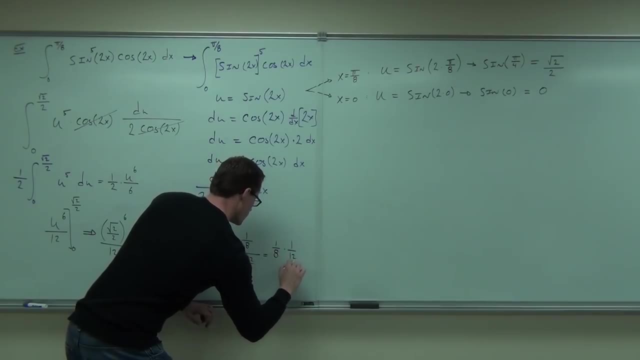 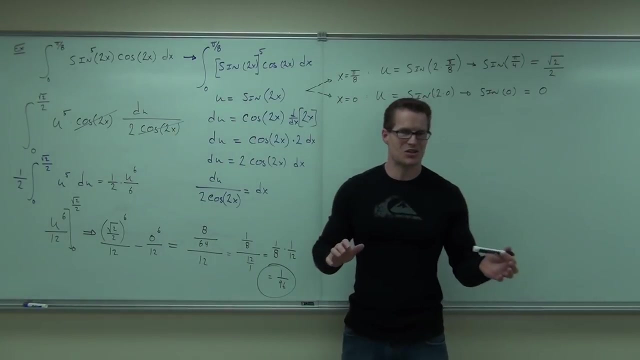 One-eighth over 12 over one, Reciprocate and multiply One-ninety-six. Okay, what I'm asking you: are you okay up to here? Are you okay up to here? After that, use your calculator, do it. 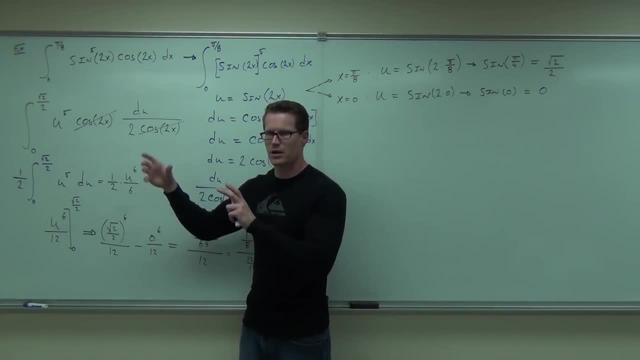 I did it because it's square root of two squared to the third. So square root of two squared is two, then two to the third is eight- That's how I did it- And then two to the sixth. I had to have hope with that. 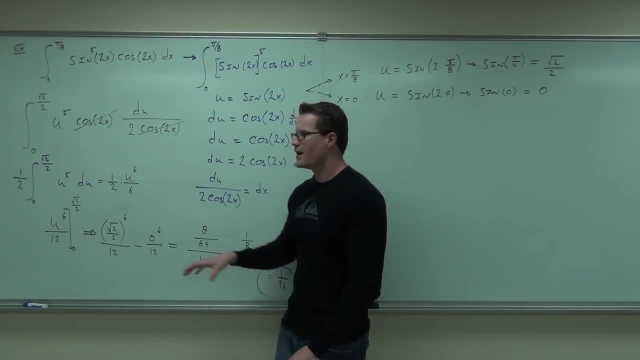 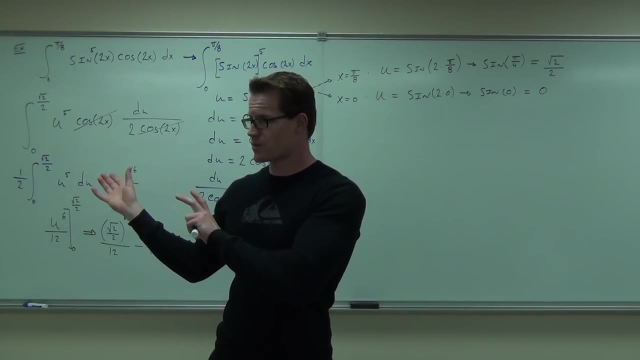 That's the 64, and then you start simplifying that. That's the way you'd probably do this without a calculator. How many people understood what we just talked about? Feel okay with both methods. You can do it without changing bounds, right? 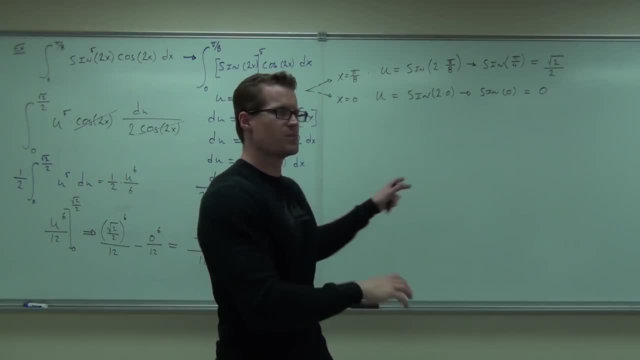 That's pretty basic. Just make sure you sub in before you evaluate. Now changing bounds a little bit more advanced of a concept, but it makes things easier sometimes. Nice, nice, doing this off to the side, You don't have to really worry about it. 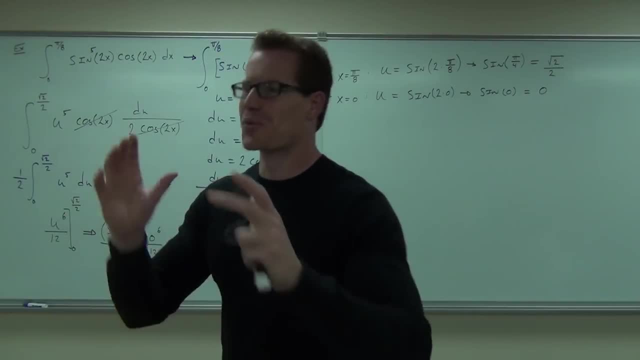 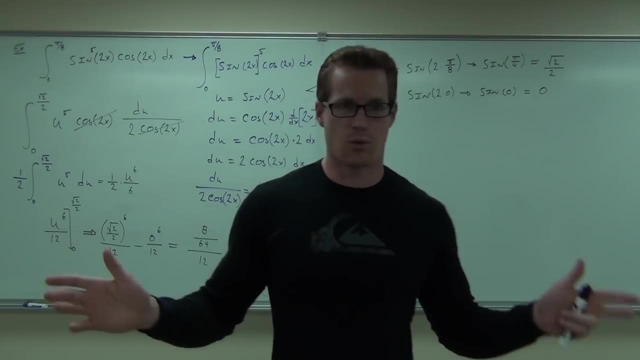 and then you just use your U. Just make sure you don't. the worst thing you can do is substitute back in for F, Just substitute back in for X here and then evaluate with your terms of U. That does twice the work with no reward. 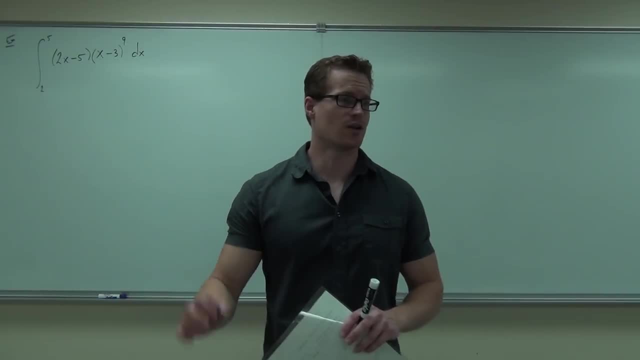 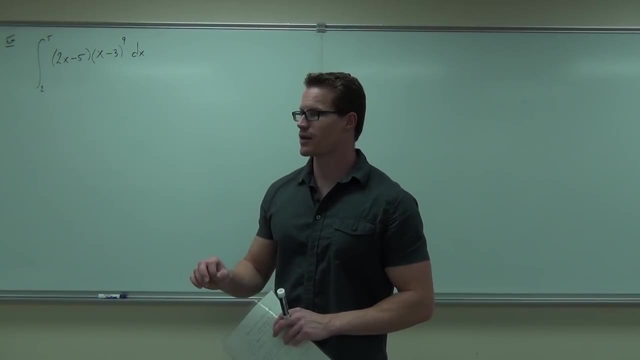 All right, let's continue. a couple examples. Like I said, we got maybe two more to do. I'll show you how even and odd functions can play a role in calculating some integrals, sometimes very nicely, And then we'll get onto how to find the area. 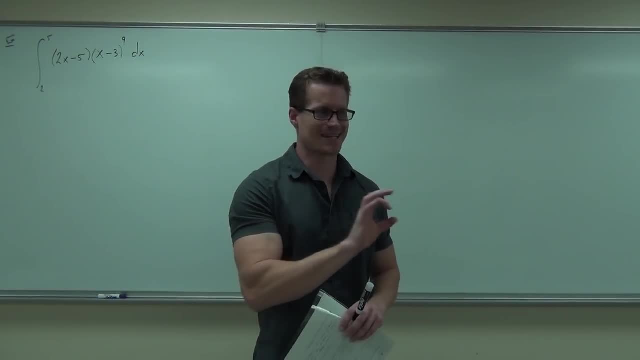 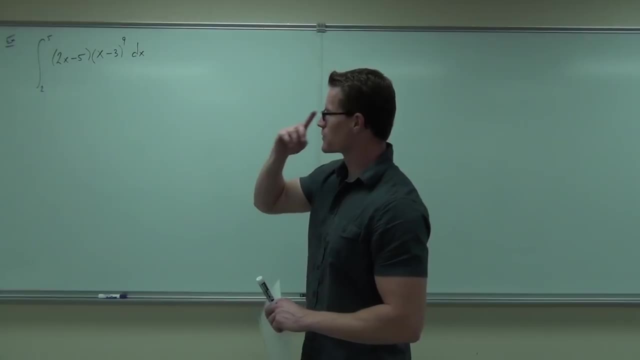 between two curves and you're gonna find out that it's just a small extension of what we've been doing so far. You guys ready for today? Let's do this. Looking at our first example, we got the integral. Of course, we're talking about a definite integral. 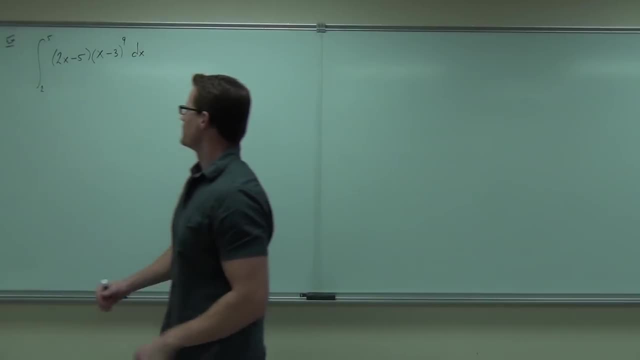 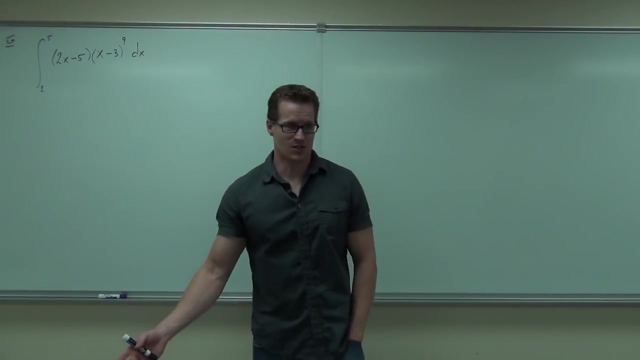 so think, in an area From two to five, of two X minus five and X minus three to the ninth power. Now, does that fit your integration table? In order to make it fit, you'd have to distribute the X minus three to the ninth. 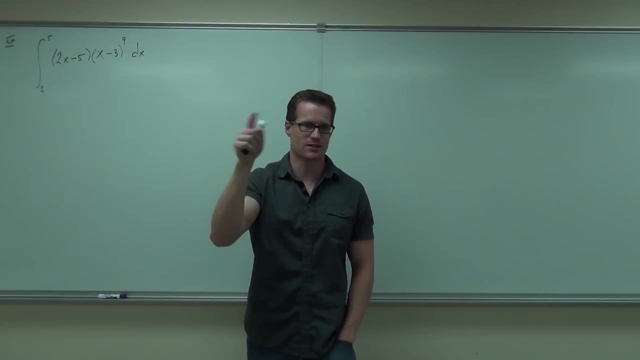 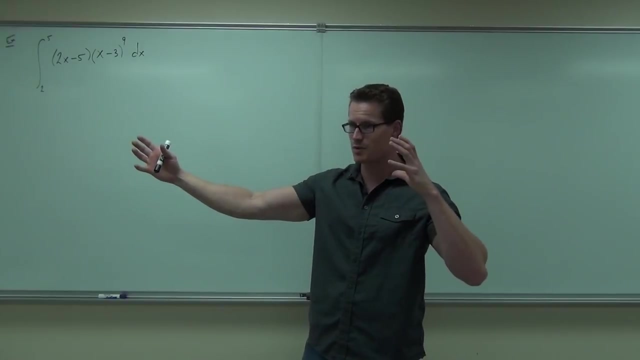 and then foil. well, foil, oil, oil, oil, oil, oil oil. first outside, inside, inside. all that, Not just foil, but anyway Several, several times, Until you got this huge polynomial. then take the integral of each piece. 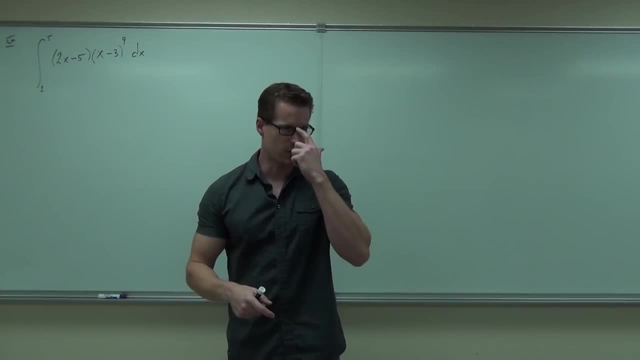 which would be fine to do. It would take you a long time, but it is possible. And then you plug in the numbers to every single variable. That'd get a little tedious, right? So if that's the case, when it looks like that, 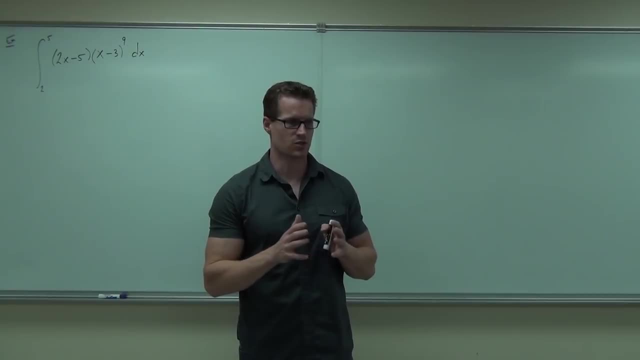 you're probably gonna try a substitution. Probably gonna try a substitution. Now, one is not readily apparent because what I've told you about substitutions is normally: usually the derivative has to be up there somewhere, right, It's gotta be. 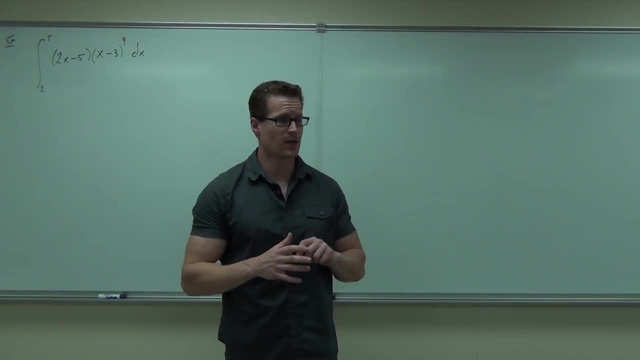 If not, you need to manipulate the substitution somehow. So let's go ahead, let's pick a substitution, the one that you probably want to pick right now anyway, and then let's see if it works for us. okay, So pick a substitution right now. 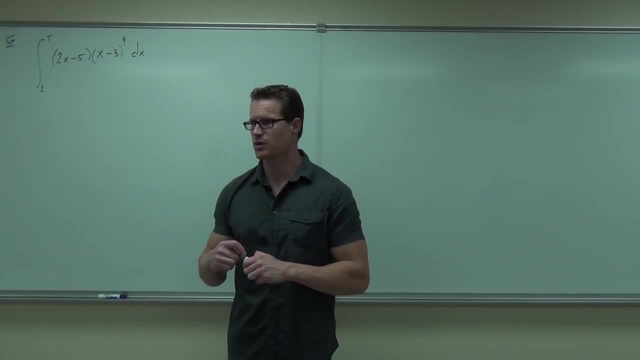 Go for it on your own, Using what I've told you. pick a substitution. Is it two x minus five or x minus three that you picked? Good, including the ninth power, or not? No, it's usually just the thing inside the power. 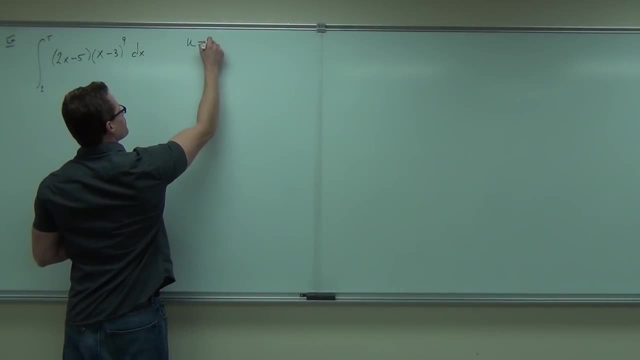 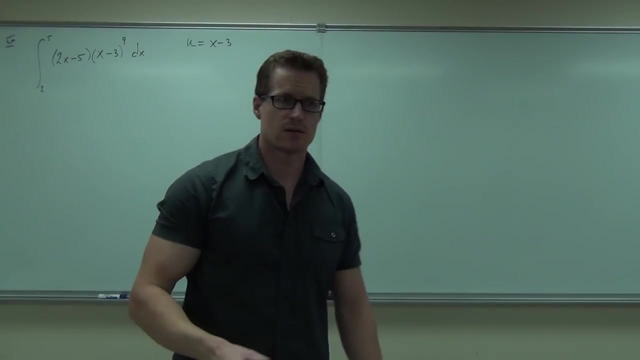 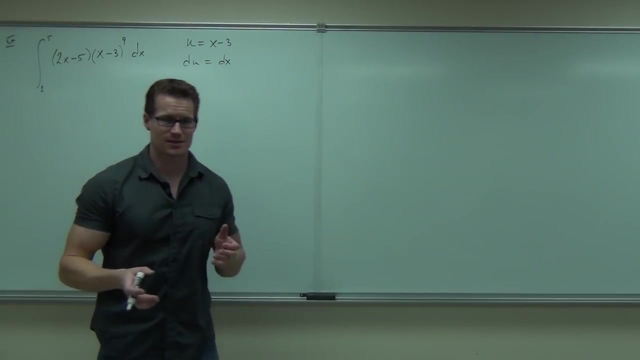 that we take. Okay, well, that's all well and good. U equals x minus three. what do we do after that? Minus the derivative, This is pretty easy. in this case, D? u equals d? x. Hey, that's nice. 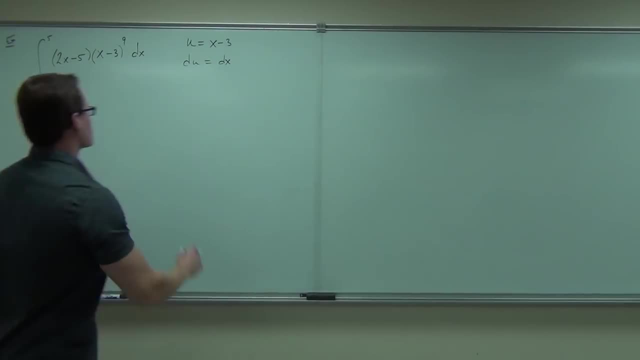 That's a direct substitution from d? u to d x. However, when you look at the problem, we go from two to five. we're gonna change this in a second. by the way, I just wanna make sure the substitution is going to work. 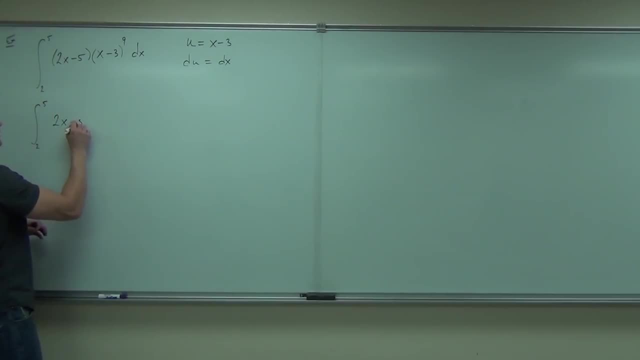 before I start changing bounds and doing things like that. I don't wanna waste any time. I still have a two x minus five, and here I'm gonna have a? u to the ninth, and my d? x will be a d? u? U to the ninth. got it. 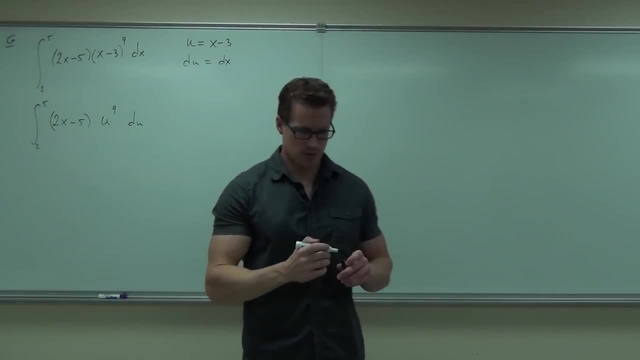 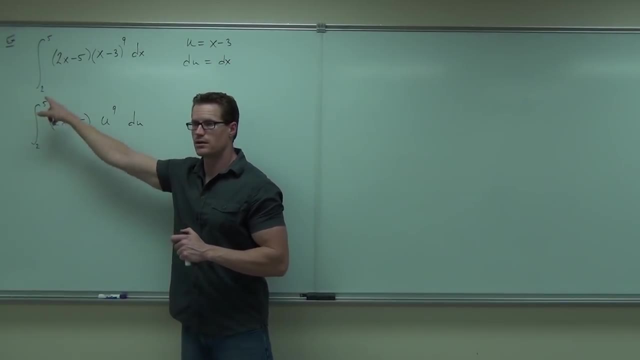 D? x is d? u got it. What's the problem? There's still an x. That's the problem. You have a d? u, but you also have a u and an x, and these are still in terms of what? X. 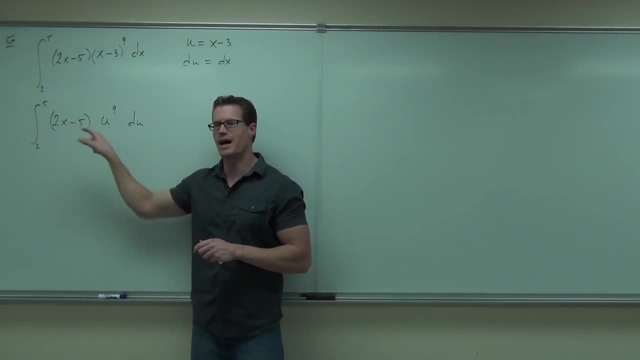 Those are in terms of x. So if we can make the substitution work, I'm gonna go back and change the bounds, but I wanna make sure it works first before I waste that time You got me When this happens to you- and it will- 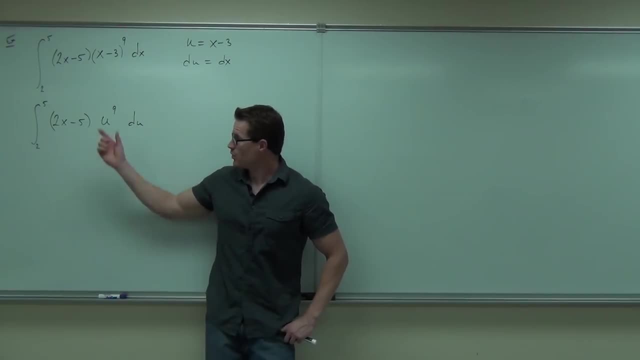 when it happens that you make a substitution and you know you made the right one. if you made this one, that certainly wouldn't work in d? u y shape or form. but if you know you made the right one, you go. wait a second. 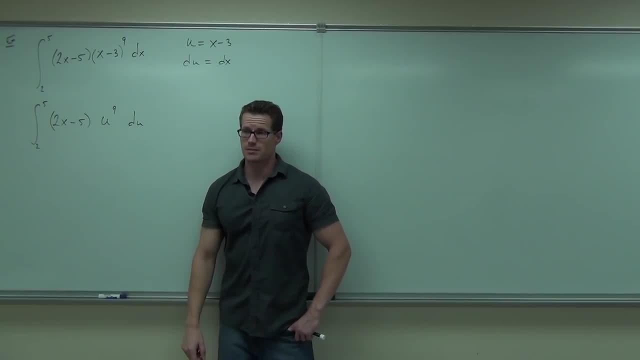 that's not falling out of my integral anywhere- Sometimes- sometimes not all the time, but sometimes- it means that you have to manipulate the substitution to solve for x and substitute n for x, and that's sometimes what it means. So when we have 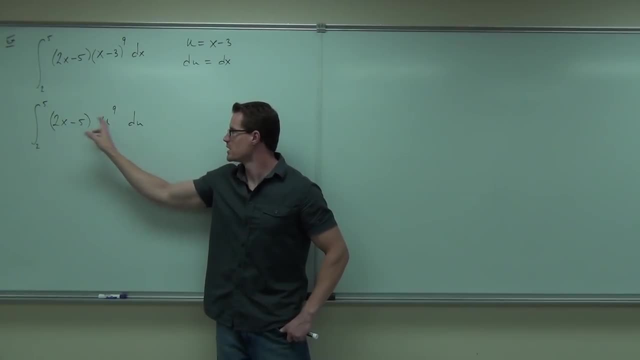 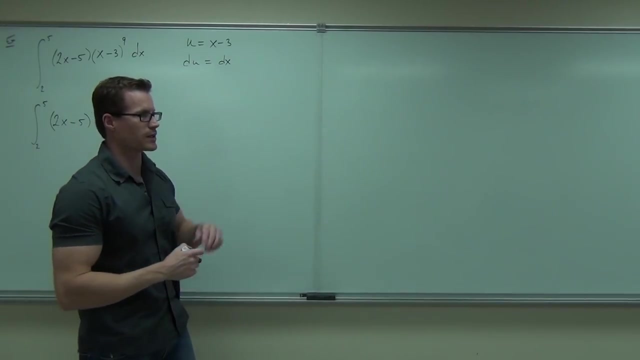 especially when there's no power or anything. you can do that oftentimes and we'll be able to distribute later. So it says: okay, u equals x minus three. can you solve that thing for x? How would you do it? 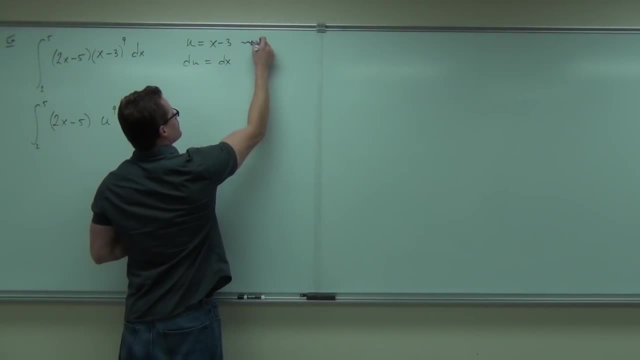 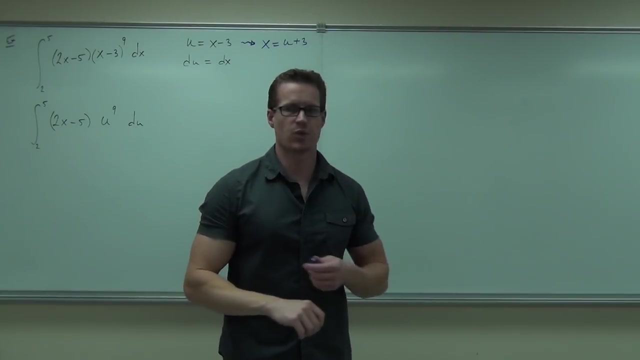 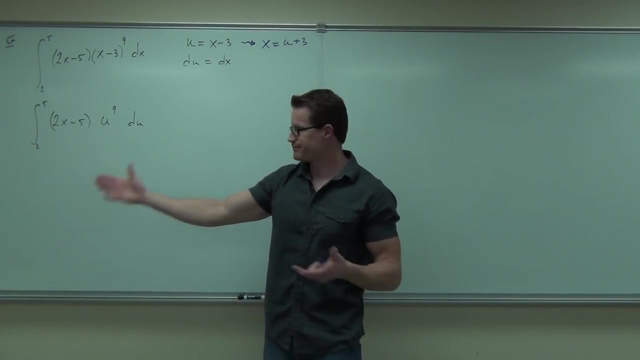 Absolutely. Very good, Then what you say is all right. then x is u plus three, correct? Now we can make the substitution instead of x. hey, what else could I write? U plus three plus three. Let's do that. 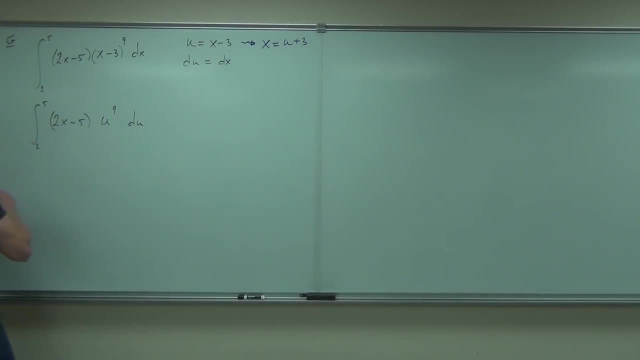 Then it changes everything into u's. So our integral- I'll do the bounds in just a second- Our integral is two. what else Parentheses? Parentheses: u plus three- I like it- Minus five, And all that wow. 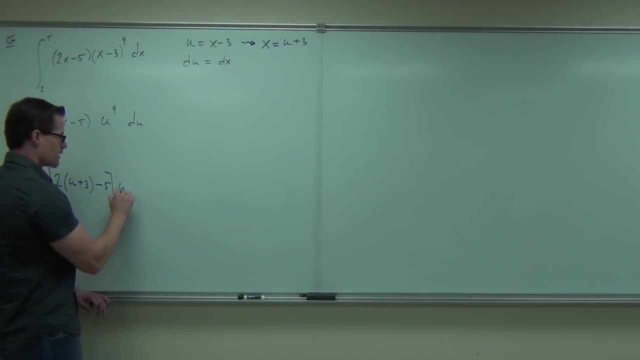 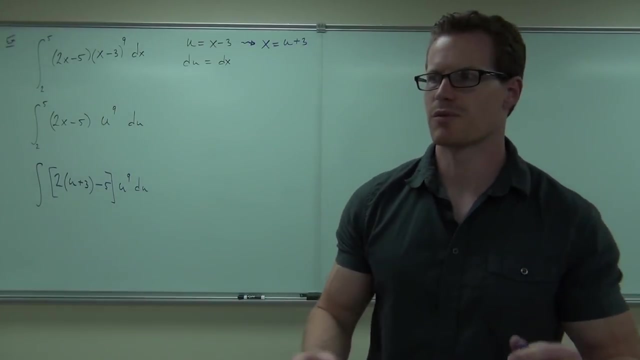 Yeah, Big old bracket, because you're still multiplying by u to the ninth. Well, let's see if we can all follow that. Do you see where the u plus three's coming from, ladies and gentlemen? So we're using the substitution we just made. 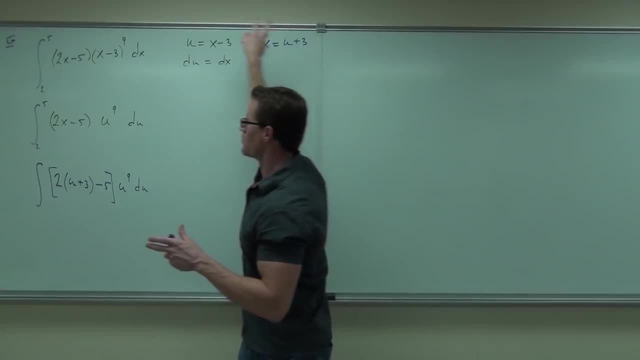 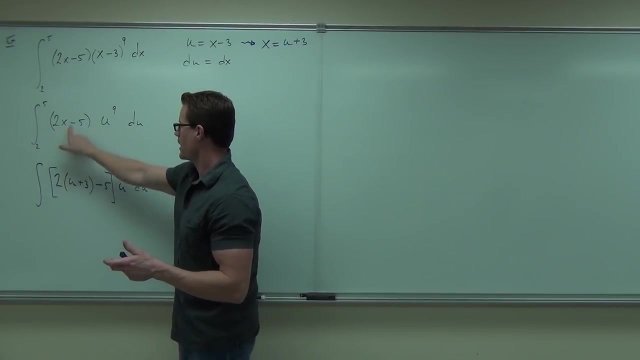 to solve it for the other variable. solve it for x. That way we can substitute that in and it changes everything into u's and that's great. So we change that into a u. We have two, that's u plus three. 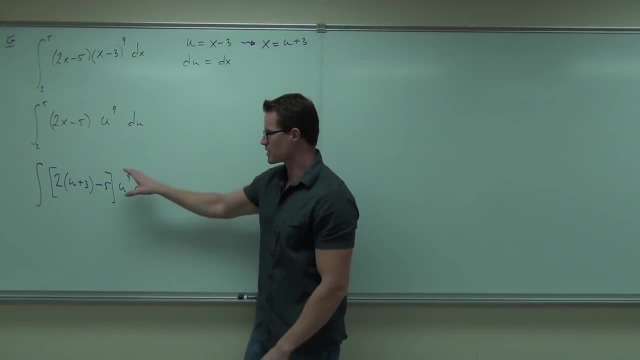 And then minus five. The whole thing's still being multiplied by u to the ninth. so I still have to have that bracket Now at the same time, since we're now all, in terms of u now's, where we probably will at least change our bounds. 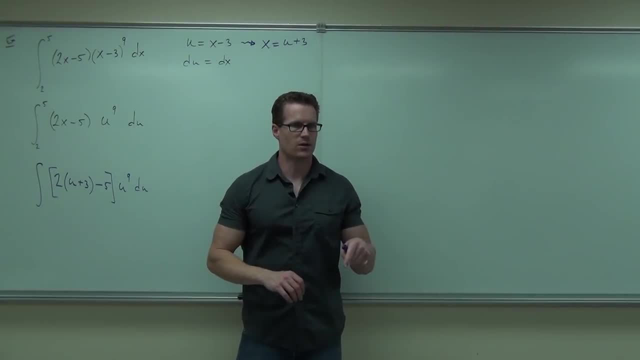 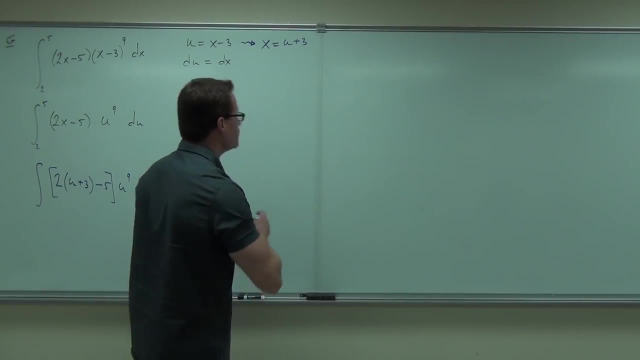 That'd be a good thing to do, So why don't you go through right now and change your bounds for me? I'll do it on the board as you're doing it, but make sure you can do it. Don't just follow what I'm giving you. 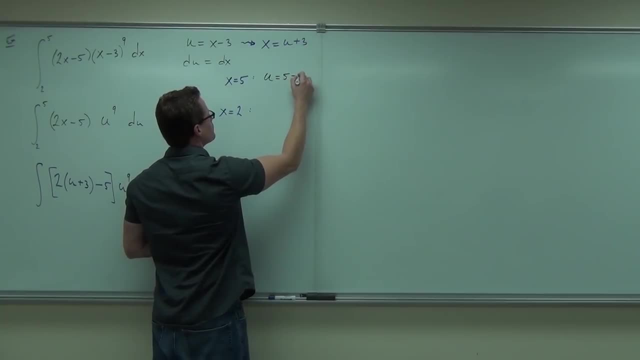 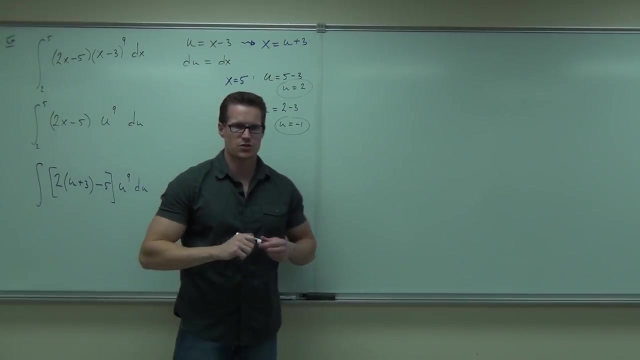 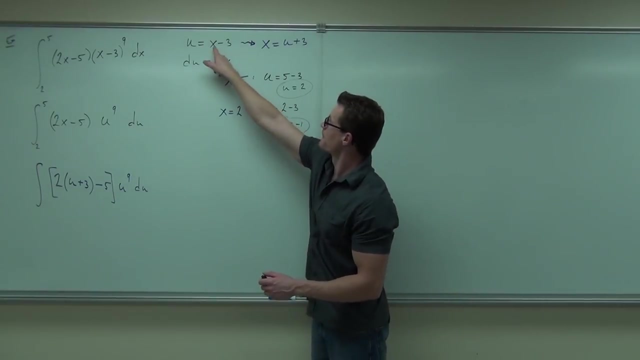 I'm pretty sure I got two and negative one. Did you get two and negative one? All right, so let's change our bounds down here Instead of going from two to five. we know that if we plug in five, we're gonna get two. 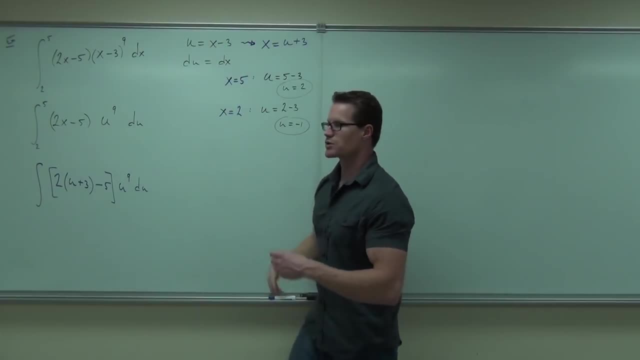 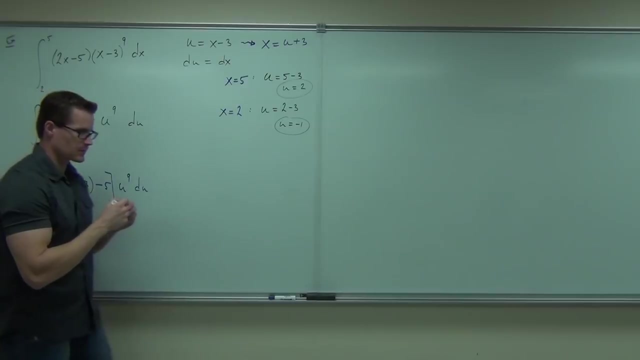 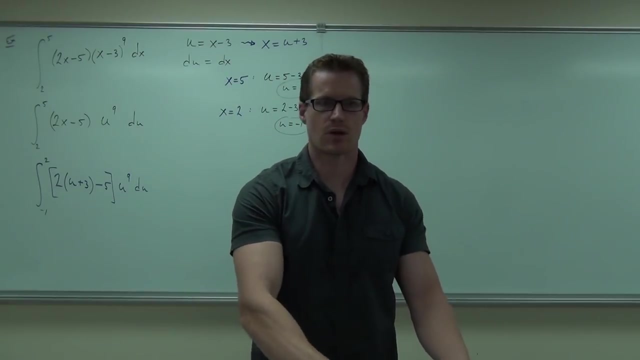 We know if we plug in two we're gonna get negative one. So that changes from two to five. That makes it negative one to two. Now a quick question just to refresh your memory: When I get down to the very end, am I going to have to substitute back in for x or not? 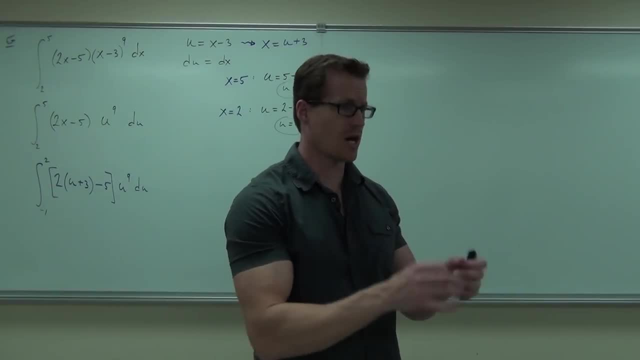 No, Because now I'm in terms of u, and that makes it nice. So at the end we're just done. We just have to plug the numbers in. That's why we changed the bounds in the first place. Okay, hey, what next? 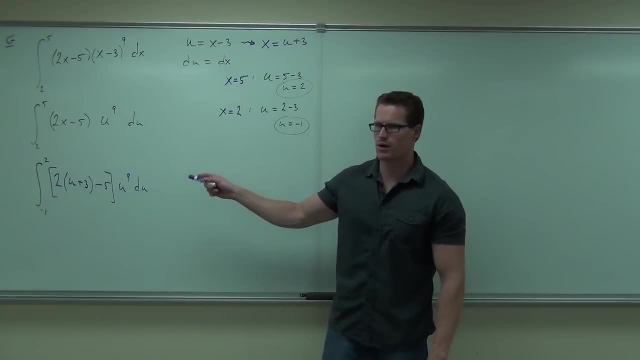 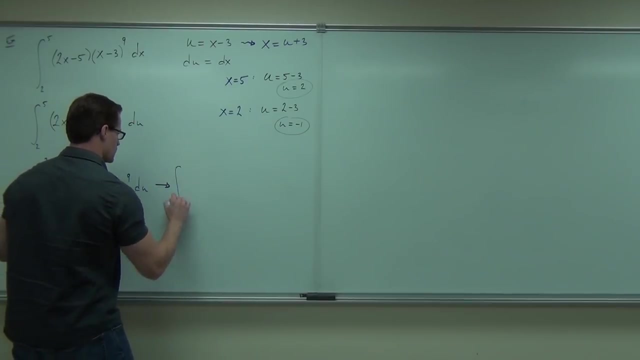 Come on, we're on the roll. You don't agree Before? I don't wanna integrate right there. You wanna simplify all that? Yeah, Distribute out your two and then add up the minus your five and then multiply by u to the ninth. 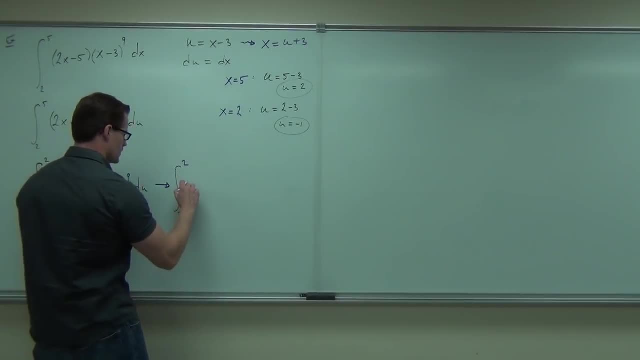 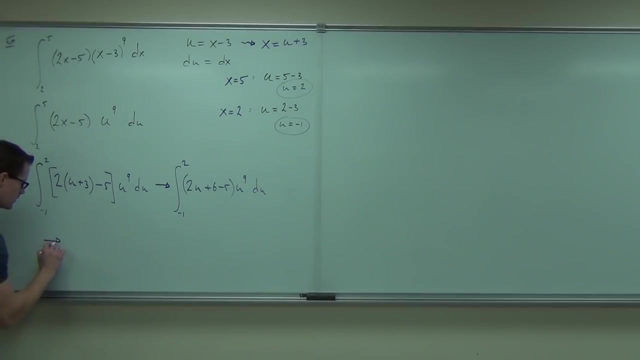 Yes, we call that tedious algebra work. Ah, two u plus six minus five. Then u to the ninth du: Two u plus six and then minus five. Okay. well, that means we'll have two u plus one, Okay. 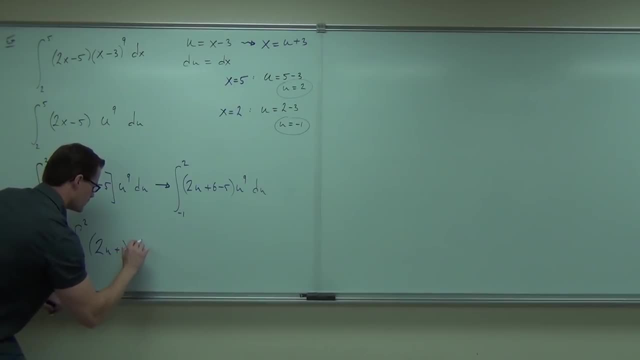 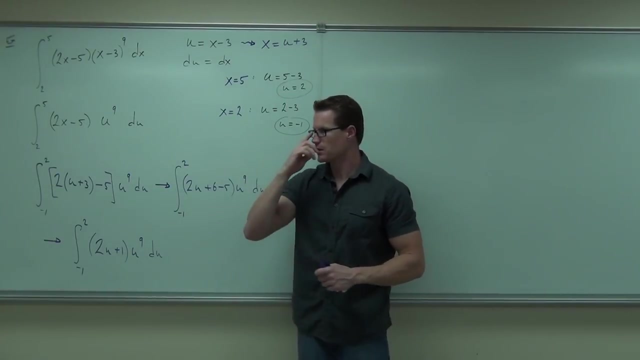 Now, let's try to do this. I can't do it. I don't know how I'm gonna try to do it. I'll try to do it. Tell me something about this integral, what I absolutely have to do in order for this to work. 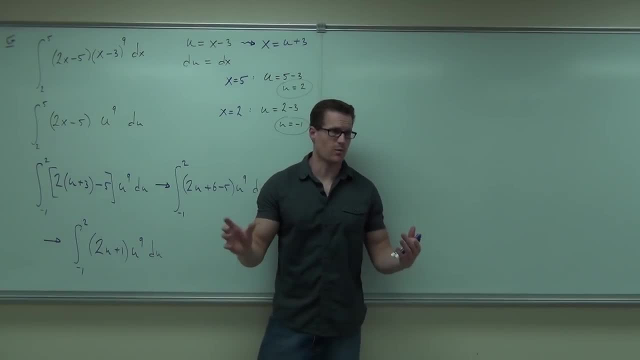 Got it. I cannot just integrate the way it is. We found out that we can't separate integrals by multiplication. The only way to accomplish this is to distribute, and then we do the integral piece by piece. So when we distribute, please note that we're gonna have same bounds, of course. 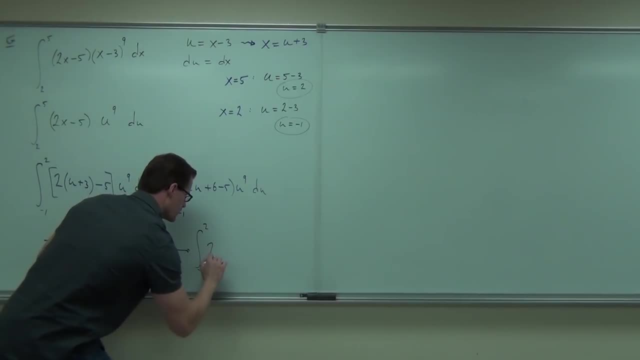 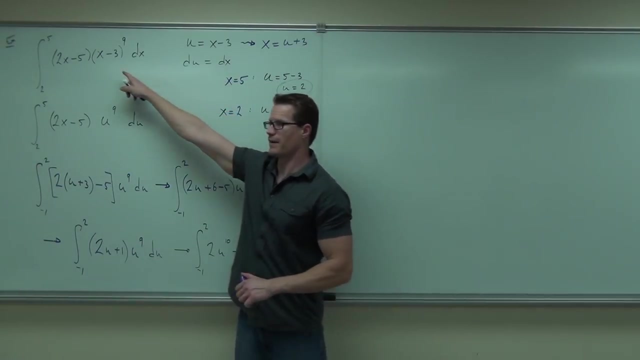 We'll have two u to the what to the what, and very good, do you? hey? that's a whole lot easier, that's a whole lot easier to integrate than that one that looks almost impossible. if you really, if you didn't have this to follow you, go wait a second. that substitution. 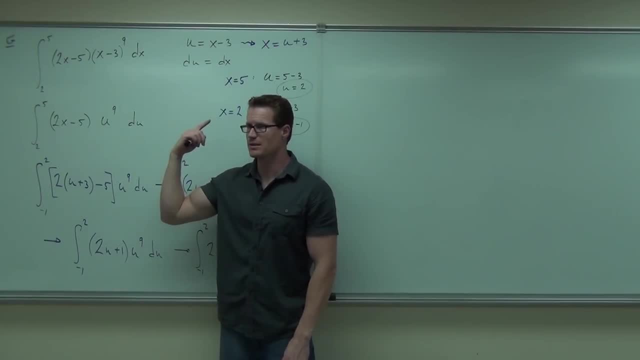 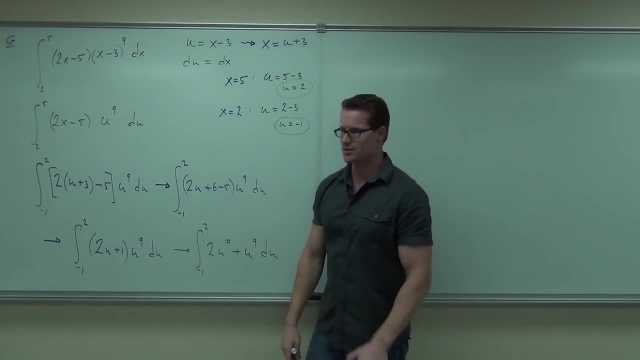 won't work. try one anyway, see if it will work. see if you can manipulate like I did, then maybe it will. if that's the case, shoot. it makes it a whole lot better to work with and your bouncer you can change, so that's even nicer. so now, 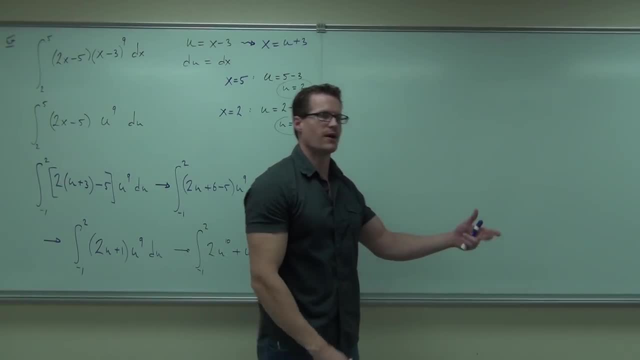 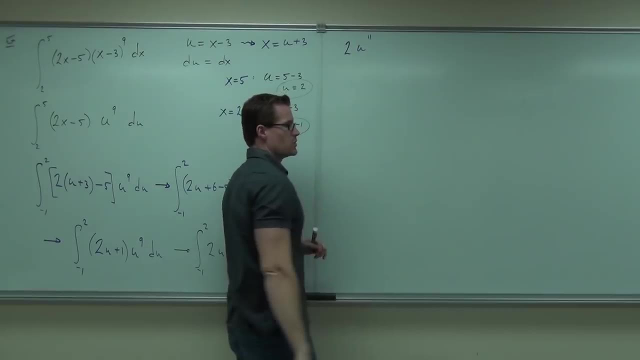 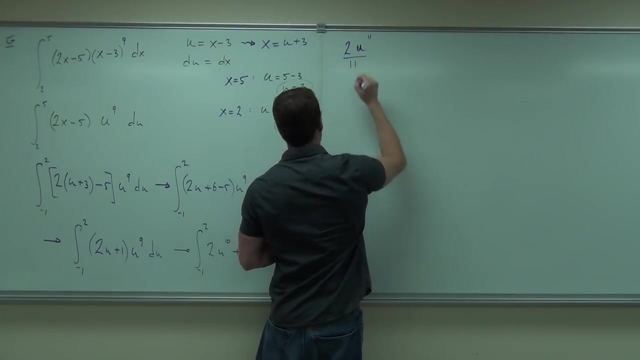 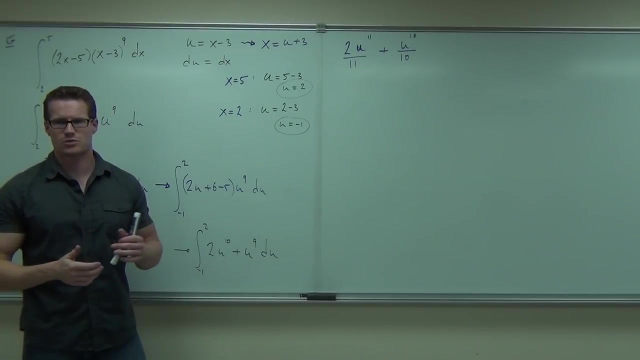 we're going to integrate. let's go ahead and integrate and then we'll evaluate. so our integral is 2u to the 11th over 11 plus u to the 10th over 10. are you guys okay with the integral? some of those integrals are pretty nice right. 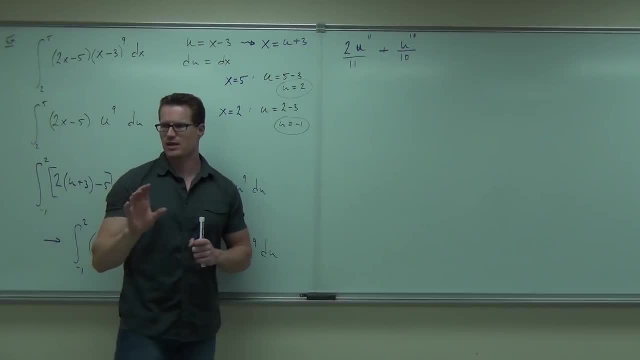 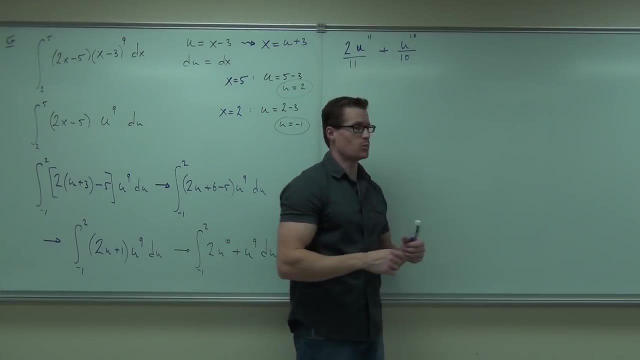 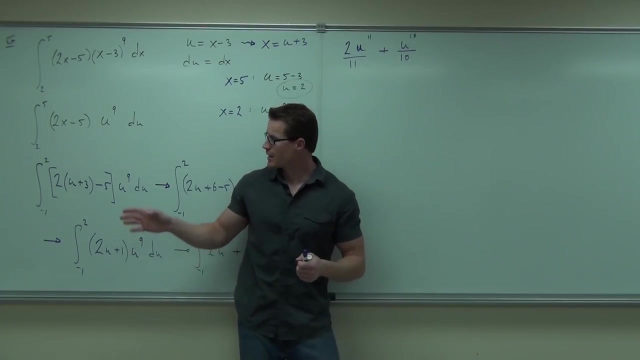 just take the basic stuff in substitutions. that's. that's what substitutions supposed to: supposed to make your integral easier, not worse, easier, as it definitely does make it easier. now, what do we do? good, because we change the balance. first, we know that our balance are in terms of you, not an. 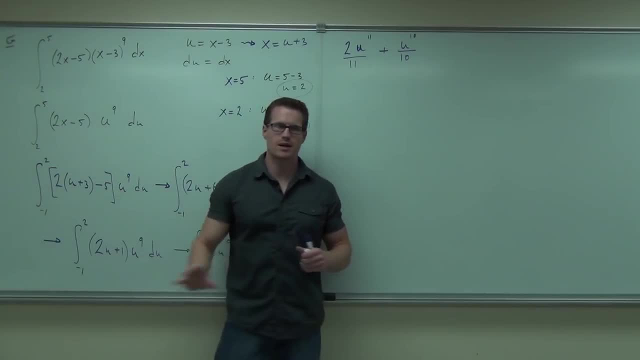 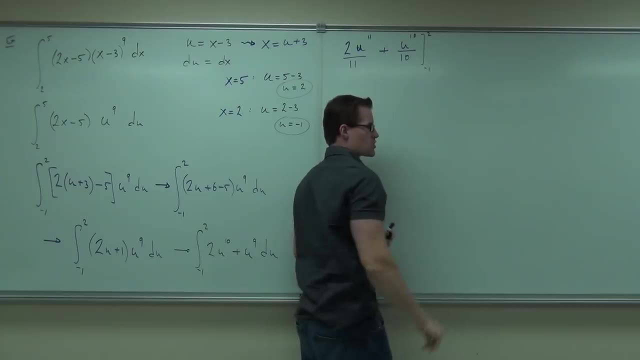 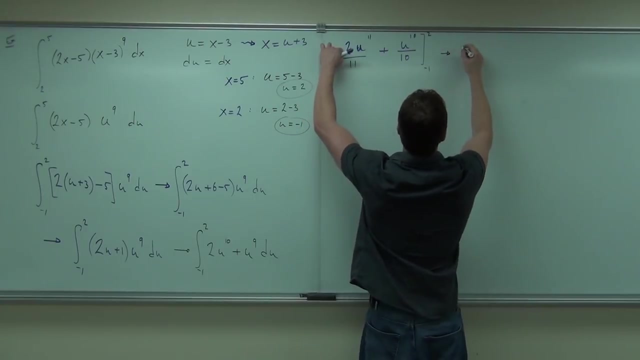 X anymore. these were in X's, those are in use. so as soon as we get out of the very end, it's now evaluation time. just make sure you evaluate very carefully. we're going to get two times to the 11 over 11, to the 10 over 10. that happens. 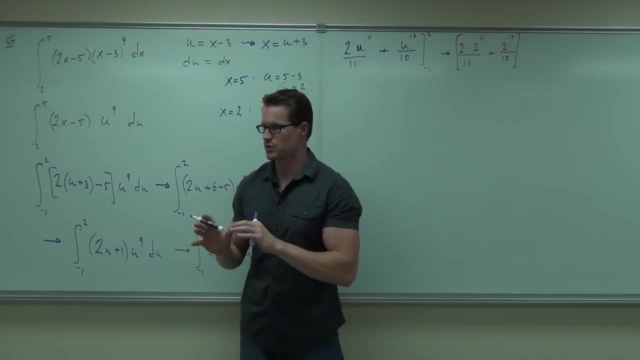 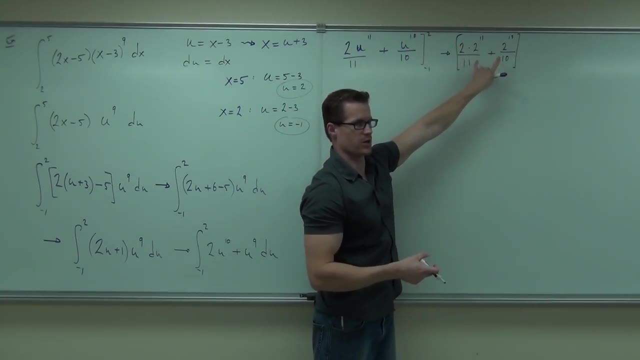 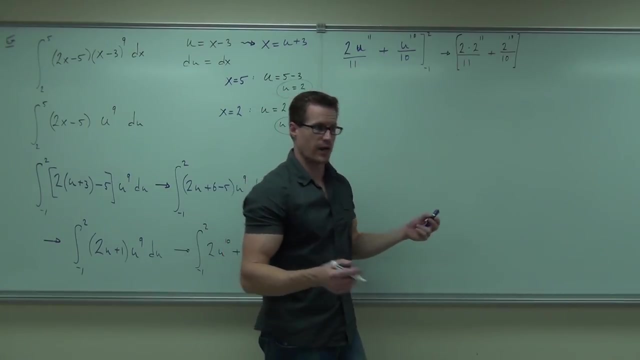 from when we plug in the two, you get it. plug into both those those terms. it has to go to both of them. so this, this piece right here, is just the two evaluated. are you all right with that? so far, yes or no, ladies and gentlemen? yeah, okay, then what do we do? subtract: all right, you gotta do that and we'll plug. 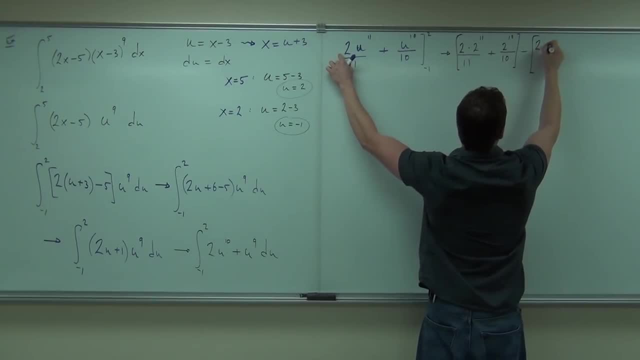 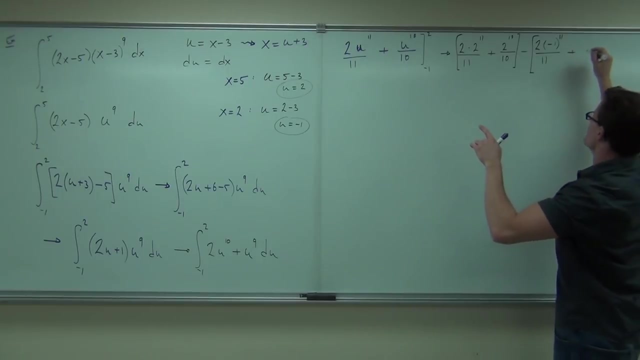 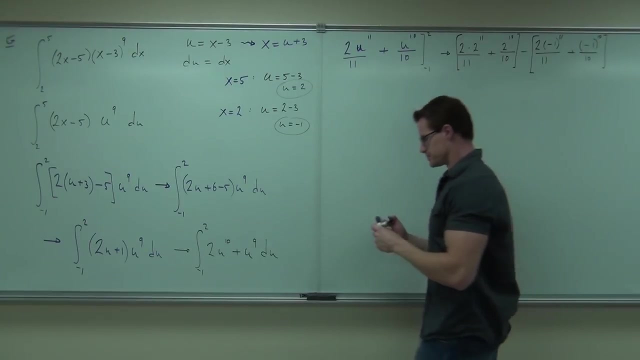 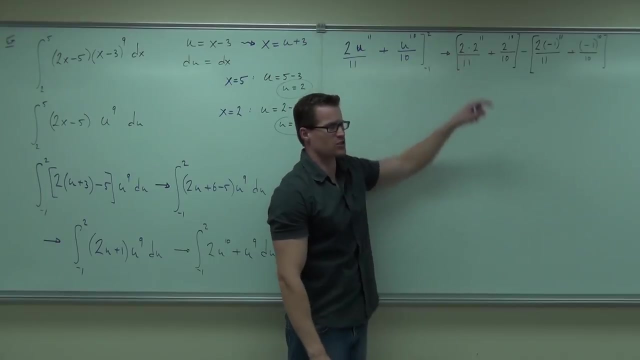 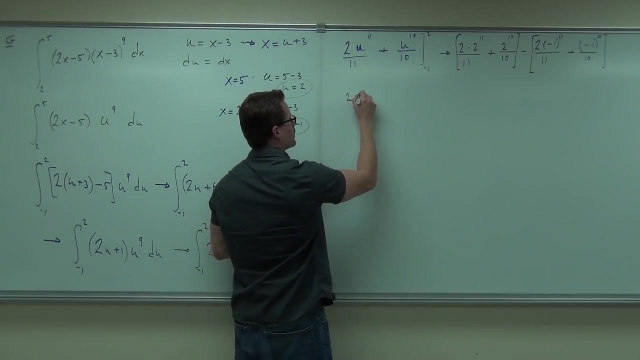 in the negative 1, 2, negative 1 to the 11th over 11, plus negative 1 to the 10th over 10. oh my, how much is 2 to the 12th? because that's what that is. that's 2 to the 12th, 2048. okay, I'll believe you. 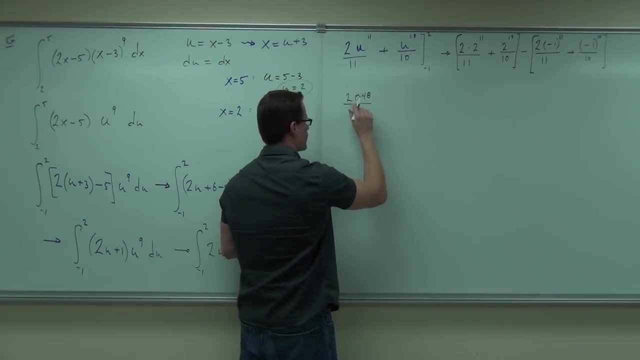 you, I meant 2 to the 12th, not 2 to the 11th. 2 to the 12th, 4,096. okay, because 2 to the 12th, 2 times 2 to the 11th, is 2 to the 12th. so you either do 2 times 2 to the 11th times 2, that's going to give you that, or just 2 to the 12 gives you that plus 2 to the 10th. 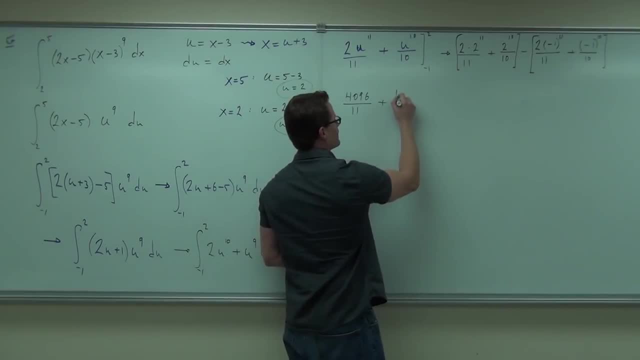 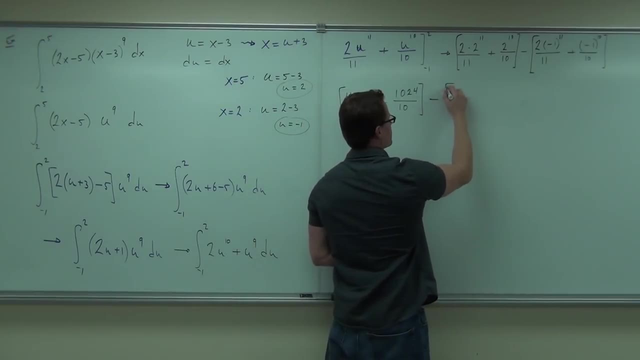 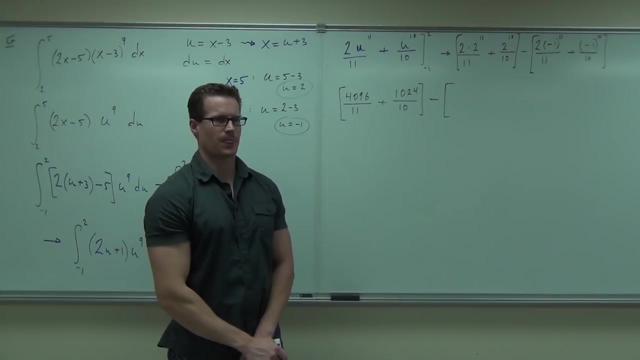 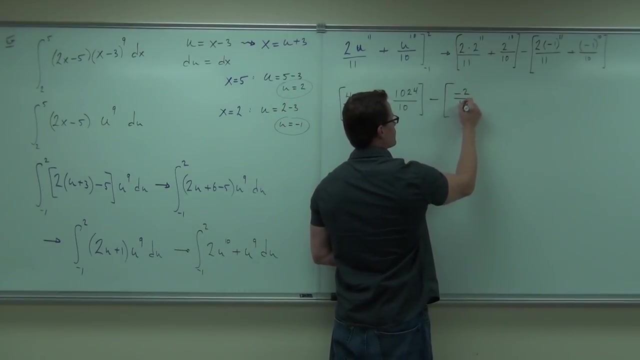 1000. okay, all right, minus well, 2 times 1 negative. 1 to the 11th, negative 1 to the 11th, just negative one. get that odd exponent up there's, get me negative. so this is negative 2 to the 11th that. 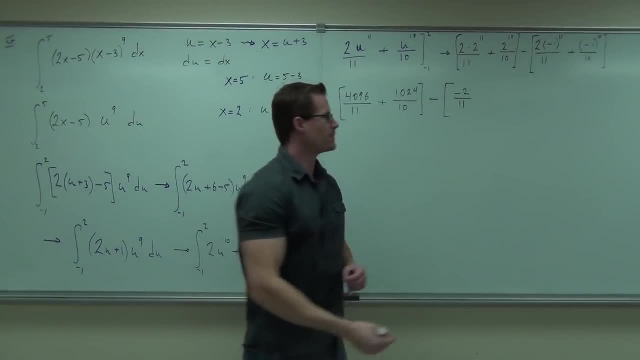 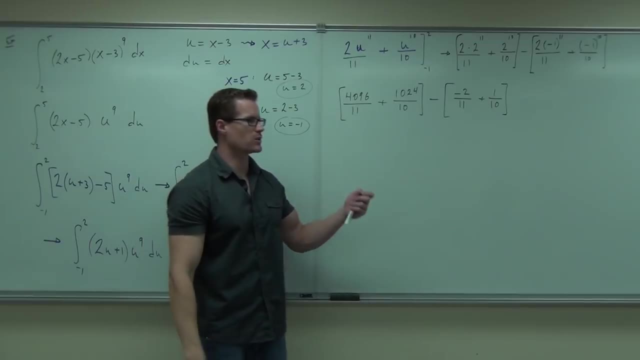 though that's a negative to the 10th power, that's gonna be positive 1. this would be plus 1 tenth. I'm going slowly so you see where all these numbers are coming from. Can you follow the fraction work? 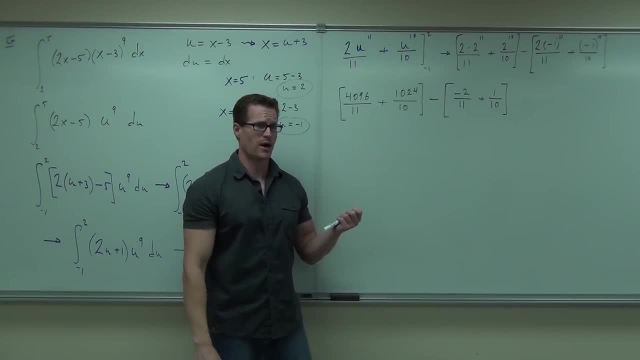 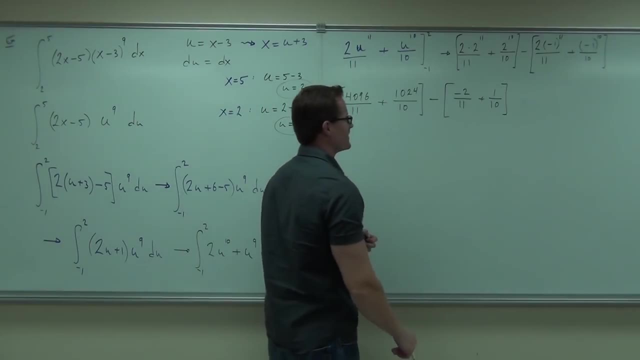 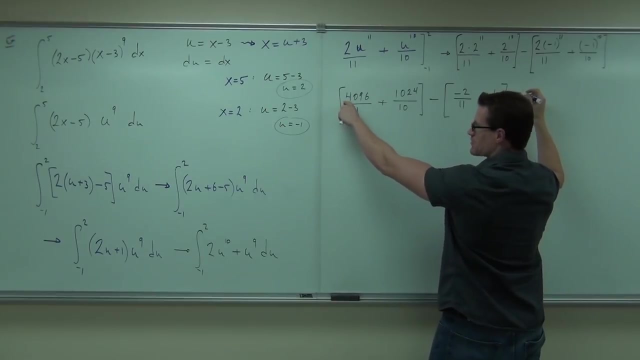 I know fractions are not your favorite thing, but it's Friday, right? What happens on Friday? Fractions, Fractions. obviously It's a fraction Friday. Okay, so we've got 40.96 over 11 plus 10.24 over 10.. 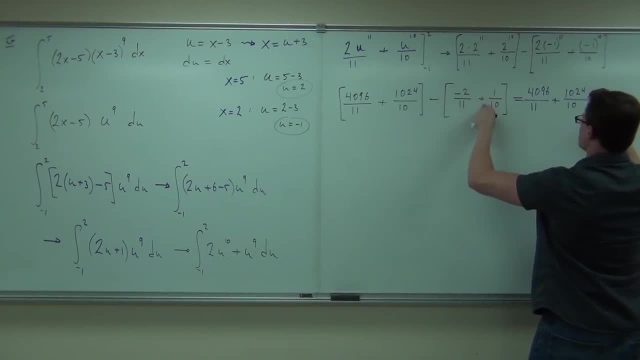 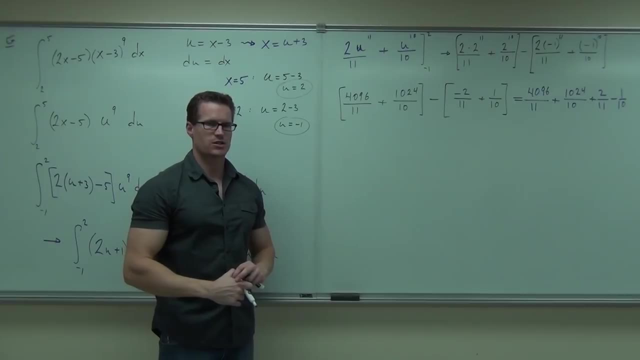 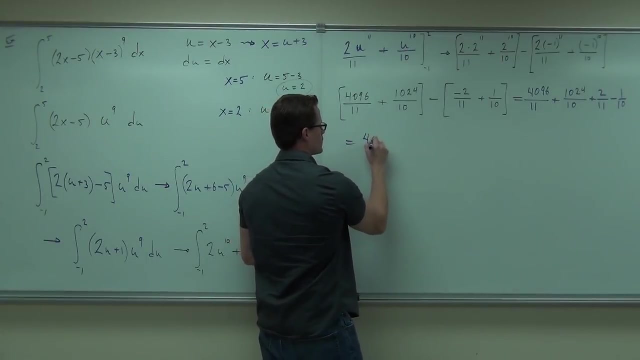 Plus 2.11, minus 1.10.. So far, so good on sign changes. All right, We'll combine some like fractions. We've got 11ths and 11ths. That's going to give you 4,098 11ths. 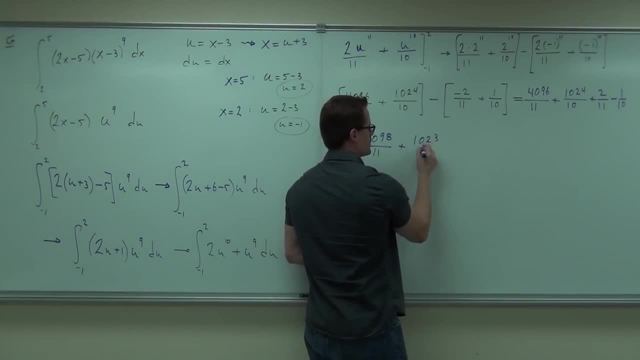 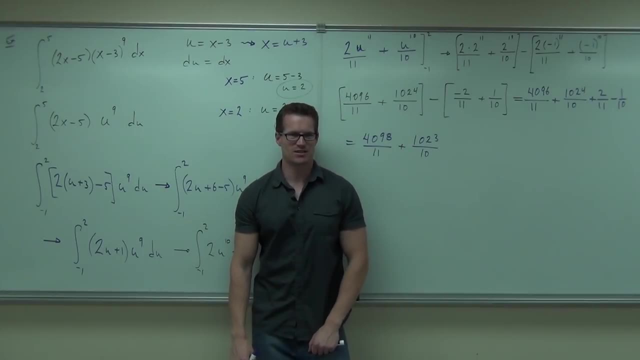 That's going to give you 1,023 tenths, And then you're going to find a common denominator- Oh All right- Which is 110.. 110. Probably, yeah, 110.. I don't want to do that. 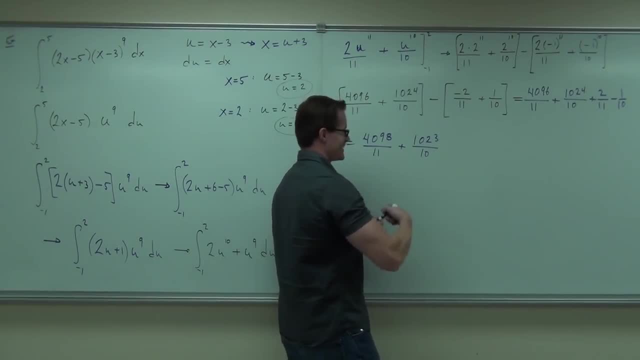 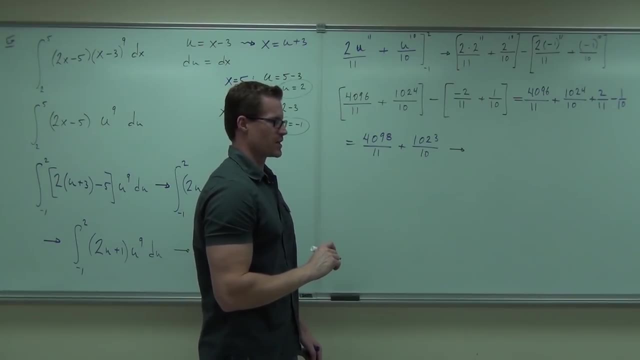 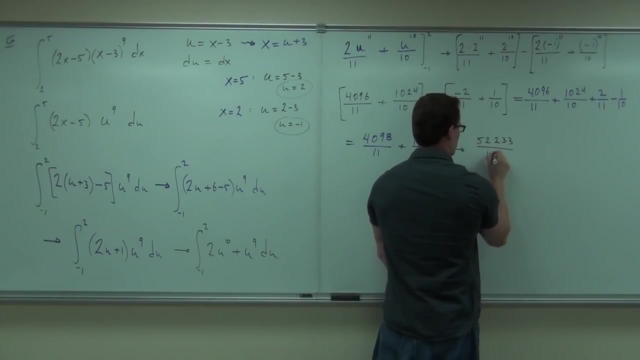 It's 52,233, 1 tenths. Wait, 52,233.. Over 10.. Over 1 tenth: That's the simplified fraction: 2,233 over 1 tenth. Yeah, That's it. Awesome, I mean, that's easily relatable, right. 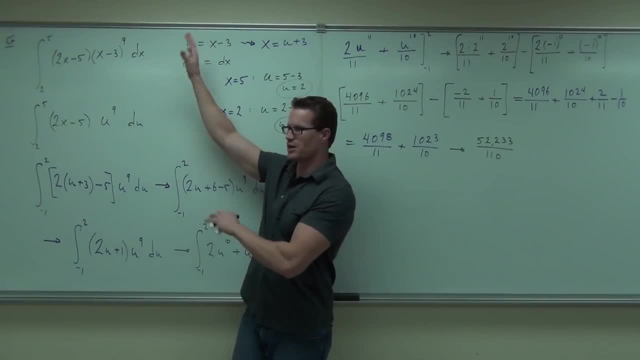 Now, of course, what is this that we just found? Don't get confused with all the mumbo-jumbo. What are we doing? An area, That's an area. Could you find a decimal equivalent for that? Yeah, If you had to actually give an approximation. 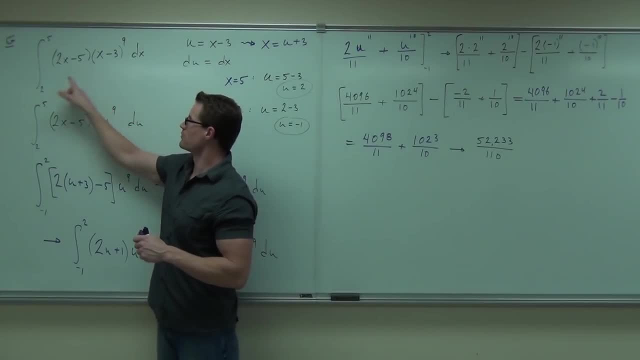 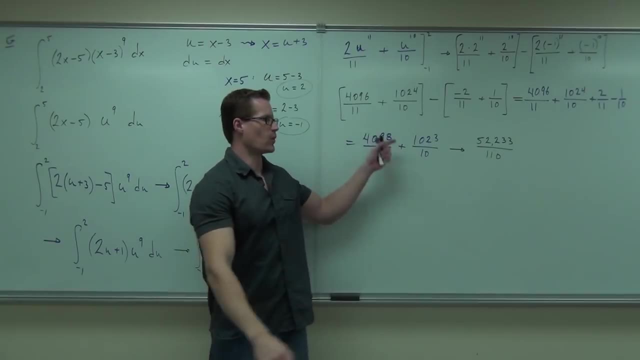 for area you could do it. That's the area under this curve between those numbers. That's what that's doing. How many people feel okay with that? Your calculator will do a lot of the fractions for you, so don't let that hold you back. 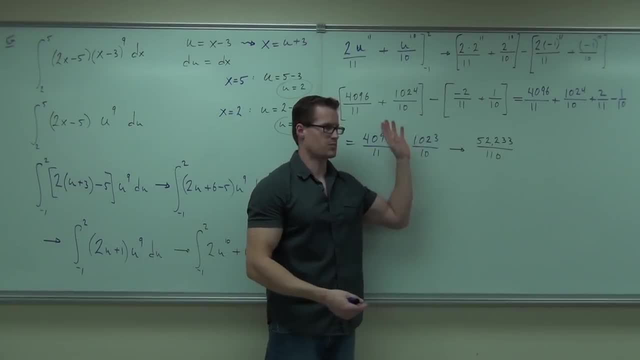 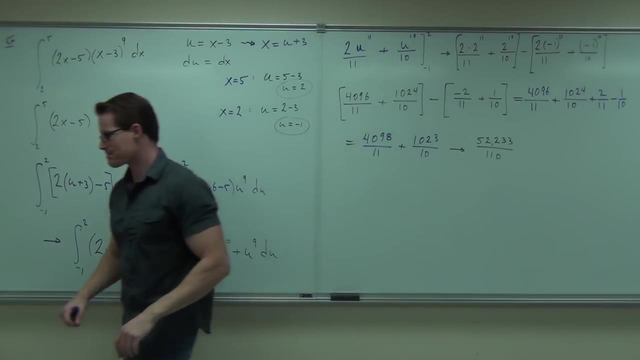 If you can get it down to here, your calculus is done. Evaluation: that's actually pre-algebra. We're doing all that stuff now. The numbers in pre-algebra aren't that big, but you can do it. You ready for one more? 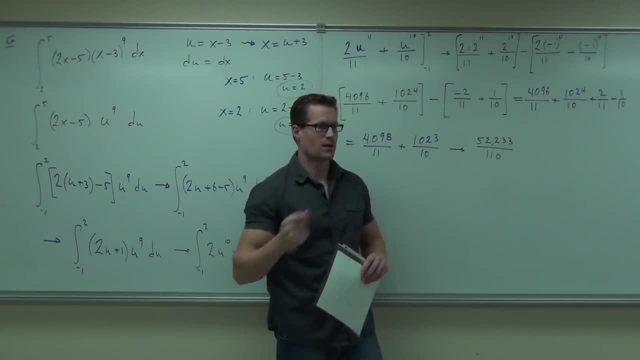 Yeah, Any questions on this one. before we begin, Your face says question. Well, yeah, Your mouth doesn't. I got to that point where I messed up my evaluation and tried to figure out where am I? Well, in fact, I screwed up. 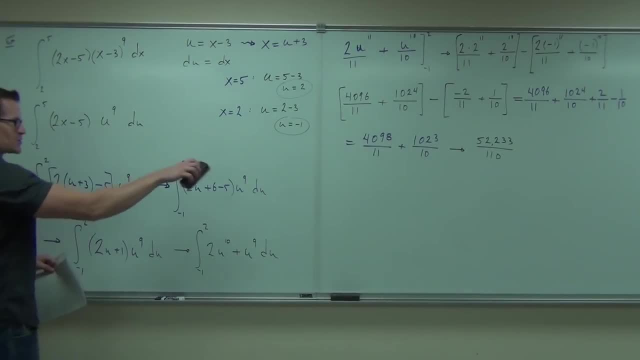 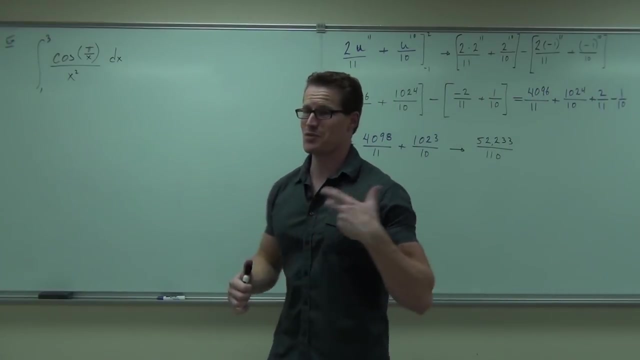 Got it. I'm going to say that's on you. Yeah, I'm going to give you a minute of blanks. Okay, okay, Okay, granted, this one doesn't look fun. It really doesn't look fun. It looks fun to me. 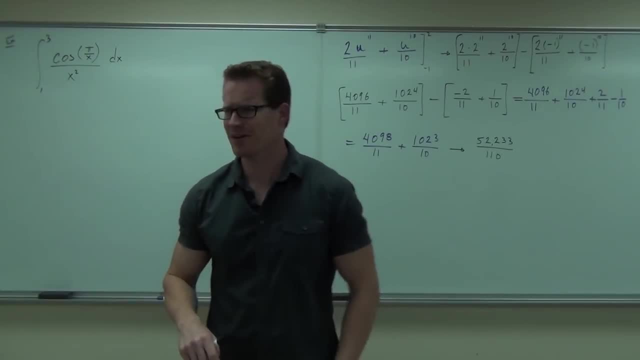 I love this stuff, but it may not look fun to you. Why does it look fun? Trig, Trig, Trig. Yeah, trig always throws you guys for a loop. You go: oh, trig, seriously, Oh, I hate trig. 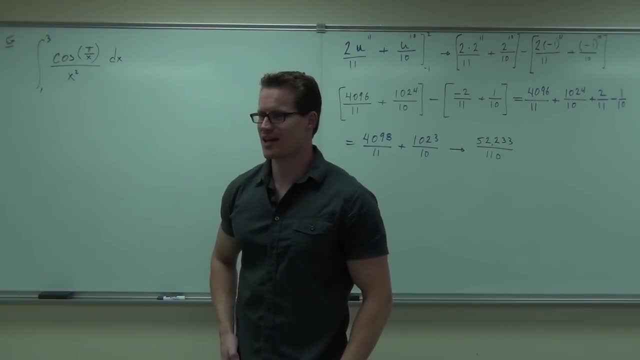 Too bad. Second, it goes, man, it's not just an x in there- which is actually fortunate, because you wouldn't be able to do the problem if it was- But it's a pi over x, And then it's over x squared. so there's a lot going on. 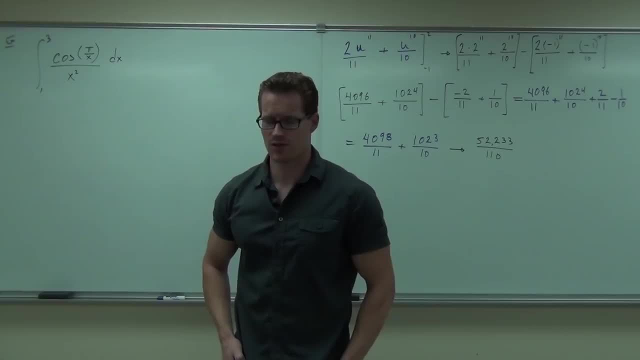 It certainly doesn't fit the integration table. One question I have for you that's going to kill me. if you get this wrong, It really my head's going to explode on the camera screen And then no more videos. So don't do this to the people at home watching me. 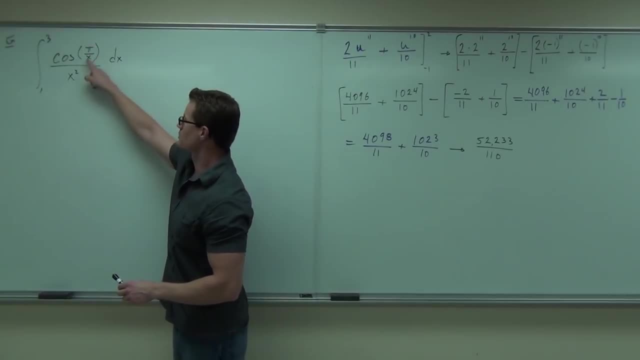 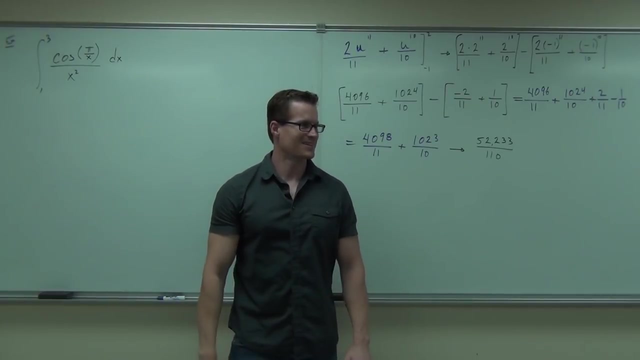 It would really suck. But let's see, Can you combine this with this And get- oh good, good, It's not cosine of pi over x cubed right, Right, Yeah, it is And gone? No, it's not. 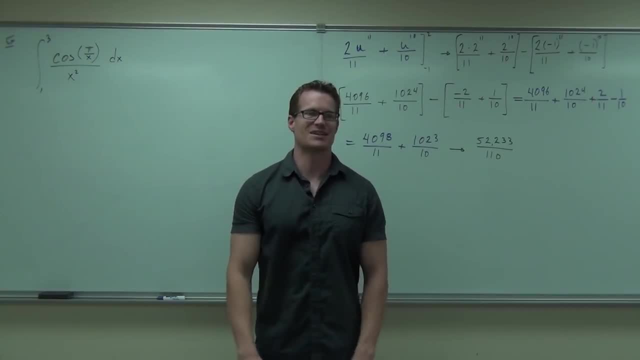 It's not that. Then you'd get cosine, Cosine of pi. that'd be very easy in the grill. That's not the case, though. This is an angle over a function of x. That's what that is, So we have to somehow use a substitution. 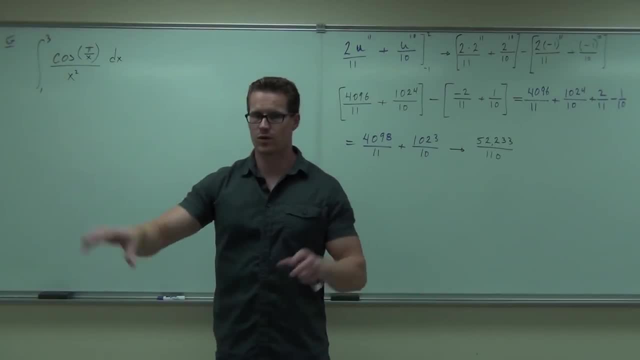 That's the only thing we have in our arsenal Right now. we have direct fit or substitution. Later on you'll get a lot more. okay, That's your next class, But right now that's two things we could choose from If it's not a direct fit and we can't combine things. 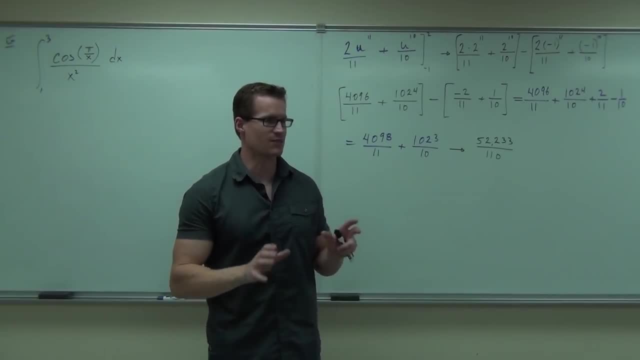 like we cannot do here, then it has to be a substitution for us to even do it. If a substitution doesn't work, then we are SOL. Sorry, out of luck, You can't do the problem. Anyway, let's go ahead and let's look for a substitution then. 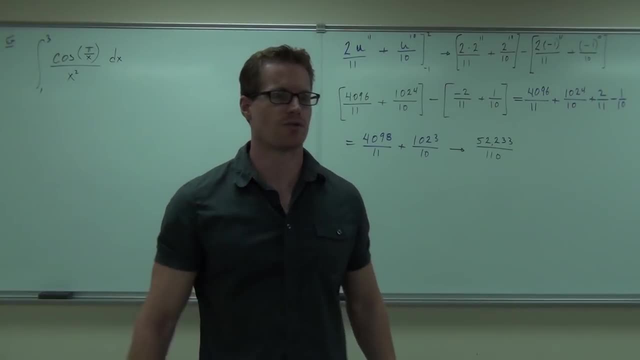 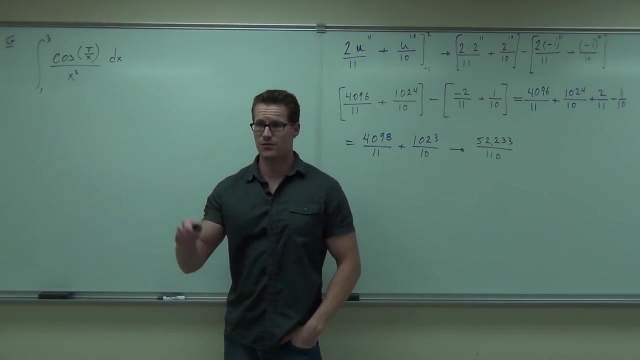 True or false. the substitution should include the cosine: True or false, False. Why? Because then you take a derivative of the cosine right And that would give you negative sine. Does negative sine appear up there? That is probably not the right choice. 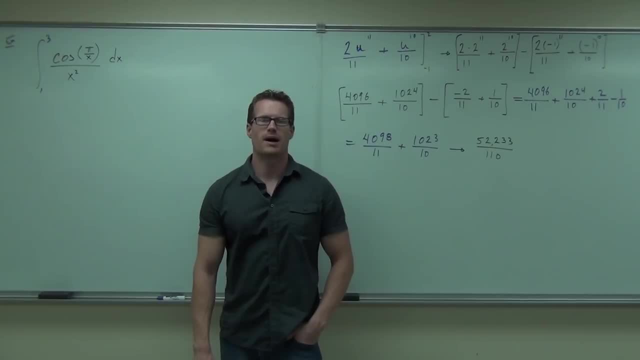 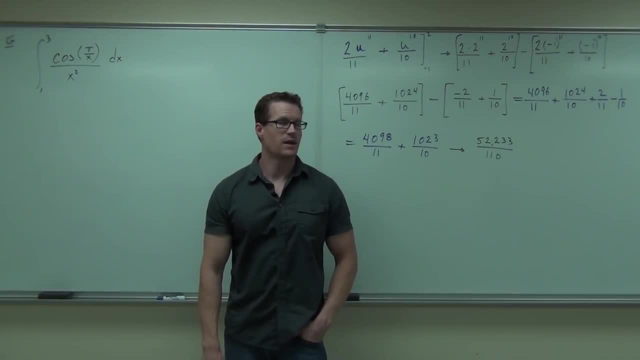 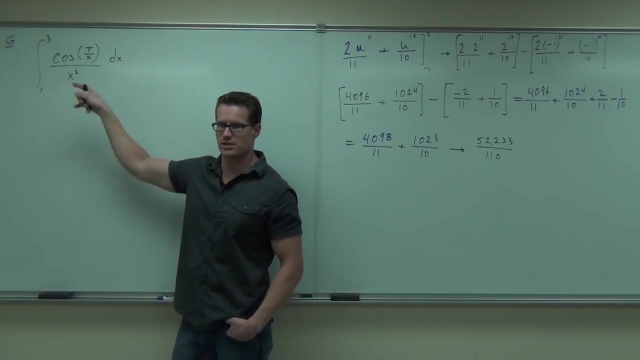 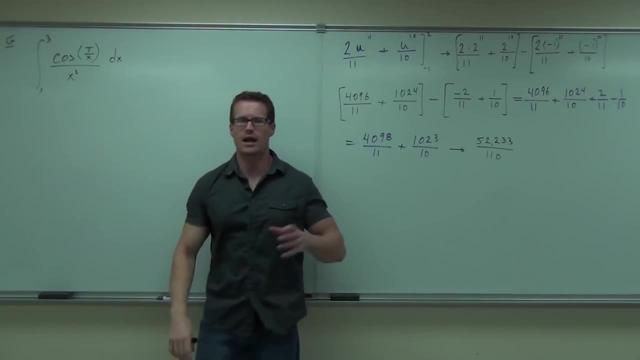 So even had you taken that as a? u, it's still un-symplified. you cannot go inside of that cosine like that unless you have one of the like double-angle, half-angle, Pythagorean theorem identities. to break up things. 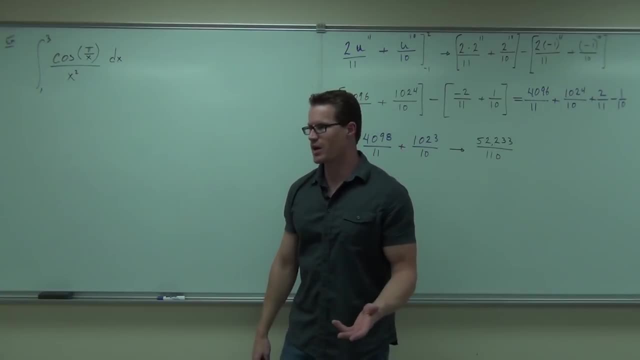 You cannot do it, And so the only option we even have is pi over x. So take a substitution of u equals pi over x. Go for that right now. Take your derivative, if you can. You know how to take derivatives, So we've passed that portion. 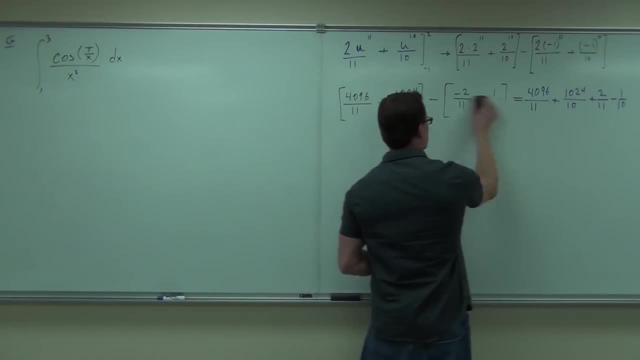 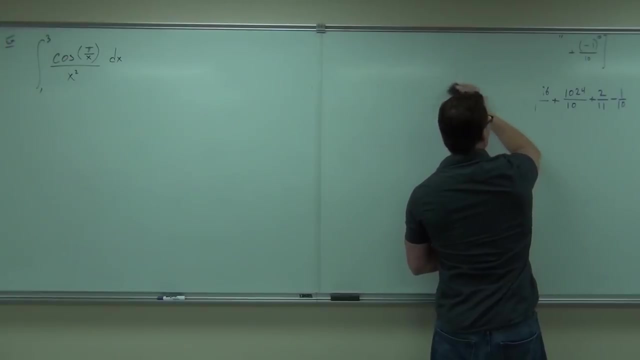 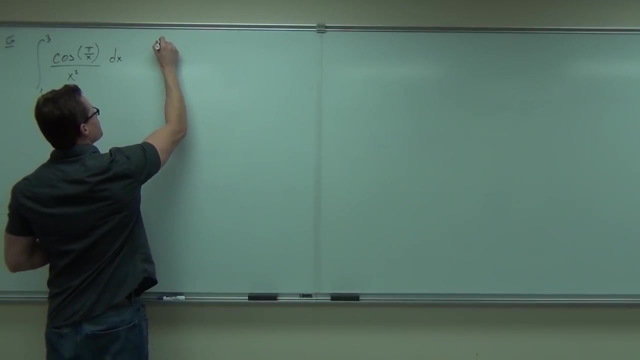 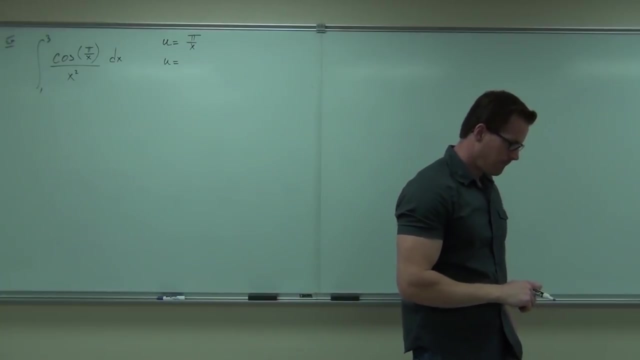 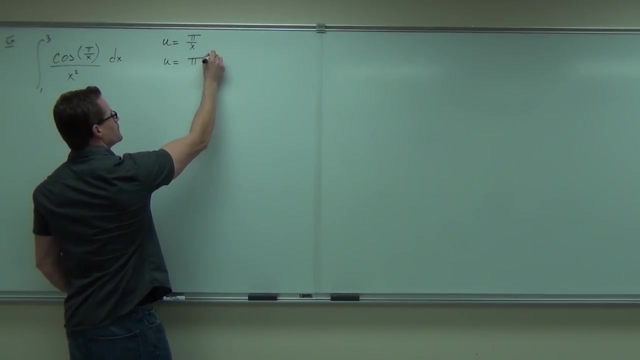 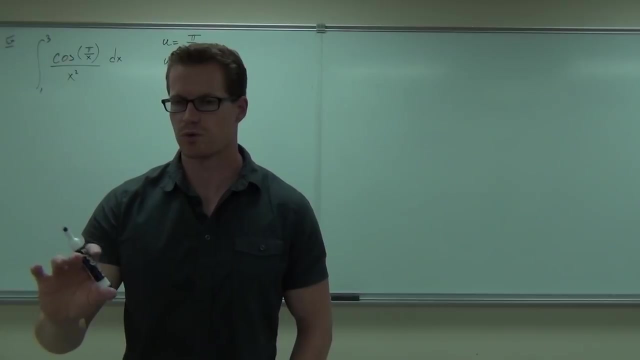 So take your derivative. Also, I want you to change your bounds right now. Notice, to take a derivative. you have to do that. You've got to bring that x up to the top to take that derivative. Did you do that? Unless you want to use a quotient rule which you don't, 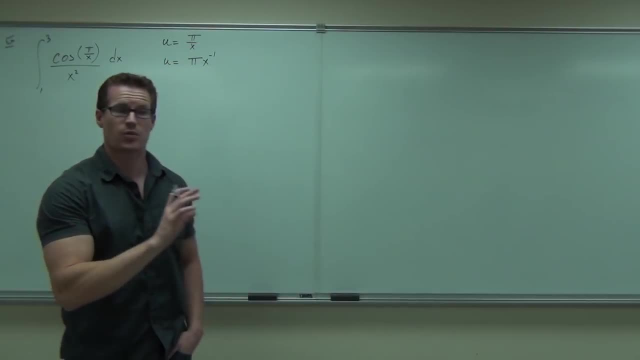 Trust me, Pi is a constant. You don't want to use a quotient rule, But this is not a product rule either, because pi is a constant. It's like the number 4.. It's like the number 2.. You don't have that here. 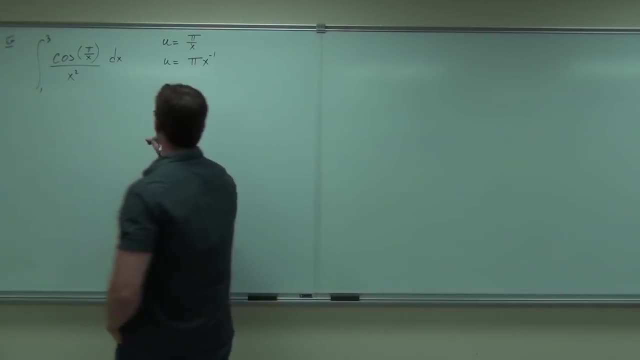 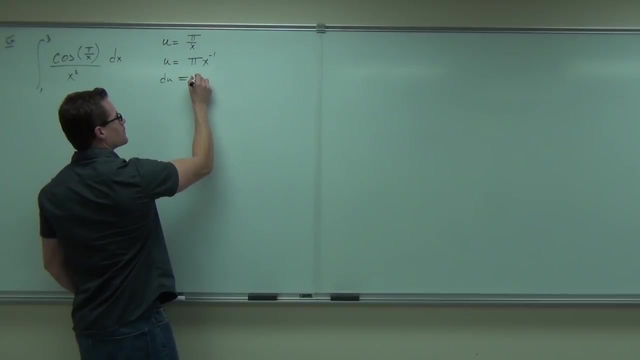 So if we take a derivative of u, We take a derivative with respect to x. on this side You're going to get what? Yeah, I'm going to do it in two steps. You see the negative pi x to the negative 2 dx. 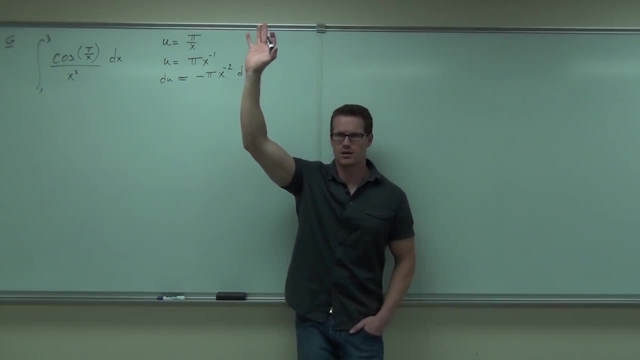 Are you guys OK with that? How many of you have made it down that far? Which one half you did Good. At least you didn't forget how to take derivatives, right. So we know how to take a derivative. And how are you supposed to solve for dx. 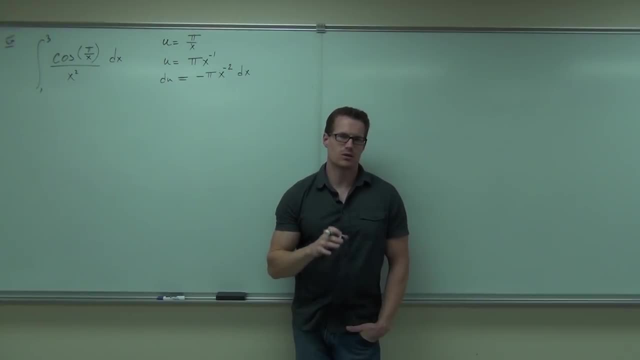 Yes, Solve for dx. Maybe make it look a little bit prettier before you do that, Because right now it's confusing. What am I doing? Am I supposed to divide by x to the negative 2?? You can, and then flip it up. 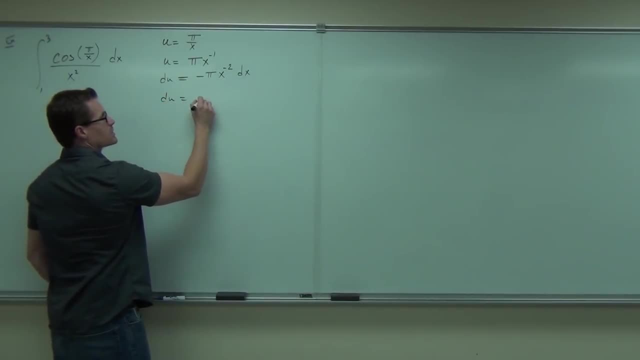 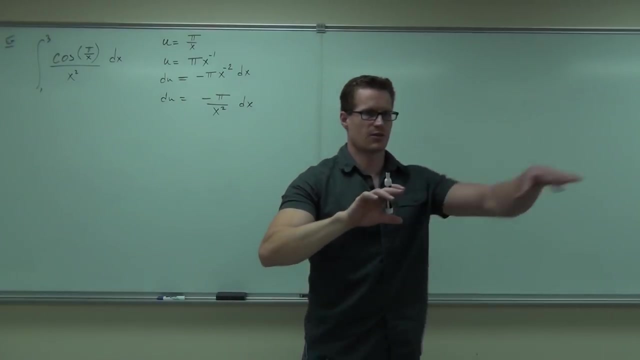 But what this really says is: du equals negative pi over x squared dx. Do you understand that? that's the same thing? The negative pi stays there, The x to the negative, 2 goes to the denominator of the fraction. Now you can solve for dx. 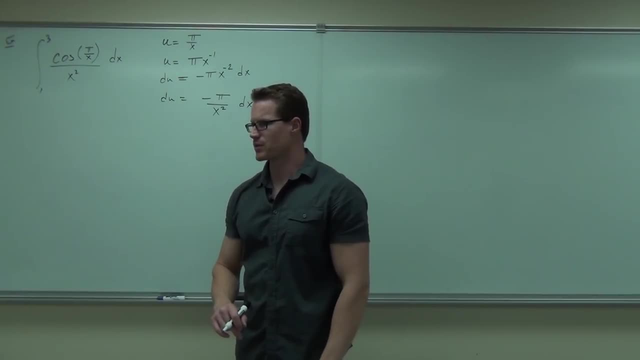 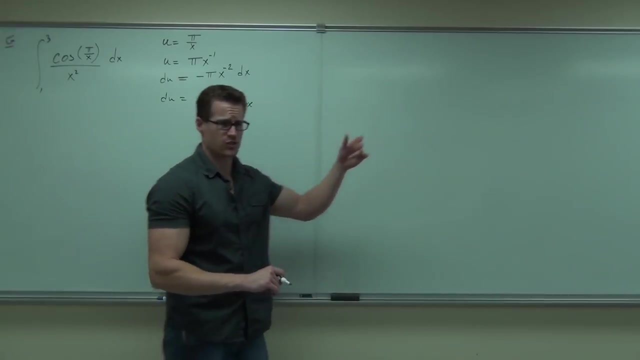 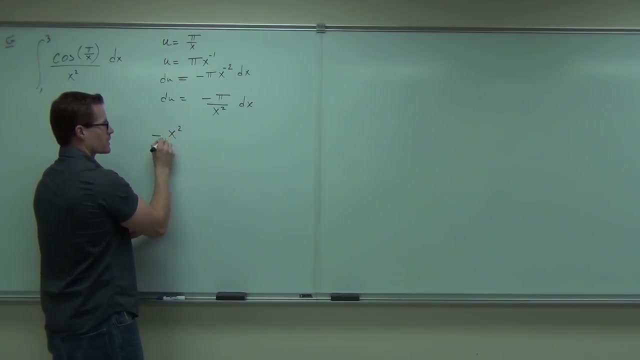 Have you solved for dx? Probably multiplying by the reciprocal would be the appropriate way to go on both sides. Or you can do two steps: Dividing by pi, multiplying by x squared. In either case, hopefully you can follow this one- You're going to get negative x squared over pi. du equals dx. 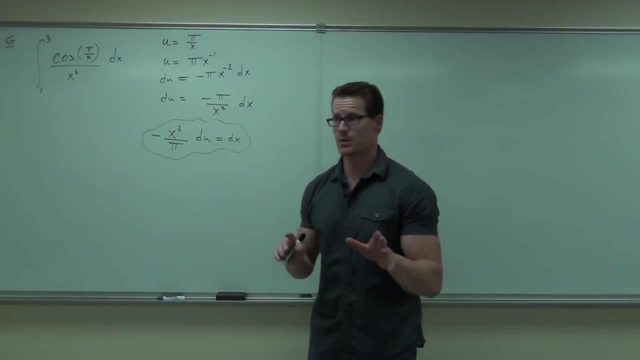 I need to see if you can make it down there on your own, Because that's some basic algebra, But you've got to be able to do it. Nudge your head if you can. Yes, guys on the left-hand side, Yeah. 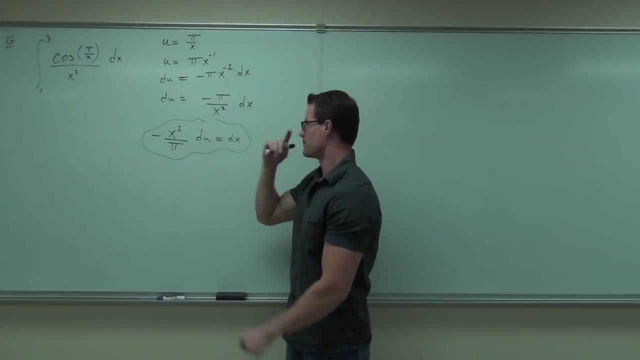 Okay, so basically multiply by the reciprocal on both sides And this is exactly what you're going to get. Also, I told you to change bounds. Where do you change bounds? Do you do it here? Where do you change bounds? Way up top? 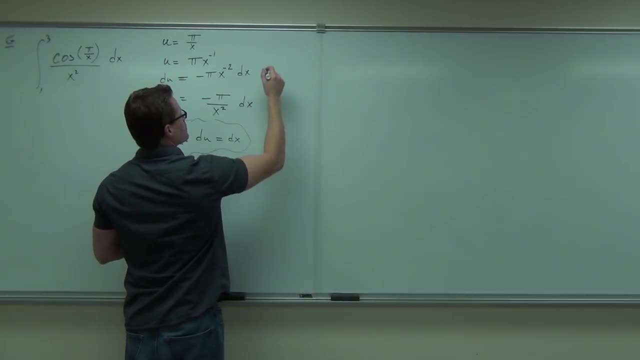 All the way at the beginning. So let's go ahead. We'll change our bounds. I'll do it right here, in this corner, When x equals 3, we want to find out what u is. 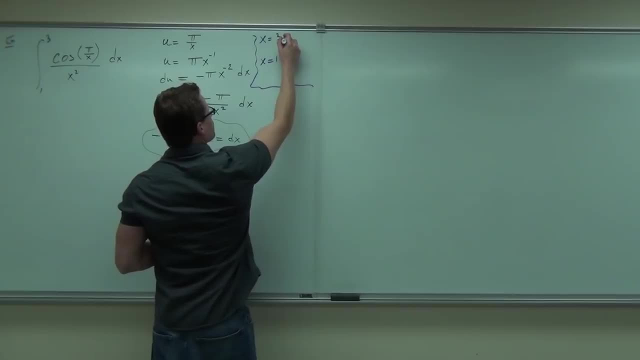 When x equals 1, I want to find out what u is When x equals 3, u is supposed to equal pi over that x, So that would be pi over 3.. 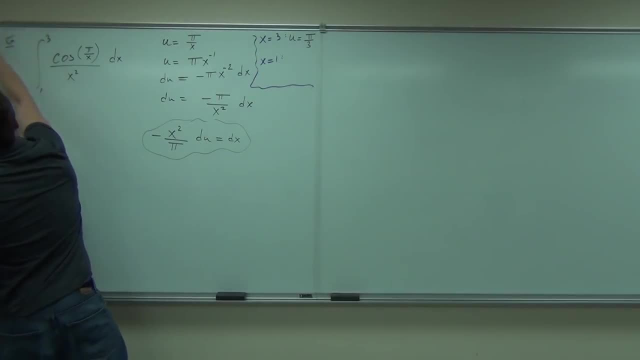 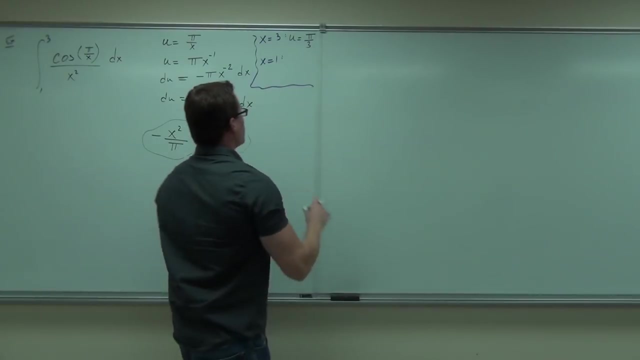 That one was almost in the way so I didn't want to confuse you. Pi over 3.. Did you get pi over 3 as well? When x equals 1, you're supposed to be pi over x. 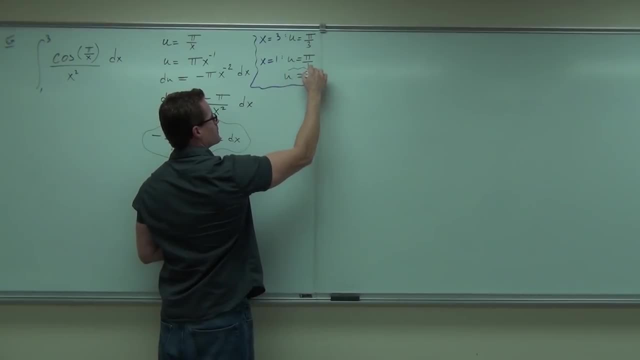 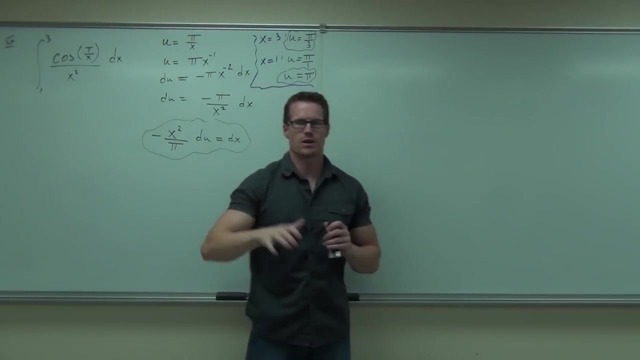 So u would equal pi. How many people feel okay with this so far? Make sure you have these in the correct order. Make sure you map them correctly, from X to U correctly. If you don't, you're going to get the wrong sign on your integral. 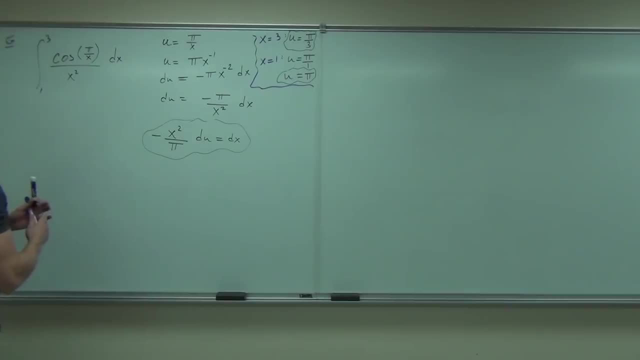 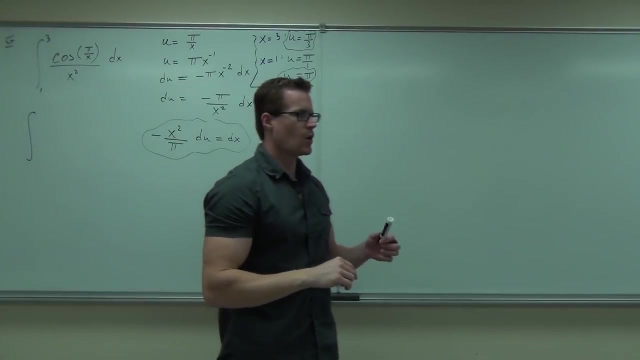 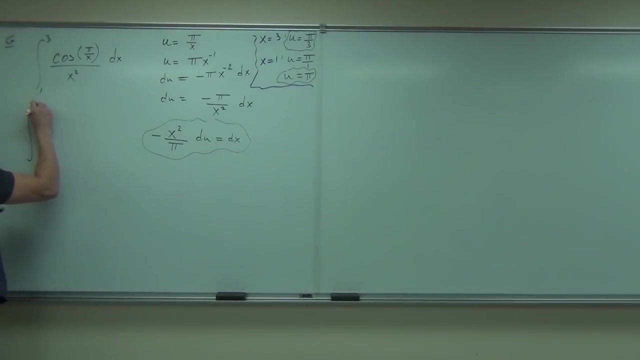 So watch what happens here When I do my substitution. what was X? Well, it was 3.. What's the U that correlates with 3? Pi over 3.. When X is 1,, what's the U that correlates with X equals 1?? 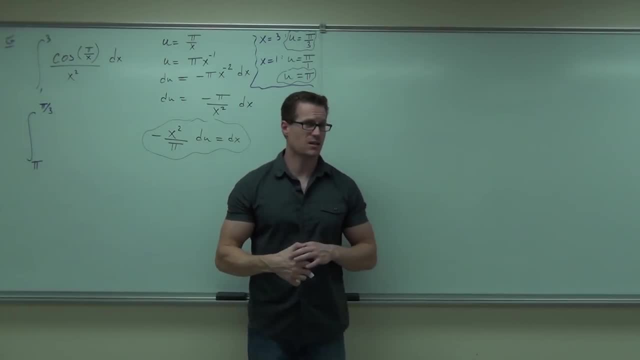 Right now you'll notice something. Do you see what's technically wrong with this picture? It is backwards. That's right. it's backwards. It's going from pi to pi over 3.. That's pi to pi over 3, which says that, if you want to, 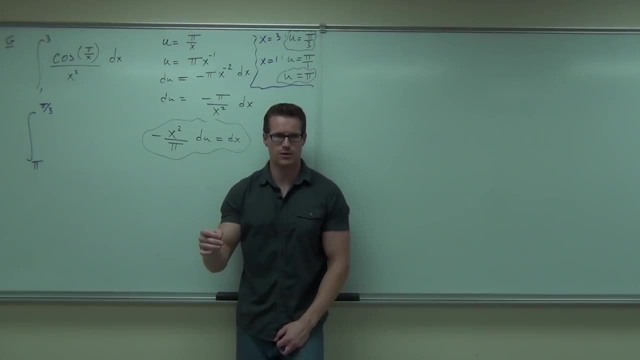 you can interchange them, but it's going to make your integral negative. I can guarantee you this integral is going to end with. well, I can guarantee you this integral is going to end with a negative area. That's what it's going to do. 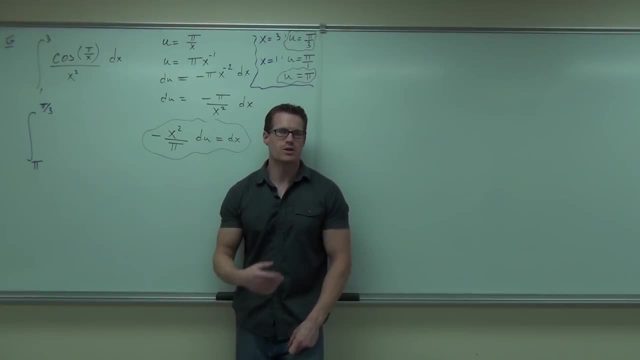 And that's because of that relationship right there. So the reason why I said be careful is because if you go- oh yeah, integrals always go from pi over 3 to pi- then you're going to miss that negative. You had to write that first because the 3 maps to pi over 3.. 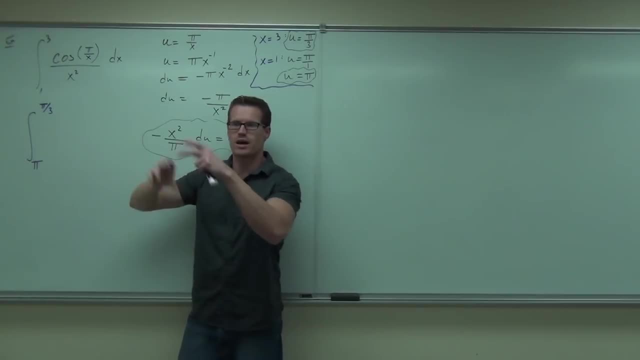 The 1 maps to pi. That's what those bounds were. You can't write them backwards just because you want to. That didn't work. We've got to really be careful on that. And if you're going to say switch them around, then you're going to have that negative out front. 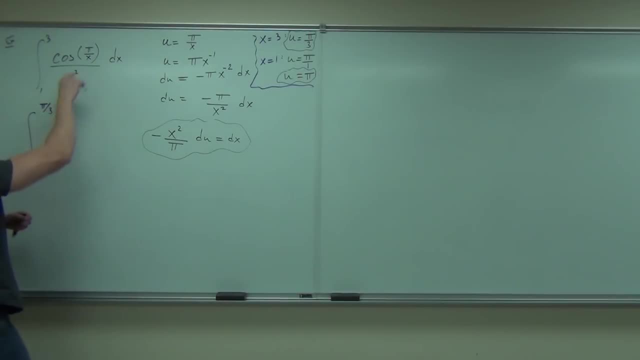 Okay, now for the other good stuff We have. what else is up here? Come on now. Cosine is still there. If it's not part of your u, it's still there. Cosine of what U X squared is still there for right now. 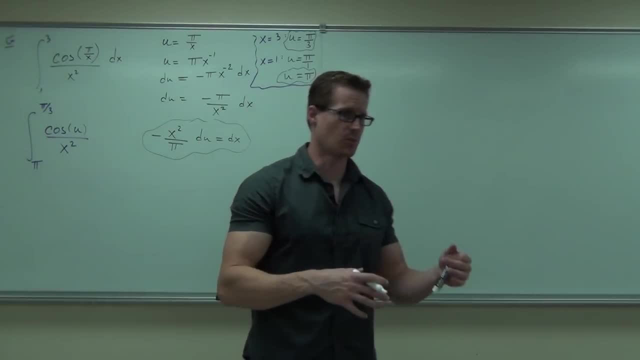 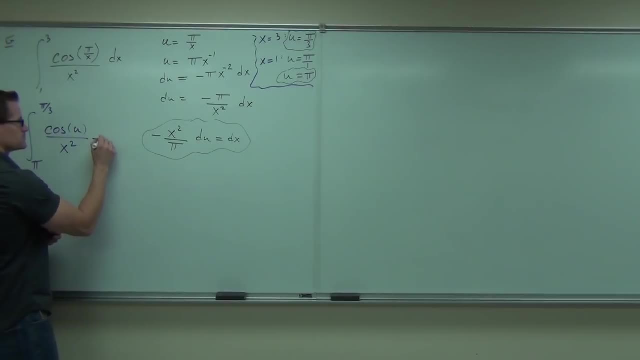 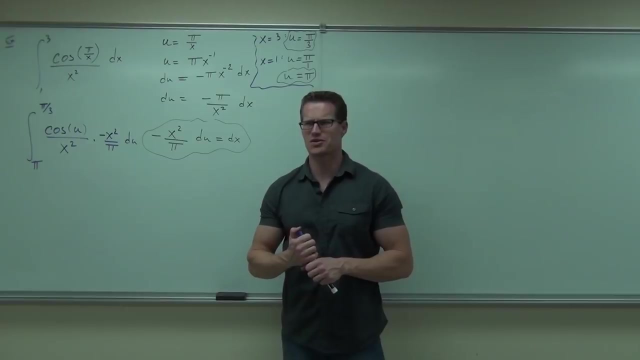 dx is definitely not there. Instead of dx, you're going to write what dx equals to. That's negative x squared Over pi. du, I do it like that for you. Now, some interesting things are going to happen. Interesting things are going to happen. 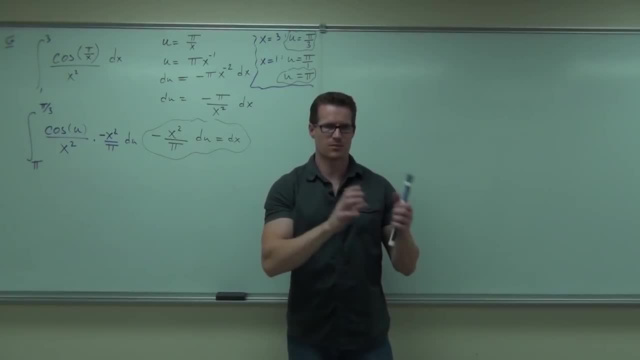 Some things are going to cross out, Some signs are going to be pulled out, Some constants are going to be pulled out. Let's see everything that happens here. Tell me one thing that happens: X squared- X squareds are great. If that didn't happen, you'd either have to manipulate that somehow, like we did before. 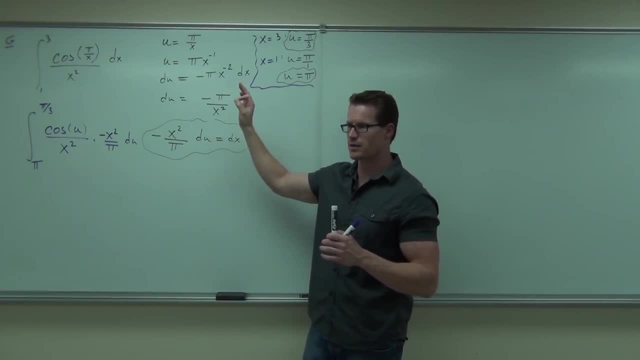 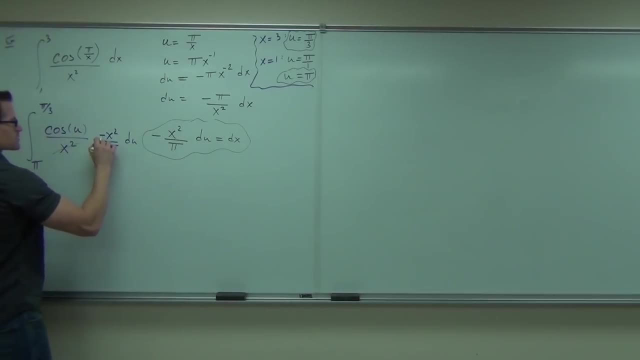 which would kind of be a PETA, a pain in the rear end. You don't want to do that, Or that's about it. You're going to do it, So cross out your x squareds. That's great. 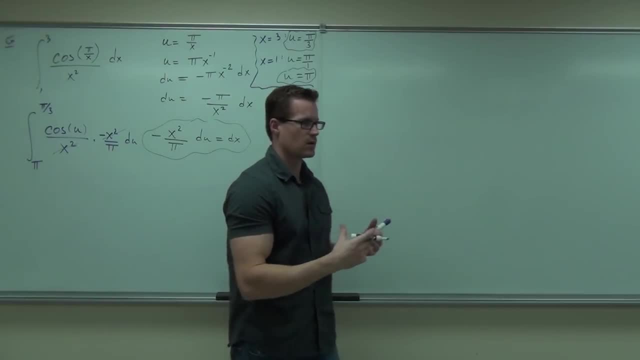 What else can I move out in front of my integral? You're a negative. Now you have negative 1 over pi. Yes, Time to already have negative is the first one. I'm not doing that yet. Okay, Let's see if we can all make it down there in our heads. 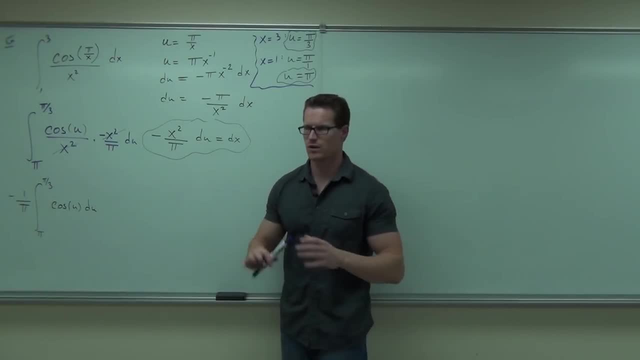 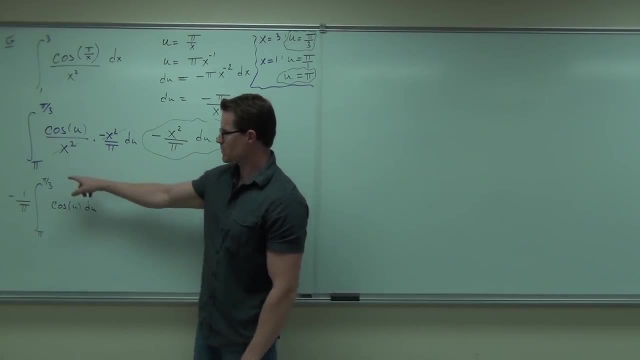 Are you feeling good with that so far? So just doing our substitution. We've simplified some algebraic things up here, moved out our constants, which is great. Now this is in the wrong order, but right here that's going to look like it helps us a little bit. 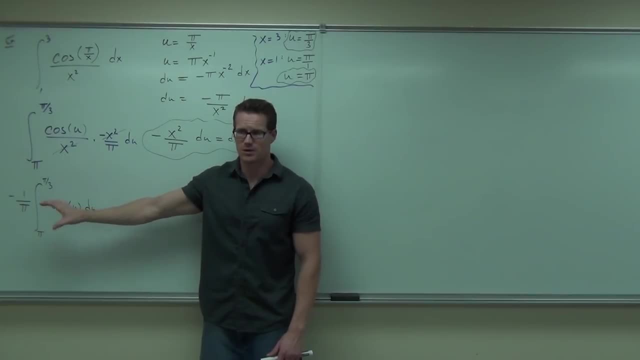 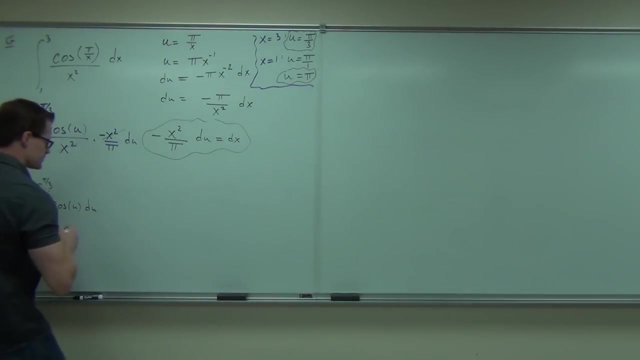 If I reverse them, notice I can change the sign right. Put them in the correct order. I'm going to change the sign. So what this says is: let's go ahead and let's, let's flip these bounds. When I flip the bounds, I'm going to get negative, negative 1 over pi. 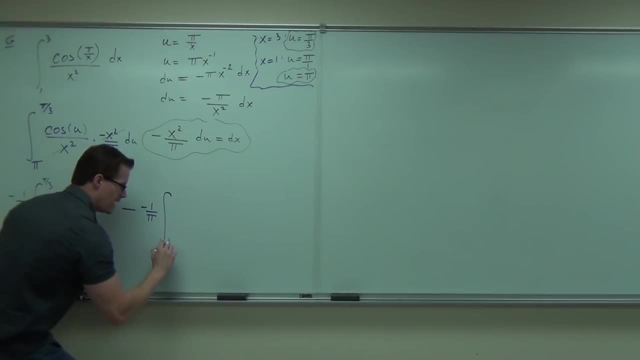 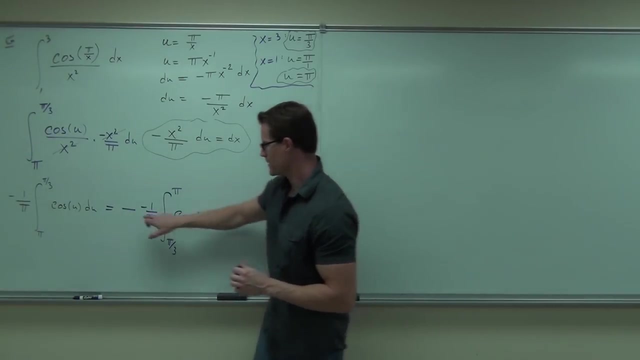 My integral will change from pi over 3, pi to pi over 3, back to pi over 3 to pi. Cosine u d u. Okay, Make that negative Way too big. There we go. But you see the negative, negative right. 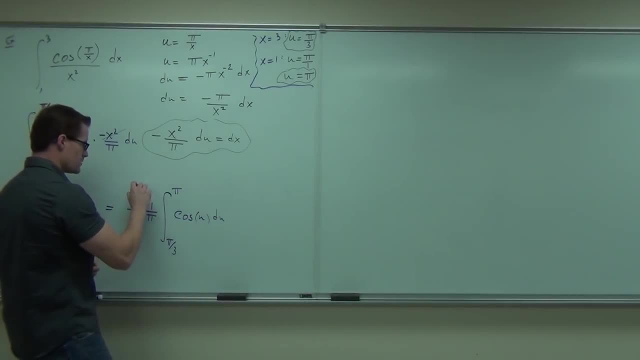 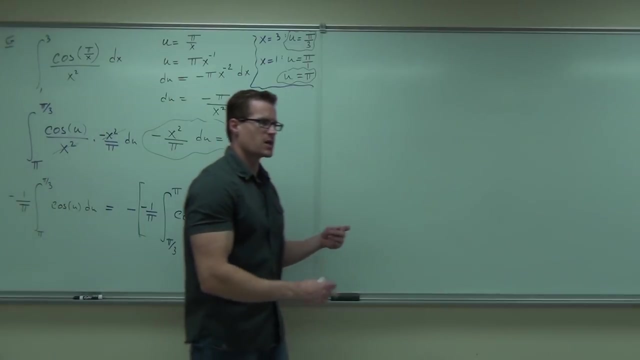 Technically, what it really should have is a big bracket around here. If you want to draw that, you can, But that negative negative is going to change. That's going to become a positive. So we get our 1 over pi. 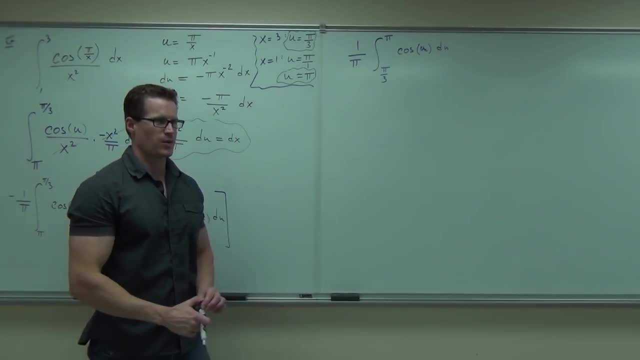 From pi over 3 to pi over 3. You get pi over 3. The negative negative negative. So pi over pi, plus pi over pi, minus pi over pi, minus pi over pi, minus phi over pi. cosine u d u. 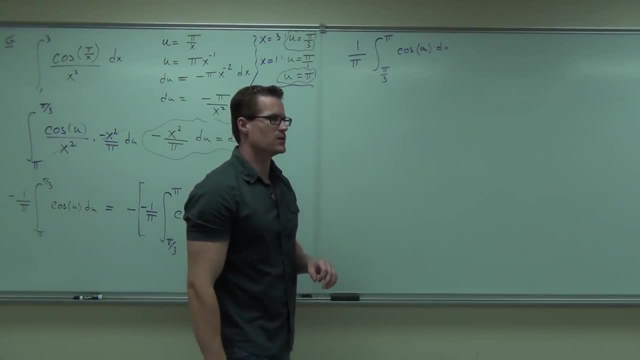 By the way, it's really nice that we changed bounds here, because otherwise we'd have to substitute back in for that And it gets a little bit more confusing. You have to figure out a couple things as you're going. It's nice that that's already done for us. 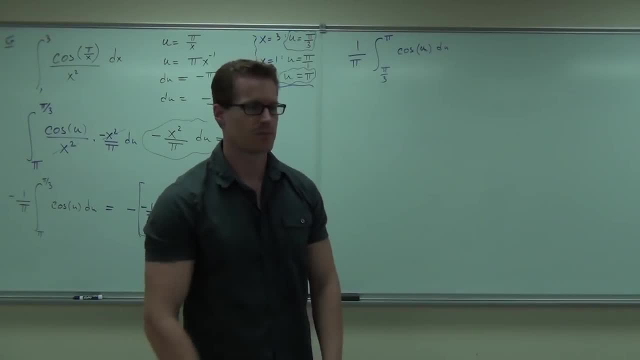 What I'd like you to do right now. would you go ahead and do the integral, Go ahead and evaluate it, the way that we've written it, the way that it's kind of nice for us, And then see what you have. Okay. 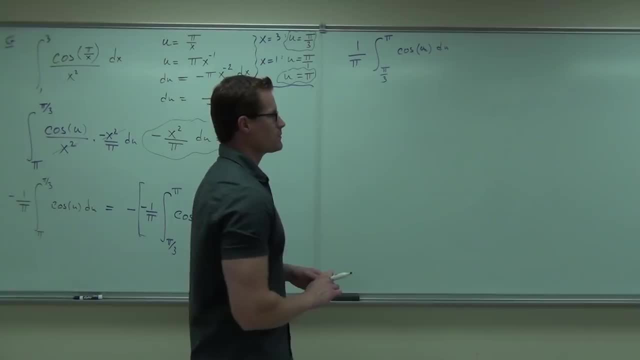 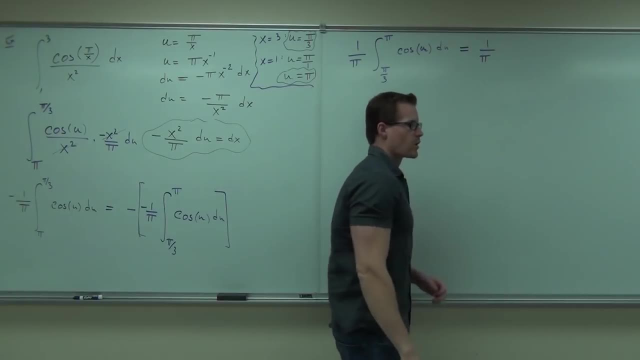 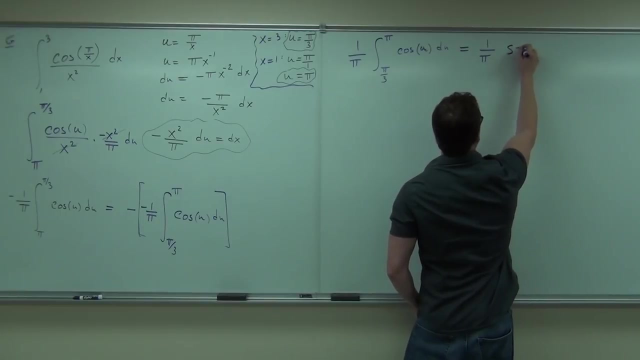 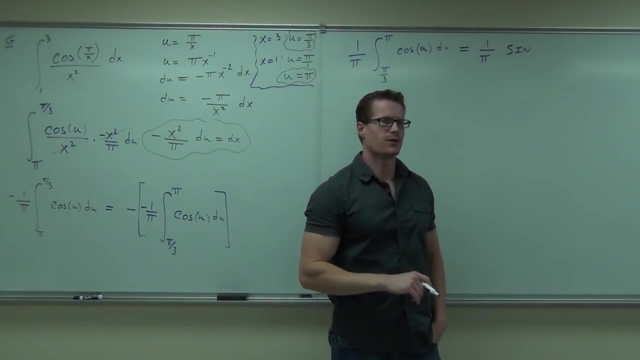 Okay, Good, Good, Good, Good. Okay, Okay, Good, All right, Don't forget about that. 1 over pi out in front. Remember it's positive now because the negative negative gave us that positive. Oh yeah, by the way, the integral of cosine sine or negative sine. 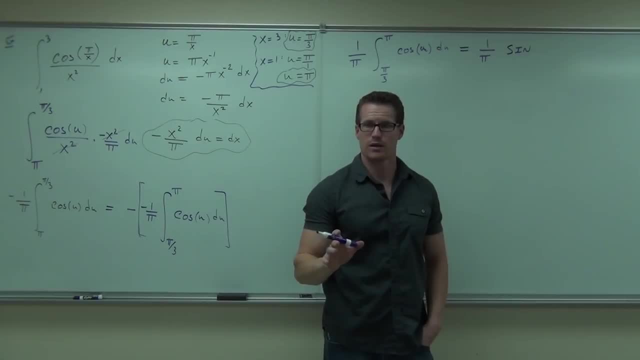 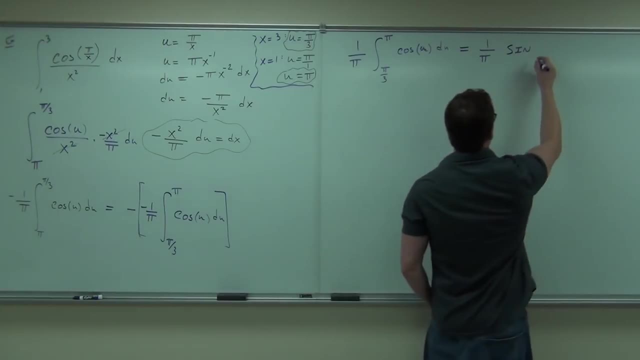 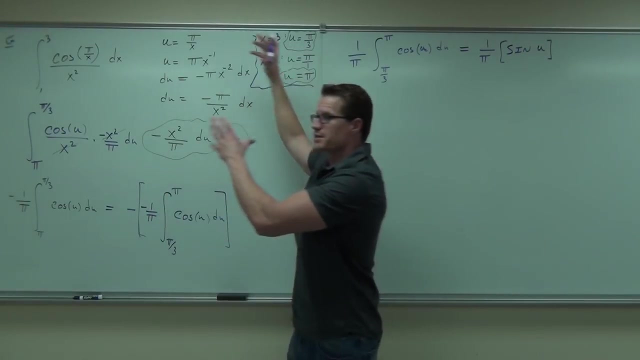 Sine, Sine. good, That would change your problem right. Remember that the derivative of sine is positive cosine, so the integral of positive cosine is positive sine. No plug-in impact for x's. We already changed our bounds, That's great, so we don't have to do this whole resubstitution thing. 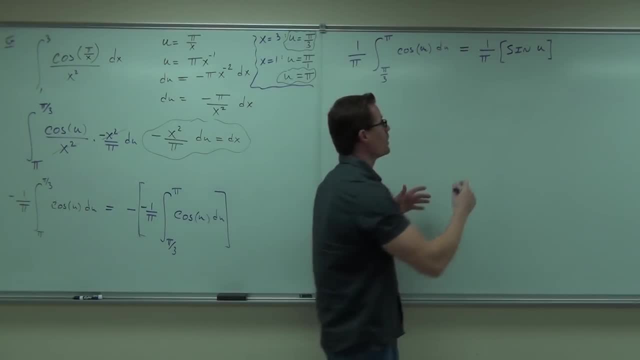 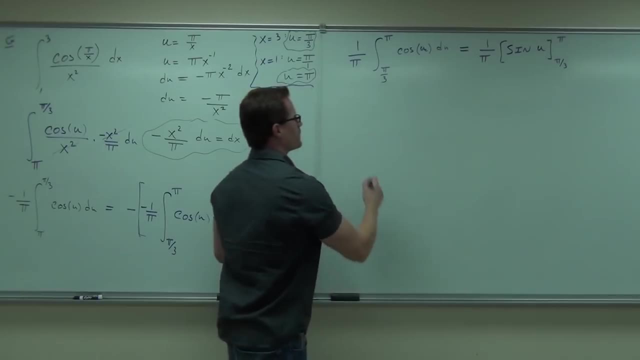 We don't have to do that. We've changed our bounds off to the side. We were already in terms of u. That just means from right here let's evaluate. So we'll do 1 over pi. That's going to be out in front. 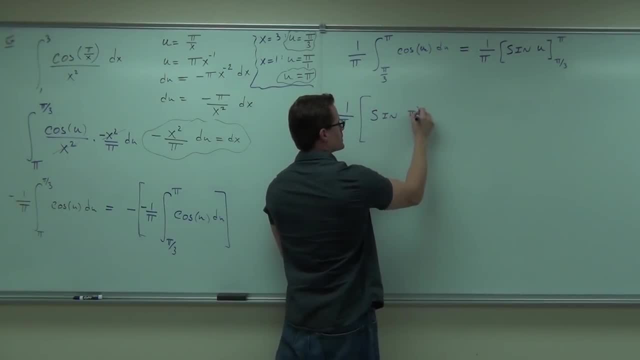 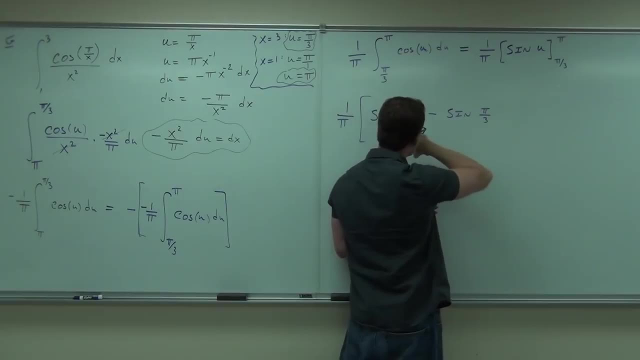 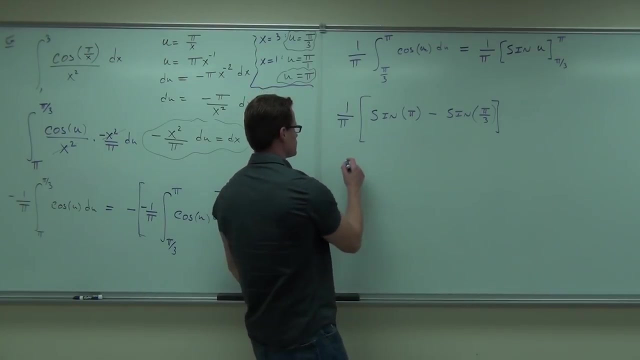 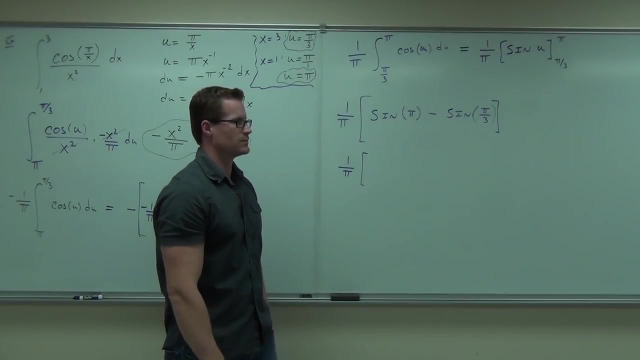 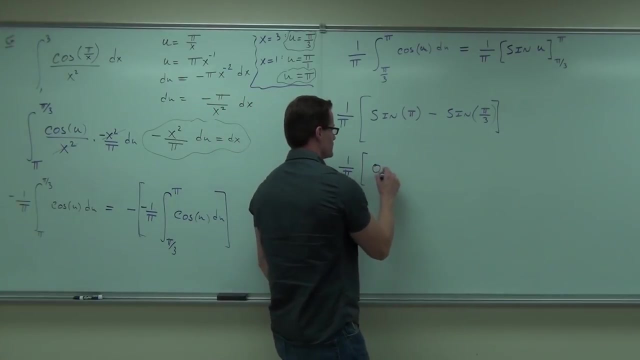 Inside we'll have sine pi minus Sine pi over 3.. Sine pi Zero. Okay, I had to be stumped for a second, I don't know why, What? Oh yeah, I had it in my head as something different. 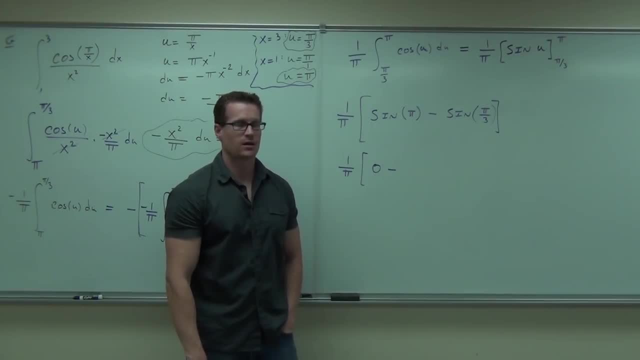 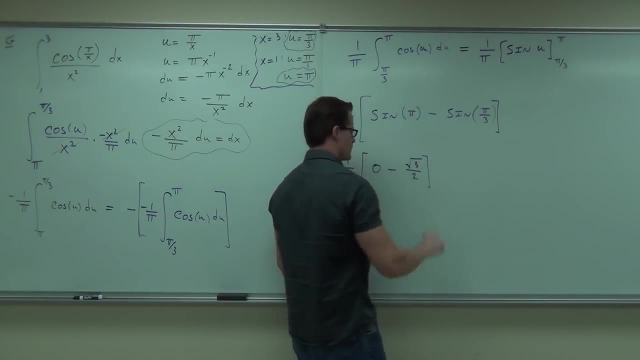 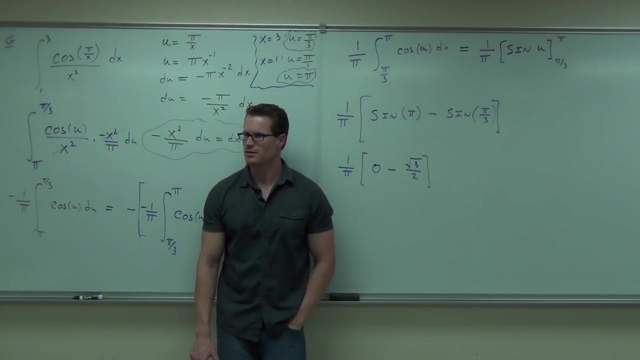 Sine of pi over 3.. How much is that? 4 over 3 over 2.. Good, Were you able to get that as well, Cool? Zero minus root: 3 over 2?. Negative root: 3 over 2.. 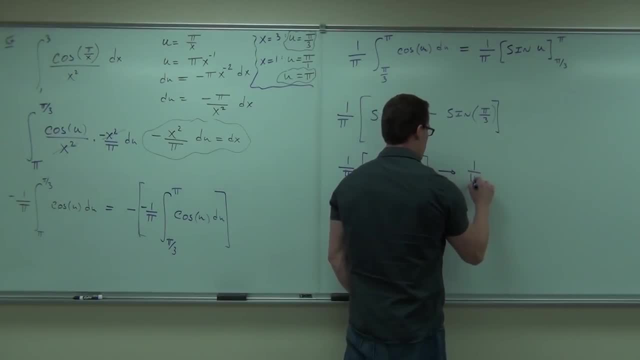 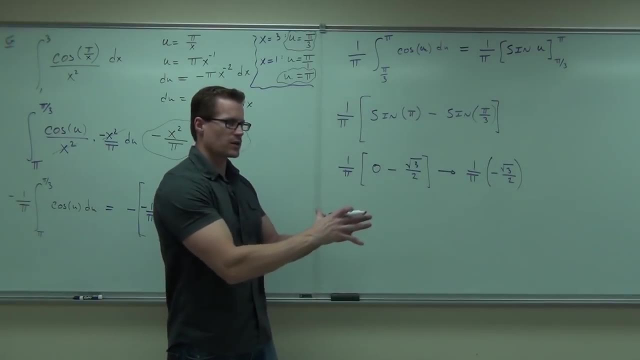 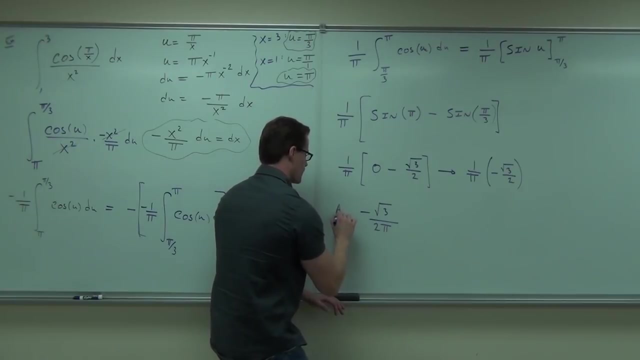 Interesting: 1 over pi. Negative root 3 over 2.. Put it all together You're going to get negative root 3 over 2 pi. That's your area. Looking at your area, would you say that this curve is above? 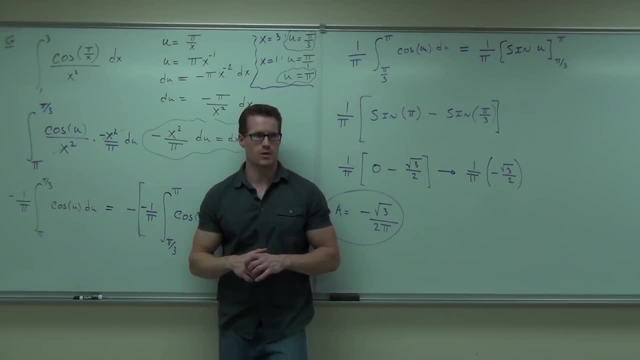 or below the x-axis for most of this region. For most of this region, If it crosses- I don't know whether it does or not, but if it crosses most of this region- it's going to be negative root 3 over 2.. 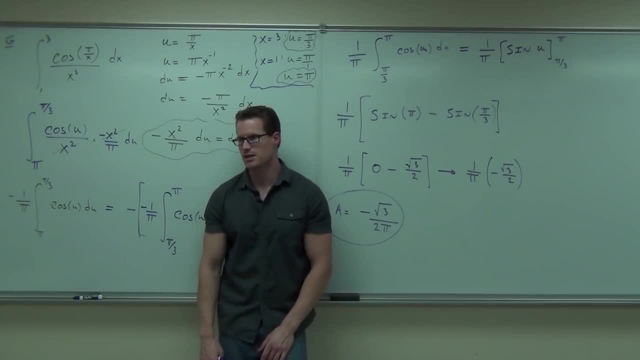 Most of it is below the x-axis, because our area is mostly below the x-axis. So, area speaking, it's mostly below the x-axis. How many of you feel okay with our example? Okay, that's the last one you get about direct substitution. 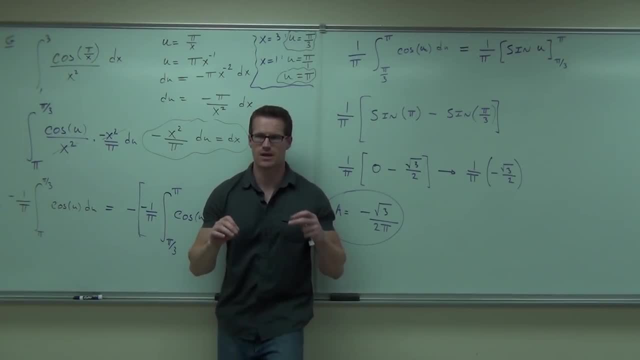 with the definite integrals and changing bounds. I'm going to show you some kind of tricks, some night-and-night tricks, properties of things you can use to make even and odd functions work for you sometimes. Are you sure there's no more questions on this stuff? 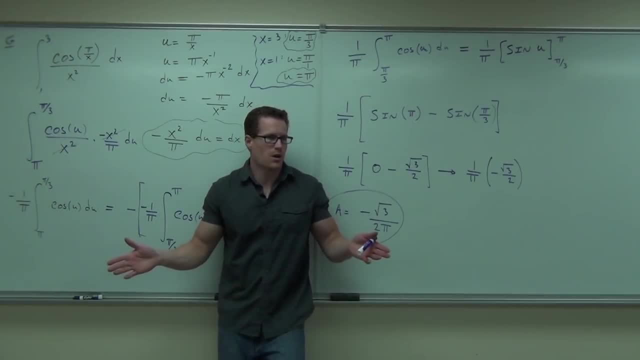 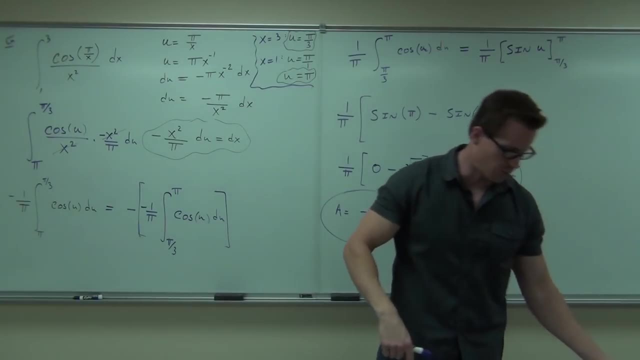 Do you feel pretty comfortable with it? Yeah, Substitution, No problem, You are doing that. Now it's just changing bounds and being able to evaluate it. I've given you some kind of nice examples that kind of illustrate that a little bit better for you. but let's talk about even. 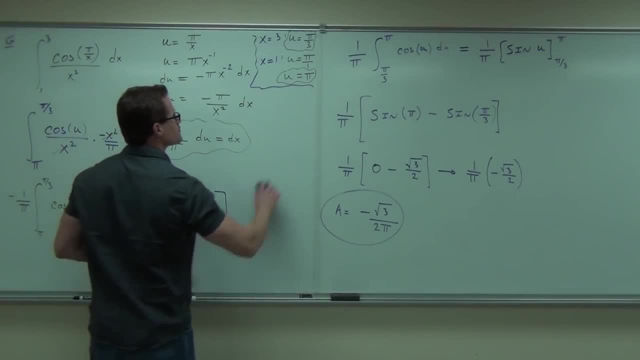 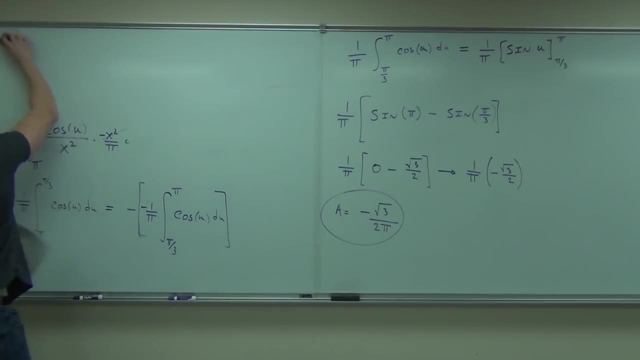 and odd functions and how we can use them to our benefit sometimes. Okay, so I'm going to go ahead and show you some examples of what we can do with this. Okay, so I'm going to go ahead and show you some examples of what we can do with this. 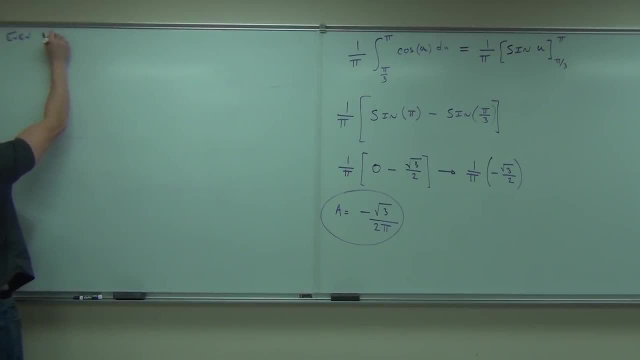 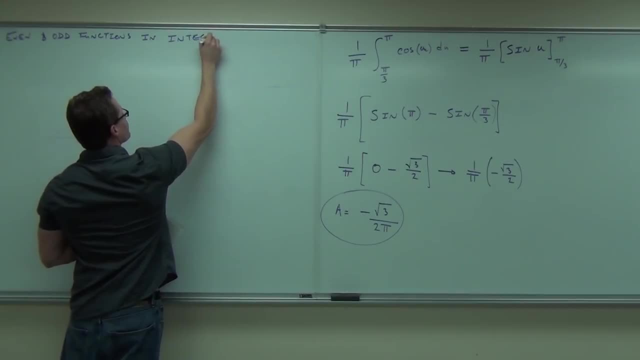 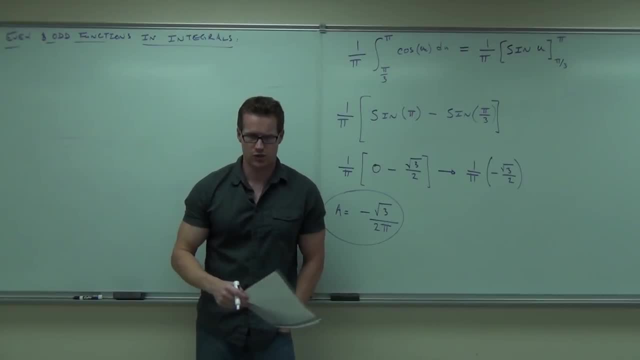 Okay, so I'm going to go ahead and show you some examples of what we can do with this. There we go: Even and odd functions and integrals. Let's talk about even functions for a second. Hey, tell me something. What do you know about an even function? 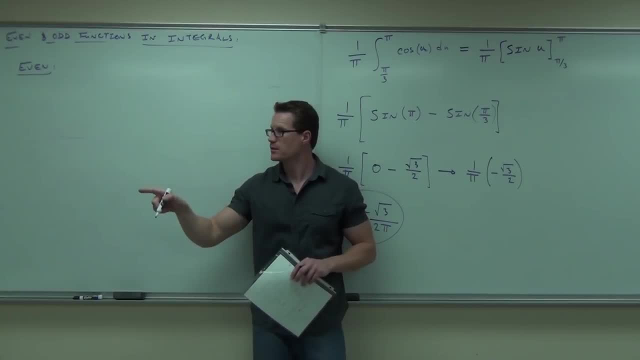 Symmetric. Oh, say that again. Symmetric, Symmetric, yes, About what, What, what Which? X-axis, No, Y-axis. Well, yeah, it's the other one. Very good, It's a genius. 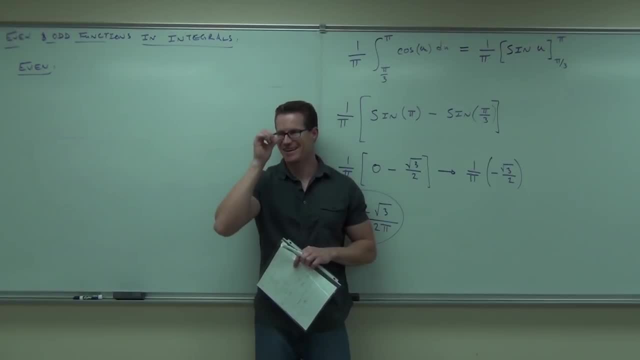 Okay, we're not on count three. Okay, yeah, it's symmetric about the Y-axis, Dear goodness me. Yeah, that's what even means. X squared is an even function. X fourth: even function. X squared minus two: even function. They're symmetric about the Y-axis, That's one thing. 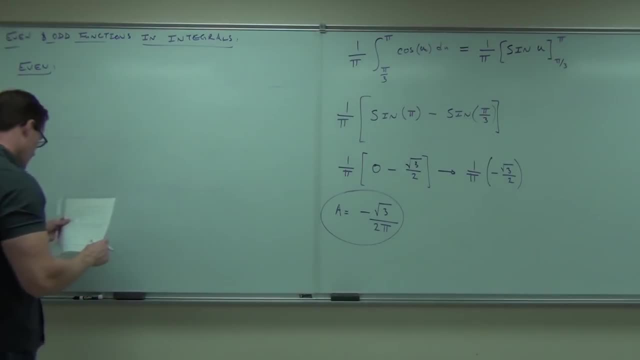 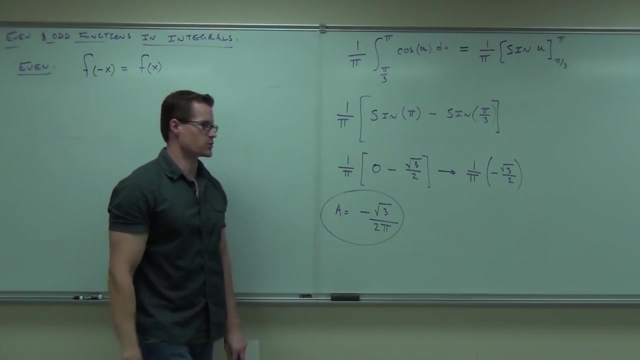 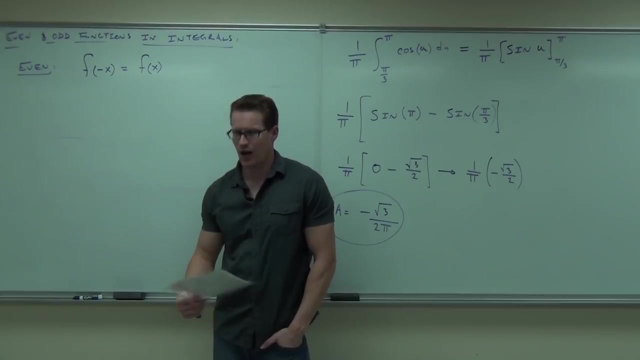 we know about even functions. Here's the definition of it. actually, Even function says that That's what an even function says. I hope it makes sense on why that would work. It says: you plug in a number or the negative version of that number. 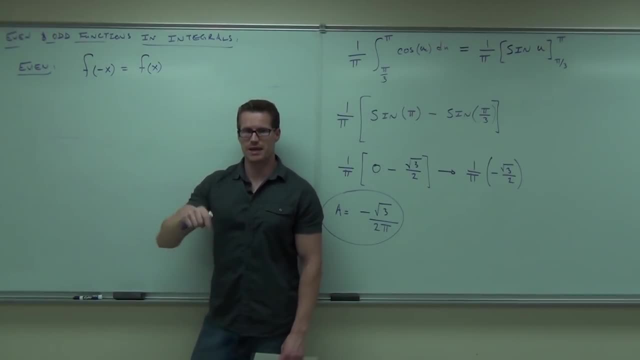 And your height is the same. What that's going to do is make it symmetric. about the Y-axis. Notice that: Plug in two, you get out seven. Plug in negative two, you get out seven. That means it's symmetric. It's going to go up at the same rate on either side of 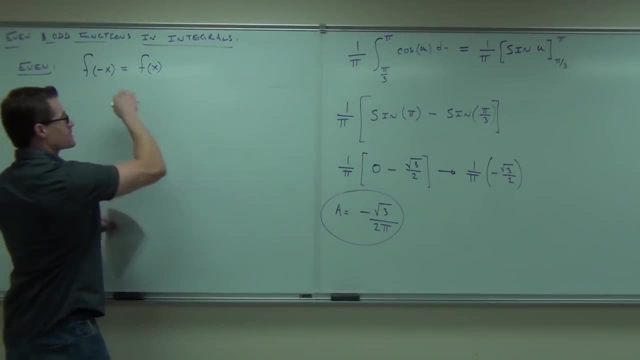 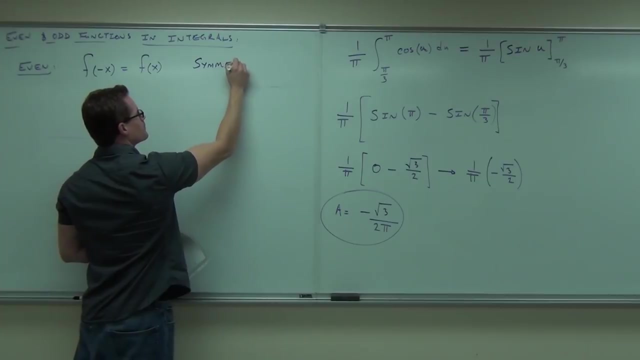 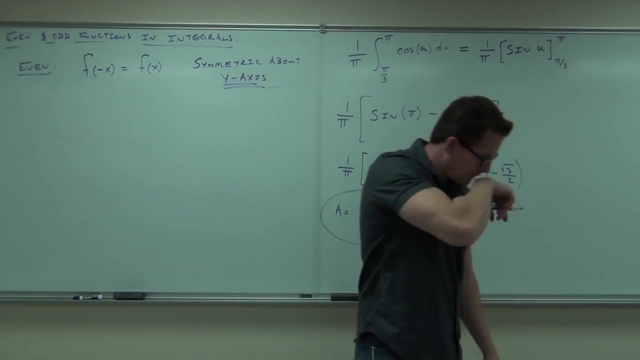 the Y-axis, And that's what this is doing. So it's this, and what it means is symmetric about the Y-axis. Just make sure you know it's the Y. Well, let's think about this for a second then. 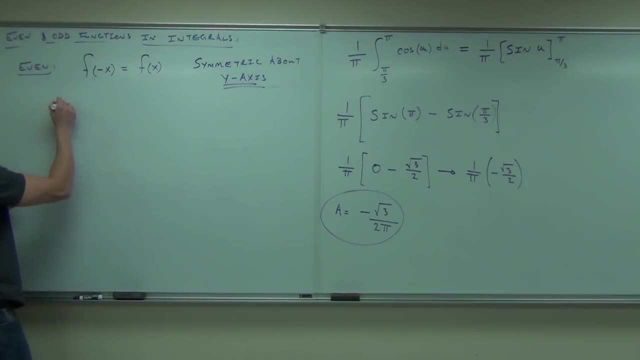 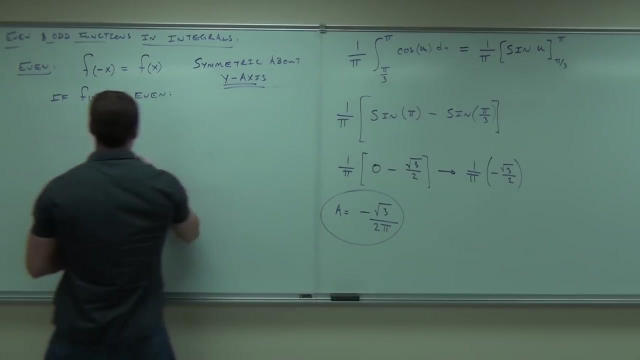 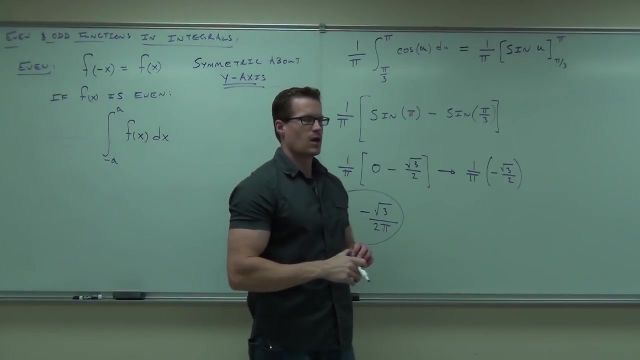 Let's suppose that if F is even- And I'm going from negative to positive a, Go from negative a to positive a- Take an integral of F of x, dx. If F of x is, let's go through the logic. okay, If F of x is even, what do you know about F of? 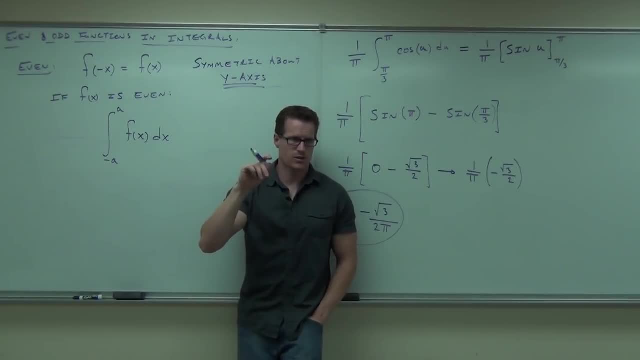 x- Symmetric- Symmetric. So that means that when I plug in negative a and I plug in a, I get the same output At any point between them. I plug in the negative and I plug in the positive Symmetric. 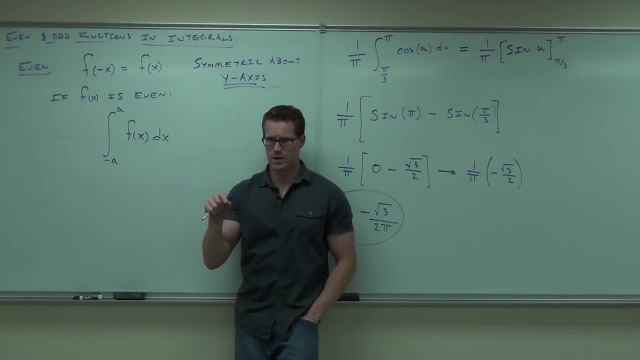 Symmetric And the opposite of that, I'm going to get the same output. Would you agree then that the area from negative a to zero would be the same as zero to A? If it's symmetric about the Y, it better be, because you're going to get a picture like: 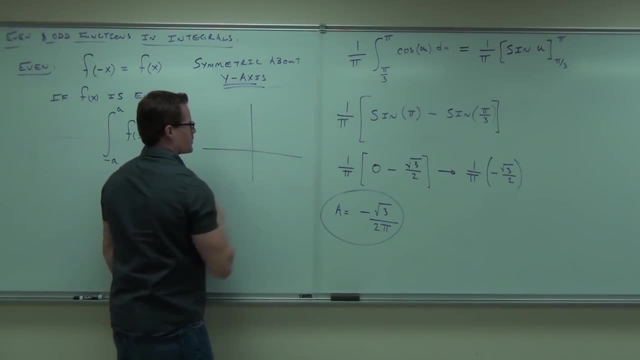 this. I don't know what F is going to look like, but I know it's going to be something like this. Whatever this does, this is going to do the same thing on the other side. It's supposed to look the same. 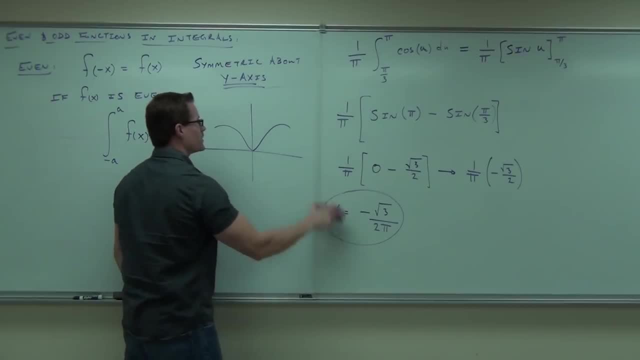 by the way, I'm not that good of an artist. My paper looks better. I should show you my paper. They're laughing at my picture. Hopefully you can't hear that in the video. They're laughing at me. Well, if it's even, you're going to get that relationship. 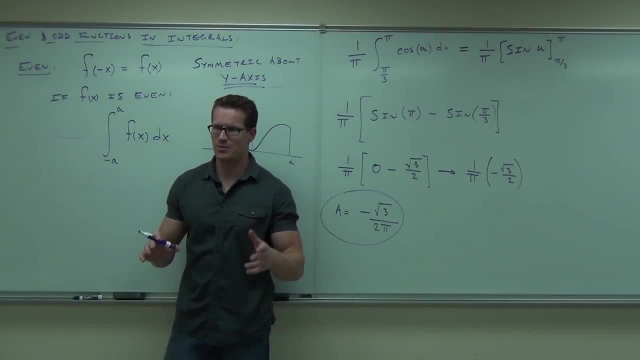 If you're going from negative A to A, that's actually a special case, right? It can't be going from, like negative B to positive A, because those numbers wouldn't match up, That would be different. But if it's going from negative to positive of the same number, 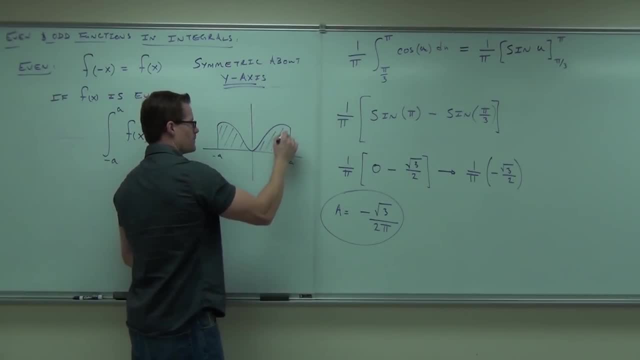 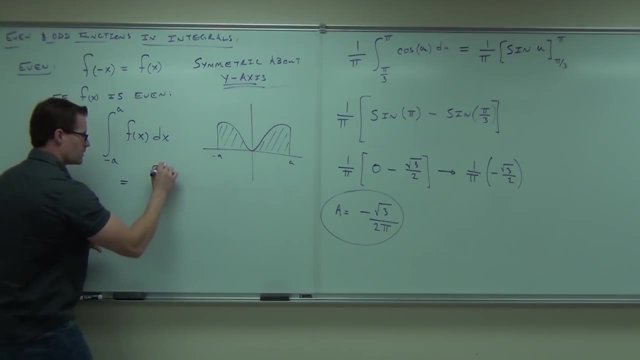 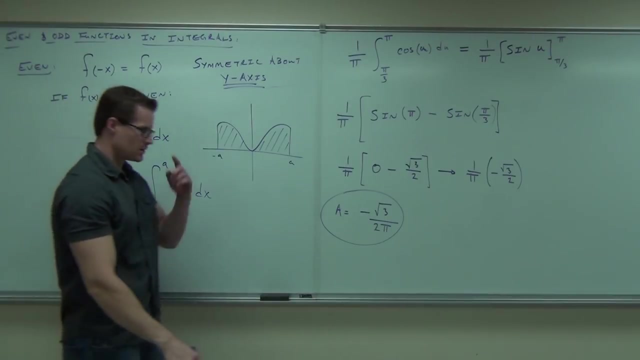 well then, you know, this area has to equal this area, which means that this integral is going to equal that integral. Does that make sense? Sometimes it's easy. It's easier to calculate from zero to a number than it is from negative to a number. 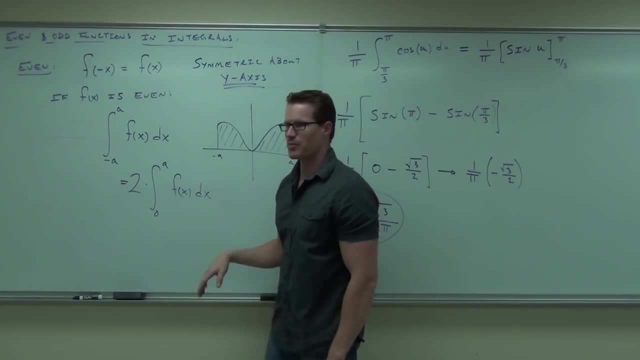 It's easier to do that. So if we can do that, well then no problem. If it's an even function, shoot we can do this. We can calculate two times that integral and we're good to go. Zero is normally very much easier. 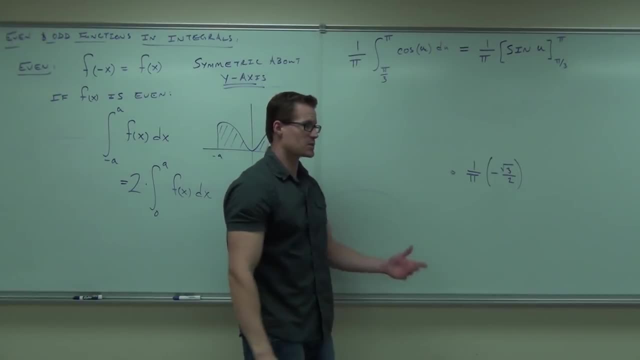 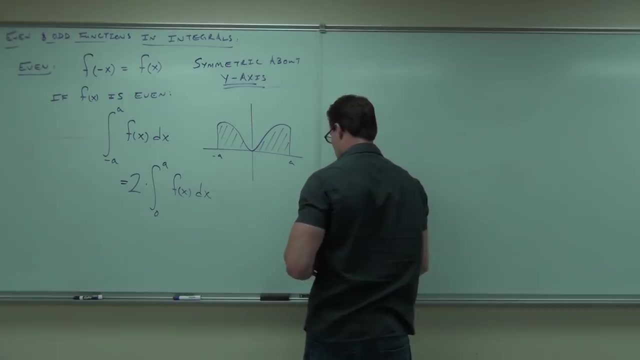 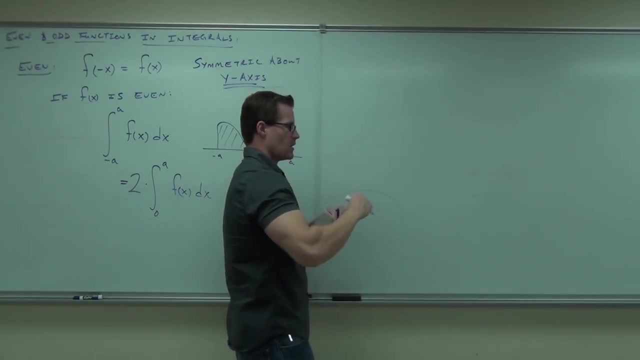 Yeah, Now, if you have to use a substitution, the zero might change, but normally zero is easier. Let me just show you with an example. Let me just show you with an example that this does actually work, The only thing you've got to do. which kind of stinks. 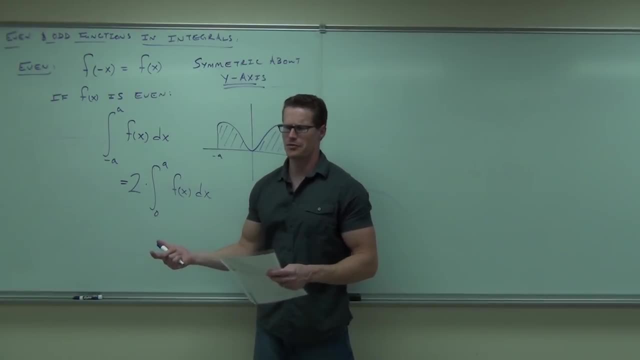 is that you have to prove it's even before you can do it. You can't just say, ah, I think it's even, Let's try it. No, that doesn't really work all the time, So you've got to show that it's even. 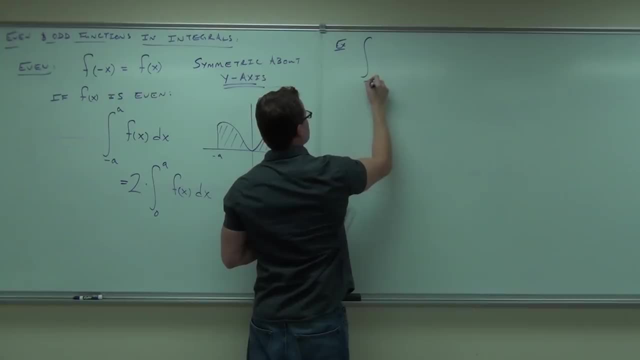 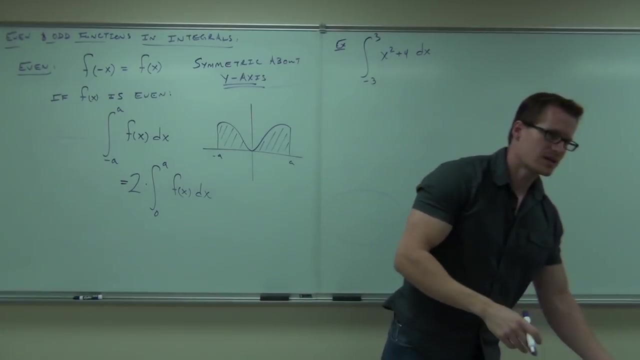 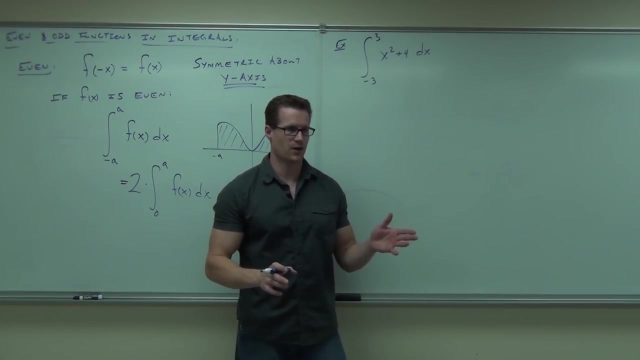 So, for instance, let's talk about that one. Now, that's a pretty basic integral. You could clearly do this integral just the way it is. You could just do it and that would be just fine. I'm not going to give you a super tough one where it's super. 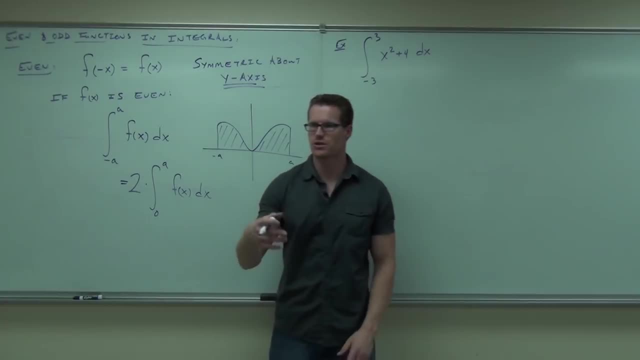 super nice to do that. I'm just going to show you with one that's easy for us to see that it is possible. First thing you do, though, you've got to prove it's even. Here's how you prove it's even. 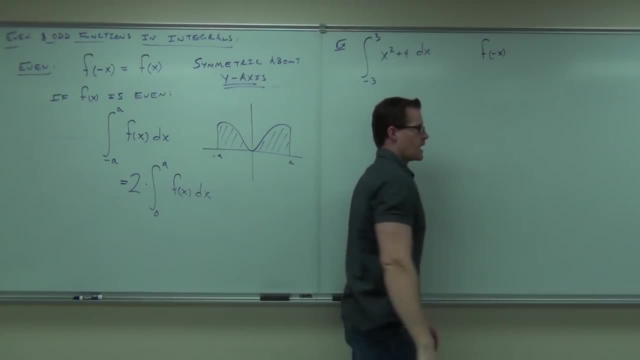 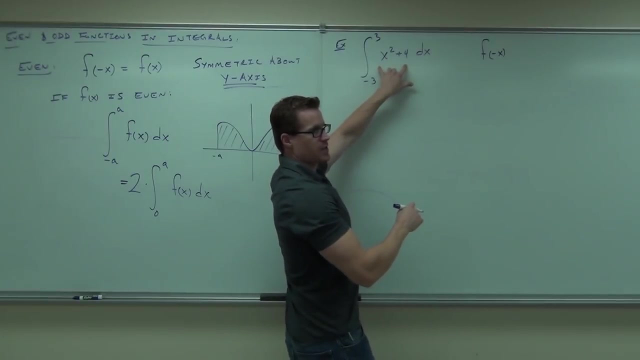 You start out with f of negative x and you have to show that that's equal to f of x. So f of negative x says this: You go to your function, f of x, and you just replace x with negative x. So for us that's equal to f of x. 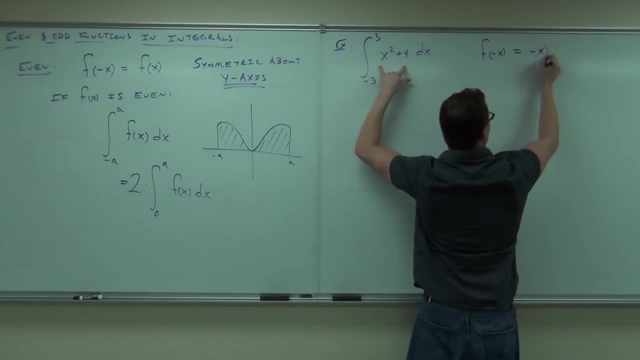 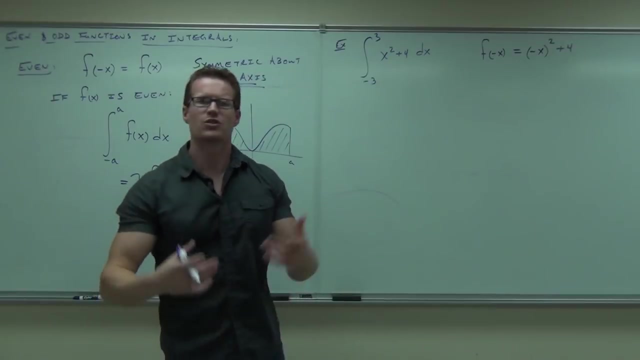 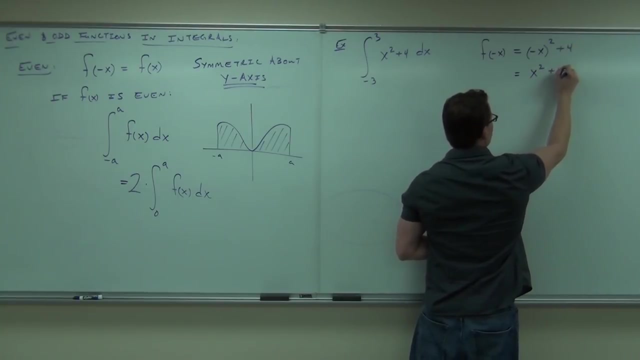 That would be negative x squared plus 4.. Do you see how I just replaced the x with the negative x And then you work it down. You see what you get. What's negative x squared X squared Plus 4.. What's x squared plus 4?? 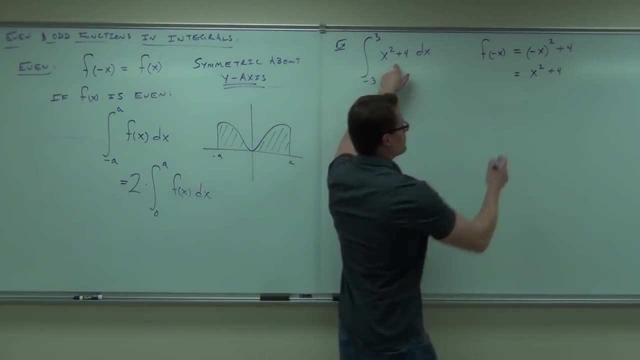 F of x. That's f of x. That's exactly what I have back here, Right there. that proves it's even. If you start here and you end here, that means you have an even function. How do you feel giving that one so far? 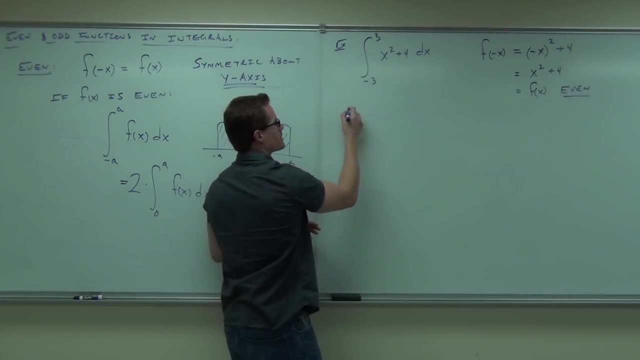 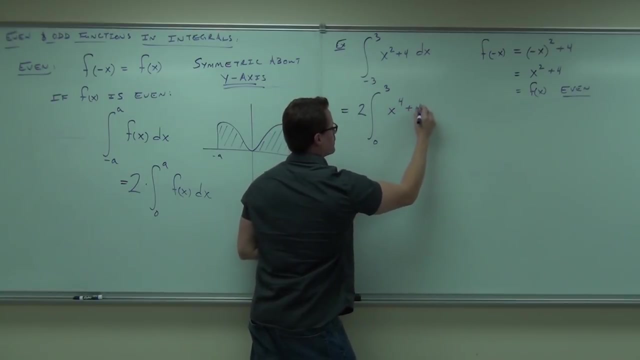 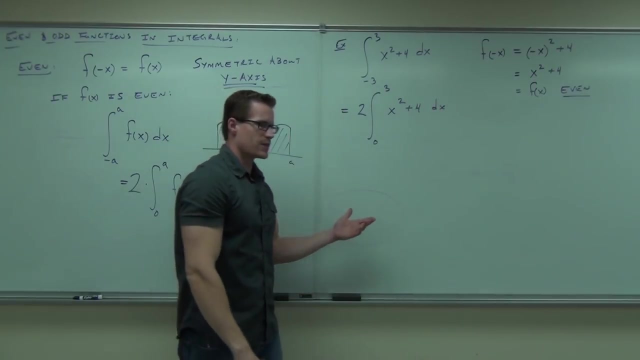 Okay. What that says is that, instead of doing this integral the way it is, I know that this is going to equal 2 times the integral of 0 to 3.. Not bad, X squared plus 4.. I'm going to let you do that the rest of the way out. 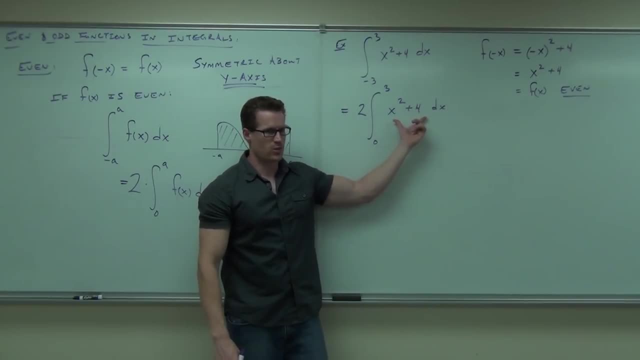 What you would do here. take your integral, evaluate it from 0 to 4.. No, No, No, you wouldn't. 0 to 3. Go from 0 to 3, and then multiply that by 2.. 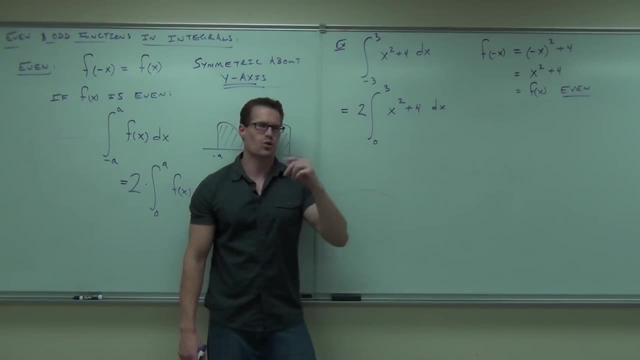 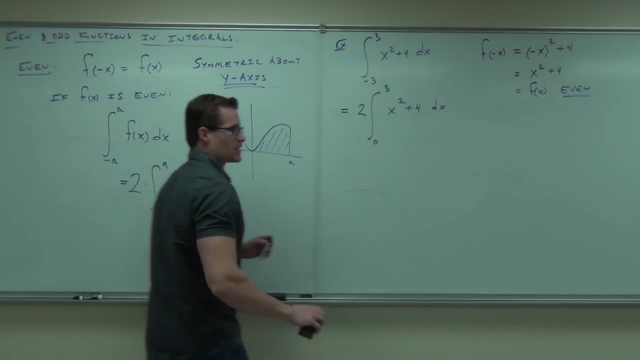 Has anyone done that already? Why don't you work on it? Let's see if we can get a couple of the same answers up here. Are there any questions on the even part of the board before I erase it? Did you understand the concept? 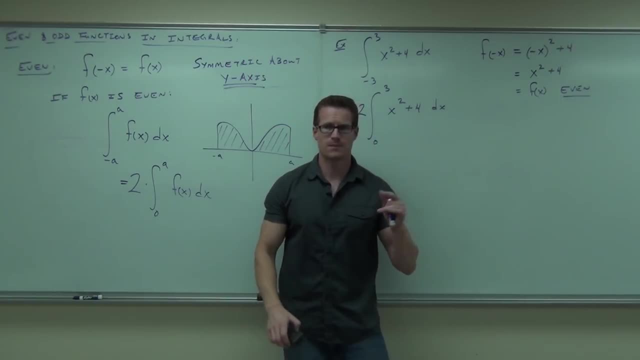 Even means to measure about the y. You prove it's even. that means the area on the left and the area on the right will be exactly the same. Therefore, you go from 0 to a. What's that 0.? Whatever that number is, and multiply by 2.. 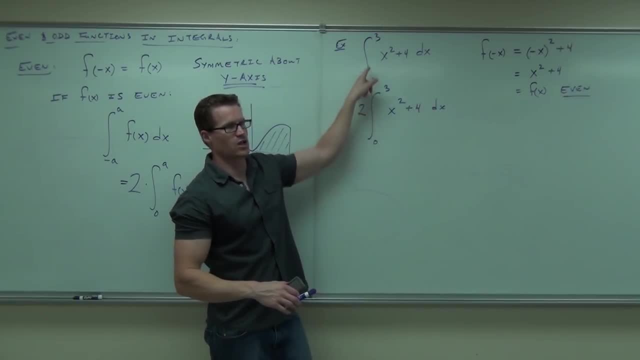 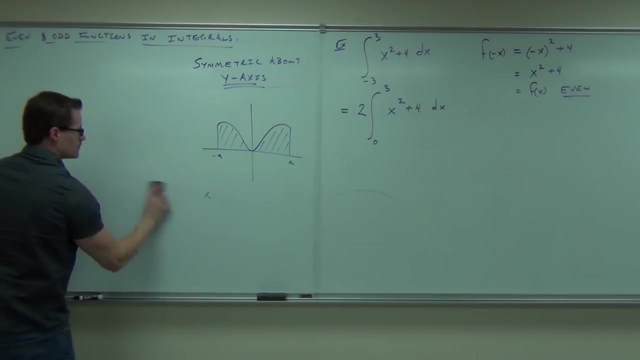 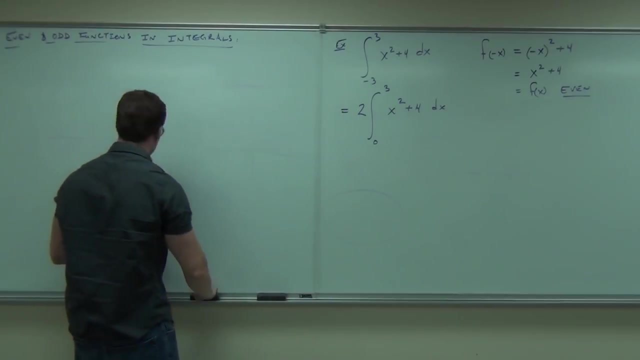 Just be very careful. These numbers absolutely must match up for this to work for even functions. If that was a negative 4 and that was a 3, all bets are off. You can't do that anymore. 42?- I have no idea. 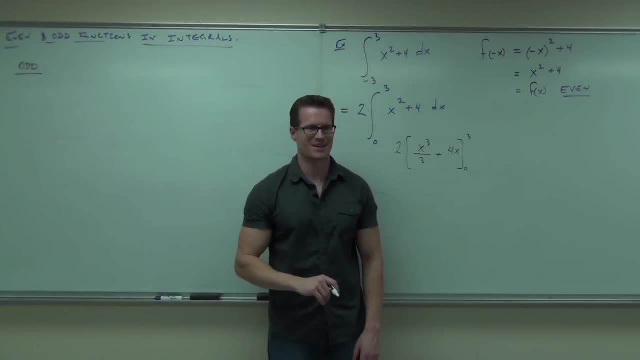 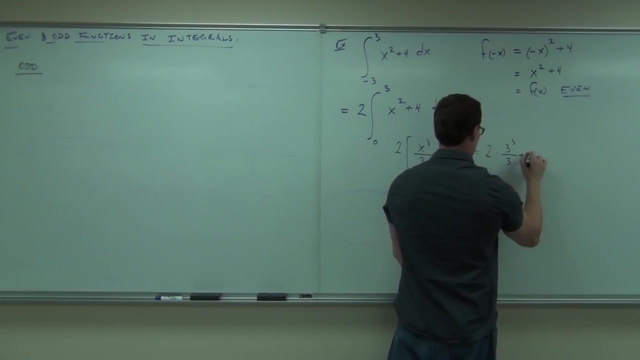 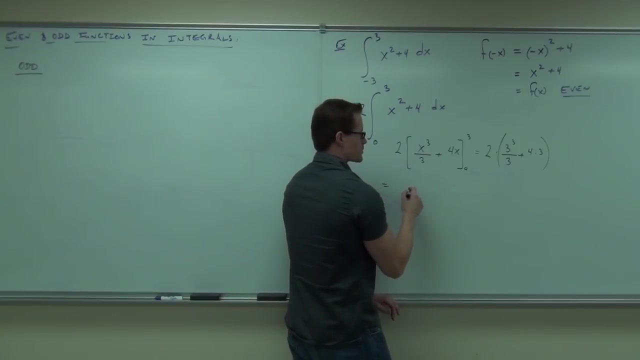 Well, plugging in the 0 is a whole lot better than plugging in that negative 3, huh, That's nice, That really is nice. Make sure you have parentheses there if you're going to do it. 9 plus 12 times 2,, 21 times 2,, 42?. 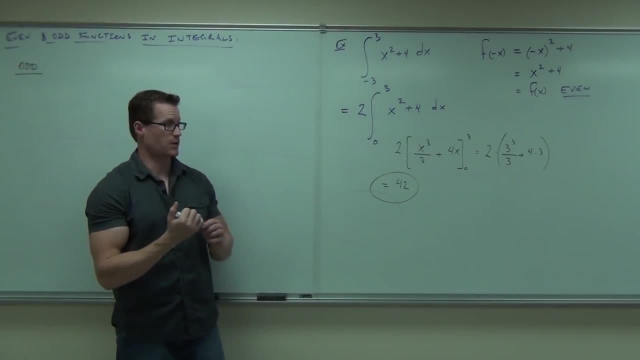 42.. Do that 42. At least I think it is. 3 cubed over 3 is 3 squared. 3 squared is 9.. 9 plus 12 is 21.. 21 times 2 is 42.. 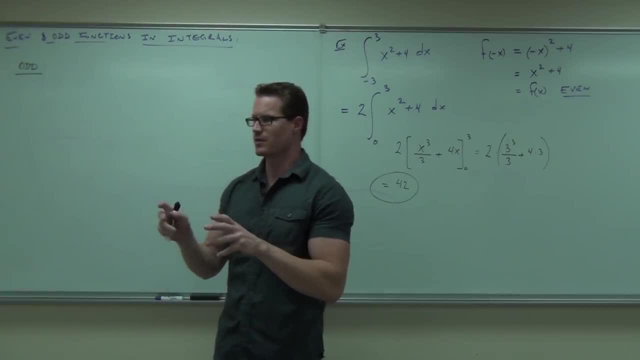 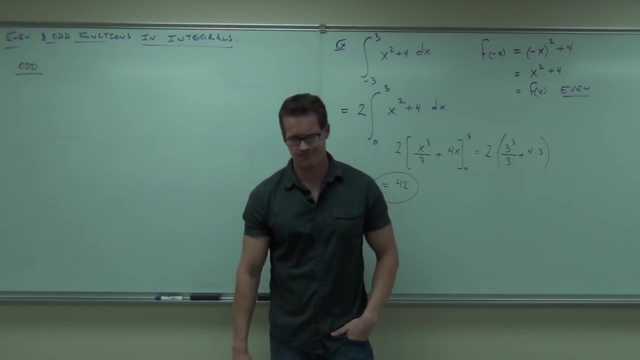 So cool deal. Did you get 42 as well? I did Awesome. So it makes it a little bit easier, since we're plugging in 0.. Now odd functions. What do you know about odd functions? Symmetrical. 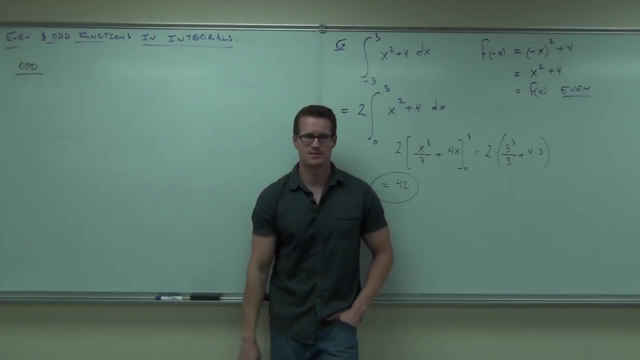 They are symmetrical, Very good. Across the y? No, No, that would be even Across the origin, Not the x. Across the origin. If they were across the x, it wouldn't be a function. Think about that. 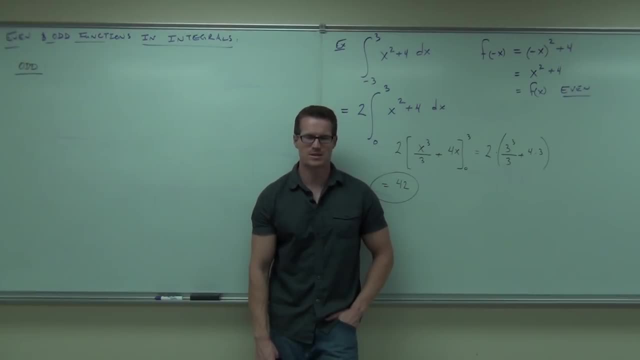 Across the y equals x. No, that's an inverse. Darn it, Darn it. What is this darn thing? I don't know. You guessed everything else. No, you haven't. Origin. Origin, Exactly right, It's symmetric about the origin, which means that it's a basic rotation of 180 degrees. 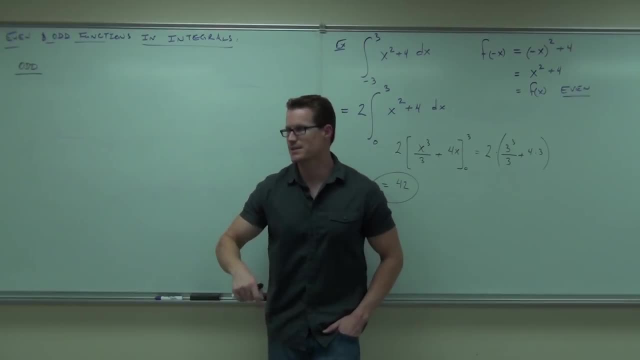 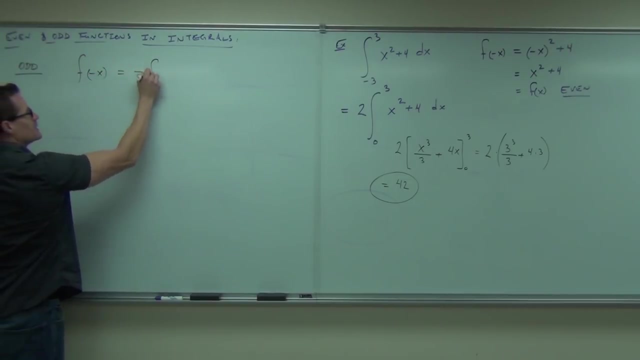 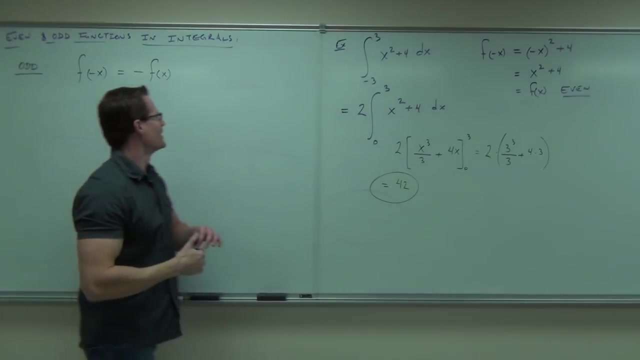 about the origin. So it says: well, it says this actually. It says when you plug in negative, you get negative of the function. So you plug in negative, you get negative of the function. It says this: When you plug in like negative 3, it's going to give you some value. 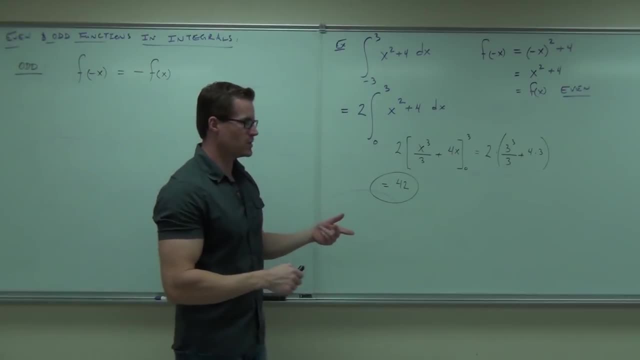 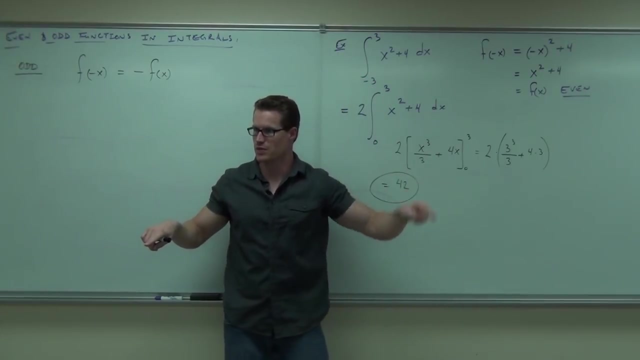 If you were to plug in 3, it's going to give negative of that value, So it's going to take it from up here and move it down here. That's a rotation of 180 degrees, or a what they call symmetric. about the origin. 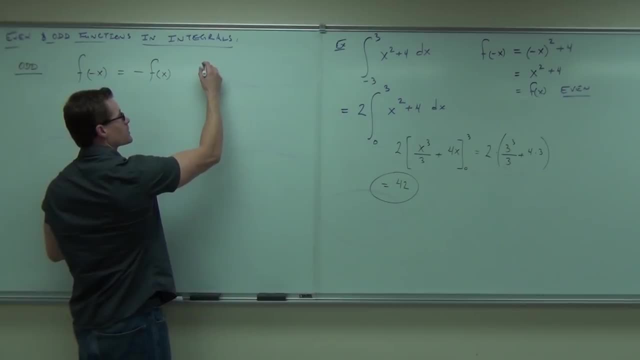 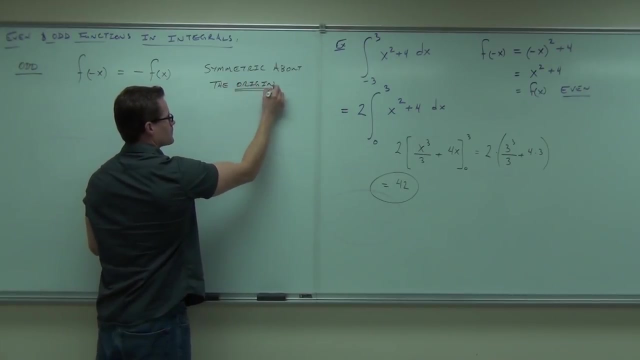 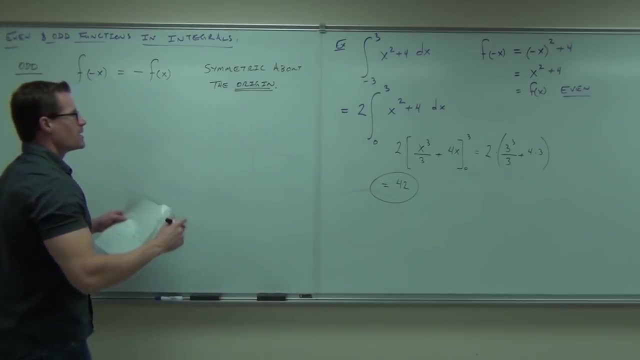 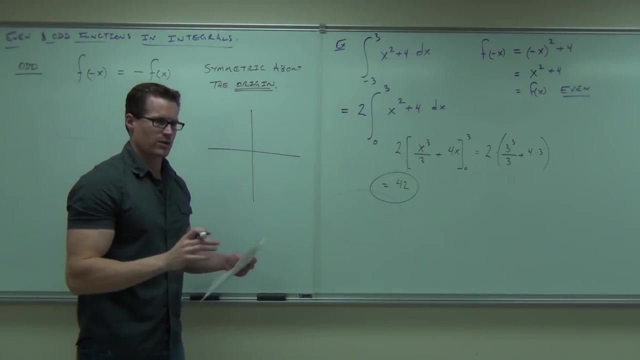 So that is the definition of odd And what it means. it is symmetric, But it's symmetric about the origin, Not in the axis of the origin. Let me give you the picture before I even do this. Here's what an odd function would normally look like. 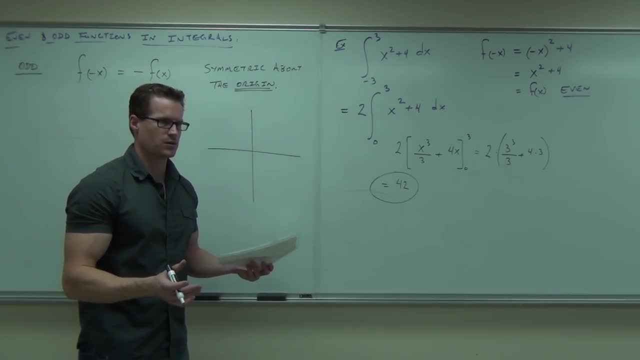 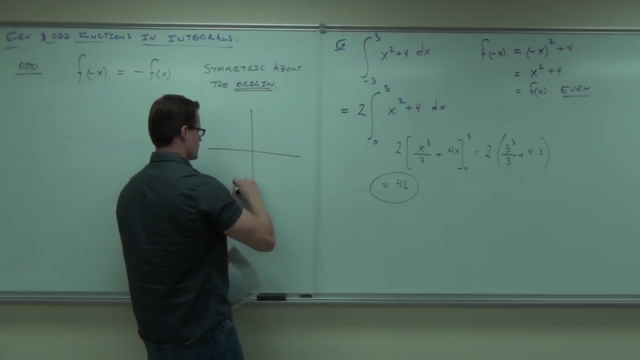 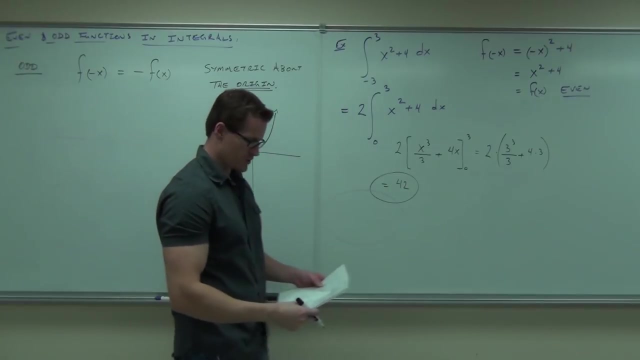 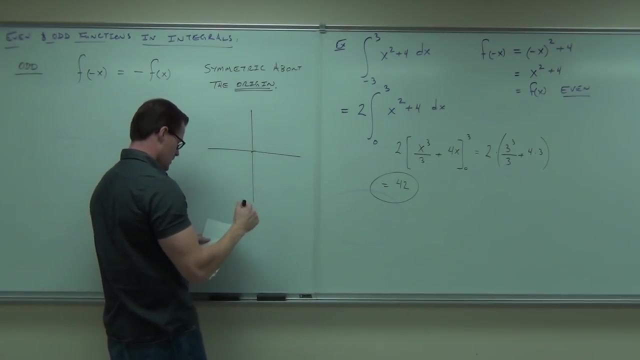 X cubed is an odd function. X to the fifth is an odd function. That's an odd function. Thank you very much. I know, You know what. Maybe I do it a little bit different here for you It's easier to see this way. 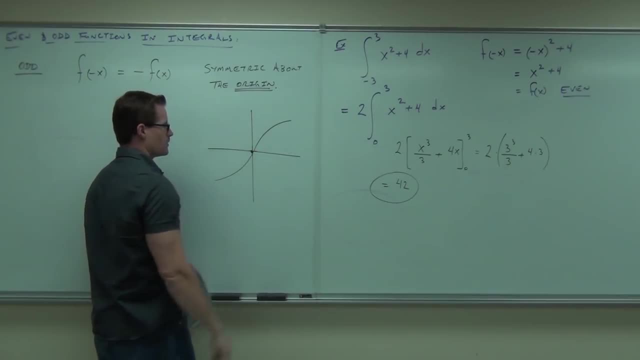 That would also be in. Let's pretend that's an odd function, A little bit easier to see here. Let's say I'm going from negative A to A. Tell me something about this area and that area If it's an odd function and symmetrical about the origin. 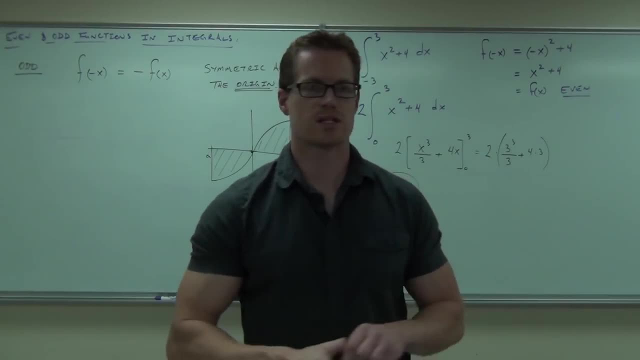 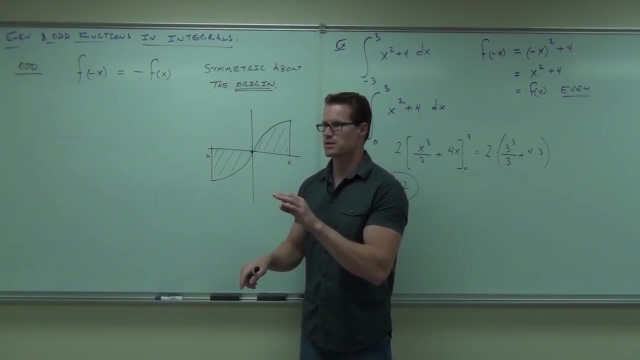 Tell me something about those areas. Wait, Explain something about the areas first. This and this: They are the same area. They are the same area. Would you agree on that? Since it's symmetric, they have to be the same. It's a rotation of 180 degrees. 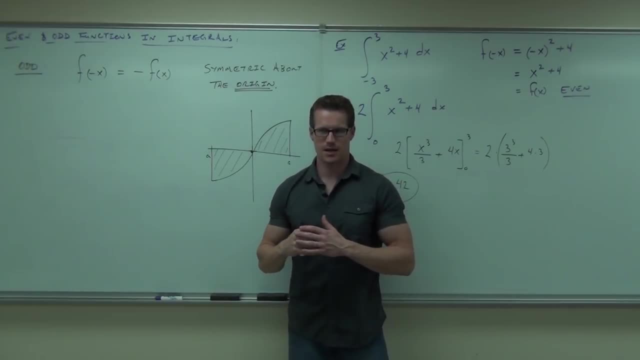 That is the same. Now tell me something about net signed area. Why zero? What net signed area says? take the area above and the area below- The area above is positive, The area below is negative- And see how much change you have. 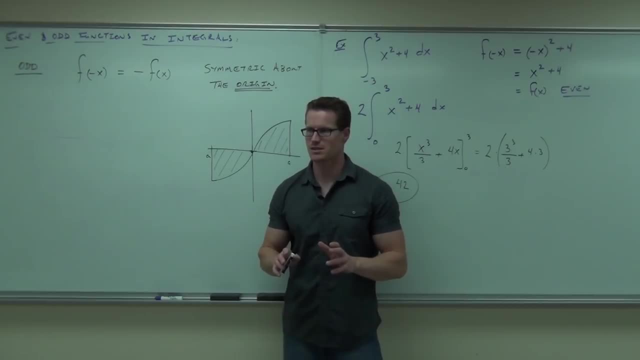 And the area would be zero. There would be zero net area out of this thing. Does that make sense? That would be for net area. If it asks for total area- total area- it would be exactly the same as an even function. 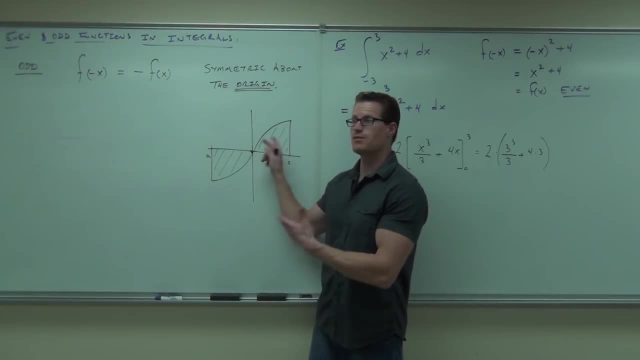 Double. Yeah, It would be this times two. Just like an even function was for total area. Now a definite integral does not automatically calculate total area. A definite integral automatically calculates net signed area, unless you have what in there? Absolute value. 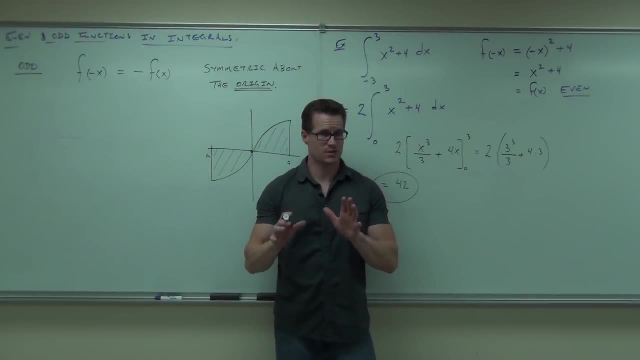 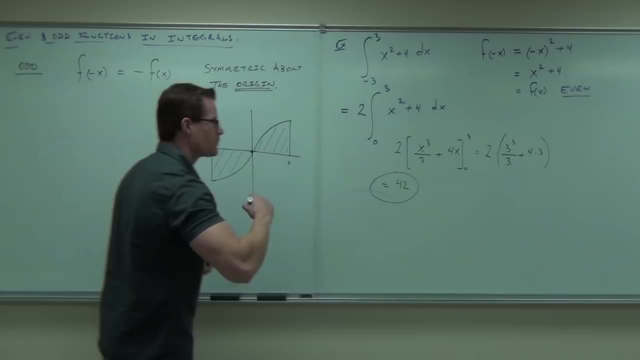 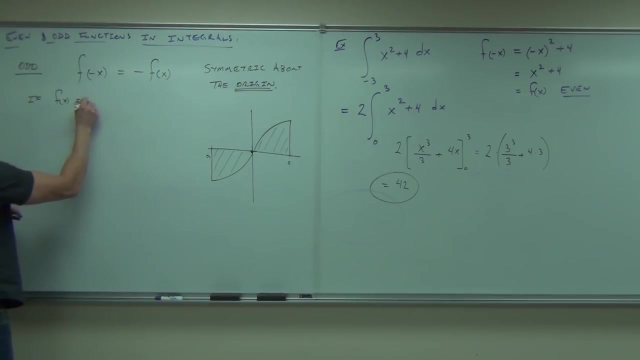 Absolute value. That's exactly right. So what this says: If your function is odd, An integral is going to calculate the net signed area. Therefore, if you have an odd function, If f is odd- And I'm going from negative a to a- 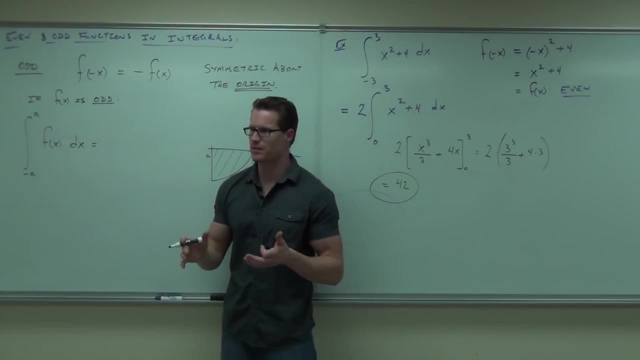 Notice that those numbers, they have to be the same. Do you see why they have to be the same? If I go just a little bit closer, Right here, Are the areas the same anymore? Clearly not, So they have to be the same. 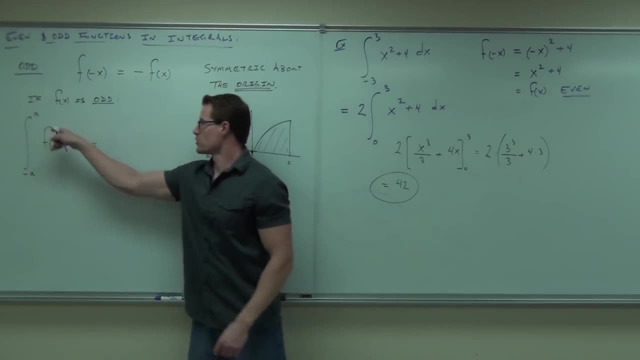 But what do you know If you're going to take an integral of an odd function Which is symmetric about the origin And you go from negative a to a Which says where you end is exactly the same, But opposite It means your area is going to be exactly the same. 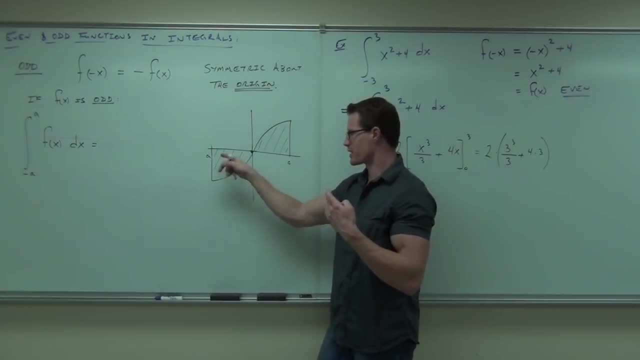 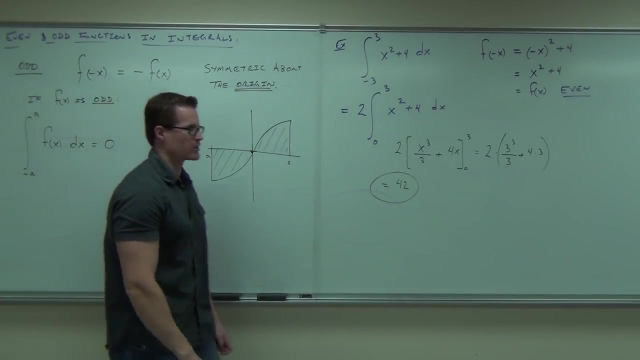 How much is that integral Two? Oh shoot, That's nice. Do you even have to do the integral? No, No, That's a beautiful thing, Not unless I ask you for total area. If I say total area, Then this is what it does. 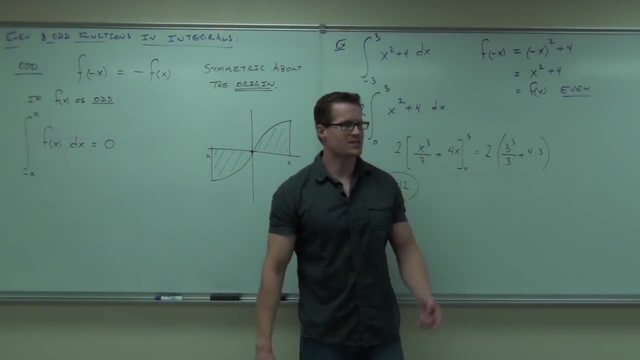 This is above and beyond what the book does right here. This is what it does. This is what it does. This is what it does, But if I ask you for total area, Then this is what it does. This is above and beyond what the book does right now. 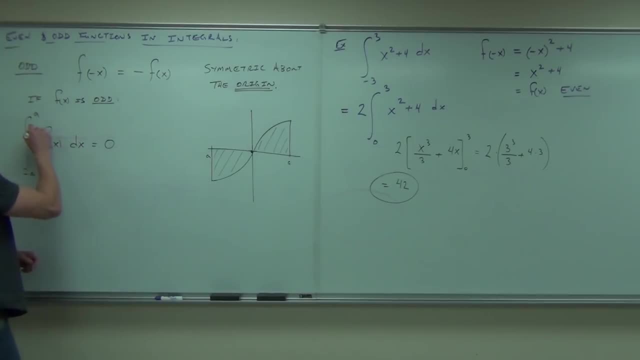 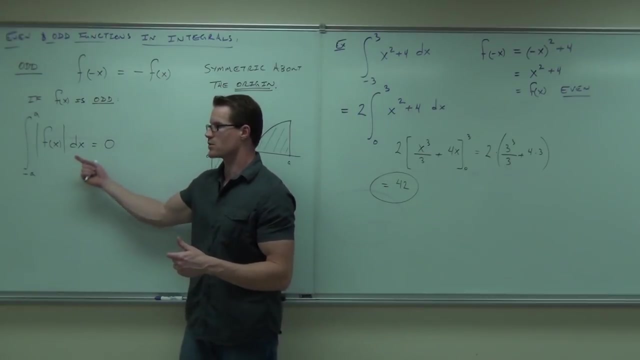 But if I ask you for total area, Then it would be this Right, And what that would be is Because they're equal areas. You'd have two times zero to a, Just like you had an even function It basically Think about what it would do. 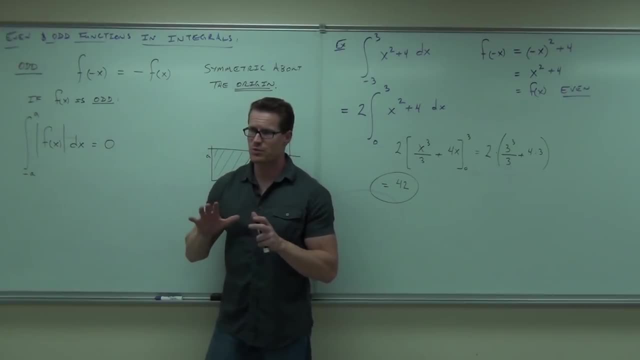 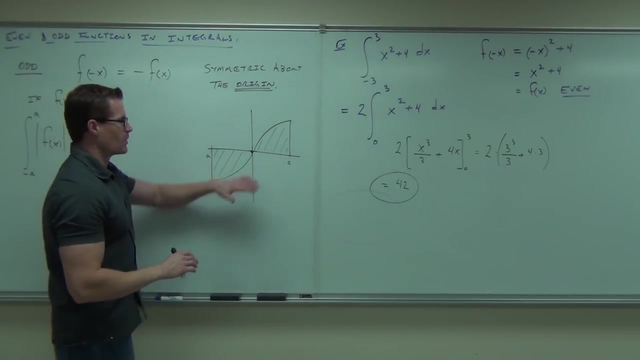 Just think for a second. What absolute value does? Absolute value pretends that anything below the x-axis is above the x-axis, Right? So absolute value? I hope this makes sense. Absolute value would go. Ah, What's that do? 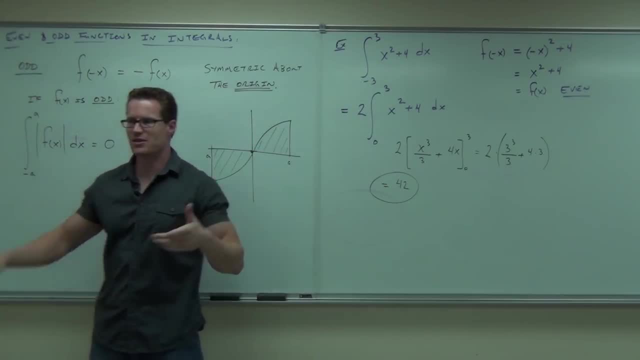 Changes from odd to even See it Kind of cool, right, And then you have exactly the same thing for even function. That would be for total area. If it's just like this, though, given to you just like that, that implies net signed area. 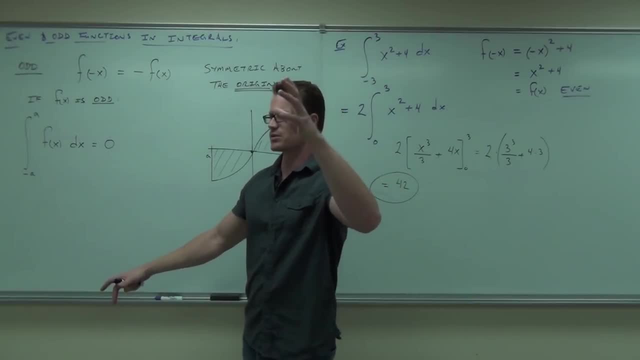 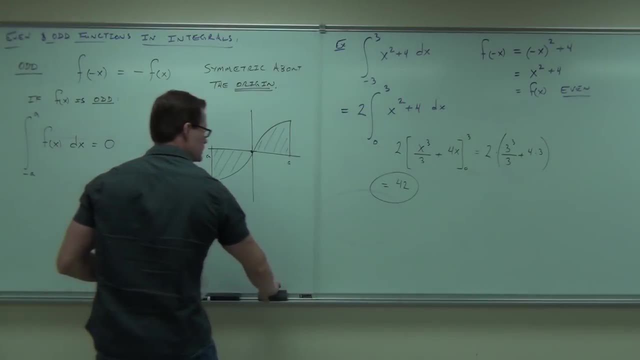 That means areas are the same, but on opposite sides of the x-axis That means the area is equal to zero. Hence the integral would be equal to zero. Would you like to see one application of this? You're going to like this. 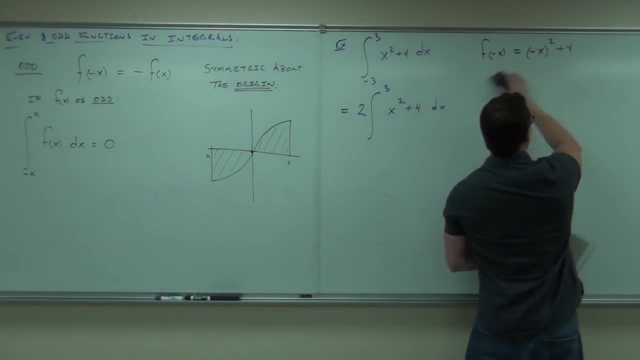 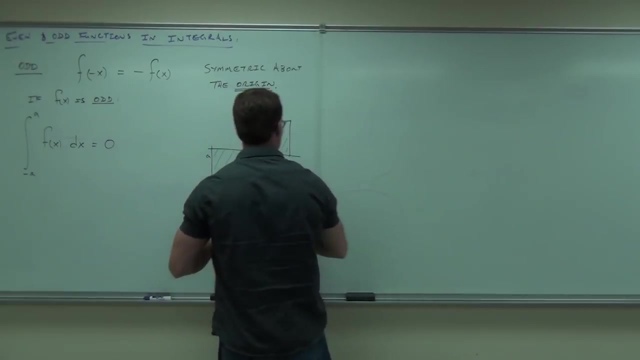 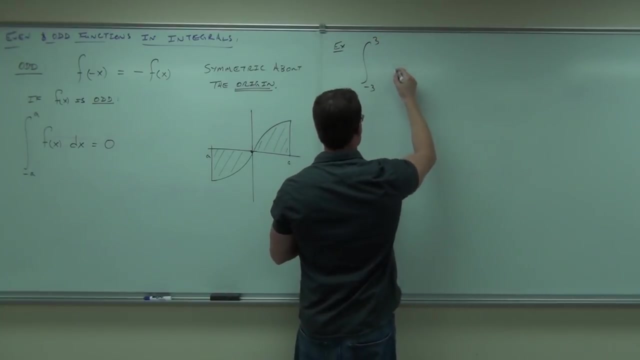 You're going to ask for 30 of these on the test. Well, maybe not, Maybe five. Are we going to get it? You can always hope. One question on this one. Expectation leads to disappointment. Give us a one-question test, though. 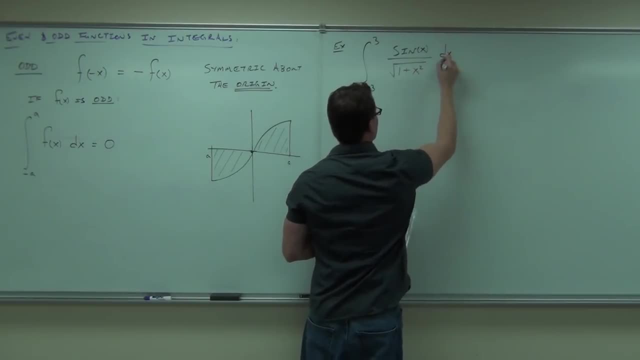 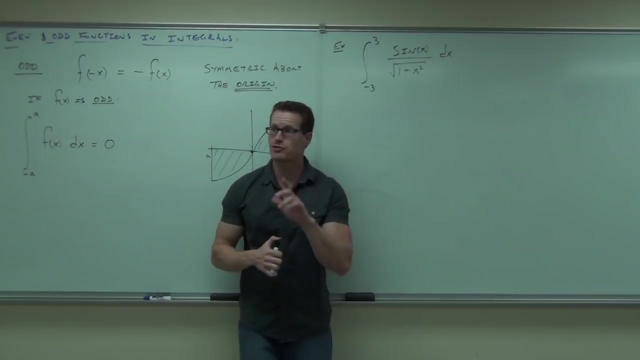 Right One person. Never mind, we lied, We don't want that on there, No, you don't. The thing about using these properties is that you have to prove that you can. You can't just say I think I can. 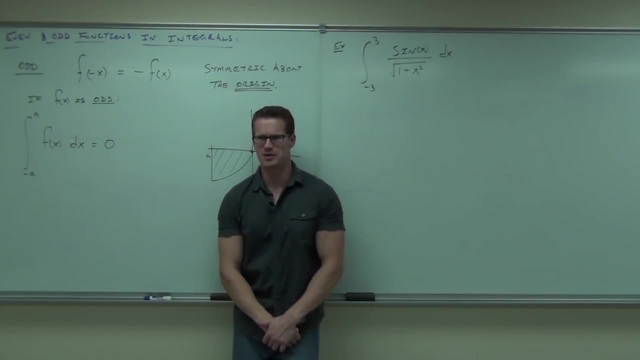 There we go, Because all of those would be zero for you guys. You'd be like, oh, negative, three to three, Zero. Oh I'm awesome. No, you're not awesome. Well, I mean you might be awesome, but not at that. 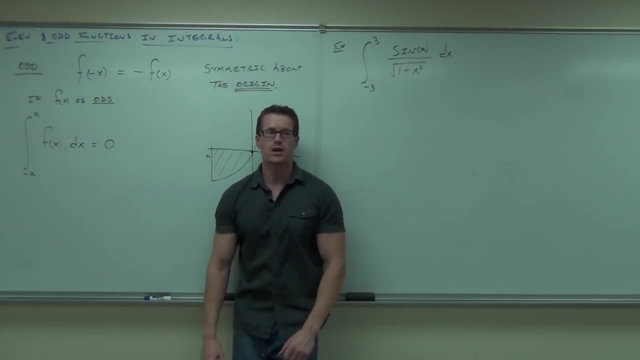 You've got to prove that it actually works, Just like you had to prove it was. even you have to prove this was odd. Now this says: I can do a lot of integrals that otherwise I couldn't do. Do you see why it says that? 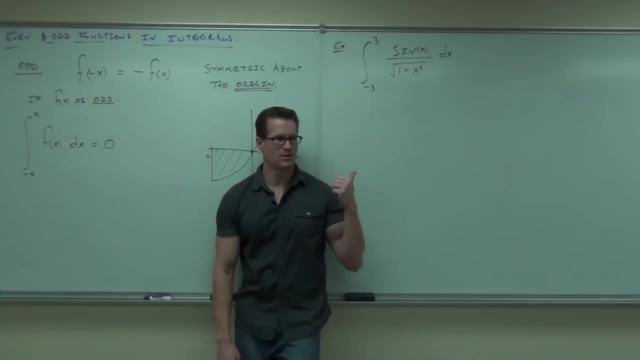 It says my gosh. I mean, do you know how to do that? Do you think that's true? I don't right now. I mean just looking at it. I'm thinking trig substitution, but you don't know trig substitution. 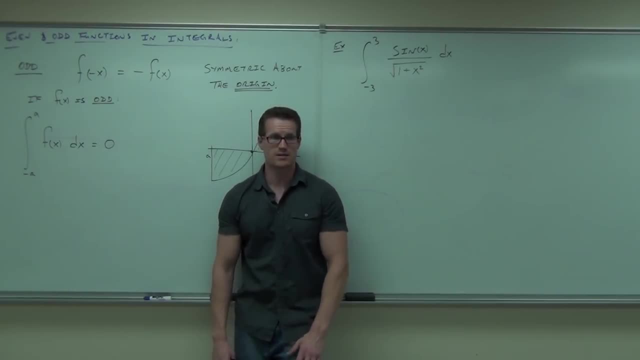 You know substitution, substitution, You know u-substitution, So that's off the table. No matter what you do with a substitution that is not going to work. Take the take: 1 plus x, squared derivative is 2x. 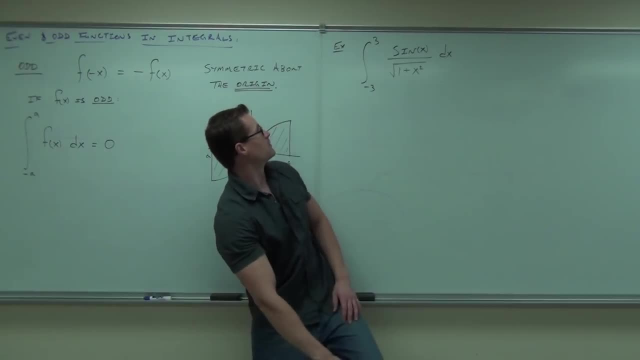 That doesn't appear, Take sine x. There's no cosine, You're stuck. The only thing you can do is say, well, it's going from negative 3 to 3.. Let's see if this is even. or let's see if this is odd. 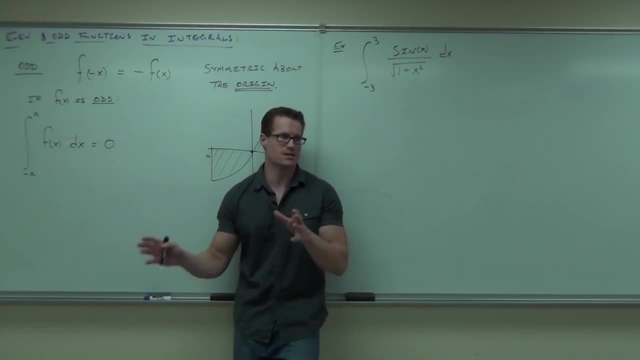 If it's even, we're probably stuck anyway because they still can't do the integral. Even doesn't get you away from the integral. It just says I can multiply by 2 and have a 0 in it. That's nice, Odd. gets you away from the integral. 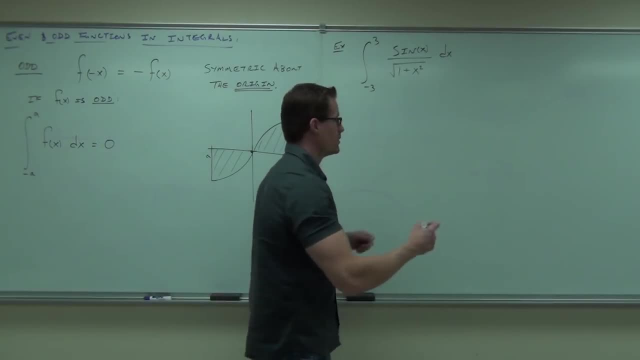 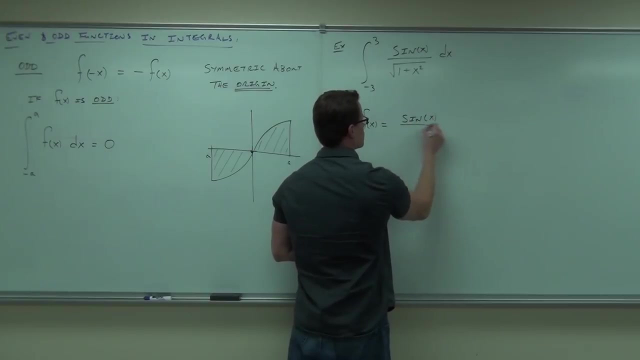 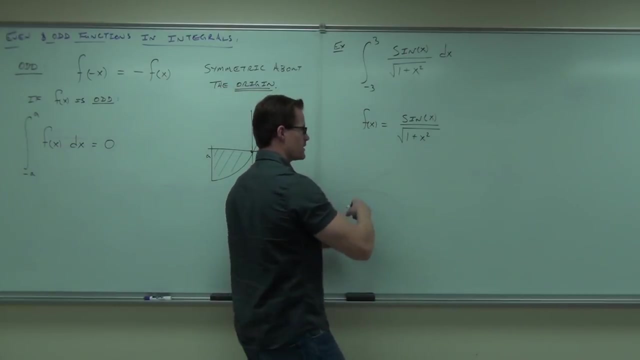 That's even better. So let's try to see if this thing is odd. What you do is you start out with your function. That's what we're trying to get to. but maybe you have a negative And you say: what I want to have is I want to plug in negative x. 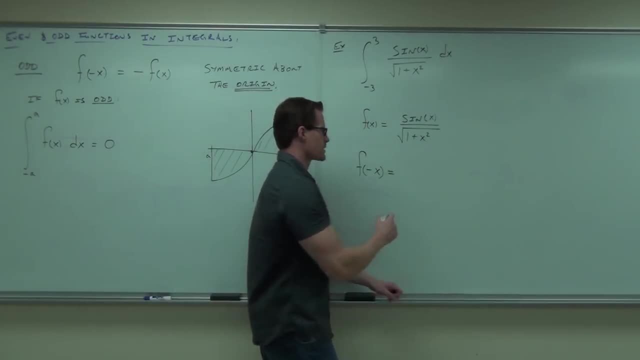 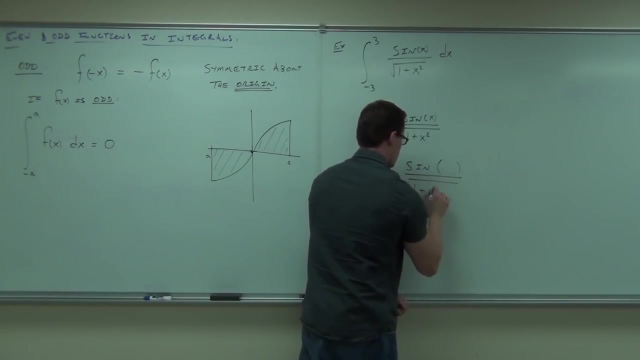 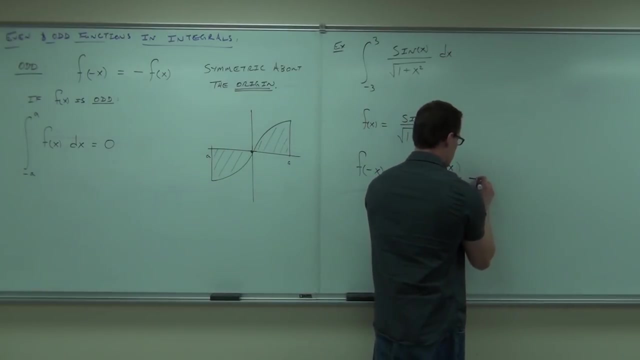 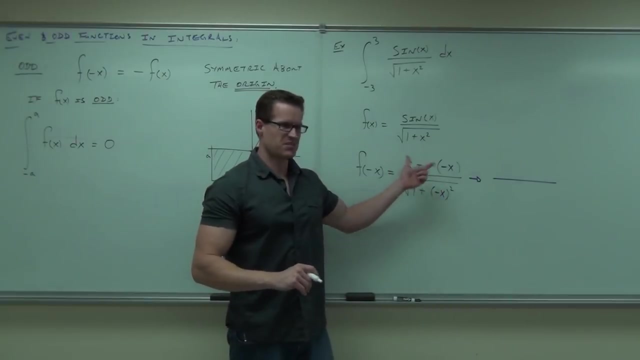 and let's see what it does for us. So take everywhere you see x And see what happens. So negative x, negative x. Well, if I do that, this actually isn't that. it looks bad. It's really not that bad. 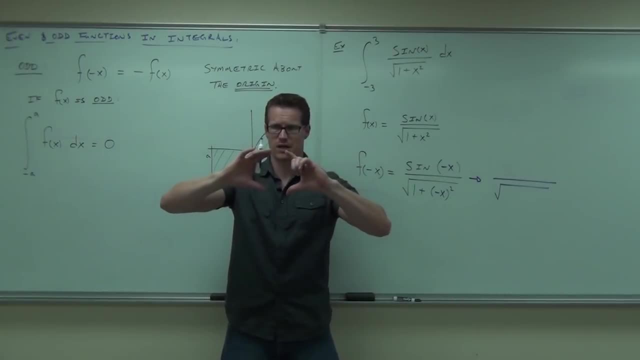 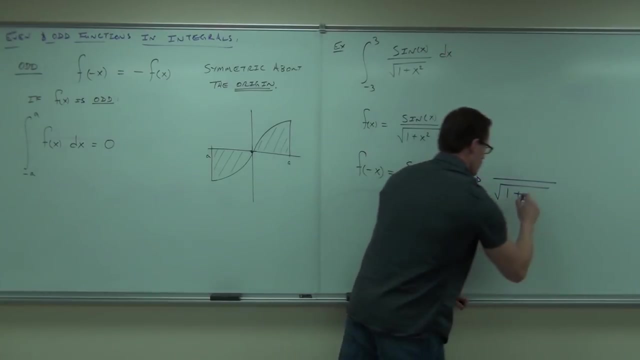 Square root of 1 minus, or sorry, 1 plus negative x squared. How much is that? Wait, minus x squared or plus x squared? Well, it's minus x squared, Okay. Does anybody remember anything about sine of negative x? 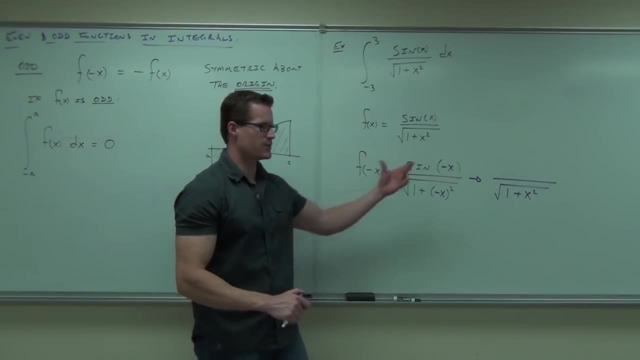 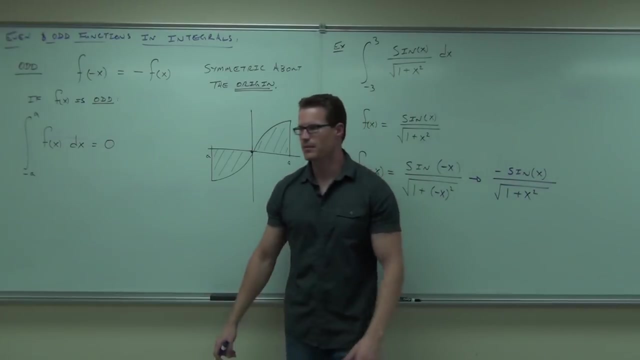 Negative sine of x. Yes, that is a property It says. It says sine of negative x is the same as negative sine of x. If you don't believe me, look it up. That's a true statement. Sine is, when you think about it, an odd function. 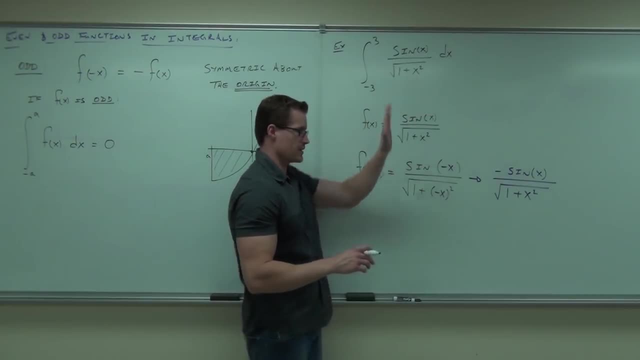 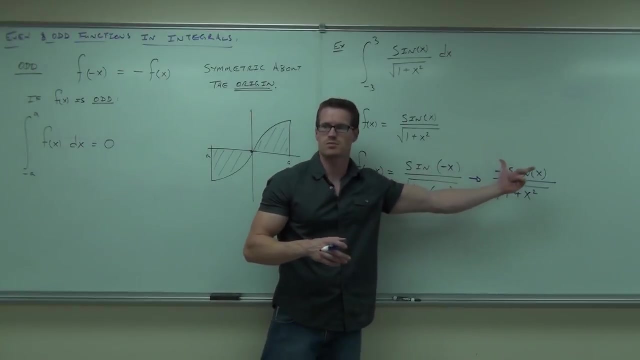 It is inherently an odd function because it does this and it does that. It's symmetrical about the origin, right? So knowing that sine's an odd function says this absolutely must be the case, right there. Sine of negative x has to be negative x. 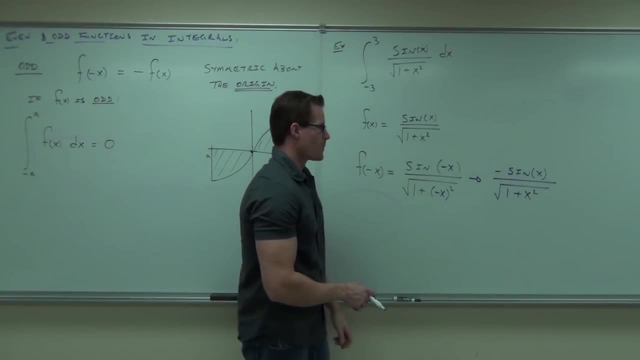 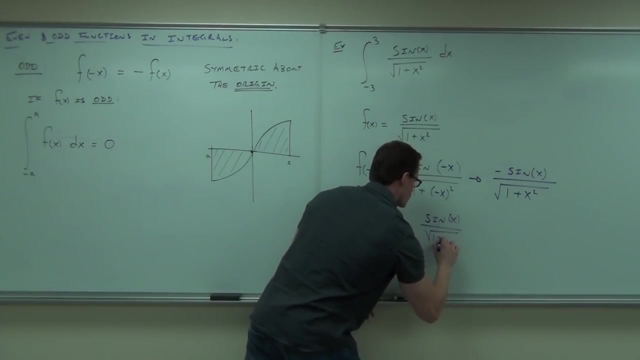 Sine of negative x has to be negative sine of x. It will work out for you. So that's true. Well, look what we can do. This is equal to negative sine x over the square root of 1 plus x squared. 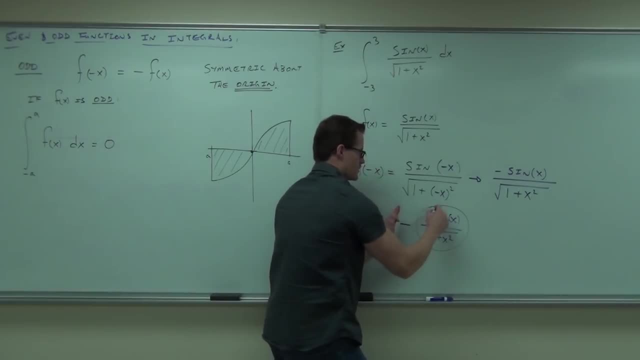 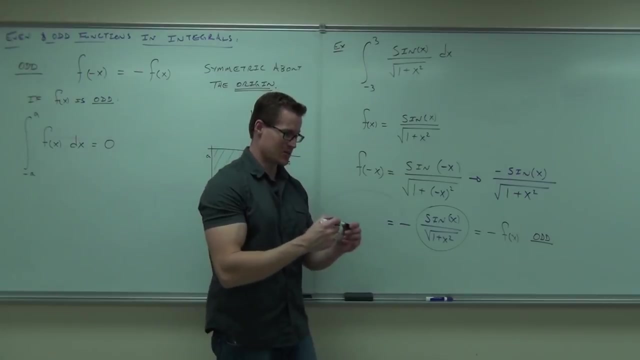 Yeah, This is this right here. this is f of x, So this is negative f of x. So right there, is it odd or not Odd? If this happens, it's definitely odd. Well, it's not so odd, which is awesome. 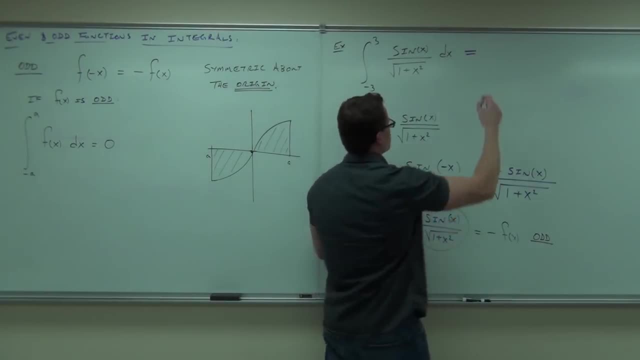 And then we can just do this and go. how much is the integral? Zero, Zero. Sweet Didn't even have to do it, It's zero. How many people understood what we talked about today?